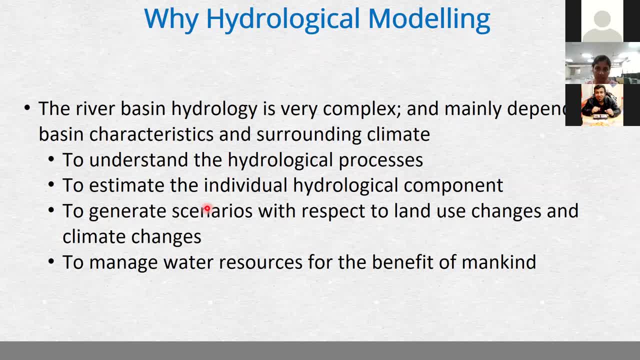 process. we need to do some type of modeling to estimate the individual hydrological component. we do that to generate the scenarios with respect to land use changes and climate changes and to manage the water resources for the benefit of mankind. So suppose, if you want to build a dam, 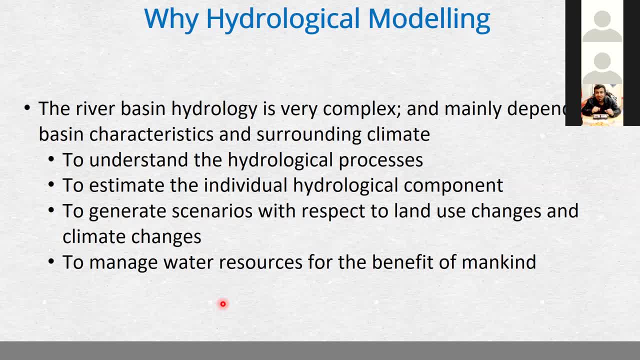 which is just a very basic idea of any hydrology or water resources field. So, in order to build a dam or a reservoir, we should have a proper understanding or a proper, you know, evaluation of how much amount of water is entering to that particular ecosystem or that particular. 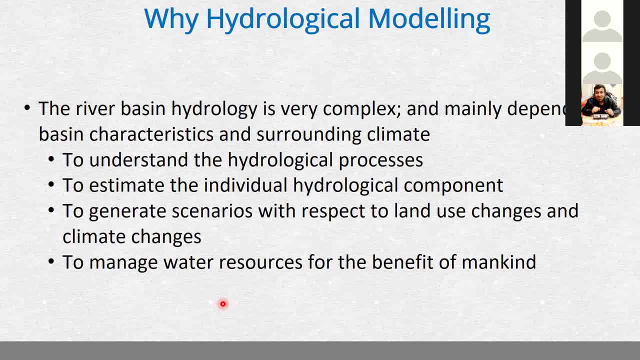 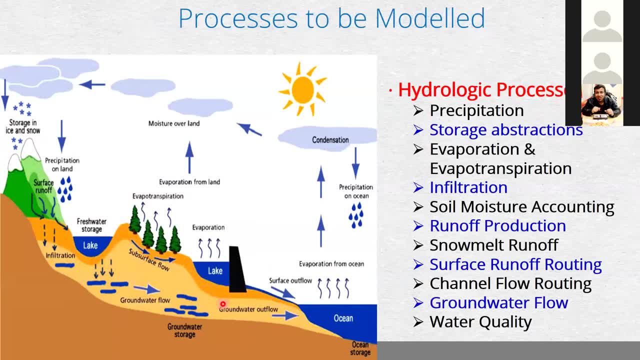 outlet or to that reservoir. So for that purpose, in order to estimate that particular amount, we generally do the hydrological modeling. So when we talk about the hydrological modeling, it is not only about the runoff or the rainfall, it is about all the parameters that are present. 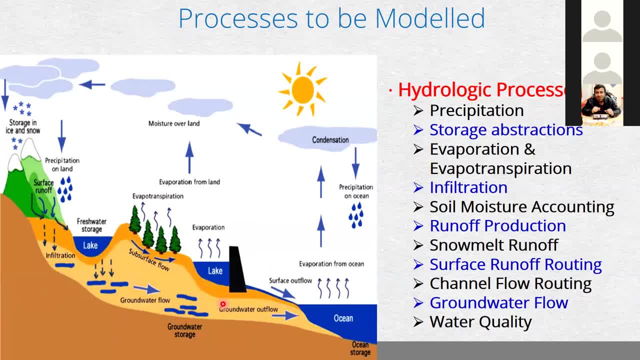 in this form of water, either through precipitation, or we need to get the storage extraction that how much amount of water is actually going to the groundwater or infiltrating. then the amount of evaporation, evapotranspiration, which is very much useful in the 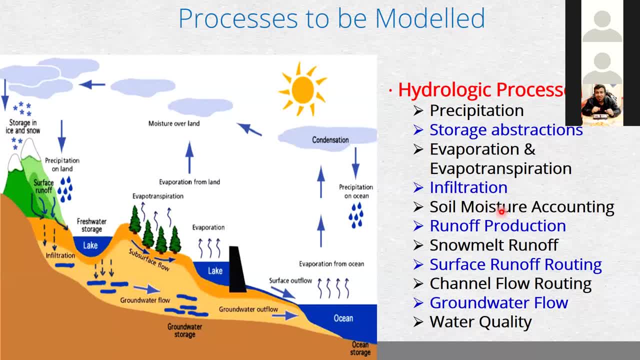 evaluating crop water demand. then we have soil moisture accounting, then we can do runoff production. we can get the snowmelt runoff because in the hilly region, like the Himalayan region, all the Himalayan rivers, like Tanda, Brahmaputra, they not only get the water from precipitation and base flow. sorry, but they also have a water supply system so that they can get the water from the soil and they can get the water through the dam. then they can get the water from the wastewater and then they can get the water through the water from the dam. So in other words, 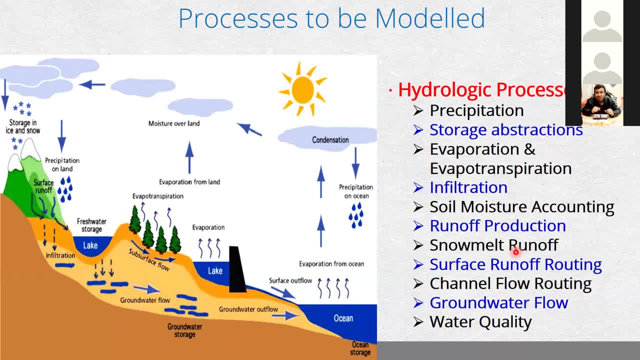 they can get the water from the dam and they can get the water from the water from the wastewater. sorry, but they also do get the water from the snow melt and the glacial melt. then runoff routing, channel flow routing, groundwater flow and the water quality modeling also. 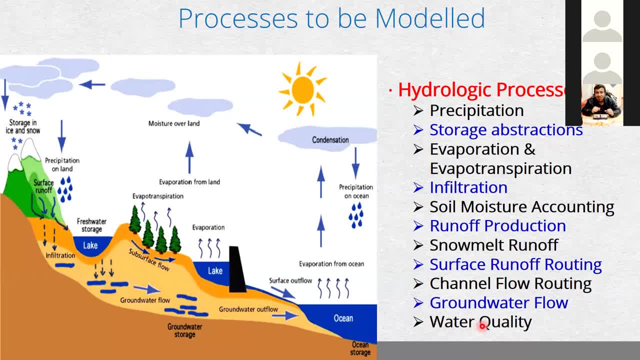 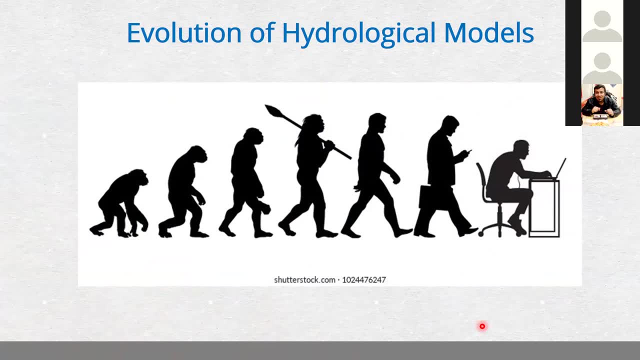 So there are n number of things that can be done within this hydrological cycle. So presently we are talking about the hydrological model. So from very beginning to at the latest stage, we have seen a various amount of advancement in the field of hydrological modeling. 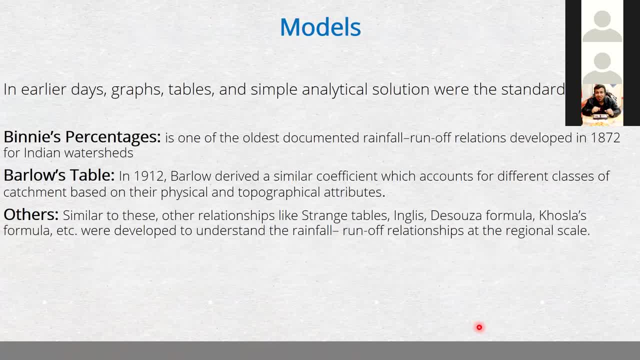 So, as we talk about the very first or the in the earlier days, what was happen? or what? the analytical approach that the previous people adopted to model the hydrological cycle? So initially in 1872, a Binney's Table is get introduced and it is one of the oldest. 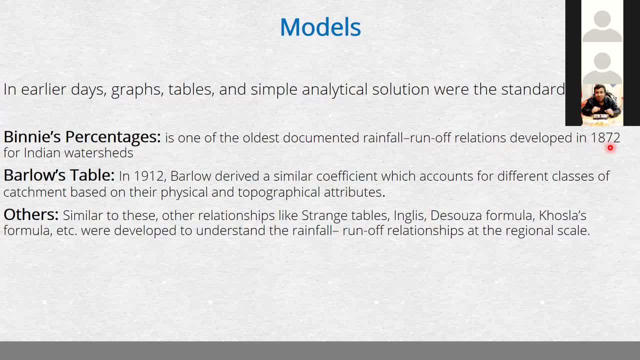 documented rainfall runoff relationship that developed in 1872 for specifically Indian watershed. After that the Barlow's Table Invented in 1912, after that some of the similar approaches, just like strength tables, English formula, D'Souza formula, Koestler formula. 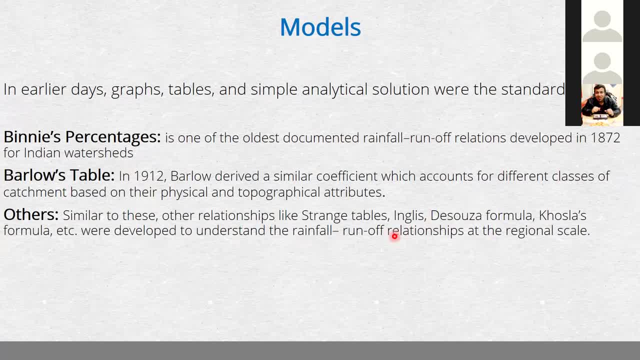 So all these are developed in in estimating the rainfall and runoff relationship. So in all of these equations or in all of these formulas, we get a: simply give the amount of rainfall as an input and we get the amount of runoff fall as the output. 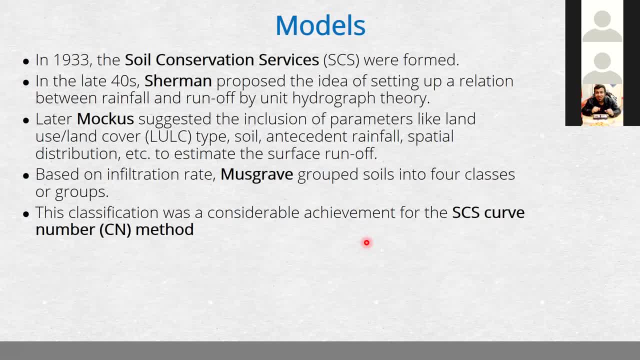 But later on, at the later stages, Some of the agencies and some of the ideas came up that why include only the amount of rainfall? Why not We use the land use land cover? Why not We include the soil moisture? Why not? 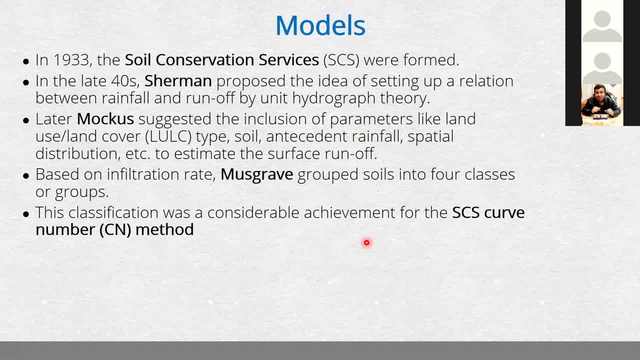 We include some other parameter in generating the runoff. So on that basis in 1933, organization named soil conservation services performed. It is an US based organization and in this organization in forties Sherman, a scientist had proposed That 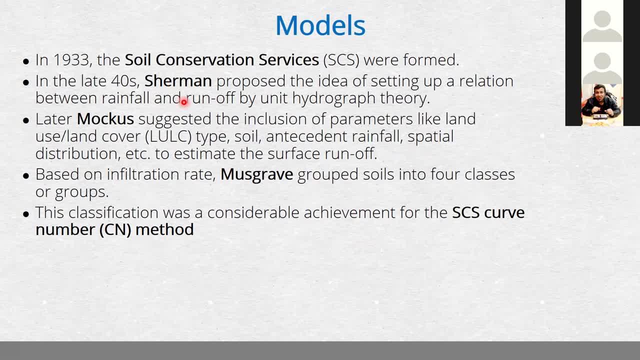 There is a definite relationship between rainfall and a runoff by a unit hydrograph theory. So later on the mockers suggested to include certain parameters like land use, land cover, soil moisture, or we can say soil type, soil texture, antecedent rainfall and the spatial 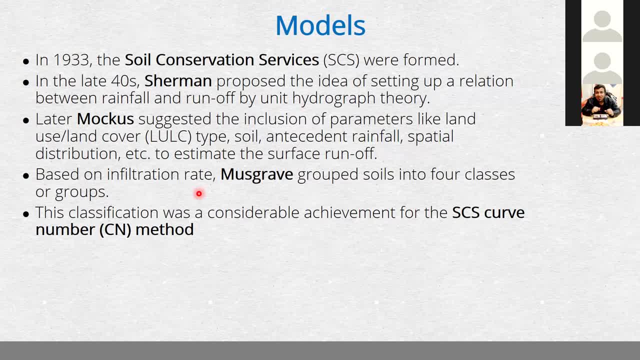 distribution of rainfall. in estimating the surface runoff And based on the infiltration rate, Musgrove and other scientists grew this soil into the four classes. So after each of these evaluation steps we get a technique known as SES, curve number technique. So these techniques actually develop on the basis of all these parameters. that first of 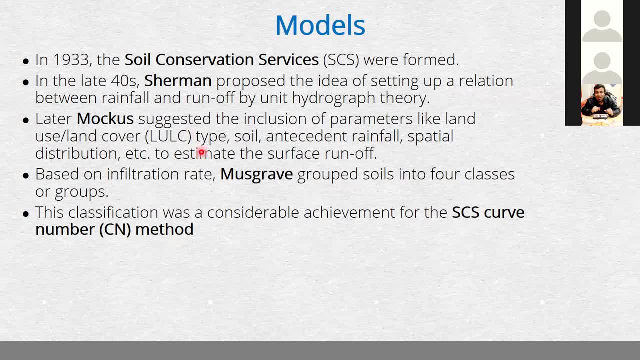 all. we include the rainfall, Then we include the land use, land cover, We include the antecedent rainfall, soil texture, et cetera, in order to get rainfall runoff model. So, um, why we are talking about this? 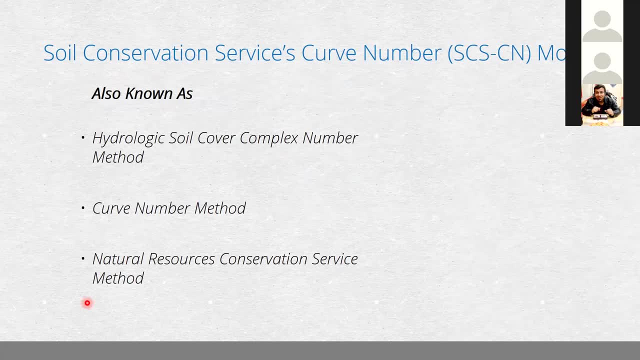 We are talking about the SES curve number, because this is the technology that is widely used in the field of hydrological domain, uh various uh advanced hydrological model, either HMS or SWAT model. So uh, most of the hydrological advanced advanced hydrological model adopt the basic. 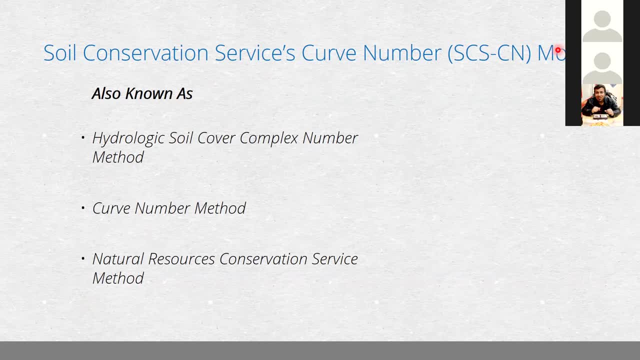 soil number, uh, soil conservation, SES, curve number technique. So it is a very uh, highly uh, very complex number of methods. Uh, it totally depends on the curve number And it is definitely a very complex number of methods. 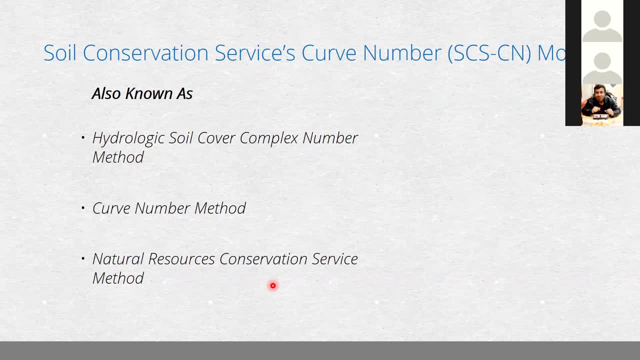 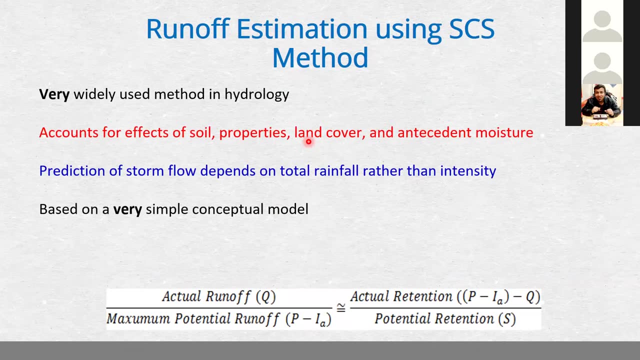 Uh, it totally depends on the curve number. So it is developed by the natural resource conservation service method. So, uh, it is a very widely used method. in the field of hydrology It accounts for the effects of soil properties if lands cover and antecedent moisture and 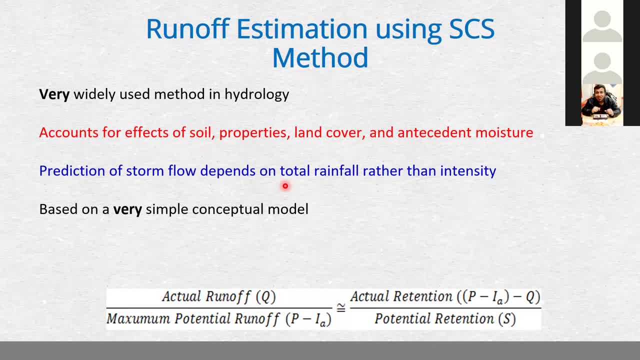 the prediction of storm flow depends on the total- or not- standard than the intensity, because most of the models, or most of the techniques, are dependent on the rainfall intensity. But this model is depend on the total amount of rainfall, not the intensity, And it is based on a very simple example. 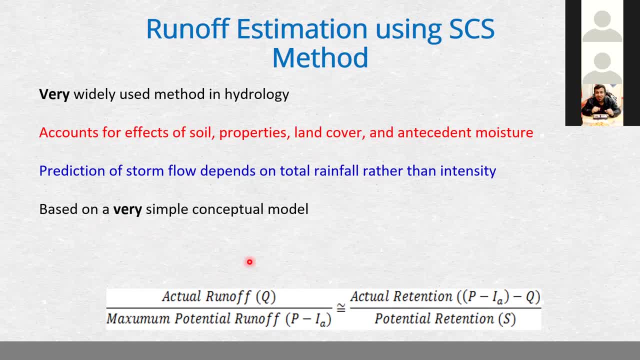 So the model, the HMS and BLS model, uh, in the field of hydrology it's level of rain flow is different- and conceptual model. So this is the simple formula that were adopted in calculating the amount of runoff using the rainfall. So this is the formula in which actual retention is. 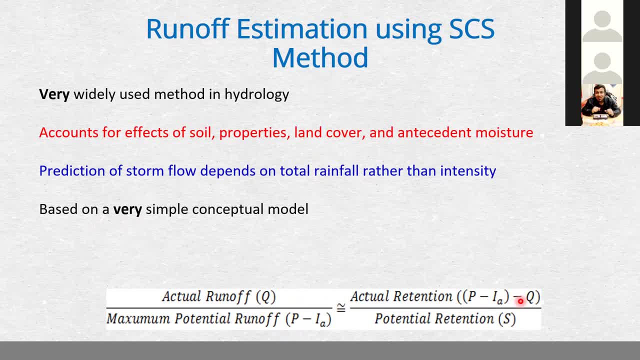 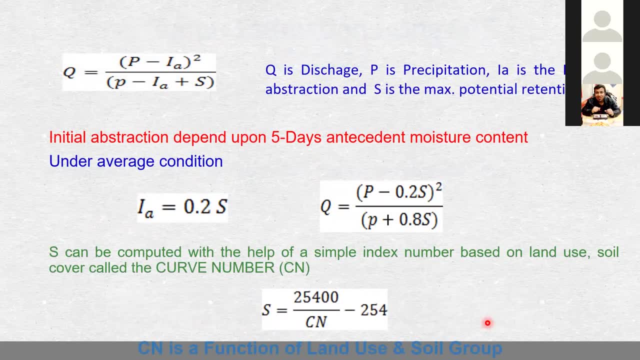 equal to P minus Ia minus Q, and we will just talk about in the next slide what is actually P and what is Ia and what is potential retention. So generally, Q is the discharge, which is the our ultimate output. P is the precipitation, Ia is the initial abstraction and S is the maximum. 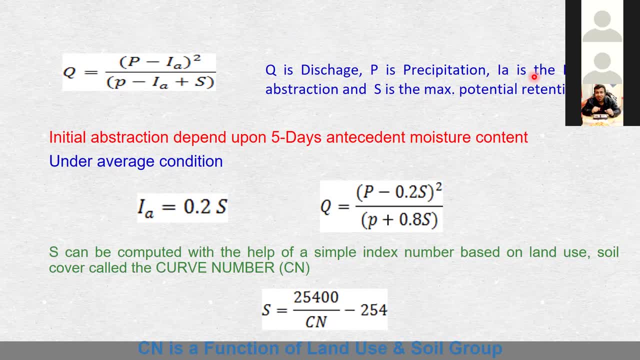 So Ia that means initial abstraction, means when the water will fall on over a ground, so some amount of water will infiltrate downwards and it totally depends on the LULC. that means land use, land cover and soil type. So inclusive of these parameter will definitely generate a Ia and S for 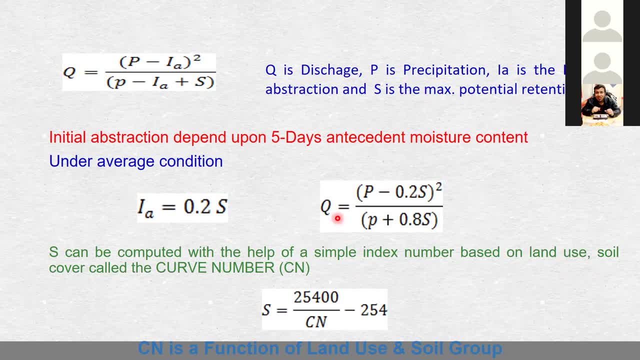 that particular ground And on that basis the final equation come up, as discharge is equal to P minus P is nothing but the precipitation minus 0.2 S and the precipitation plus 0.88 S, and where the S is depend on the curve number, and this is the formula for the S. and so ultimately we get the one thing that 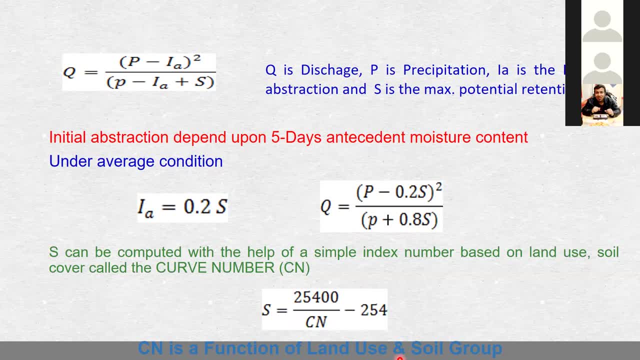 curve number is a function of land use and soil growth. So if land use or soil is changing, curve number will change. if the curve number will change, the S will change. And if the S will change for the same precipitation, the runoff will definitely change. 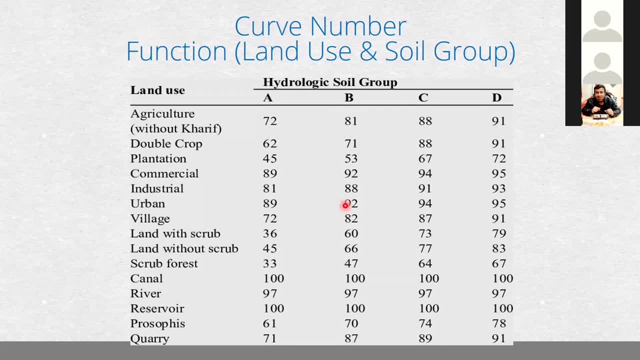 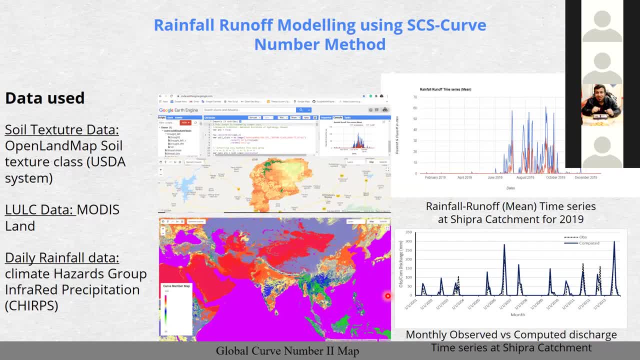 So in this method we have used the three datasets: first is soil texture dataset of open land map, soil texture UST system, then we have used the LULC dataset of MODIS and then we have used the Daily Run of Fall datasets of CHERV. 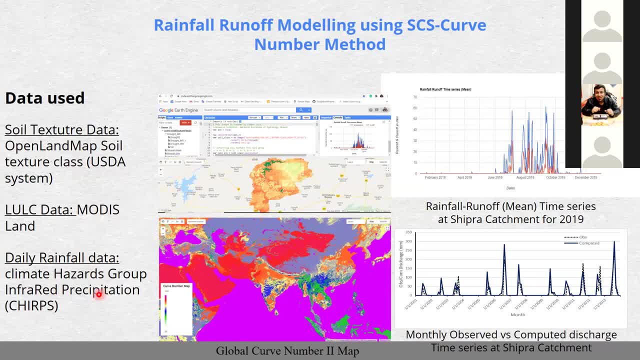 that means Climate Hazard Group Infrared Presentation. So and when we have write this script of combining this dataset and calculate the global curve number and harness the global curve number maps to estimate the rainfall uh runoff time series for that particular area, and not only that, we have compared our uh. 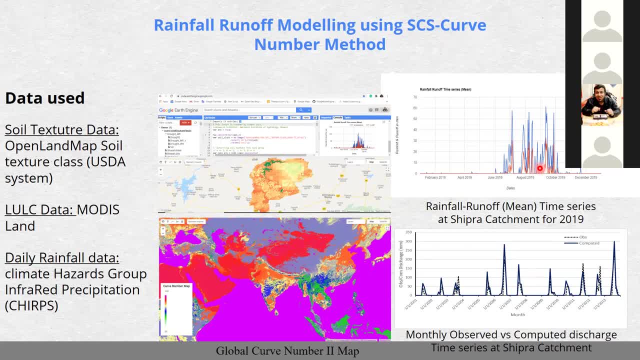 the result from uh, the ground station. that means gate discharge data and when we have found very good interpretation uh in the monthly observed and computed discharge data, at particular not only shibra, but we have performed this study in different parts of india and three to four basins. 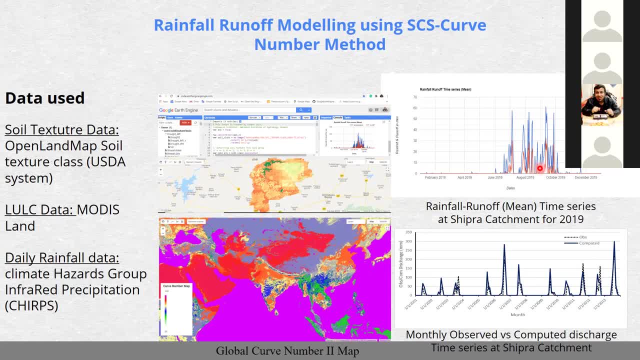 uh, at the end of the session, i will uh give you a link of the paper that we have published, through which you can get the details of these models and you can compare your result for your own area also. so, uh, the thing that i have told you in the presentation, that very good thing about the 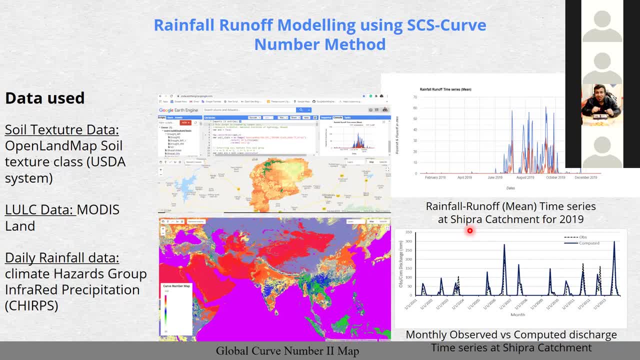 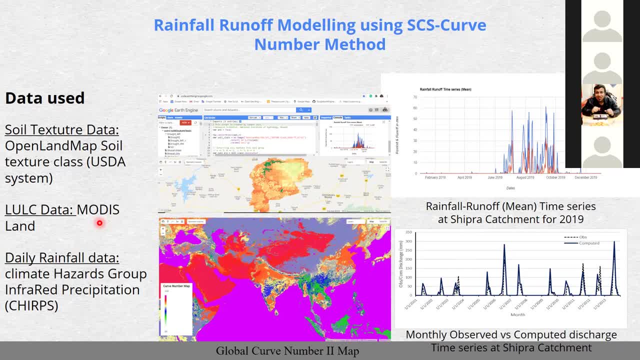 or not perfectly rely on this modest land cover, Then you can prepare your own land use land cover and ingest it and use this product in the countable material. For example, you don't want to use the rainfall data from Chubbs. You want to use the rainfall data either from TRMM 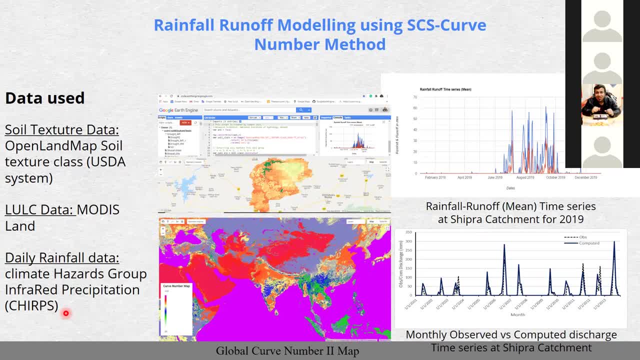 or you want to use the rainfall data from the IMD source, Then you can ingest your data in the Google Earth Engine and you can utilize this product either in either with any data or for any area. So let's proceed to the hands-off session. 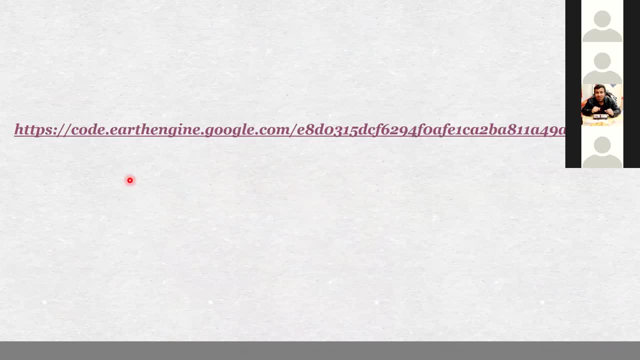 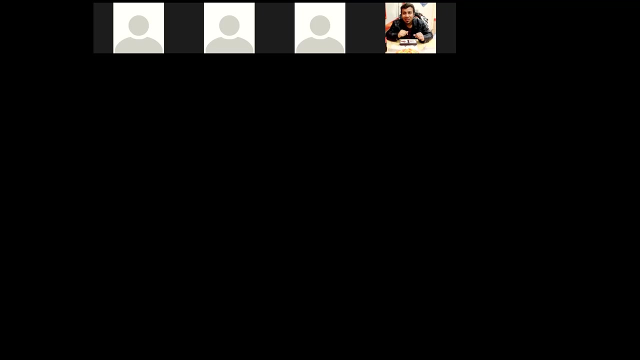 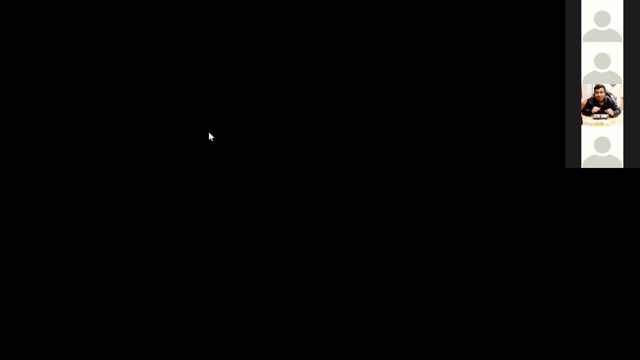 So this is the code for which I'm going to use. First of all, I'll just open the link and show you the product that we are going to demonstrate. So when I click the link on the PPT I, my system opens this web page. 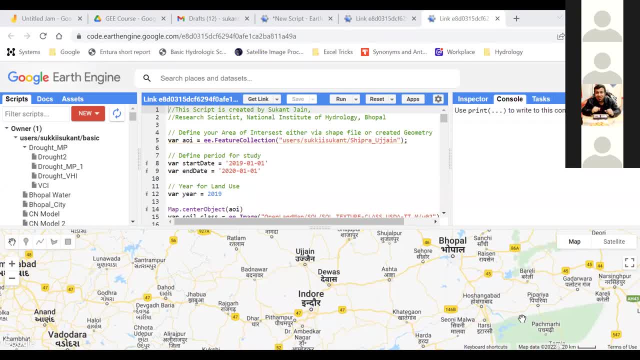 and this is the Google Earth Engine platform in which the script is already there, because I have saved my data set And if I just click on the run and wait for a few seconds or a few minutes, it will show me the data set that I have saved. 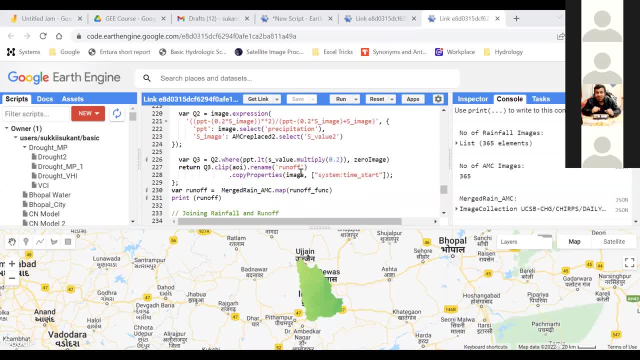 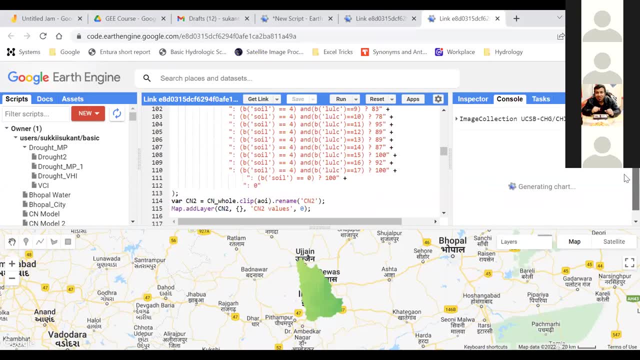 So this is the data set that I have saved And if I just click on the run and wait for a few seconds or a few minutes, it will show me the data set. And if I just click on the run and wait for a few minutes, 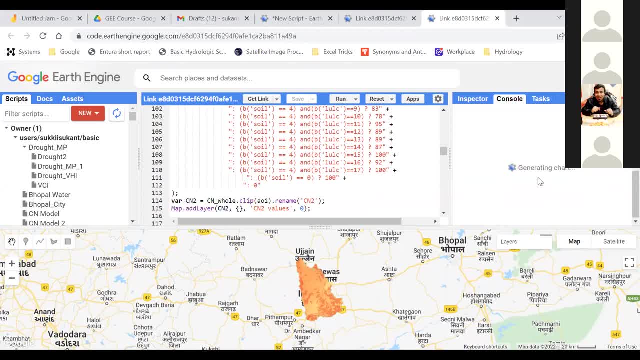 then I get it is actually generating. then I get the rainfall runoff model for the Shipra basin And the result can be in the form of maps. You can see there are different types of maps, like combination of soil, curve, number two maps. 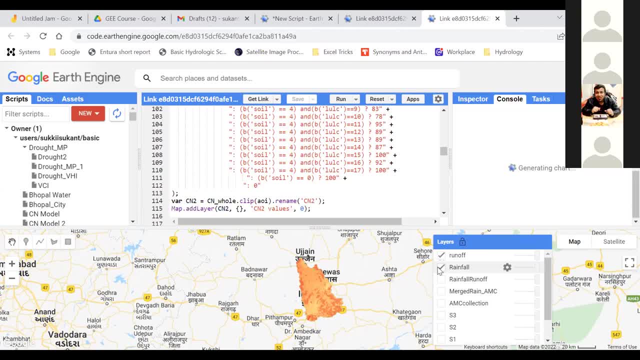 S1,, S2, S3 maps for different EMC, then rainfall runoff maps, separate maps are also there. But the ultimate goal is to get the chart And in preparing chart it will take some few amounts of, I say, one or two minutes to get the data set into a screen. 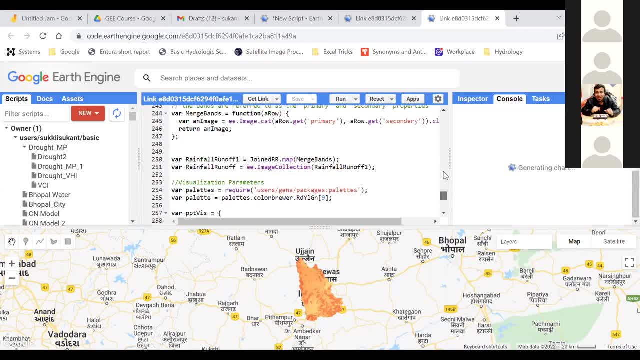 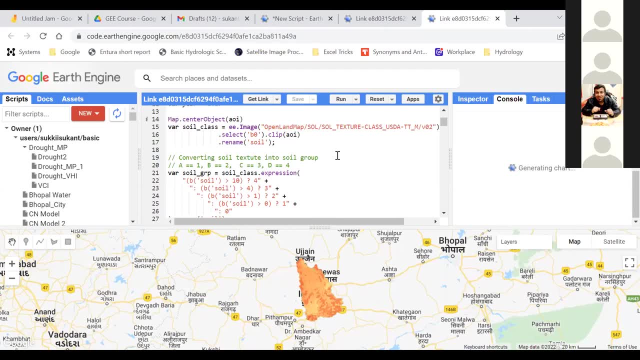 So this script has been returning over approximately 300 of lines. So at the end of this session I'm going to share you with the script- Actually, it is already in the GitHub or in the paper- but our objective for today's session is to go each component of this script. 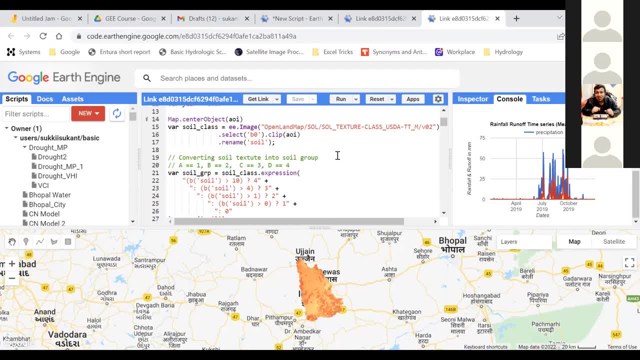 so that you will be getting the data set. You will get the understanding how the Google Earth engine and this model works to get the required amount of data set. So you can see there is a chart has been developed. I just click to open this chart. 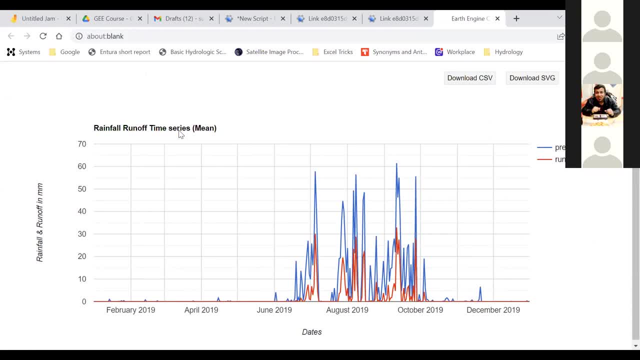 Now you can see, this is the rainfall runoff time series from the month of January 2019 to December 2019.. And in this chart we are actually comparing the runoff rainfall in the blue line and the runoff in the red line And in the MM. 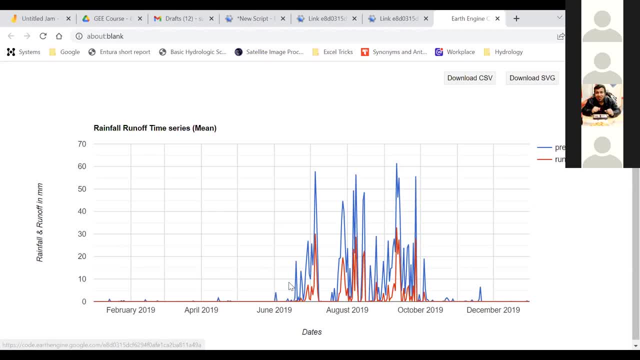 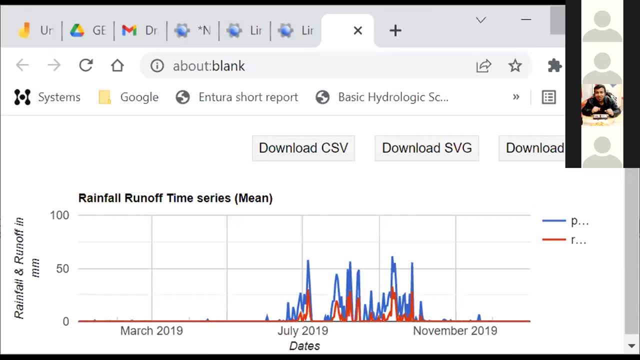 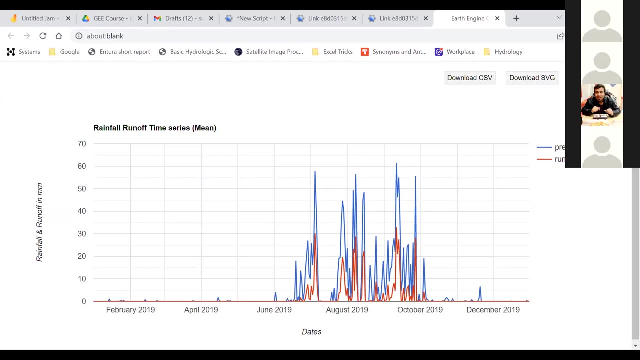 and you can download this chart in the format of CSV. That means you can download the data set in the CSV. You can download the chart into PNG or SVG also. So before proceeding, there are few questions in the chat box. So if any student coordinator. 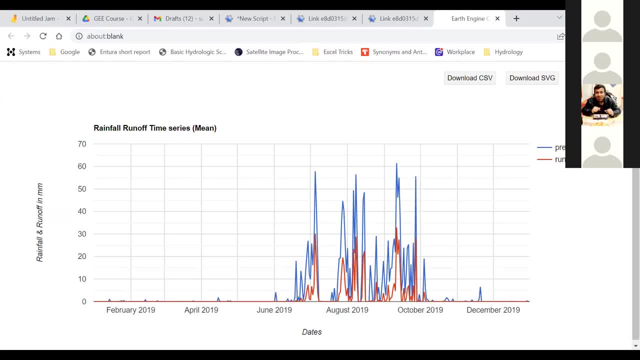 if they think that the questions are relevant to the session, then we can take those questions and we can proceed to the hands-on session. Yeah, Mr Shubkant, I think we do not really have questions. There were some related to the links and all. 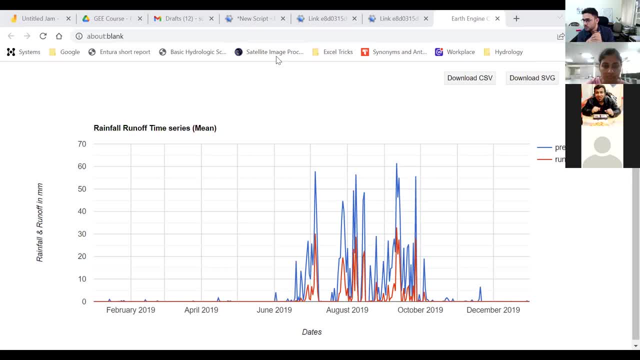 but those have been addressed. Oh, there's a question coming up. So some Anant Patel is asking: is this model in GEE is lumped Or distributed Or semi-distributed? Yes, So, Anant Patel, I think. 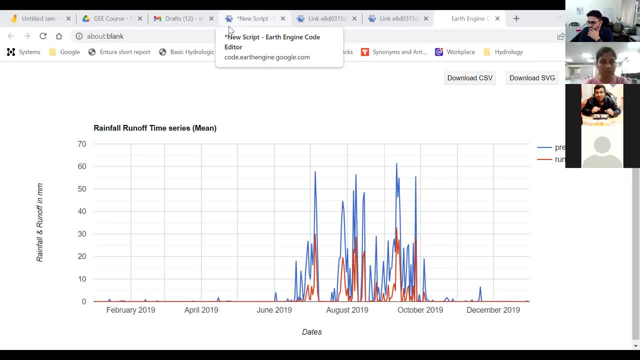 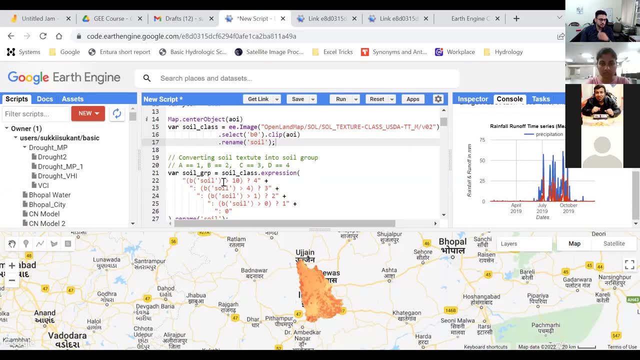 Okay, So you have asked that this model is lumped, distributed, semi-distributed. So actually in this model the curve number model is actually a semi-distributed model because here we are using the composite curve number technique. That means we are not using curve number for only specific area. 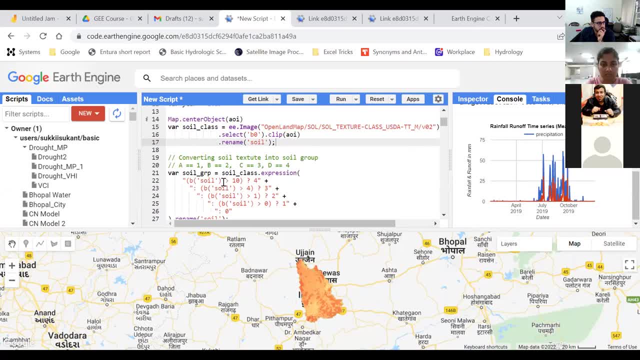 or not only for specific basin, but we are developing the curve number for specific basin, So we are developing the curve number for specific, each and every pixel. So like, for example, MODIS data set is of 500 meter pixel. So that means we are getting the curve number for every 500 meter. 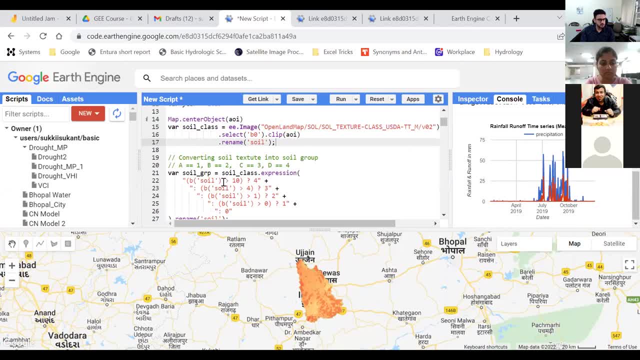 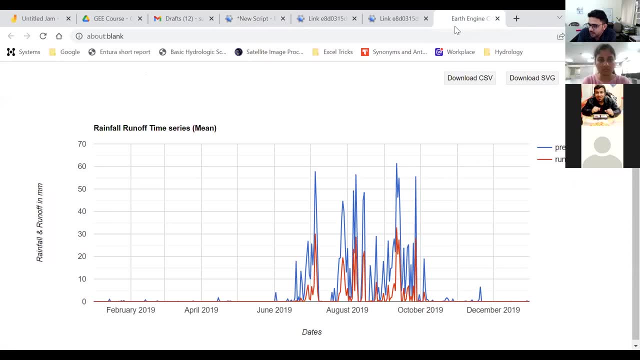 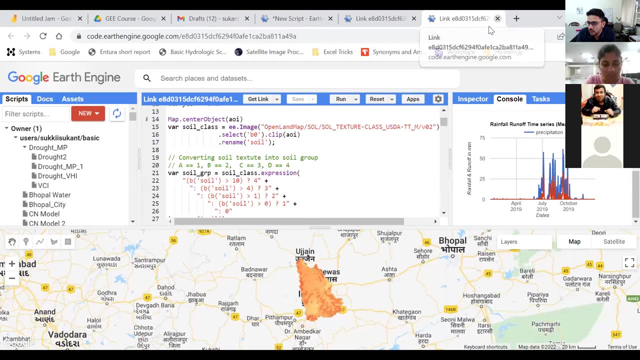 So on that basis we can say that yet it is a semi-distributed or very highly distributed model. Great Thanks, Shubkant, for answering that. If there are any other questions, please feel free to raise your hand in the comments. 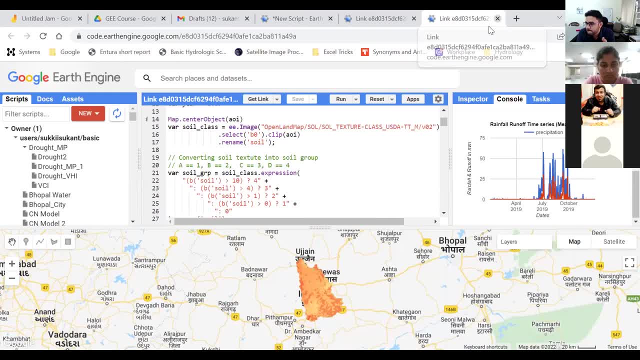 We can take some questions now, Otherwise we'll proceed. Okay, I think there are no further questions. Okay, So we will proceed with the handover session. So, first of all, in order to perform this modeling, the first thing that we required is: 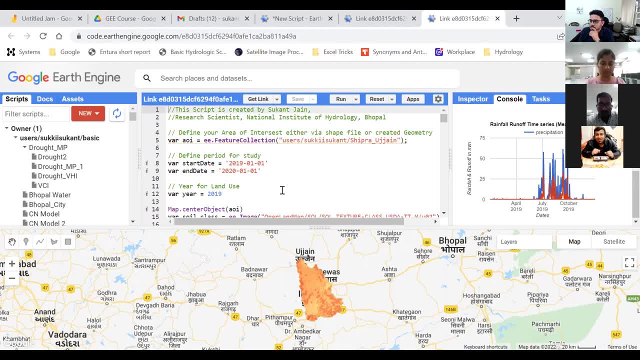 we should have an access of Google Earth Engine. So I think a few of you participants have already had the Google Earth Engine account, Or, if you don't have it, so I'll just tell you how to create the Google Earth Engine account, so that there will be very least chance of 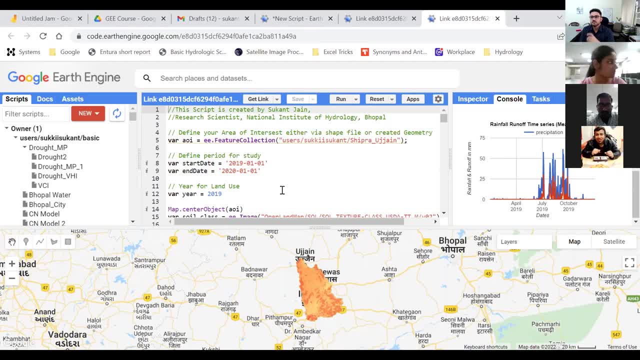 getting rejection for creating, because it is up to the Google that they will allow you to open the Google Earth Engine account or not. So, in order to open the account, what you will can do- I'll just open another in Contineto mode. There is a question in the question in the chat box. 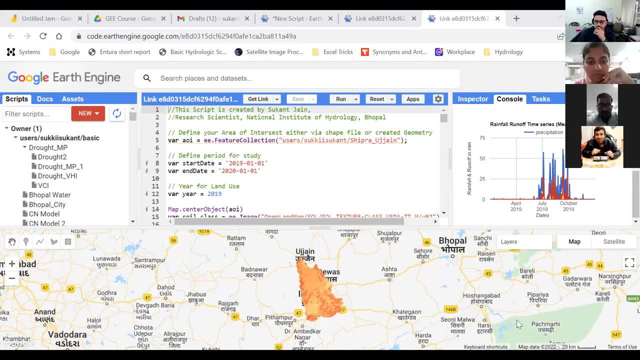 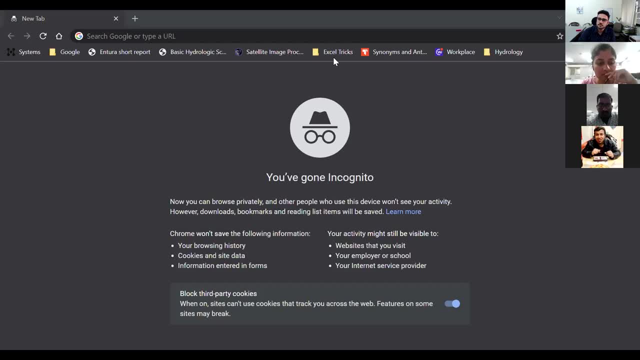 Yes, you can read. Can you please tell about calibration from Hanu Parmar? Okay, So yes, in the curve number method the calibration is actually depend on the curve number, because that is the main driving factor of this whole modeling technique. 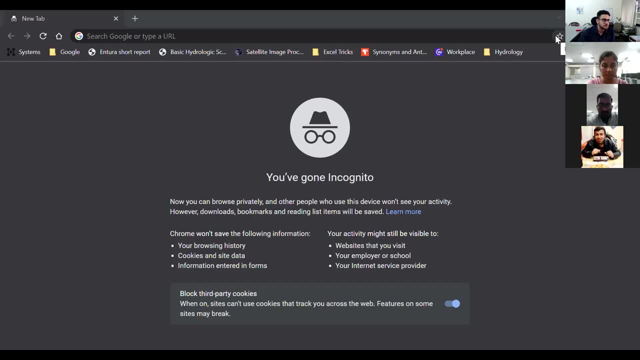 So it is for calibration. you have to do the manual part. You can repeat this question at the end of the session so that I can tell you where you can actually play with the curve number to calibrate your model to get more optimum output. 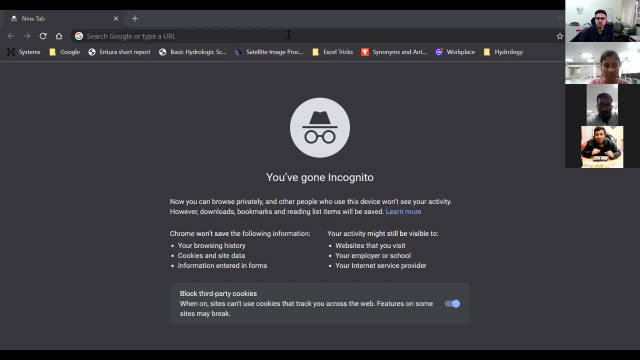 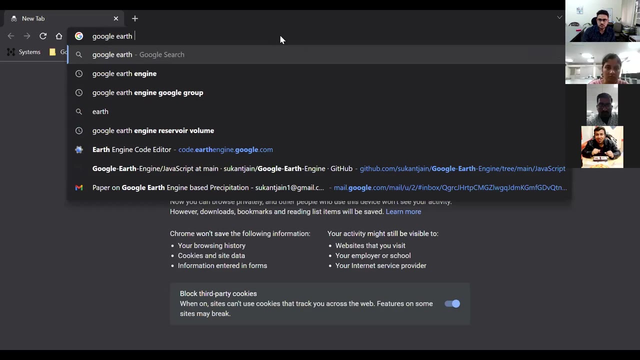 So I have opened the in Contineto mode because I don't want to. I want to start freshly that how to open the Google Earth Engine account. So if you simply search for Google Earth Engine page, I think the session is recording now. Yeah, 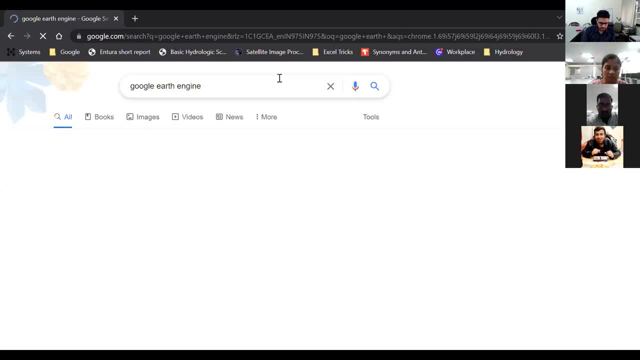 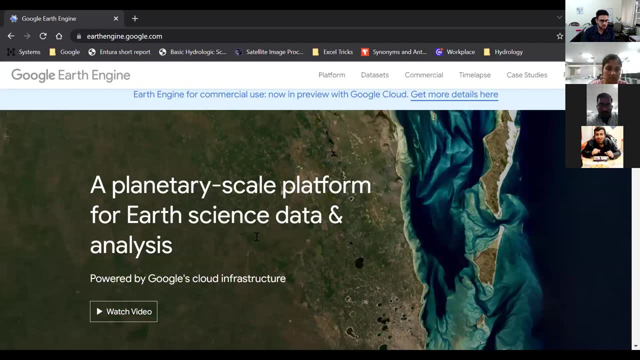 we are recording this. Yes, Yes, sir, Thank you for the response. So if you simply go to Google Earth Engine app, simply the very first page is the Google Earth Engine, their own page, and they have if the detail that: what is the Google Earth Engine? 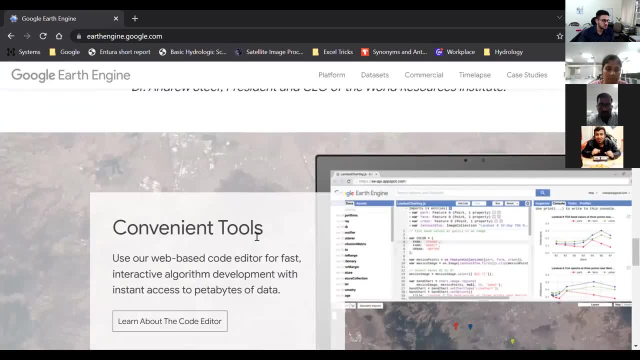 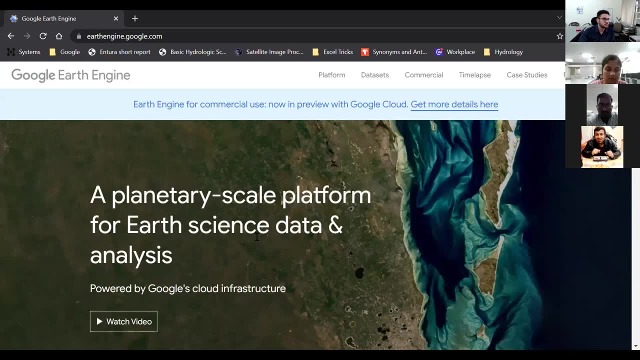 and how it is very much useful in exploring the data sets algorithm for betterment of any type of studies. Okay, so I'm not going to detail into that because you can explore on your own, but the very two things. which is very important is the data set tab. 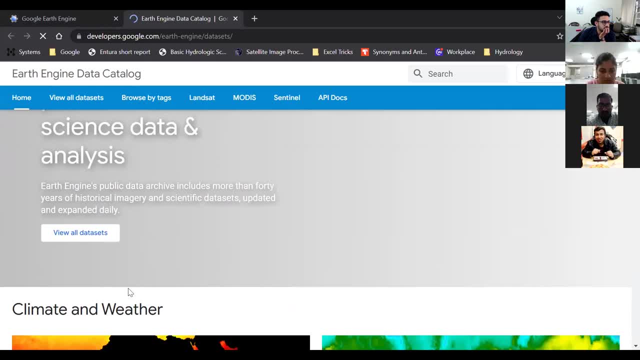 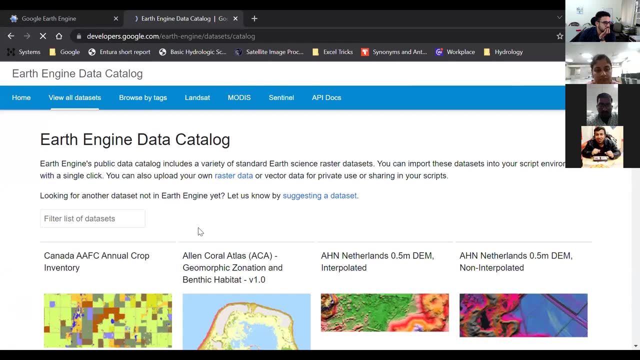 So if you go to the data set tab, you can find the enormous amount of data set that are already ingested in the Google Earth Engine platform. And not only that, they regularly keep on updating their data venture. That means you get the satellite data from the recent part. 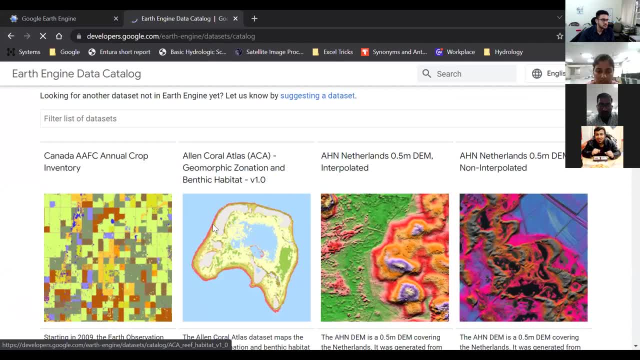 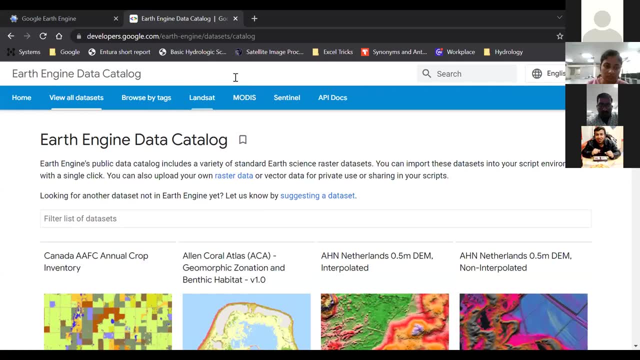 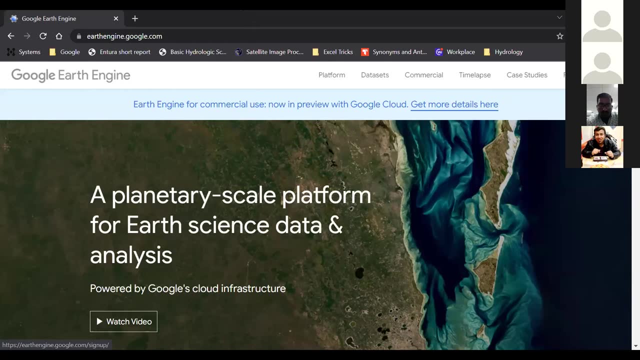 That means if the Landsat has released the data in previously- one week or maybe yesterday- then you can get those data set in the Google Earth Engine platform. The next important thing is that if you don't have the account, then you can go to the sign up page. 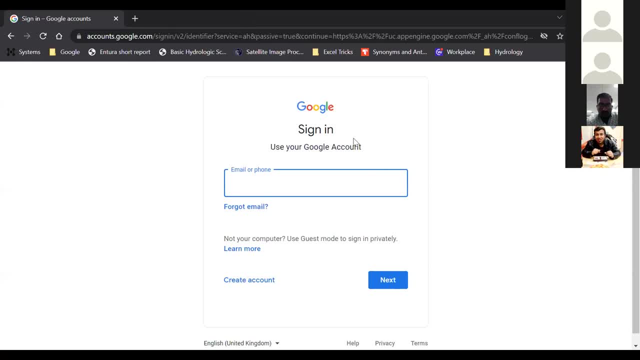 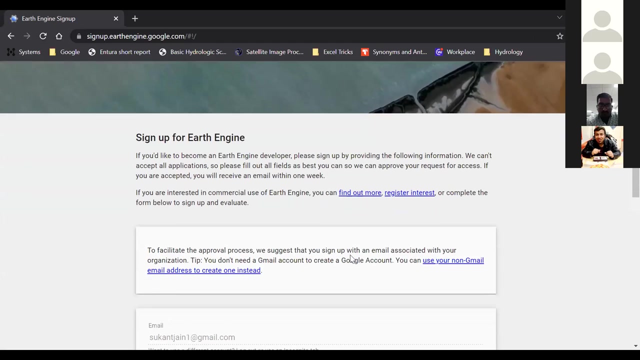 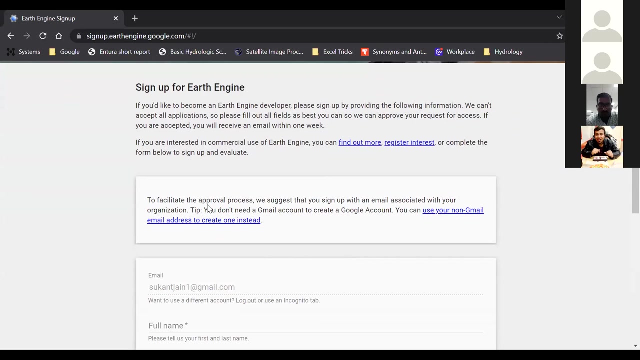 and when you can go, they will ask you to sign to your Google account and give your Gmail account. So this is the sign up page and they are asking few things And after submitting your page, there is an approval process that your page will go through. 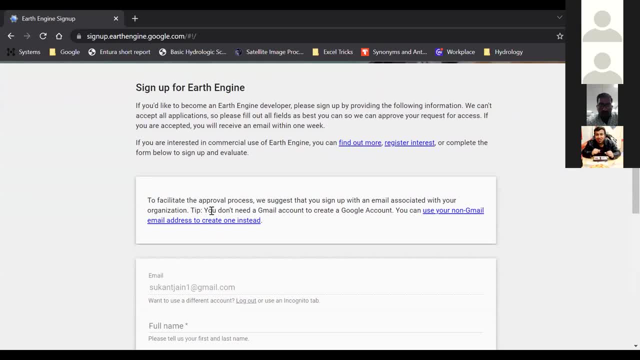 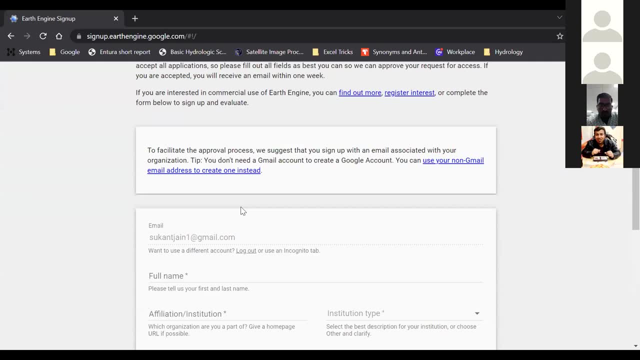 and they will analyze your inputs to let you know that you are okay for having the Google Earth Engine account or not, Because there is a very high amount of chances that they will reject your application. But it totally depends how you fill the form, First of all. 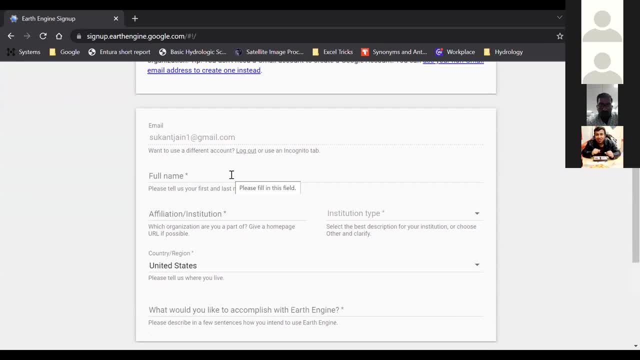 you need to prepare, give your email ID and your name- The very first thing that you have to keep into your mind- that you don't use- you're not going to use- any short form. That means if you're instituting IIT. 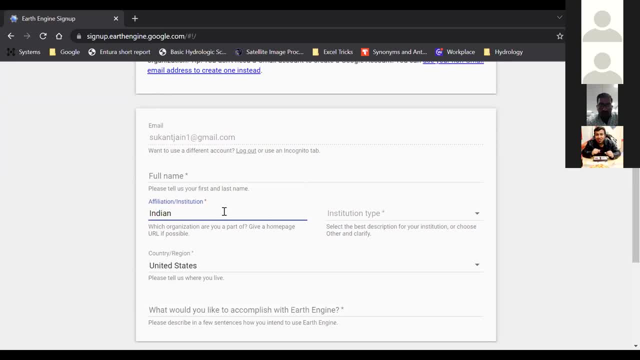 so don't give IIT right. Complete Indian Institute of Indian Institute of Technology in Burki. The next thing that you will do is give a proper denotation what your organization is there. For example, your organization is academia, So you will get academia. 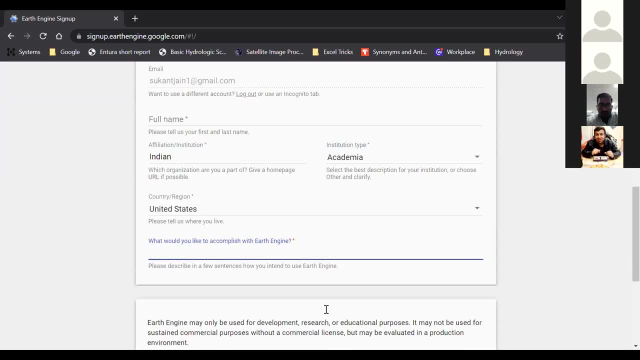 and then state- Then you have to give some small introduction- that why do you want to use Earth Engine? Either you can get write in a small paragraph or you can give in some nomenclature. For example, I'll just write hydrology. 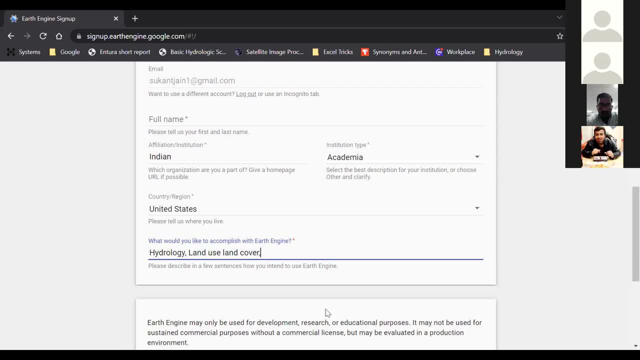 land use, land cover bodies or et cetera. You can type any of things, But please remember two things: that if you select the academia, there is a very high chance of your selection, And if you select the commercial, there is a very less chance for the approval. 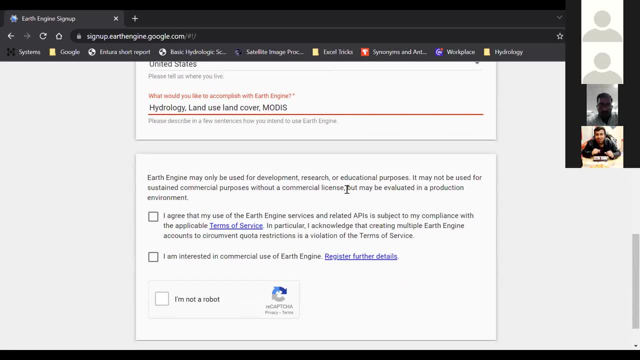 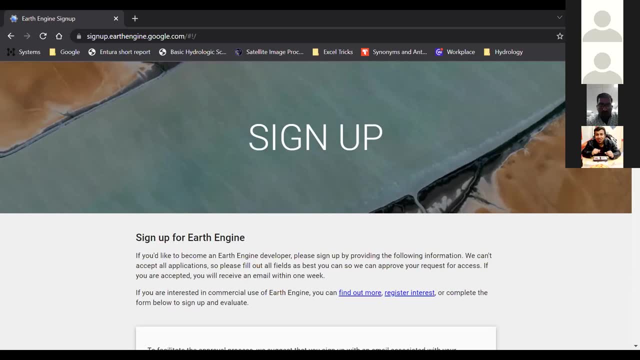 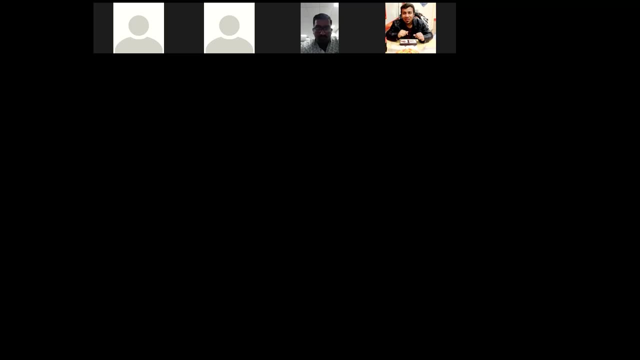 And after submitting this page, after agreeing all of these terms and technology, you will get an email that your account has been your application has been accepted or not. So I think most of you have already opened the Google Earth Engine account, If not, 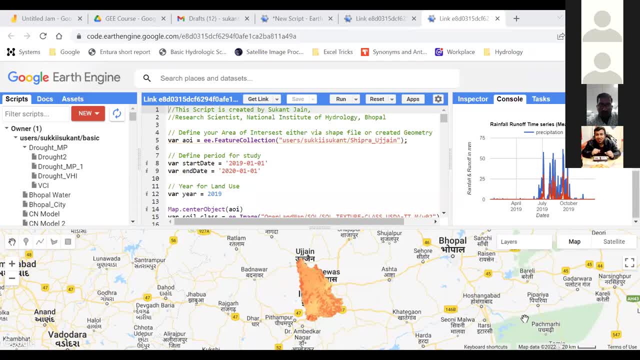 that you can open by the procedure that I told you, And it may take one or two days for the Google authorities to give approval or disapproval. So, after you have created your account, if your Gmail is accessible to the Google Earth Engine account, 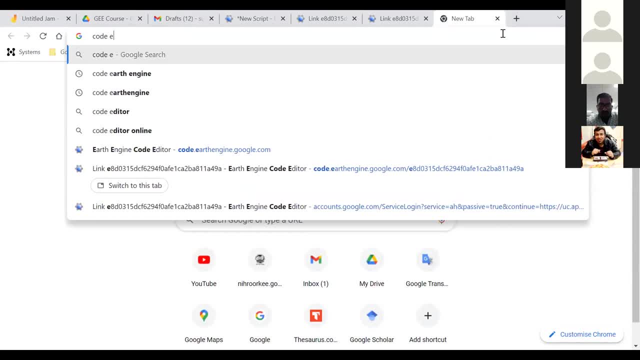 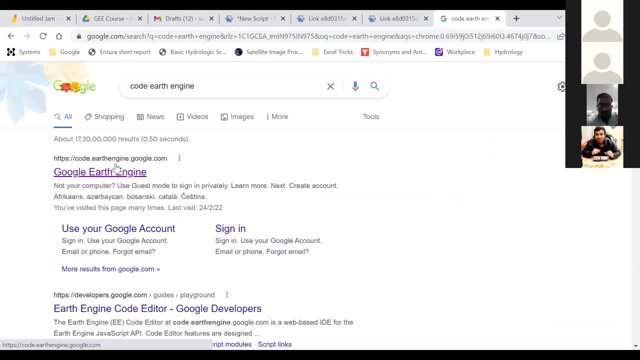 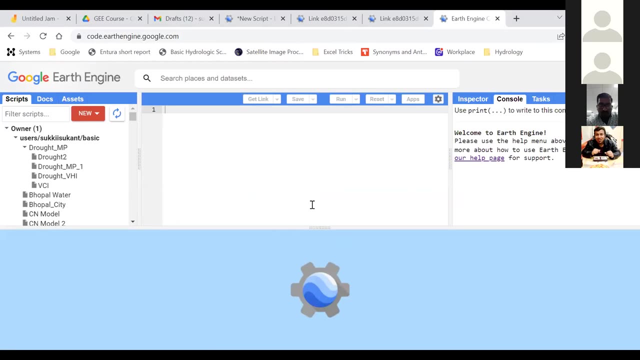 you can simply go to the Google and type code: earth engine. Okay, So if you go to a website known as codeearthenginegooglecom, you can get this page. This is the main code editor of the Google Earth Engine platform In this. 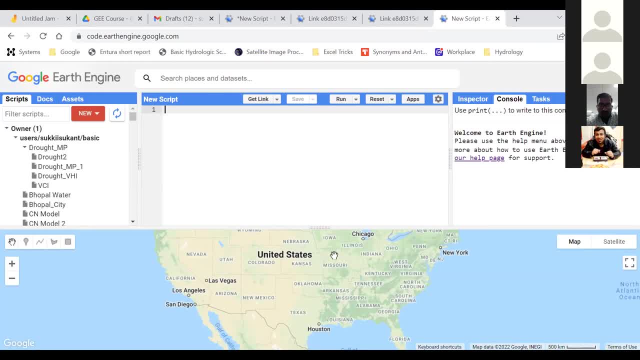 you can find the very two things. That means a script editor and the map, And in the right-hand side there are three tabs: script, docs, assets And in the sorry. this is the left-hand side. This is the right-hand side. 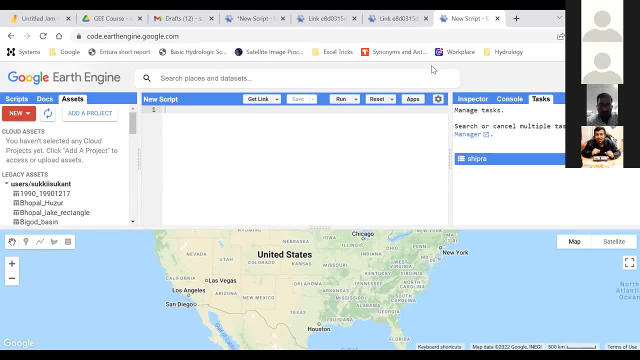 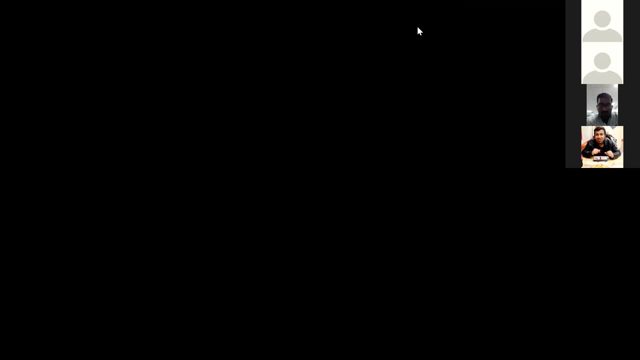 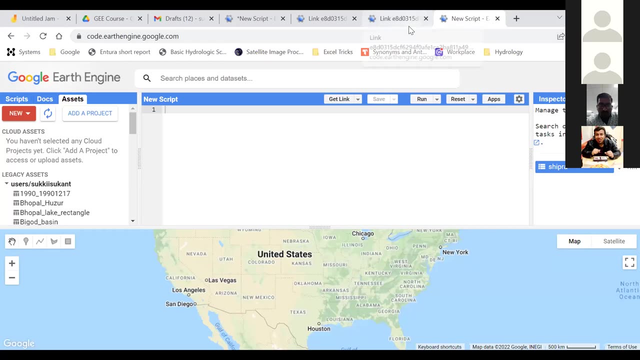 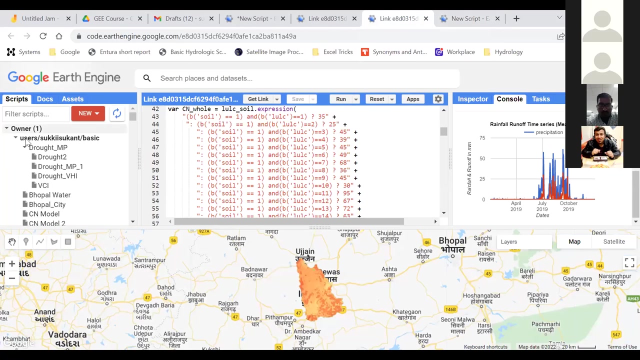 You can find inspector and task. So if I go to my script, the model which I have, So this is the link that we have prepared, our model. Okay, So in the script segment you can find all those scripts which we have developed by you. 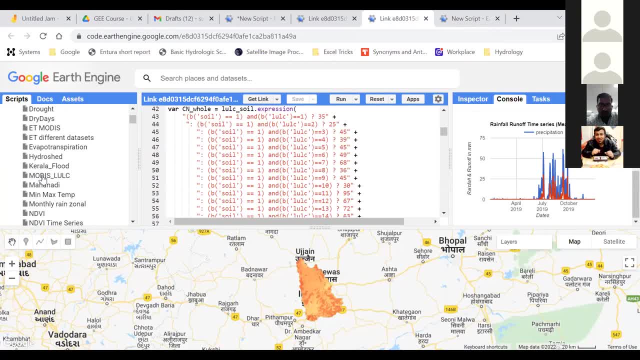 or have been shared for you or towards you. You can find, for example, I have prepared these number of script and save so that I can access all of this script whether I'm using this laptop or some other PC, or if I want to share this script. 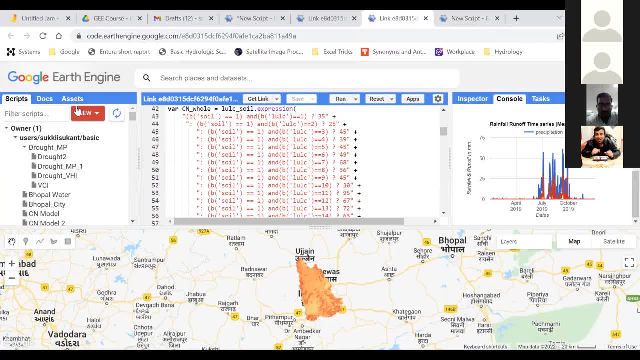 I can simply go the particular script and share that particular thing. The next thing is. the third thing is assets. Assets is nothing but your own data set, which I've told you that you can always ingest your own data set, And these data sets are: 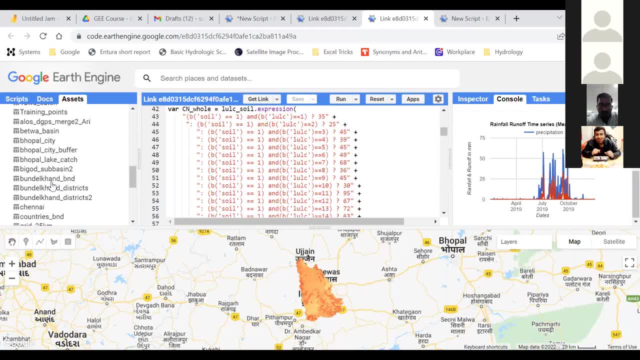 will be available in the asset tab. That means all these vector file and raster data sets are uploaded by me And most of the time you will get to upload the vector data set because for a vector data analysis, Google Ads engine is not a very good tool. 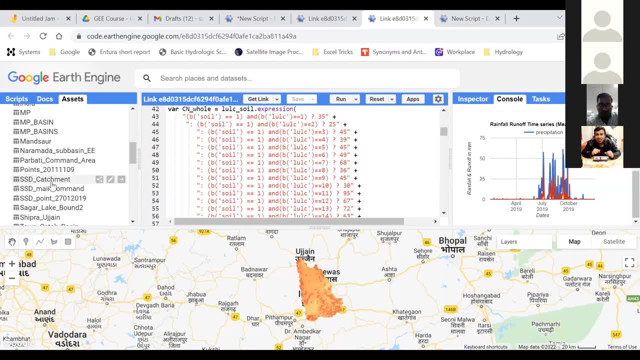 But for a raster data analysis it is a very good tool. So you need to upload your own special- what we can say- vector data or share file to get the things done. Then the very next thing, important thing, is that docs. 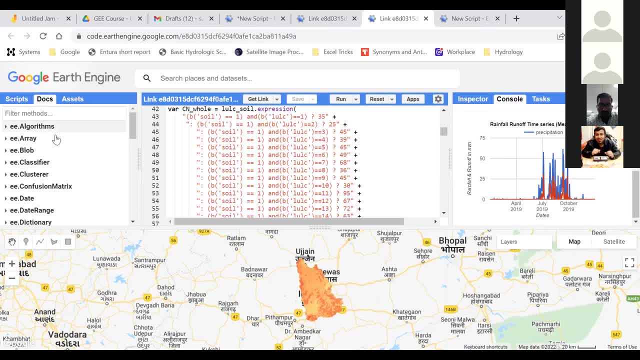 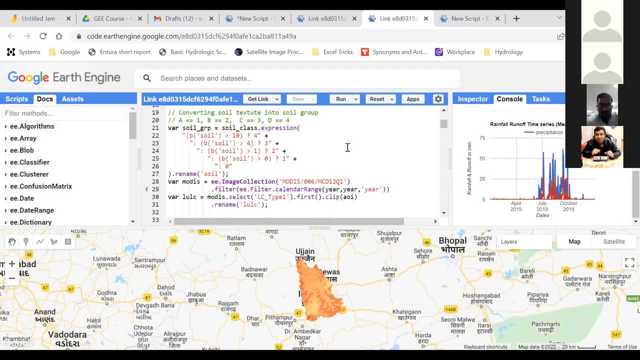 So it has all the data, it has all the algorithms and all the functions that are available in the admin. So we will explore this thing one by one when we are actually scripting our model. So the next thing is the when we write down our script. 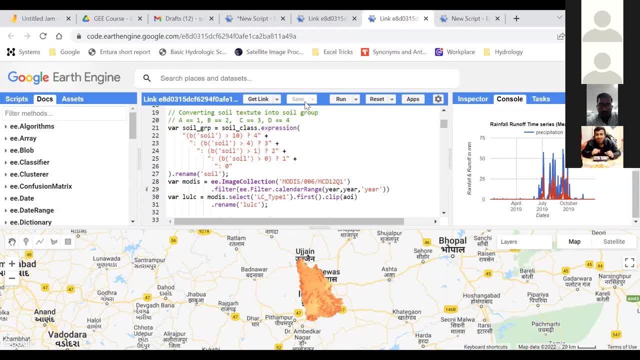 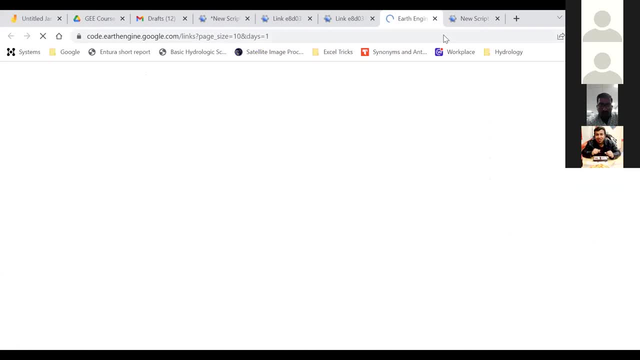 either we can run, we can reset the page and we can save the data script into our script tab, or we can click on this get link so that a link will be generated. a link will be generated and if I share you this link, 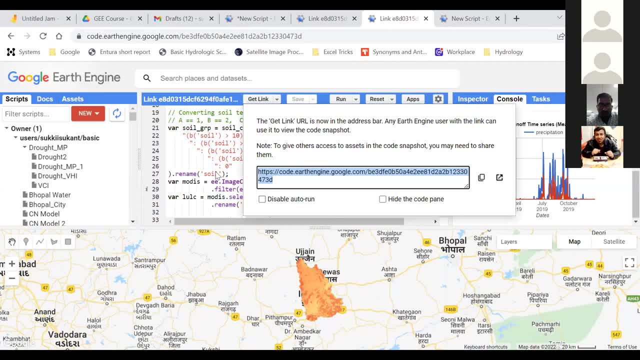 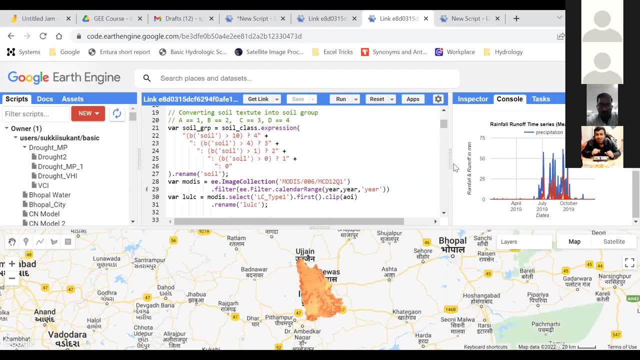 so then you can access with this code in very handy manner After that when I click run, so all the output that are in the map format will be displayed over here. You can find in the map we have certain colorful map And if we go to the layer tab, 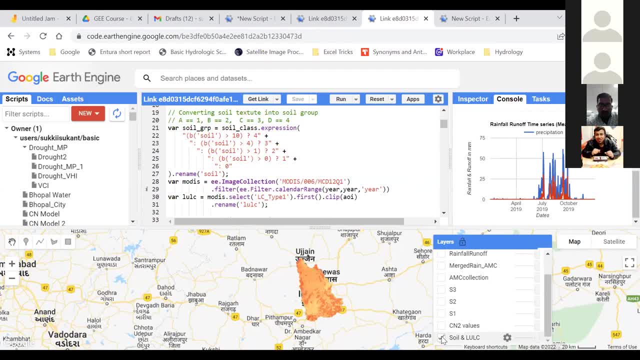 we can see there are five to six maps are there, For example, sign in LULC, because we have prepared this map for this particular task. You can always check on and check off this maps. Then in the console panel we have all the amount of output. 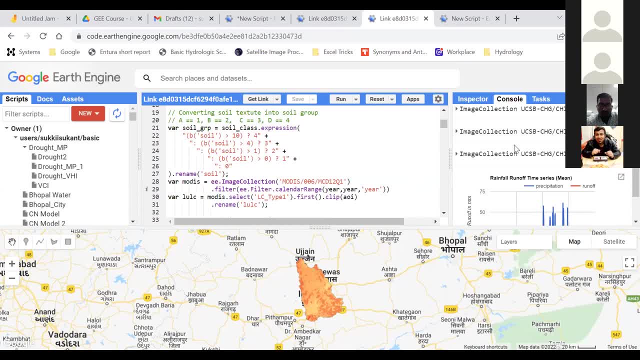 that are in the format of either string or tables or chart. You can see the chart is actually displayed in the console panel. Then task is there. If you perform any task, either uploading or downloading any dataset, then you can go to the task. 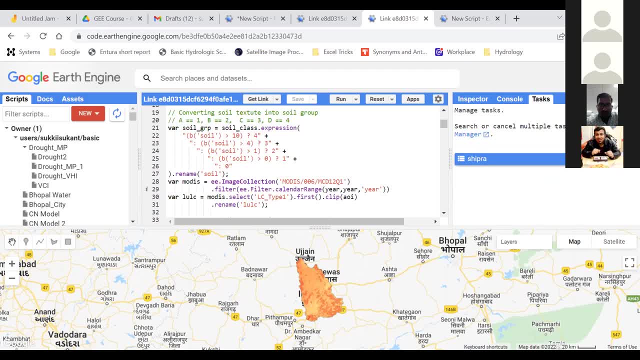 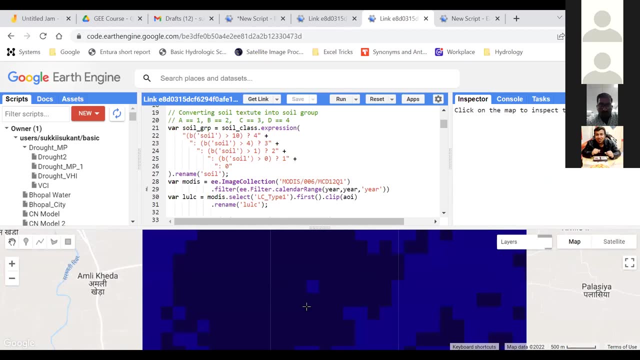 and check the status of your task, Then inspector tool. So inspector tool is nothing. but if you want to inspect each and every element, for example, if I zoom to this layer and if I want to inspect this particular pixel, okay, this particular pixel. 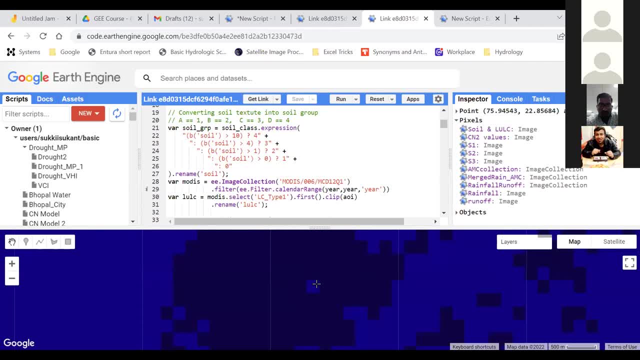 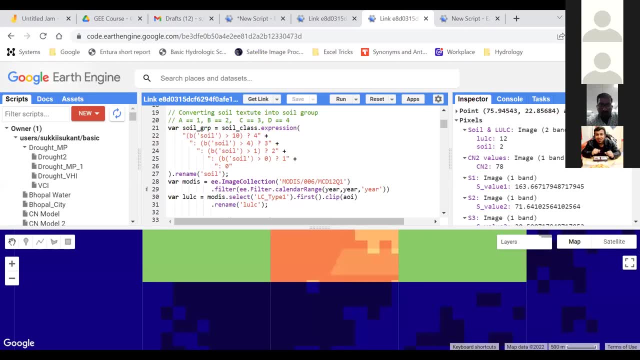 if I click on this inspector tab and I click on this particular pixel, so all the information related to this particular pixel, of all these data set, will be displayed over here. For example, this particular pixel have a LULC class of 12,. 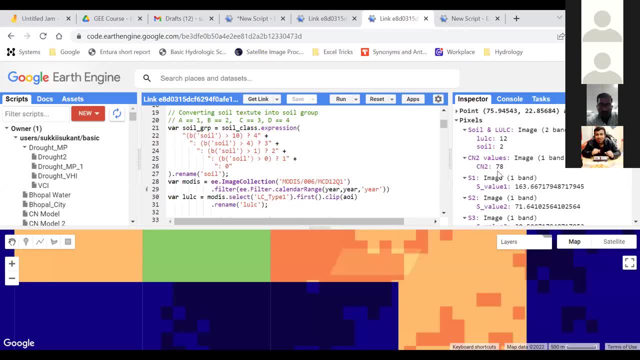 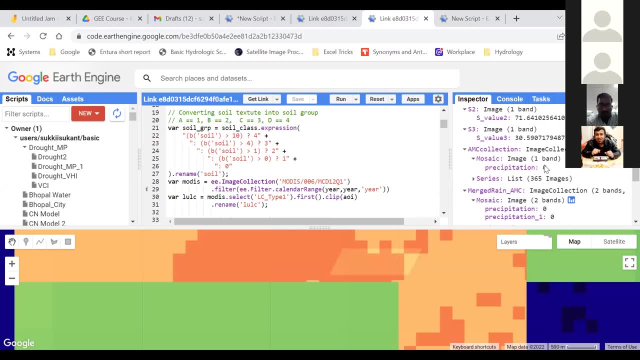 soil class of 2,. it has a curve number of 78, CN2.. It has a S value of 71,, 163, 30.. Then it has a precipitation. The latest precipitation value is zero. It has a series of precipitation. 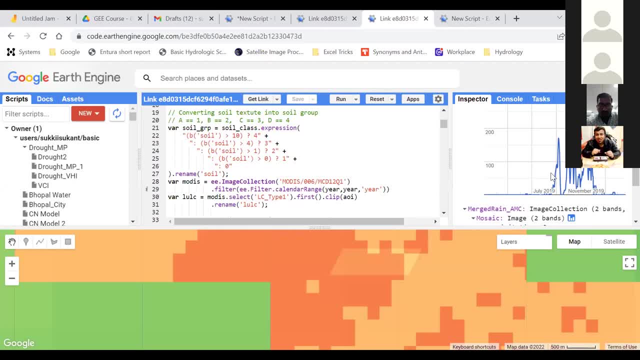 That means 365 images of a single year. That means over this pixel. these are the precipitation values in mm. Then, finally, we have the runoff series for this particular pixel, But in the console panel we are actually getting the runoff for whole this pixel. 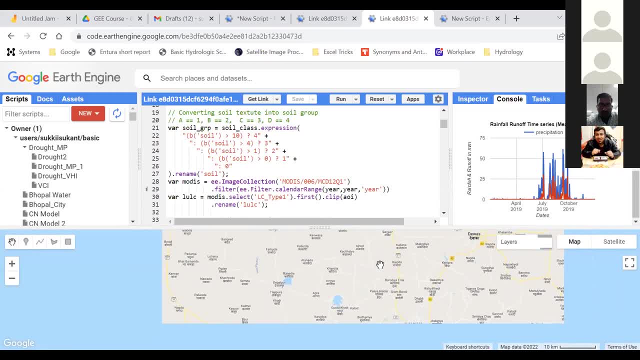 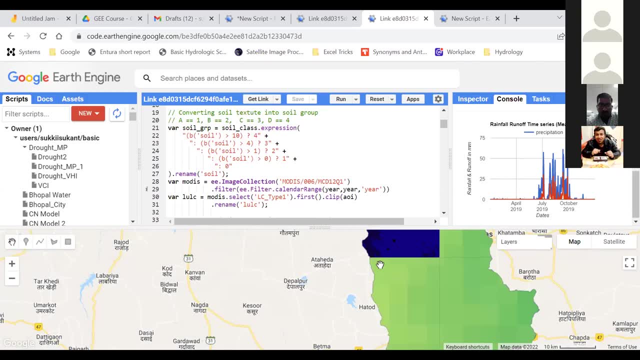 For whole this area. So similarly, you can always inspect any special rainfall and runoff for a specific pixel or for a specific area also. So this is how the whole things in the Google Earth region works. So initially I'll just I will try to demonstrate this model. 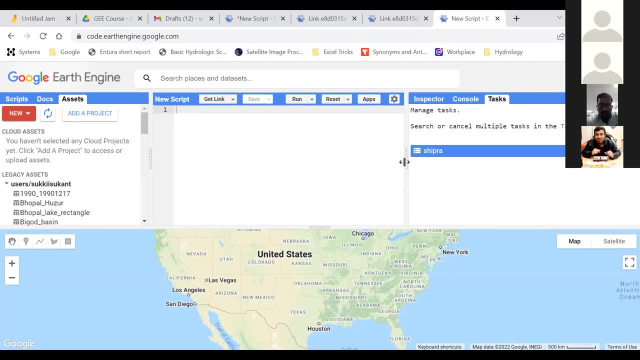 in very different segments, so that you can clearly understand how the things would work. So, first of all, the very first thing that we required is the shapefile of your area. So, for example, if you are working in any South Indian basin or any type of basin, 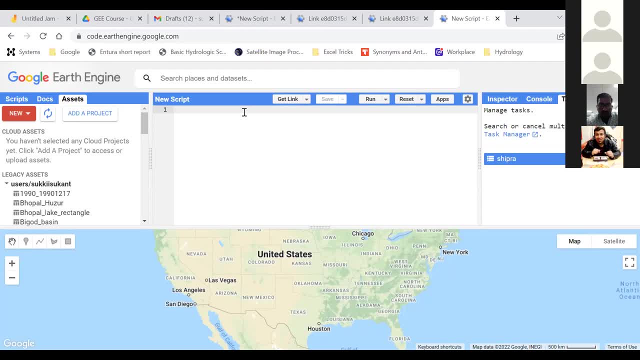 so you should have a shapefile, and the shapefile can be in the format of. sorry, the vector data can be in the format of shapefile, TML file, GeoJSON, et cetera. That means the cachement boundary. 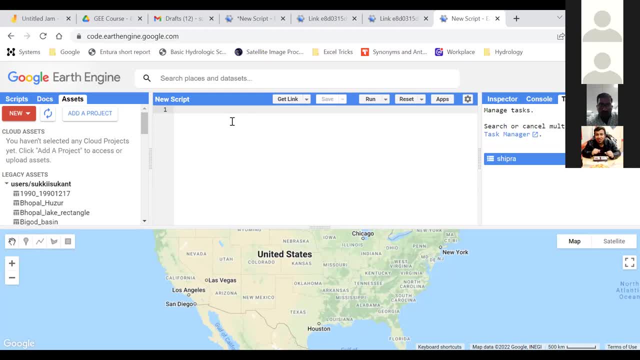 So first of all, we can upload our own cachement boundary. When we go to the assets, we can click new Okay. Then the data sets can be uploaded in two format, either the GeoTIFF or the image upload. the table upload. 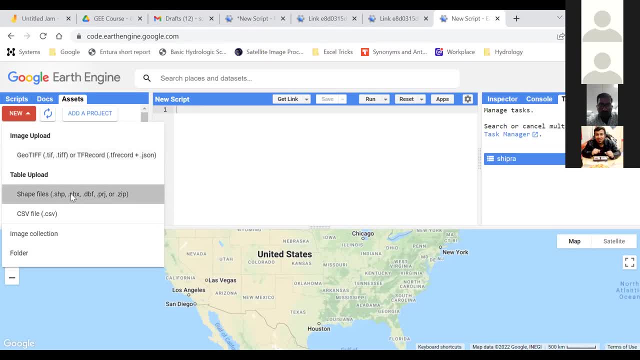 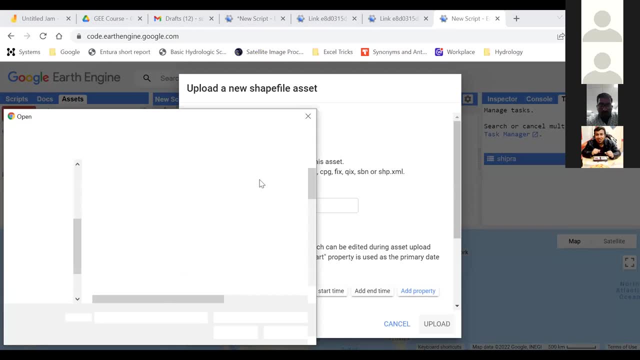 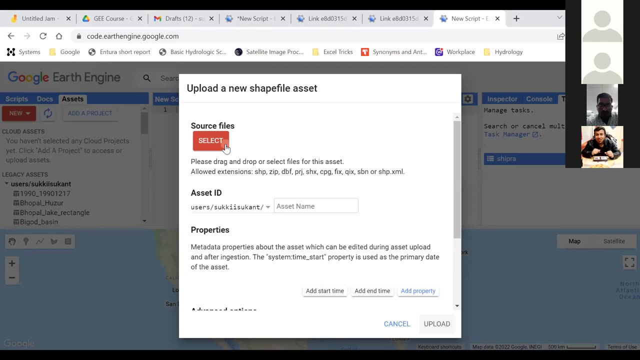 So we'll click on the shapefile And in order to update the shapefile we should have all the supporting extension. That means SHP, ZIP, DBF, PRJ, SHX, et cetera. All of the things should be there. 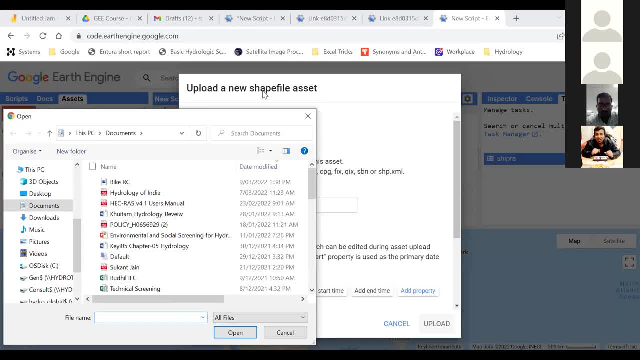 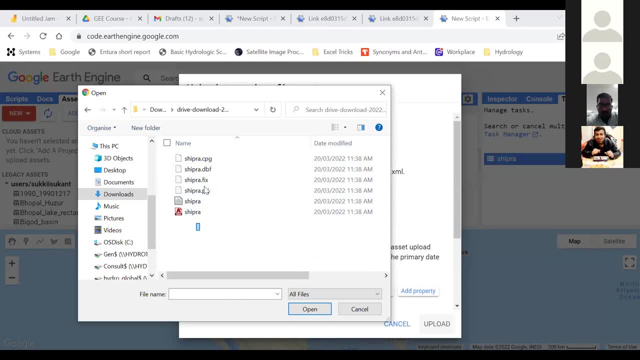 If I go to select. this is my local directory, I will go to the. so this is my SHPRA shapefile. These are all the supporting file. Either I can select all or I can zip this folder. I can compress this folder. 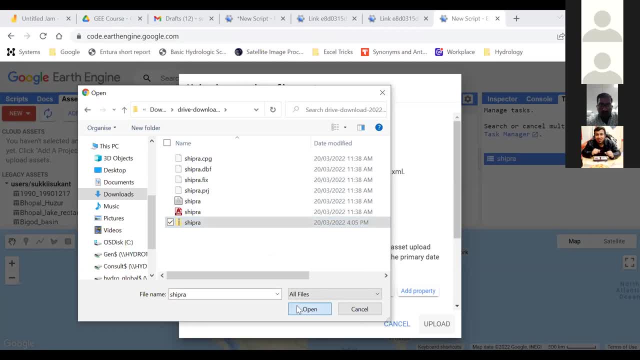 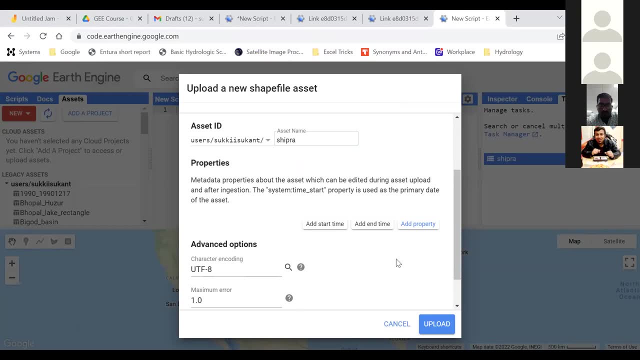 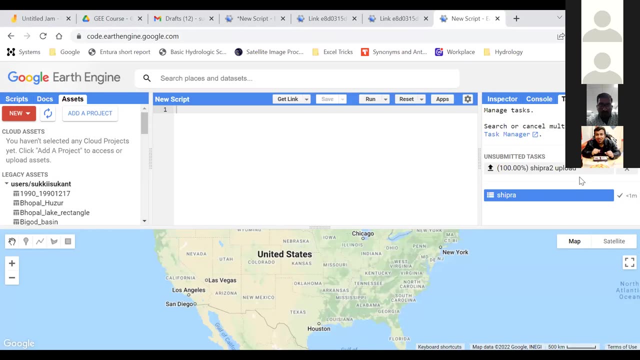 and upload only this compressed file also Open. So asset name is SHPRA and this is my user ID. I just simply write SHPRA2, because with the name of SHPRA is already uploaded. Now you can see this in the taskbar. 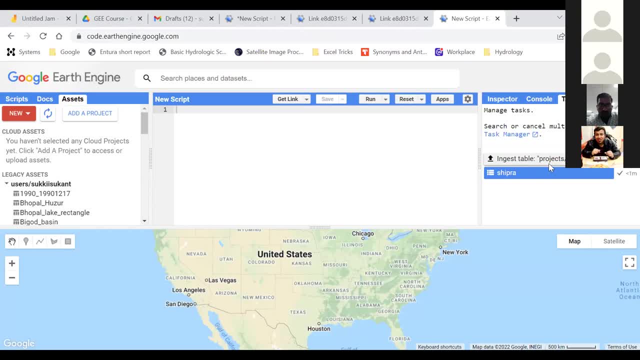 There is a task It's actually happening. That means ingestion of table with the name projects earth engine SHPRA2.. And then we have to wait approximately 30 to 50 seconds to get our assets in the in this tab. So after this has been finished, 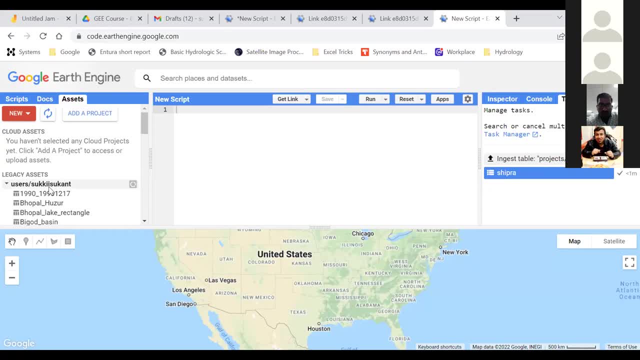 you can check by clicking on this refresh button And if you can find it, SHPRA2 is there or not. The SHPRA2 is my old file. It may take one to two minutes depending on the area of your catchment boundary. 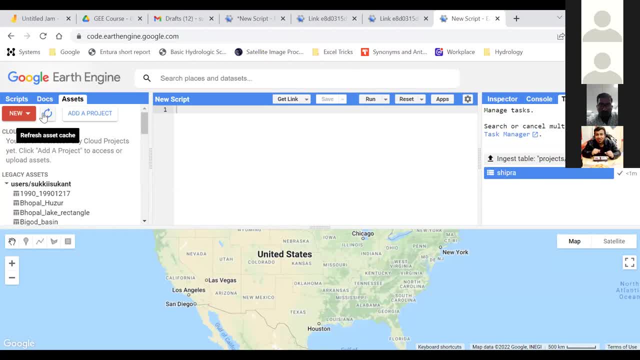 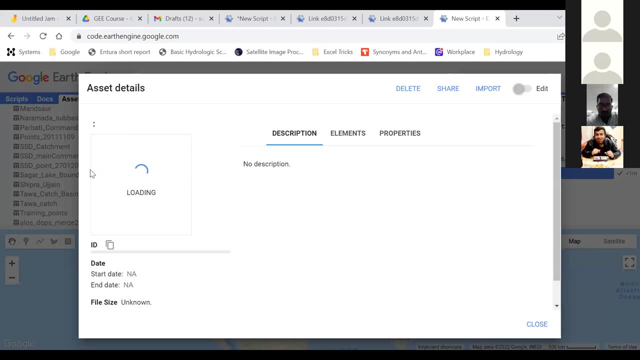 Okay, meanwhile it will upload it. I'll just quickly demonstrate how we can actually use this boundary. Suppose this is the SHPRA underscore gen has already been uploaded, So if I click on this so we can get actually these amount of properties like description features. 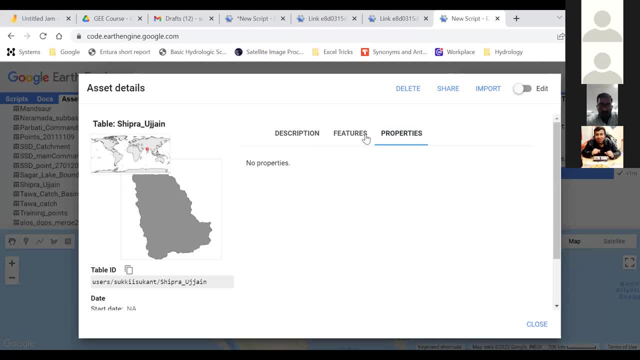 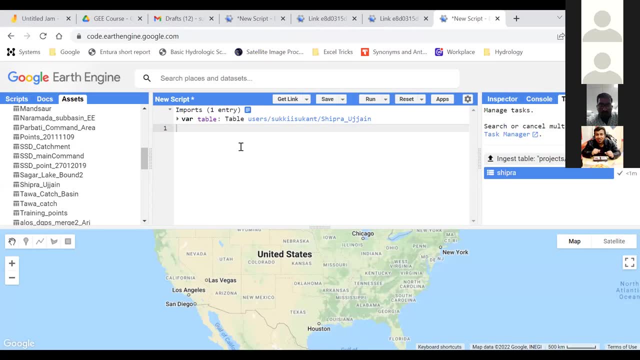 There's a single layer, its properties, And in order to import this data set into the script, we'll just click import Now, after clicking import, you can see in our script editor. a data set with the name of table is already uploaded. 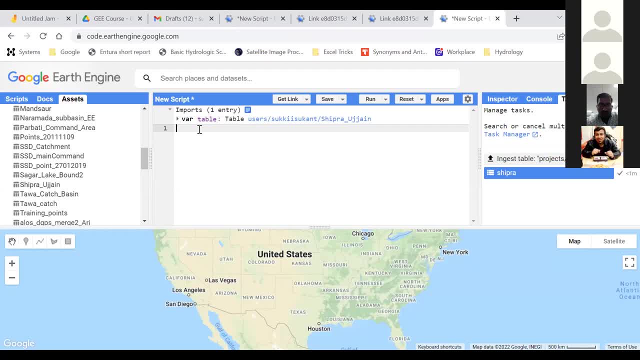 Okay. So first of all, we will change this table with the name AY so that it will be easy to access or change the data set. So what we have done? we have created a separate variable with the name AY and we have assigned the table. 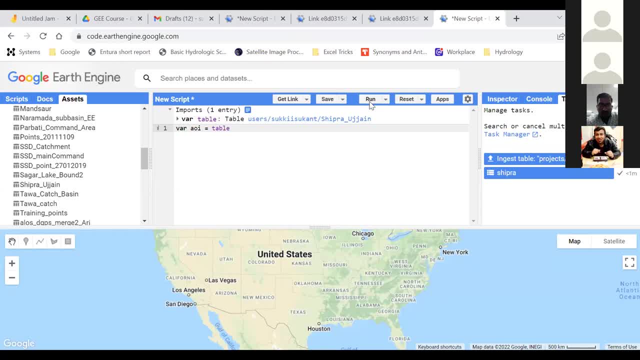 That means our data set, Okay. And if we print, click, run, so nothing will be happen. If you go to the console panel, there will nothing will be print. But if I click, if I write, print, AY, so what will happen? 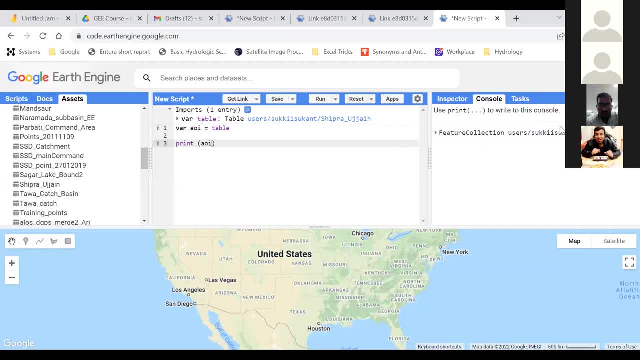 It will show me that it is a feature collection with the name SHPRA, But nothing is actually happening over the map. That means I cannot see my shapefile. So what I will do in order to display any type of data set. there is one thing that is. 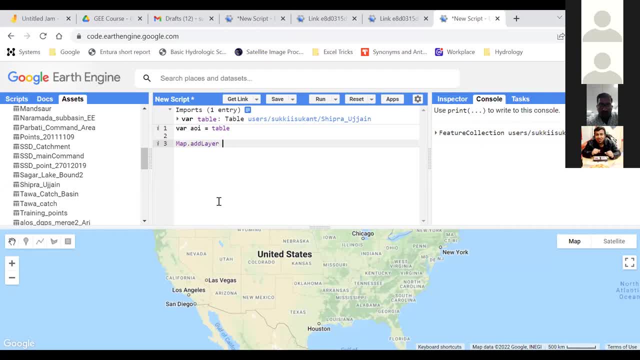 one thing, that is, map dot add here So you don't need to write all the things that script data I'm writing on the parallel mode At the end of each section. I will share this script, what I've written over in my screen. 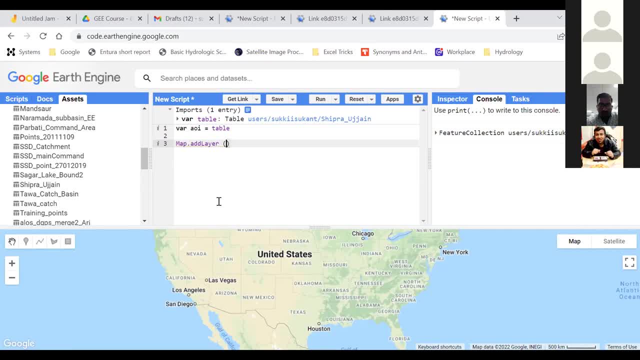 You can use this into your own screen and get the thing that how the things are actually working. So don't bother about the script, Don't try to just copy my what I'm doing. Just try to understand what is actually happening behind those. 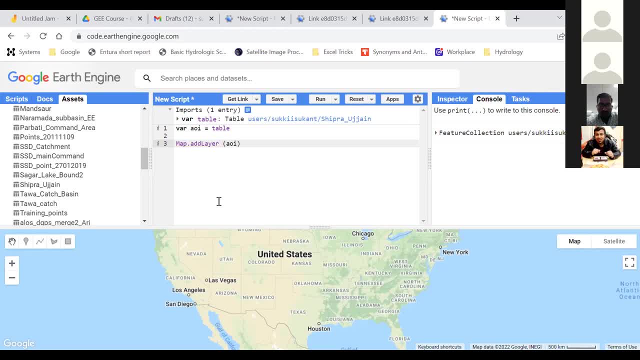 So what? we have written map: add layer AY. So if I click run so nothing will happen over there because my output will be in the format of map. So in the layer panel I can see a layer has been generated, but I cannot see over it. 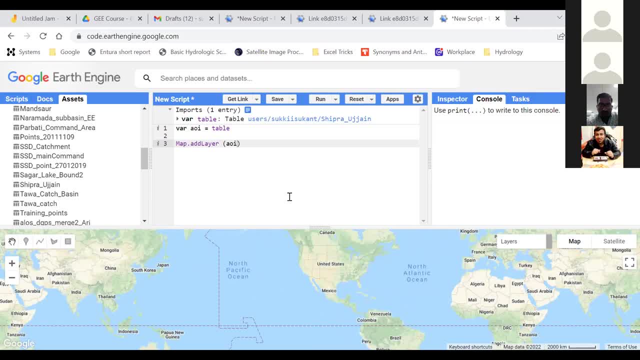 Why? Because it is in the some other area, other part of the world. So what I will do? I will just zoom my layer For that. it is a function Known as map dot center object, And I will just click AY. 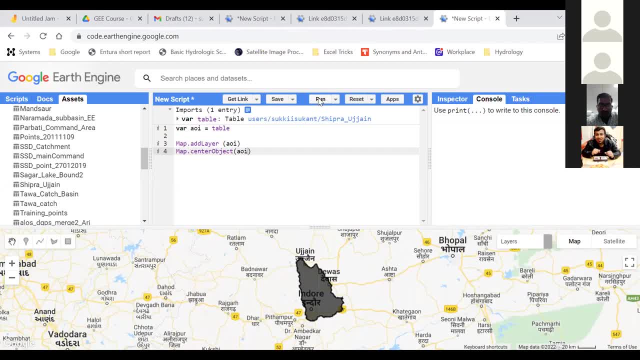 and I will click run Now see what will happen. It will automatically zoom to my area for which I uploaded the shapefile. Next thing, it has already. my shapefile is there and it is with the name of layer one. Okay, I can change this name also. 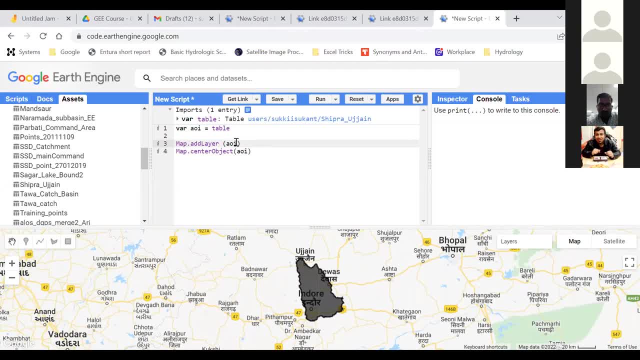 For example, map dot add layer. I can just give this two bars And give any name, For example Shipra, catch file, And I click run Now can see this. Now this layer has been with the name of Shipra. 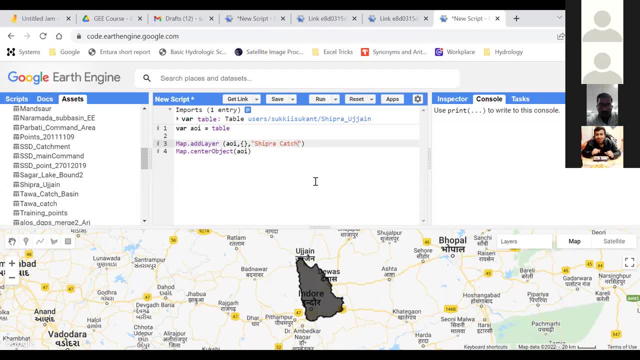 Okay, So this is how we can actually ingest our data set into our Google Earth engine script editor. Okay, So, first of all, the very first task is to define our area. So we have defined our area. Next thing: define the period of study. 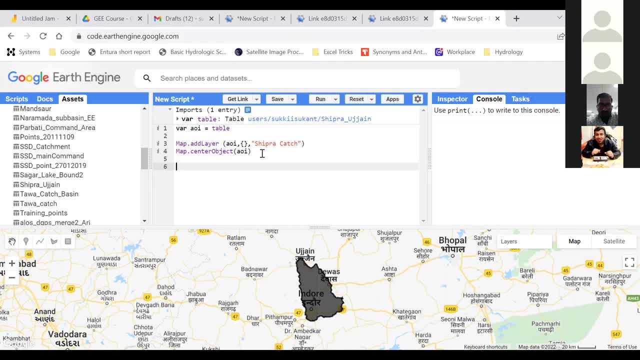 So, for example- okay, so we will talk about it later- So, first of all, we have to define any year for which we have to get at the LULC data set. For example, we are working for the data set of 2019.. 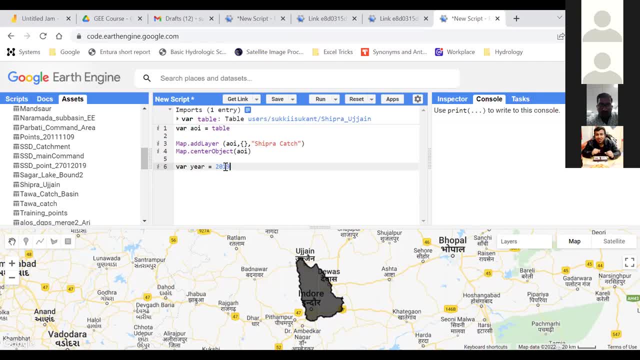 So we will get the land use land cover of 2019.. And we have stored the value of 2019 in the variable year. And next thing that we are doing is all the two data set. One is LULC And second is soil texture. 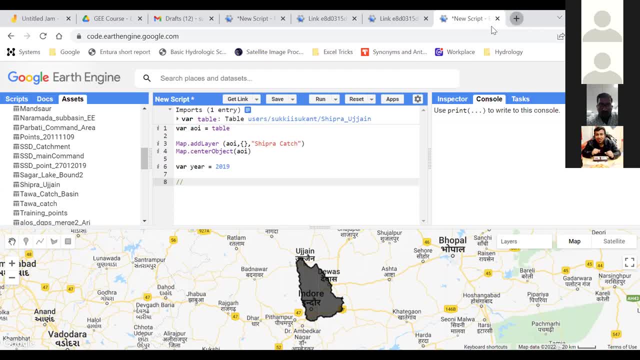 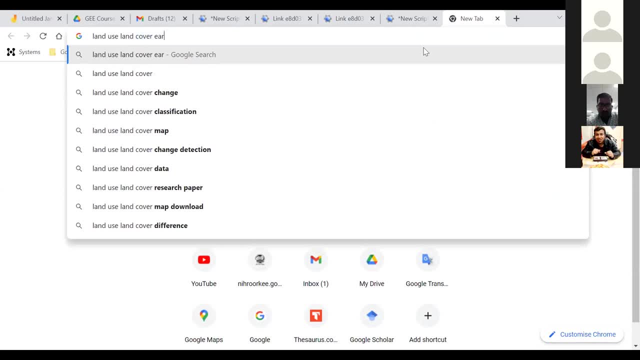 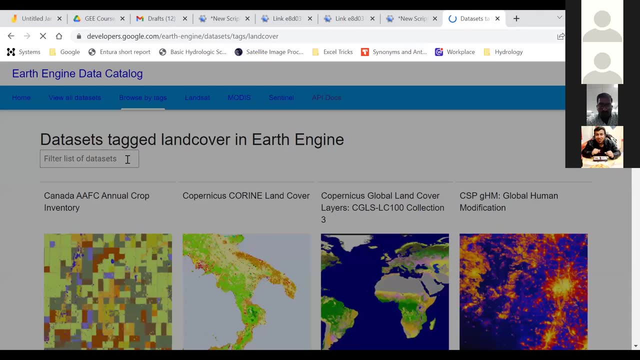 So, in order to explore the different type of data sets, we can simply use the Google Either, for example, just simply write land use land cover earth engine And we simply open the Google Earth Engine tab, And these are all the data set related to land use land cover. 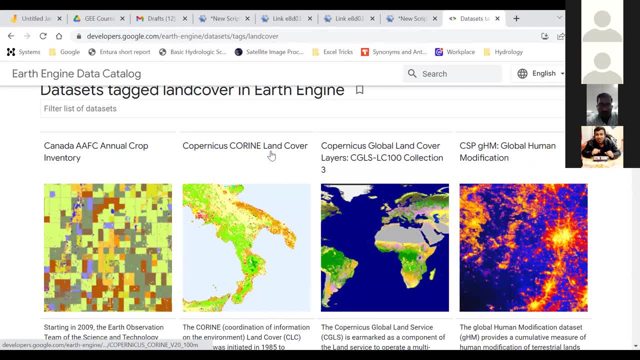 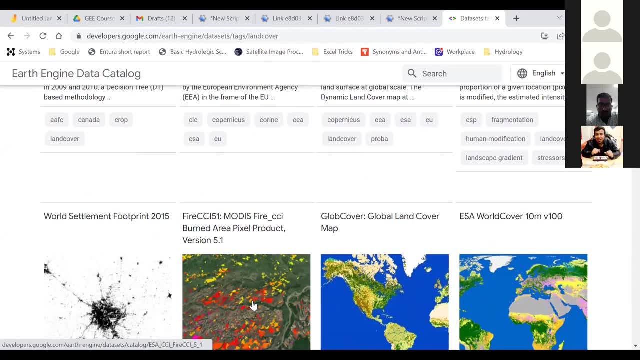 For example, it provides the Copernicus land use land cover for a specific area. It will be written over here that this land use land cover belongs to the whole world or for a specific area. That means globe cover land use land cover. 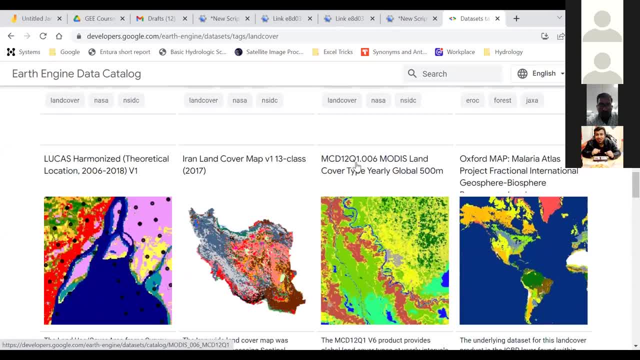 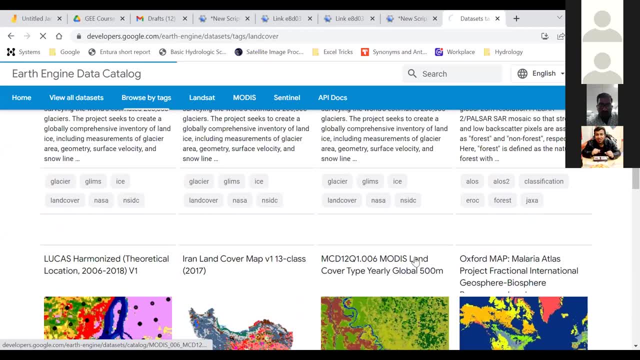 and the MODIS will be there. The MCD12Q1 MODIS data set is there, So in this case we are using the MODIS data set, So we'll just open this data And this is the detail about the data sets of MODIS. that. 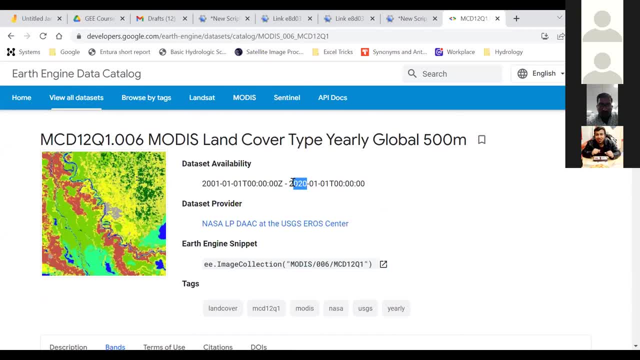 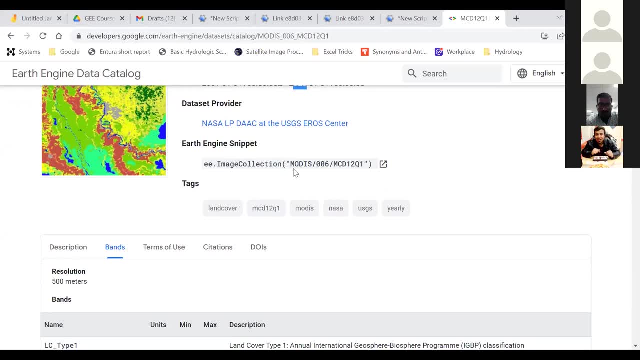 the data set is available from 2001 to 2020.. These are the, these agencies, the data set provider, And this is the Earth Engine snippet through which the data set can be called. And in the description you can see the the data set. 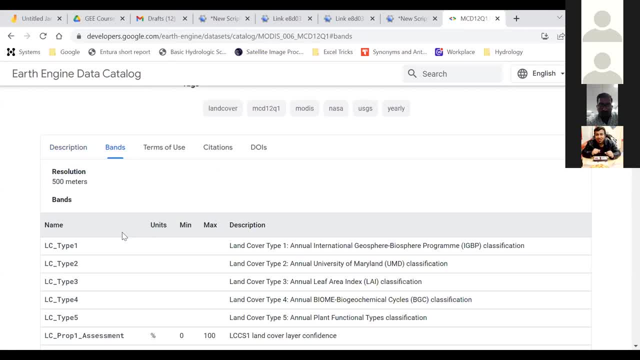 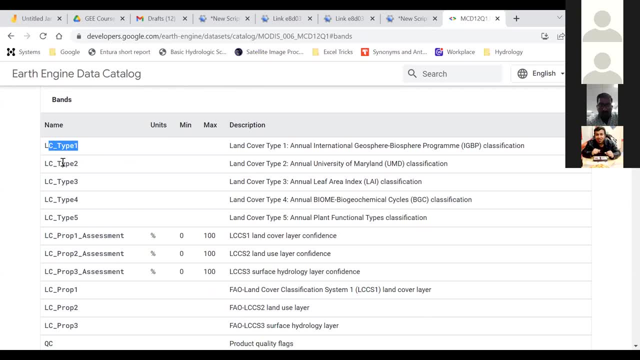 the information about the data set And in the bed in the band, you can see the different type of bands that this data set has, that this has the LC type 1, LC type 2, LC type 3, and number of things are there. 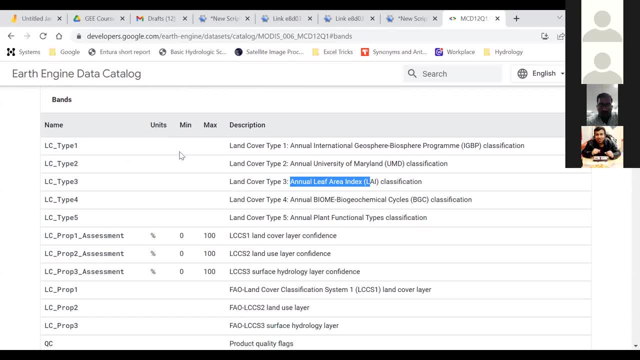 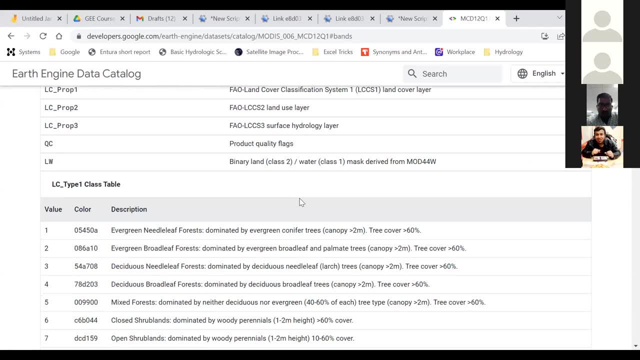 That means LC type 3 denotes the annual leaf area index. LC type 1 denotes the annual IGBP classification. And what are the classes for? If you go down, you can find this. These are the values. That means 1,, 2,, 3,, 4,, 5,, 6,, 7,, 8,. 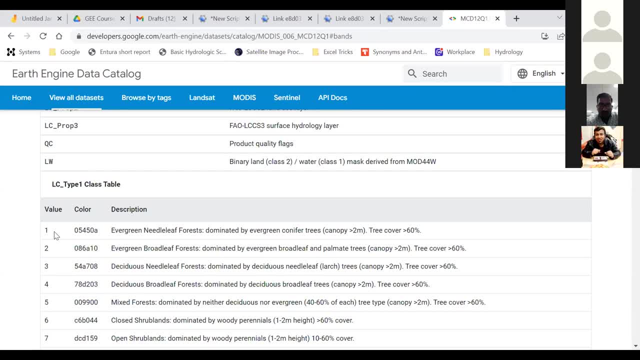 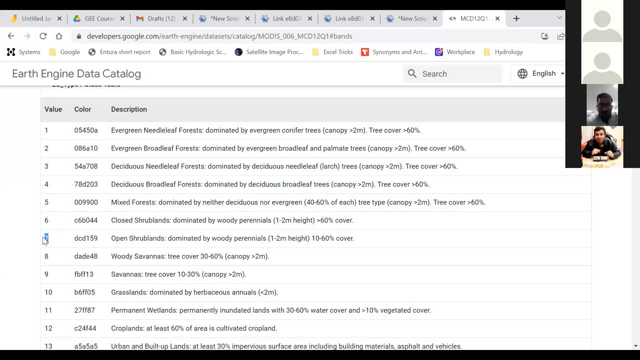 up to 17.. And these are the respective classes. For example, in the map, the value 1 denotes the evergreen needless forest. The value 7 denotes open shrublands. The value 40 denotes croplands. Okay, 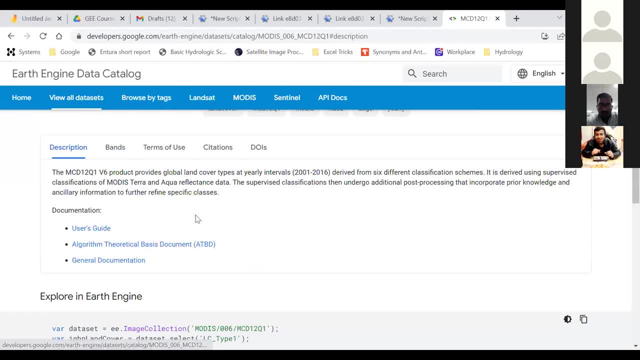 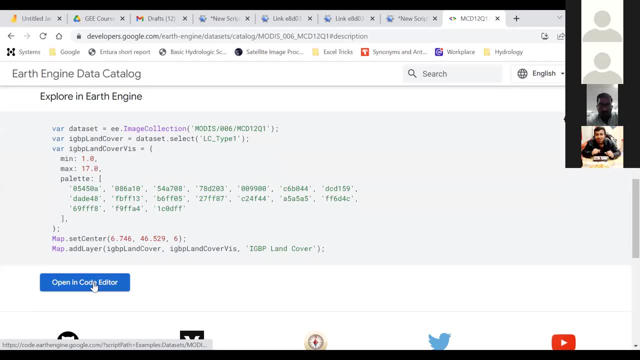 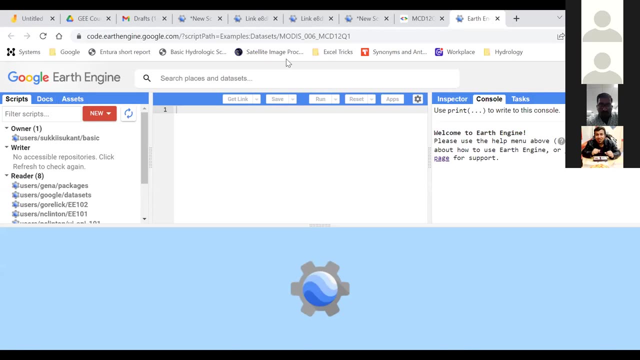 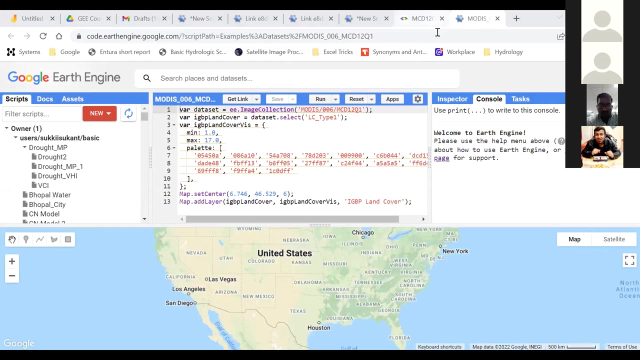 So, in order to explore this data set, if you go to the description, there will always be a sample script. will be always be there for each and every data set. So if I just open this, click in this, open in code editor. So this particular script. 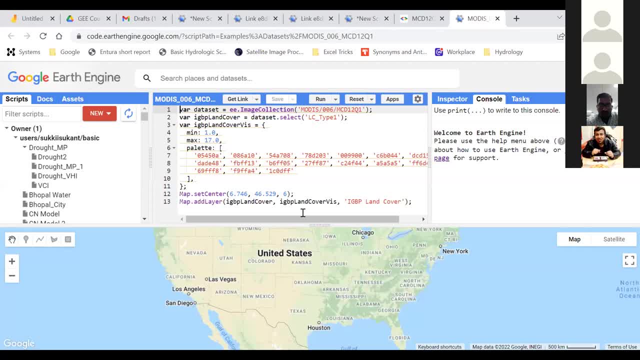 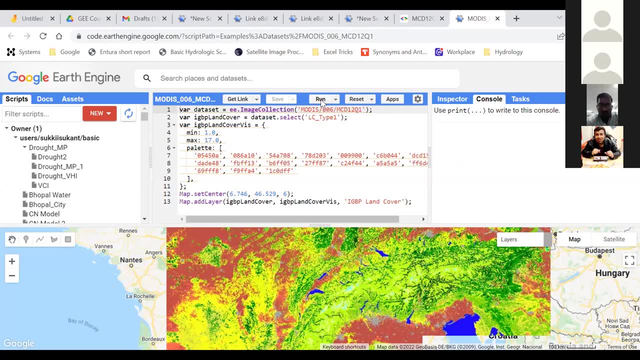 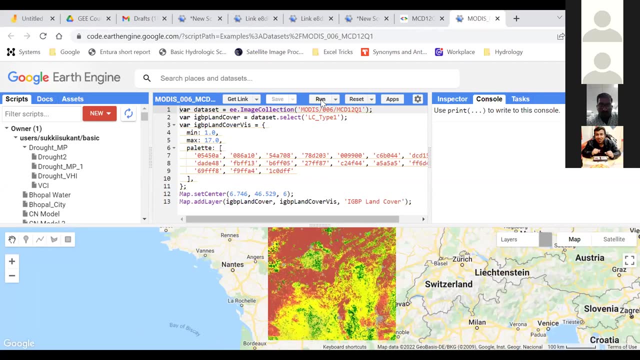 this data, available with the modest data set, will be displayed over here And I just need to click the run. Now I can see the LLC map of whole world in my Google search engine. Suppose if you want to do the LLC analysis for your area. 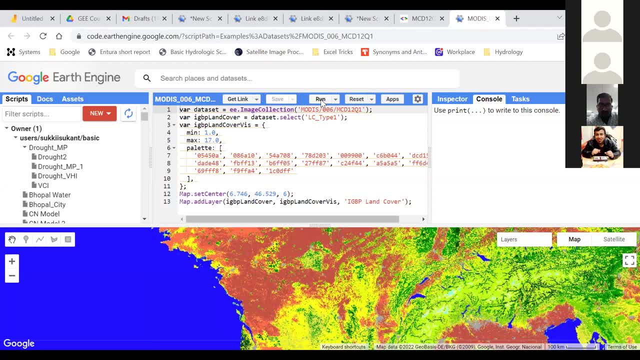 So what you will do in traditional methodology, you will download the LLC data set, You will create the mosaic, You will create some different, what we can say- color combination, symbology, play with the symbology. Then only you will get this map, But with just simple few lines of script. 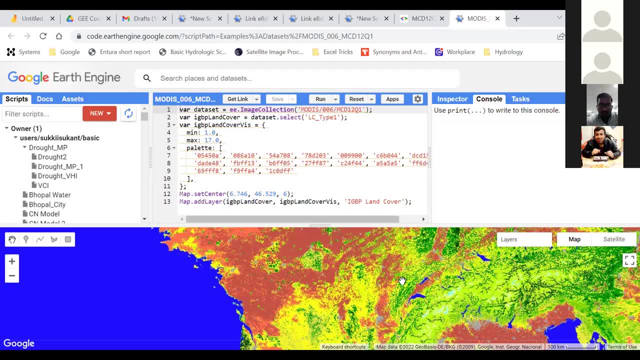 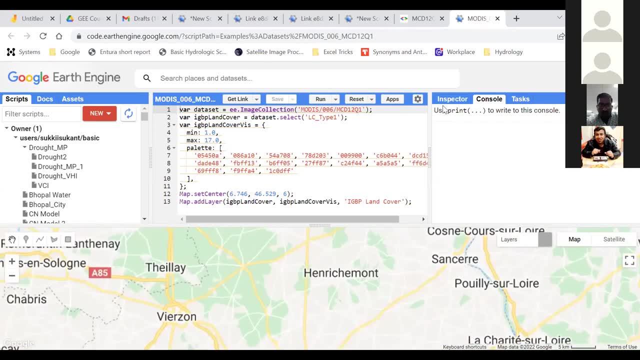 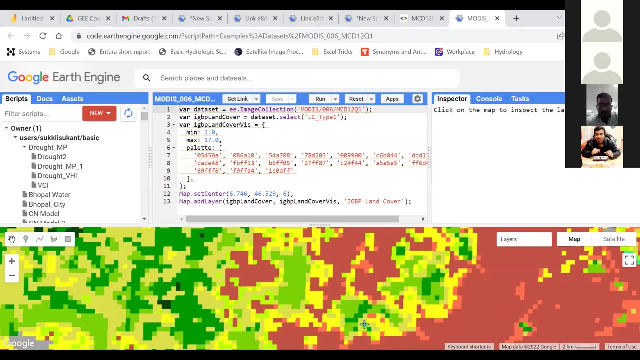 we can get this amount of data set in just few seconds. So if you go, if you zoom into any area, Okay, And if you go to the inspector task, you can see, you can click, click anywhere there. For example, if I click over this pixel. 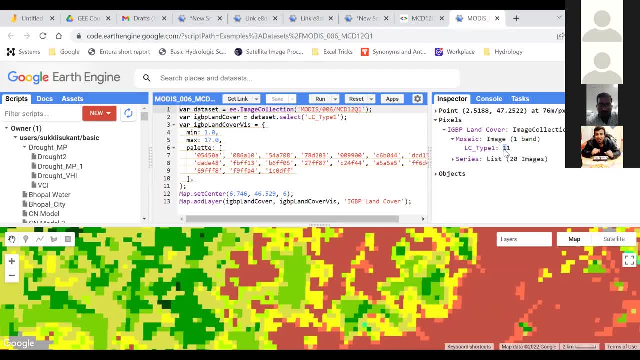 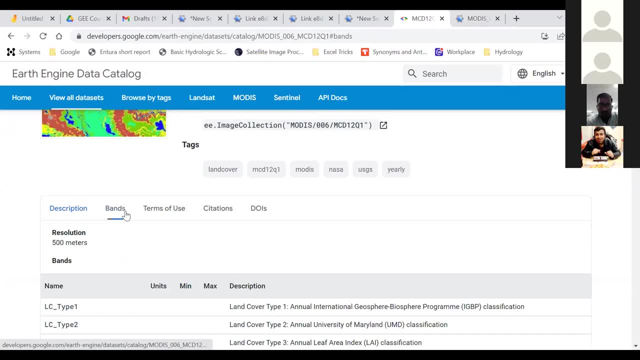 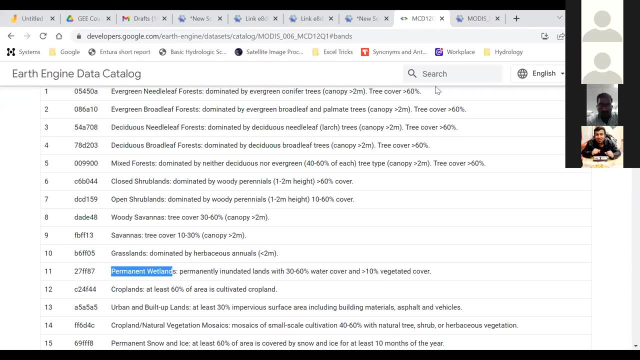 So I can see this. this is the class number 11.. And if I want to see what is actually class number 11 is, I go to this page of modest data set. I go to the band and see: class number 11 denotes the permanent red lines. 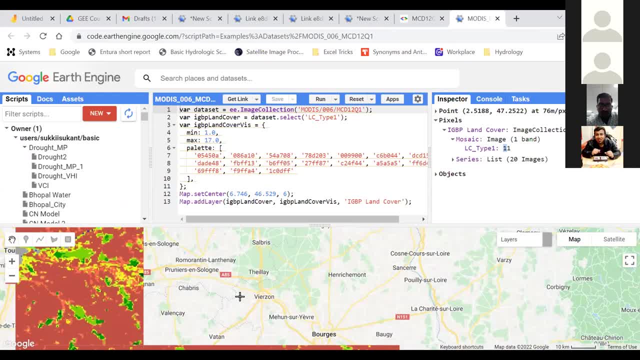 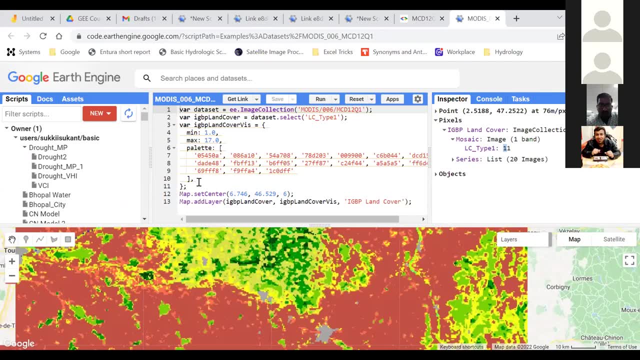 And similarly, I can extract the amount of information through this tab. So what we have to do? we don't want to display all this color palettes, We just want to get our data. So either we can copy these two lines, either from here: 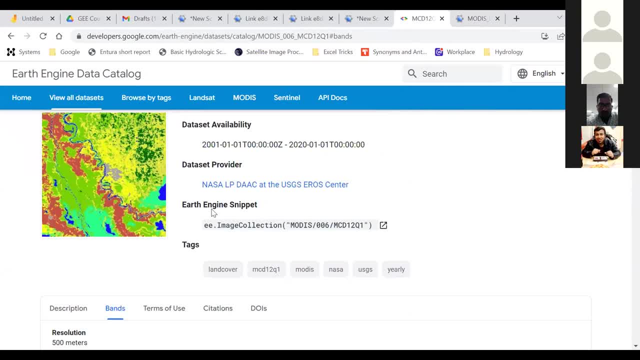 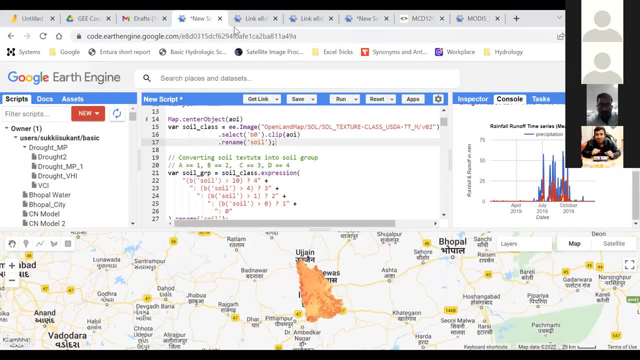 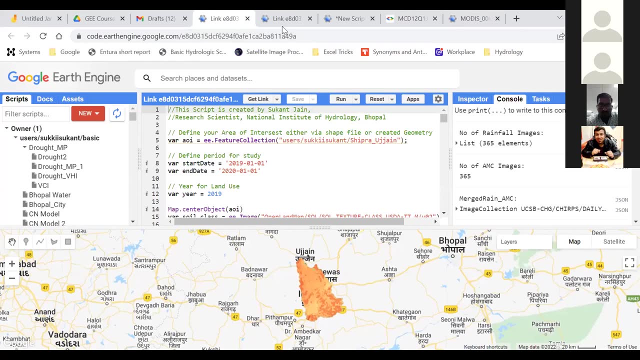 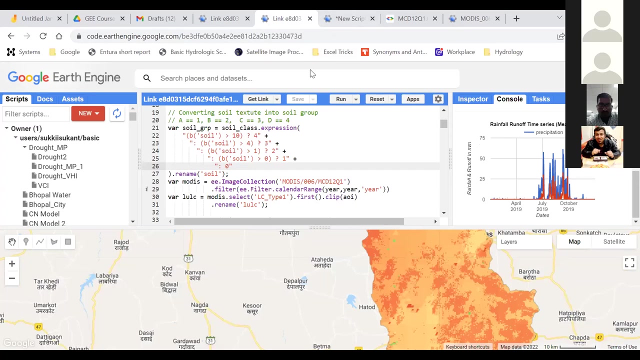 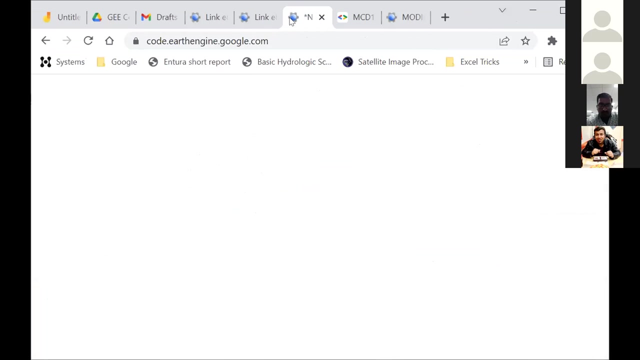 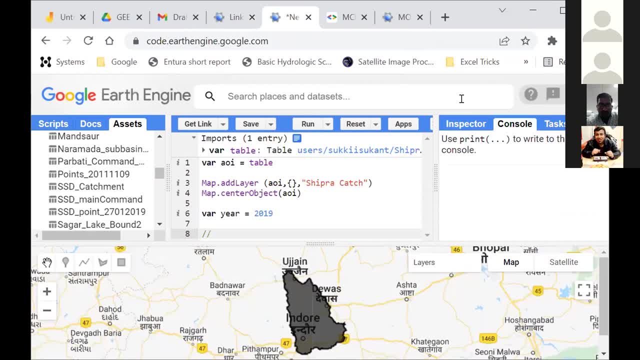 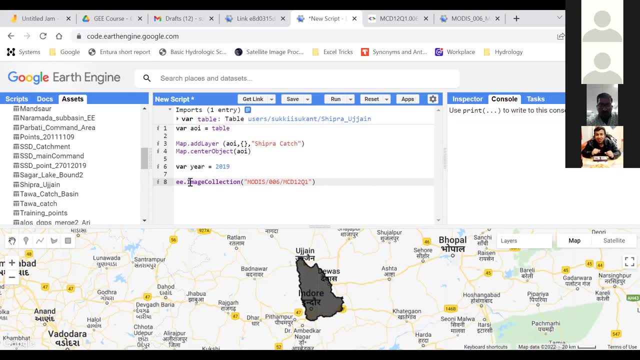 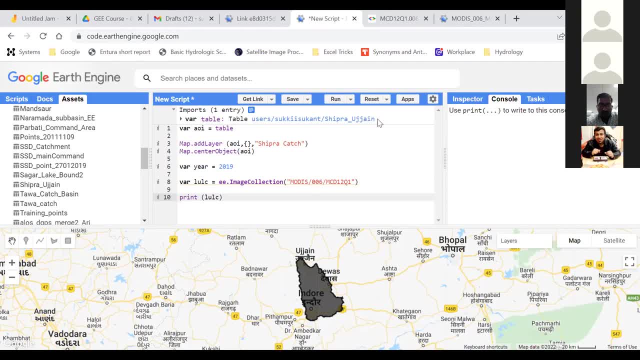 like war, LULC equal to EEimageCollectionModel, And if I print this data, that means LULC. what I will get in the console panel I can get. i can get there is an image collection of 20 elements because this data set is providing. 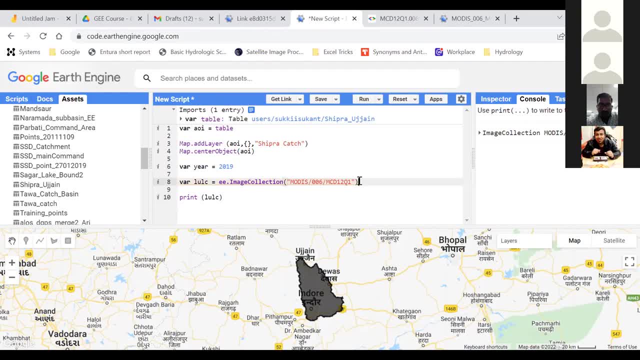 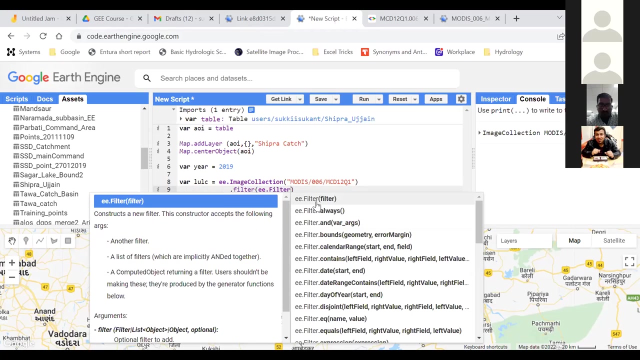 llc of 20 different years. so in order to filter from varieties of image collection to a single image, we can use a filter. so for applying filter, we just use dot filter. open the bracket. open ee filter and if i use control plus spacebar, i can see all the functions that are related to ee filter. 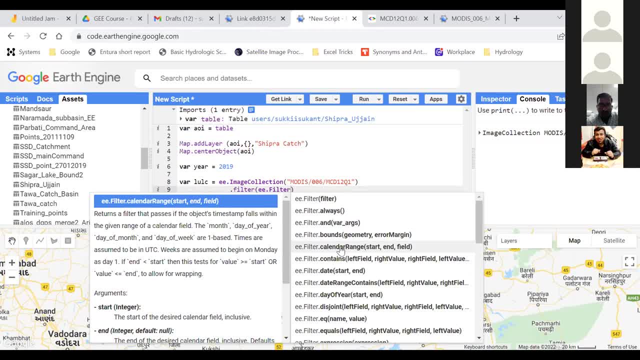 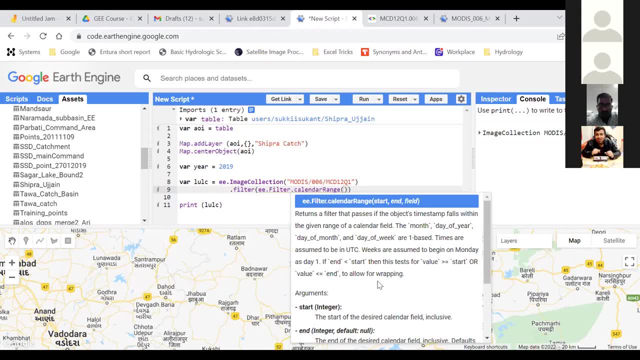 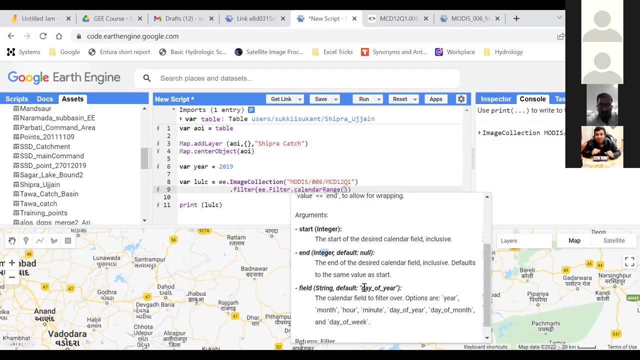 so presently i am going to use ee filter calendar range. okay, in this function there are asking three arguments: start year, end year and field. that means start in the form of integer and in the form of integer and field in the form of either integer and field in the form of either. 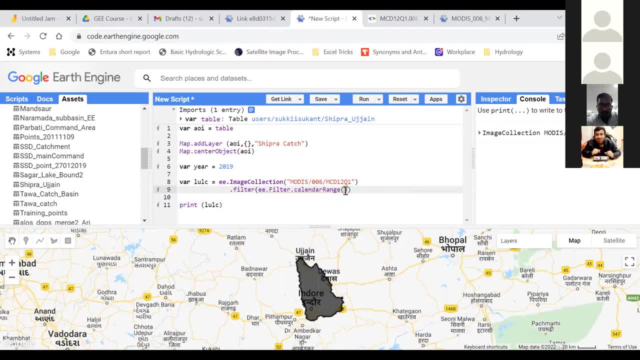 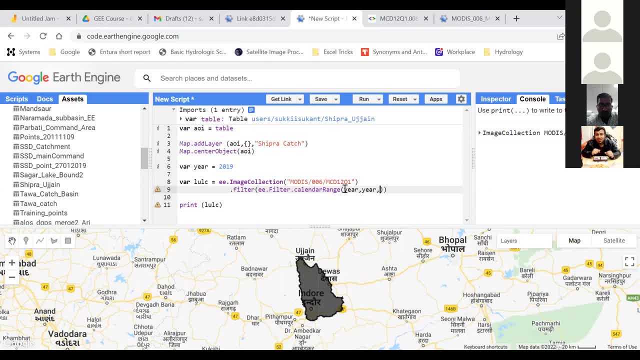 so what i will do. i will just type this. so what i will do. i will just type this here, here, here, here and in the brackets. i will type here, here and in the brackets. i will type here, here and in the brackets. i will type here and if i print, run again. 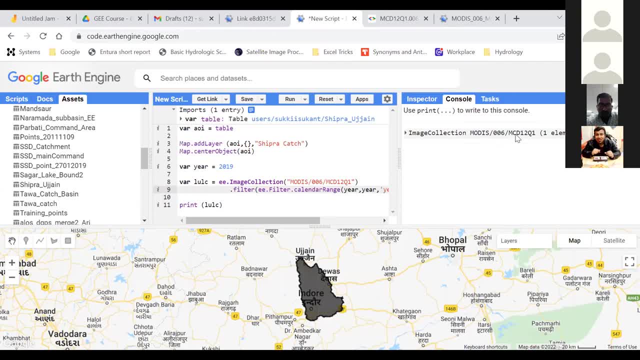 and if i print run again, and if i print run again, so now, so now, so now, this giving me uh this, giving me uh this, giving me uh llc of single year. that means only one llc of single year. that means only one llc of single year. that means only one element of two thousand and 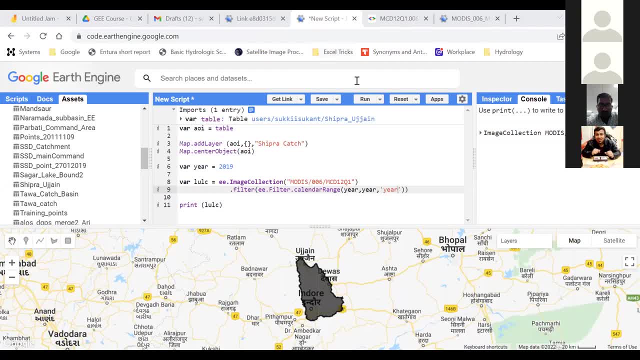 element of two thousand and element of two thousand and nineteen later on. uh, if you can see this later on, uh, if you can see this later on, uh, if you can see this. the earth engine has two, two type of the earth engine has two, two type of. 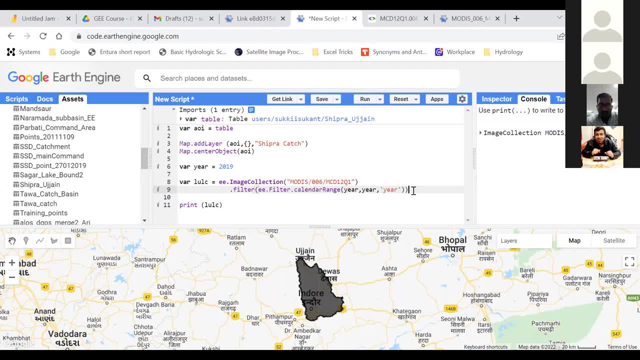 the earth engine has two, two type of images. one is image collection and images. one is image collection and images. one is image collection and another is image. image collection is another is image. image collection is, another is image. image collection is nothing, but when we have and when we have. 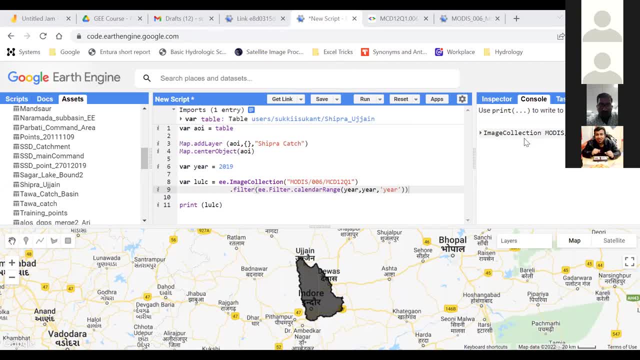 multiple images, then we are in the form multiple images, then we are in the form multiple images, then we are in the form of image collection. but when we perform of image collection, but when we perform of image collection, but when we perform, uh, we need to get only a single image. 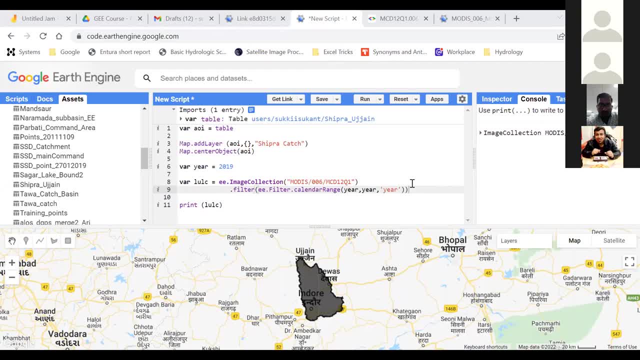 uh, we need to get only a single image. uh, we need to get only a single image. then it is in the form of image, then it is in the form of image, then it is in the form of image, collection, collection, collection. uh, image, not the image collection. so if 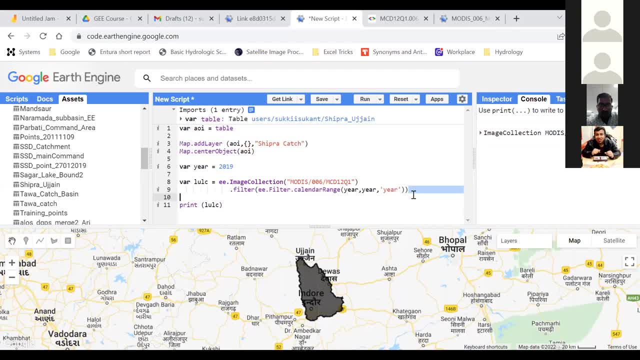 uh image, not the image collection. so if uh image, not the image collection, so if you want to convert this image collection, you want to convert this image collection, you want to convert this image collection of single image into a sing of single image, into a sing of single image, into a sing uh one image. what we can do, we can apply: 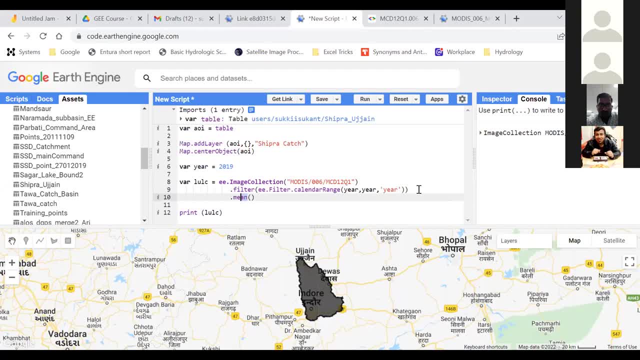 uh, one image, what we can do, we can apply. uh one image, what we can do, we can apply either mean, either mean, either mean, we can write median, we can write median, we can write median. or we can simply write mosaic. or we can simply write mosaic or we can simply write mosaic, we just simply write first. 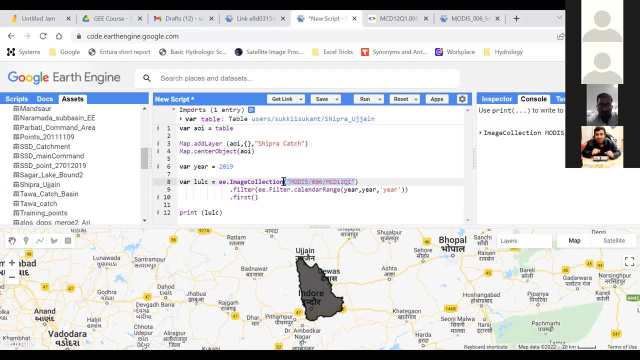 we just simply write first. we just simply write first. so what it will do first of all, it will. so what it will do first of all, it will. so what it will do first of all, it will gather all the stores data set with the. gather all the stores data set with the. 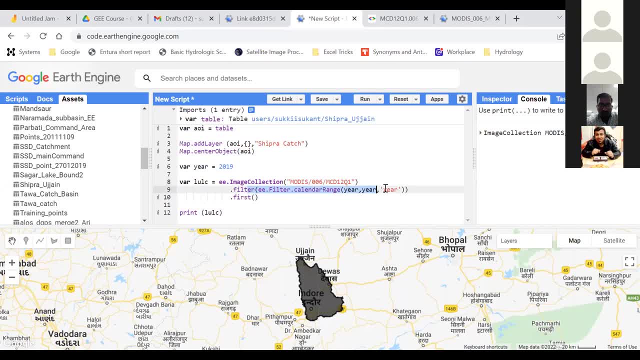 gather all the stores data set with the this code. then it will filter our image. this code, then it will filter our image. this code. then it will filter our image with this, with this, with this particular year. then it will select the particular year. then it will select the. 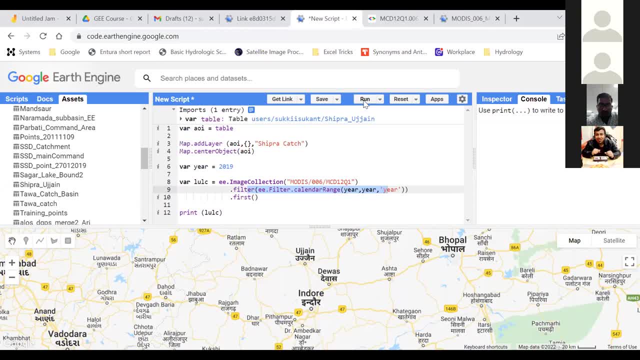 particular year, then it will select the first image and if i click run so we can get this. if this particular so we can get this. if this particular, so we can get this. if this particular image has total 13 bands. image has total 13 bands. image has total 13 bands. and if i go to the page, 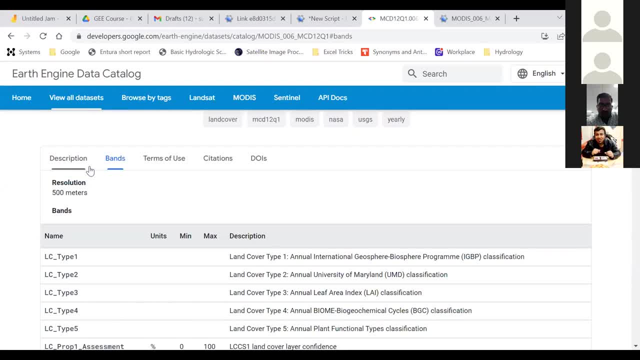 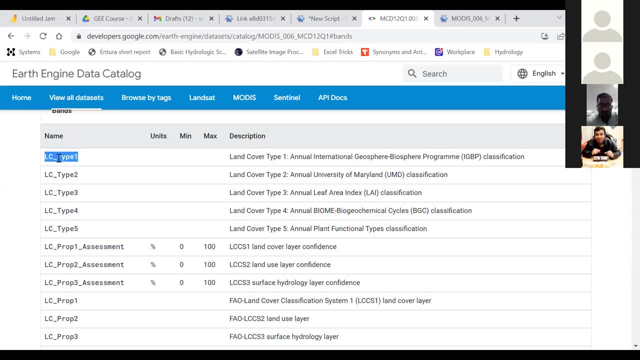 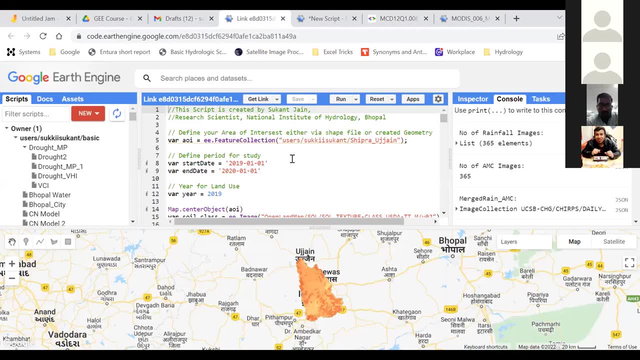 we can see l2125 total 13 bands. we can see l2125 total 13 bands. but we are interested only in this band, but we are interested only in this band, but we are interested only in this band. that means that means, that means lc type one. 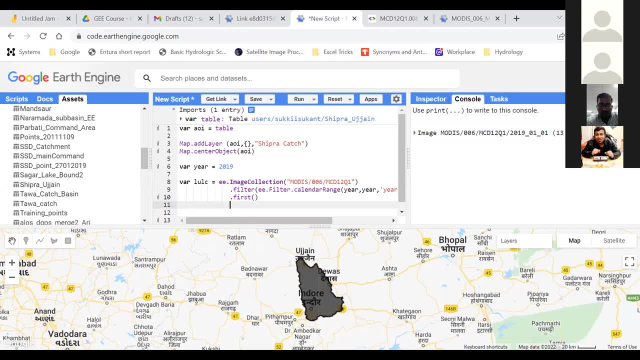 so i will do select. we will, so i will do select. we will, so i will do select. we will write dot. and what is the band name it is in the? and what is the band name it is in the? and what is the band name it is in the commas, lc underscore. 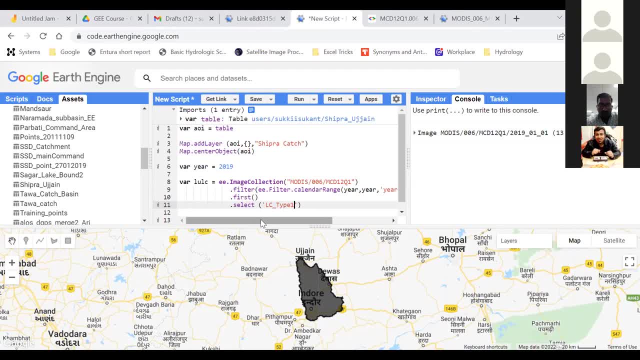 commas lc. underscore. commas lc underscore p y p e 1. p y p e 1, p y p e 1. and let's see if i, and let's see if i and let's see if i. just so now we have filter our image from 13. 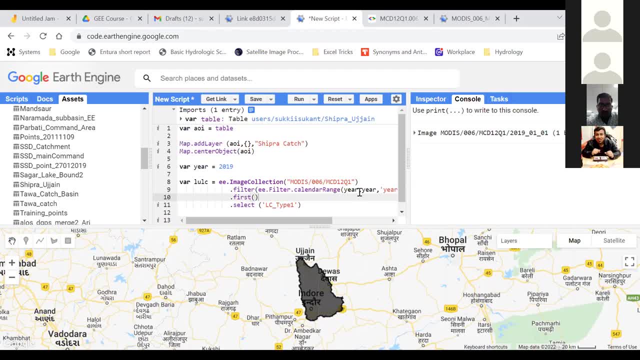 so now we have filter our image from 13. so now we have filter our image from 13 from 20 different image collection to a. from 20 different image collection to a. from 20 different image collection to a single image- single image, single image. and from 13 different bands to a single. 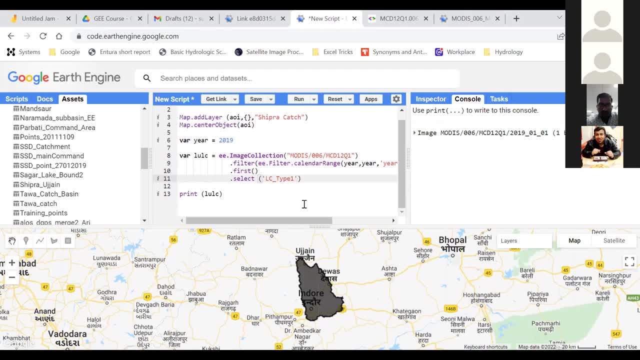 and from 13 different bands to a single and from 13 different bands to a single: band with the name, band with the name. band with the name lc type 1- okay, and if you want to change lc type 1, okay. and if you want to change. 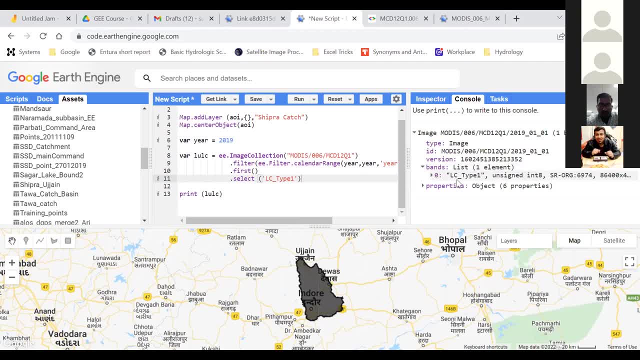 lc type 1. okay, and if you want to change, if i just open this image and open the, if i just open this image and open the, if i just open this image and open the band, so the band name is lc type 1 band. so the band name is lc type 1. 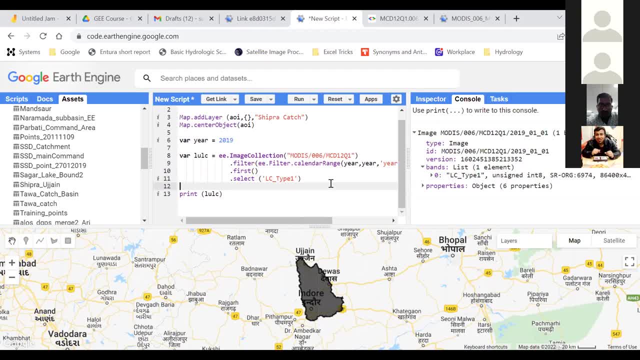 band. so the band name is lc type 1. so if i want to change the name of this, so if i want to change the name of this, so if i want to change the name of this band, i can simply band. i can simply band, i can simply type dot name. 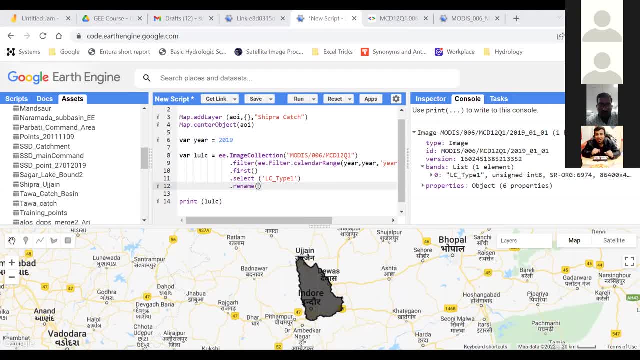 type dot name. type dot name, and i can give the band name as, and i can give the band name as, and i can give the band name as either lulc or either lulc or either lulc or for example, for example, for example. you will see, and i just 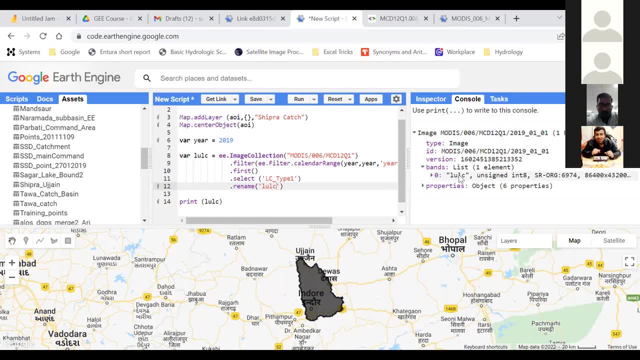 if i open this image, i can see this now. if i open this image, i can see this now. if i open this image, i can see this now: it has only a single band with the name. it has only a single band with the name. it has only a single band with the name lvc. 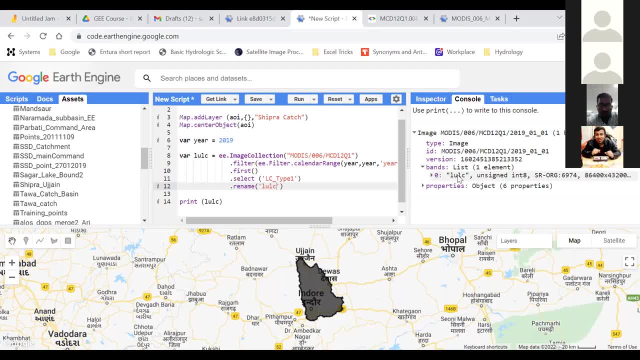 lvc, lvc, lvc- that means 20 years of data set. we have that means 20 years of data set. we have that means 20 years of data set. we have filter only for our respective year. filter only for our respective year. filter only for our respective year. we have converted this image collection. 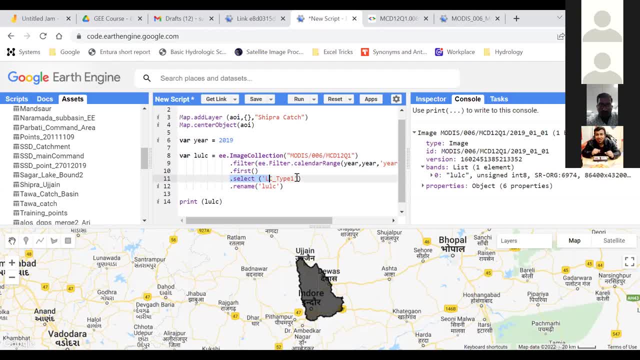 we have converted this image collection. we have converted this image collection into a single image. we have selected into a single image. we have selected into a single image. we have selected from 13 different band to a single band, from 13 different band to a single band. 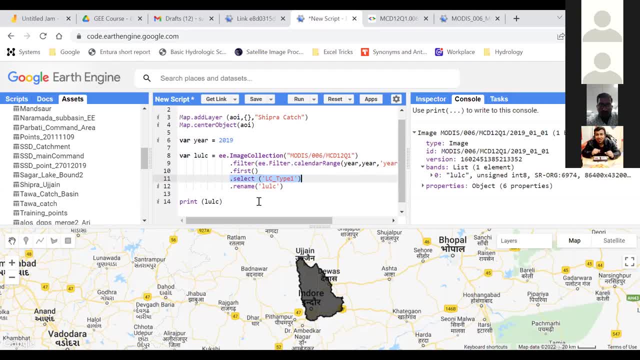 from 13 different band to a single band and we have renamed our and we have renamed our and we have renamed our band name. and if i band name, and if i band name, and if i uh instead of print, if i just use map, uh instead of print, if i just use map. 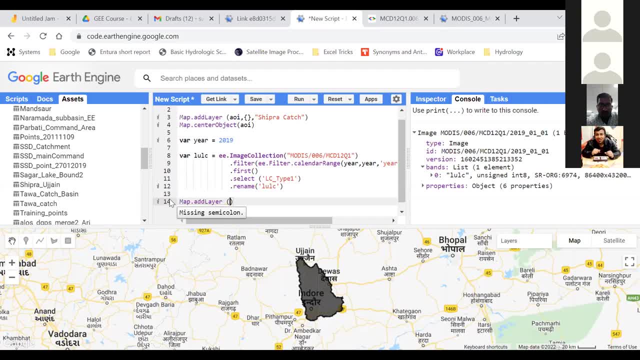 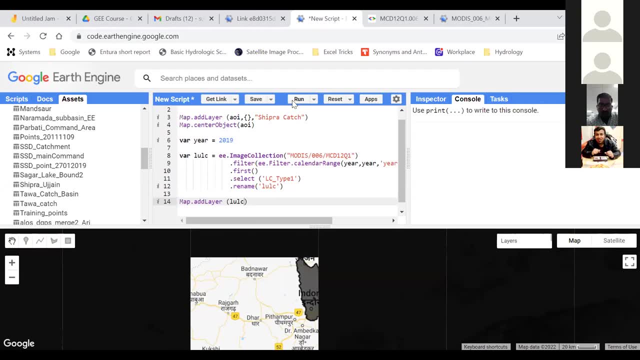 uh, instead of print, if i just use map dot, add layer and type lulc- that means variable name, and type lulc- that means variable name, and type lulc- that means variable name. if i click run. okay, now you can see this over my in the. okay, now you can see this over my in the. 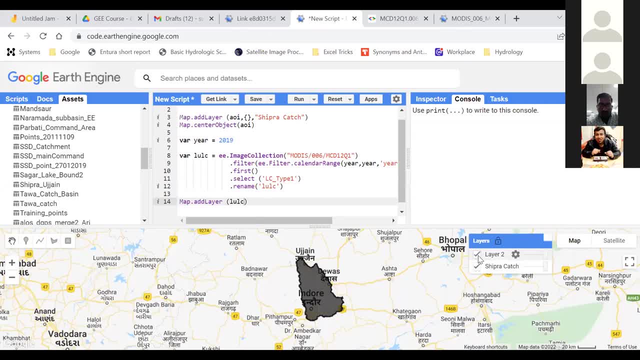 okay, now you can see this over my. in the layer tab there are two layers. there is layer tab. there are two layers. there is layer tab. there are two layers. there is shipwreck admin and layer two, shipwreck admin and layer two, shipwreck admin and layer two, and layer two is nothing but our. 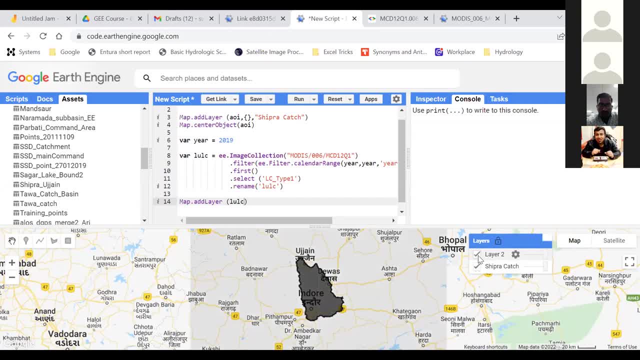 and layer two is nothing but our and layer two is nothing but our land use land cover, but land use land cover, but land use land cover. but in the visualization it is not looking. in the visualization it is not looking. in the visualization it is not looking good. so we can always change the 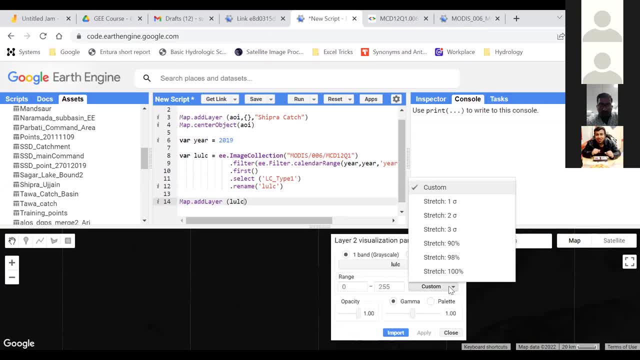 good, so we can always change the good, so we can always change the visualization, visualization. visualization by clicking this gear sign and clicking, by clicking this gear sign and clicking, by clicking this gear sign and clicking on this, on this, on this stretch hundred percent because we have stretch hundred percent, because we have 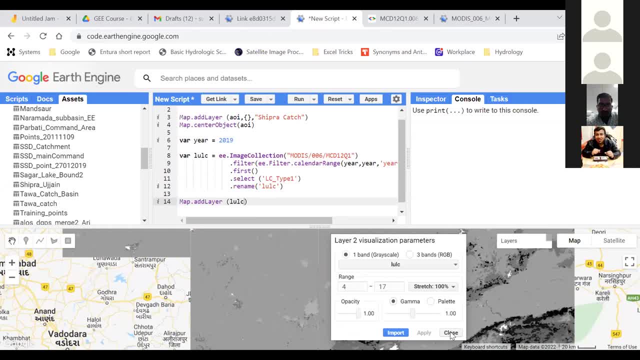 stretch hundred percent because we have class range from 1 class range from 1 class, range from 1, 4 to 17. we click apply now we get the 4 to 17. we click apply now we get the 4 to 17. we click apply now we get the land use, land cover in the. 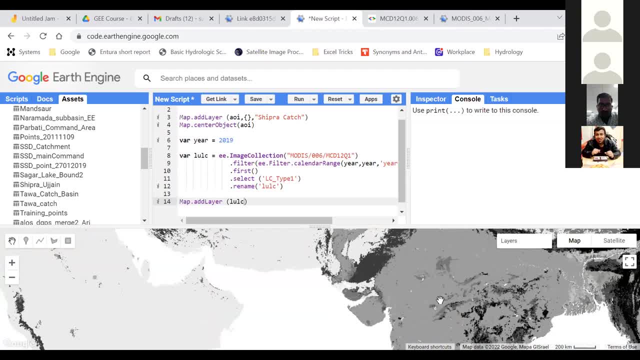 land use land cover in the land use land cover in the black and white format. and if we black and white format and if we black and white format and if we incorporate the palette that were given, incorporate the palette that were given, incorporate the palette that were given in the 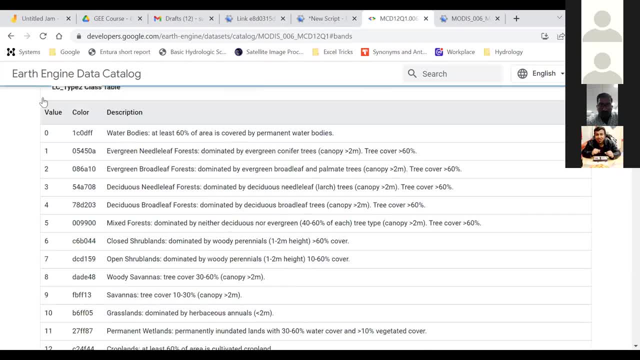 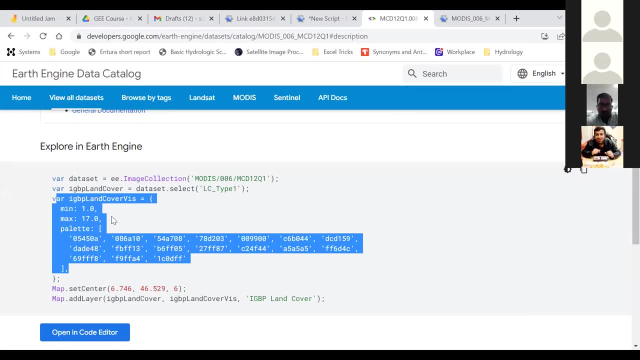 that we're giving in this code, that we're giving in this code, that we're giving in this code: if i go to the, if i go to the, if i go to the description, if i use this color palette description, if i use this color palette description, if i use this color palette, so we can convert this black and white. 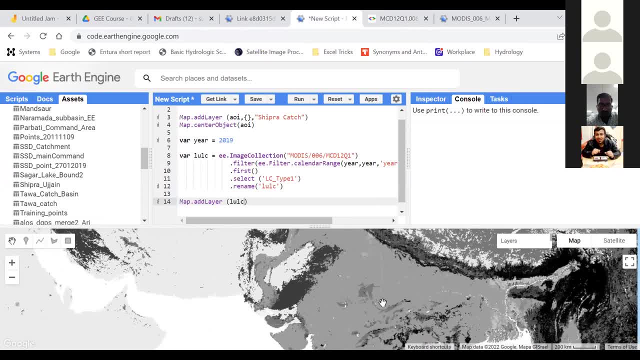 so we can convert this black and white, so we can convert this black and white image into a beautiful color, but image into a beautiful color, but image into a beautiful color. but presently we are not looking for the presently, we are not looking for the presently, we are not looking for the beautification, we are just looking for. 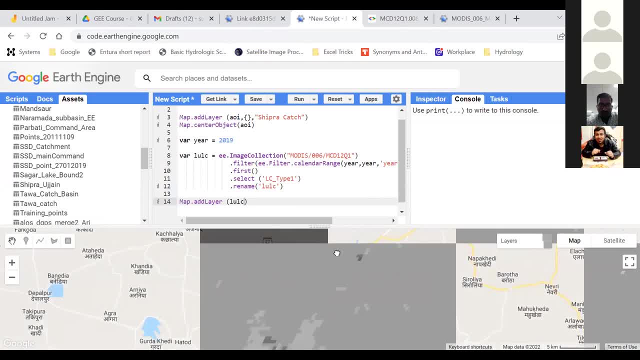 beautification. we are just looking for beautification, we are just looking for the information inspection, the information inspection, the information inspection. so, if i zoom to my area and, if i want so, if i zoom to my area and if i want so, if i zoom to my area and if i want to explore the land use and cover classes, 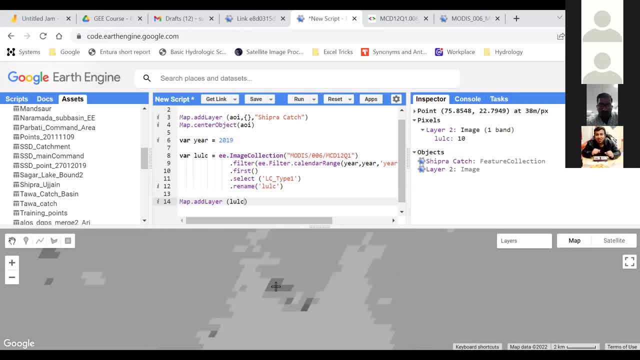 to explore the land use and cover classes. to explore the land use and cover classes of this pixel, i go to the inspector. i'll just click this and we can see the. i'll just click this and we can see the. i'll just click this and we can see the lulc of this particular thing is. 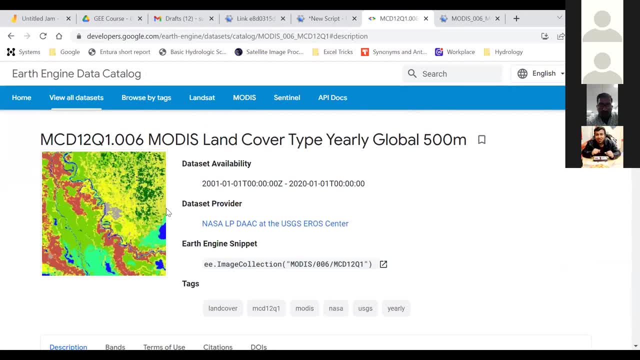 lulc of this particular thing is lulc of this particular thing is lulc 10. and if i go to this tab- lulc 10- and if i go to this tab- lulc 10- and if i go to this tab, i go to the pants. 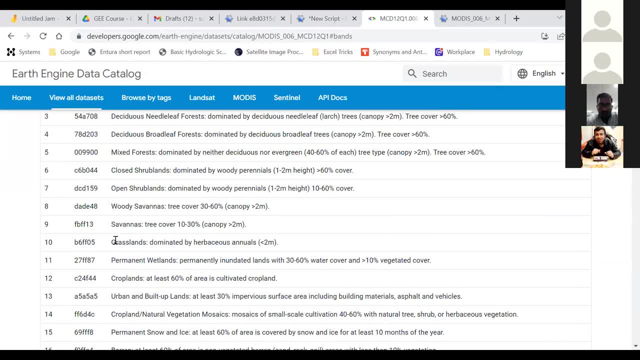 i go to the pants. i go to the pants, i can get the. i can get the. i can get the. lulc 10 means it is a grassland. lulc 10 means it is a grassland. lulc 10 means it is a grassland dominated by. 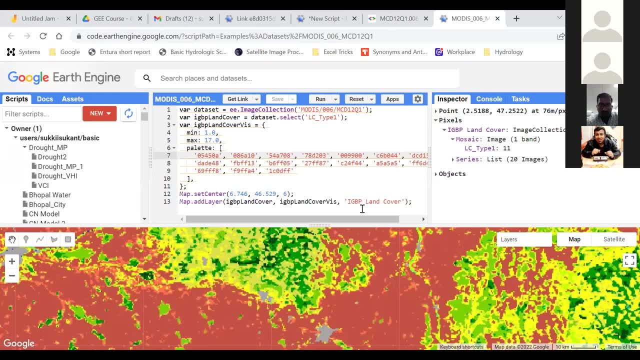 dominated by. dominated by herbaceous animals. herbaceous animals, herbaceous animals. so this is how we can actually get the. so this is how we can actually get the. so this is how we can actually get the data set of lulc. similarly, we can get data set of lulc. similarly, we can get: 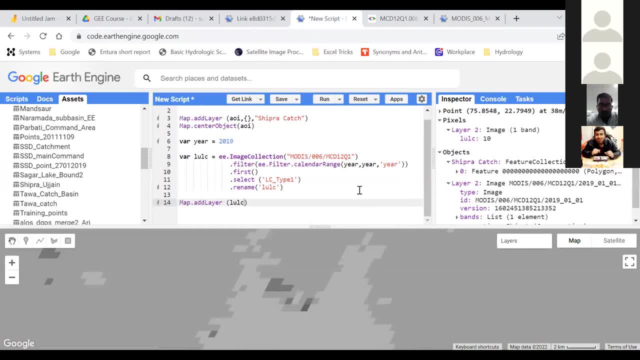 data set of lulc. similarly, we can get the data set of the data set of the data set of soil and etc. so next thing that we are soil and etc, so next thing that we are soil and etc. so next thing that we are going to do is actually extract the 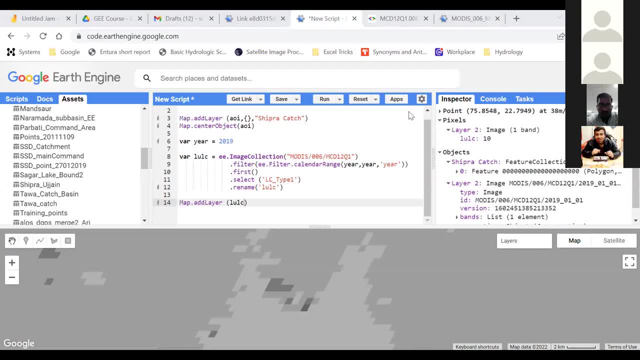 going to do is actually extract the going to do is actually extract the soil data set and after that i'm going to soil data set, and after that i'm going to soil data set and after that i'm going to share this amount of code. share this amount of code. 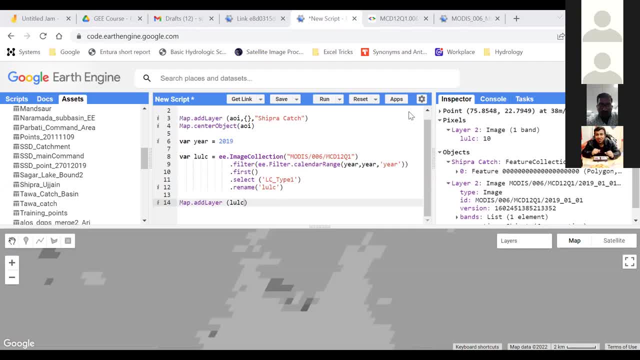 share this amount of code with you, and you can do on your own and with you, and you can do on your own and with you, and you can do on your own and you can put your ocean after that. so, in order to explore the soil data, so, in order to explore the soil data, 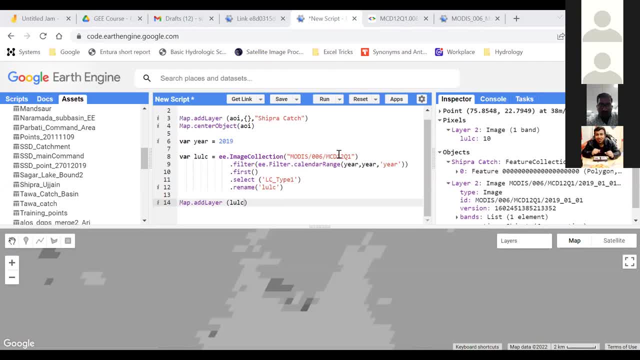 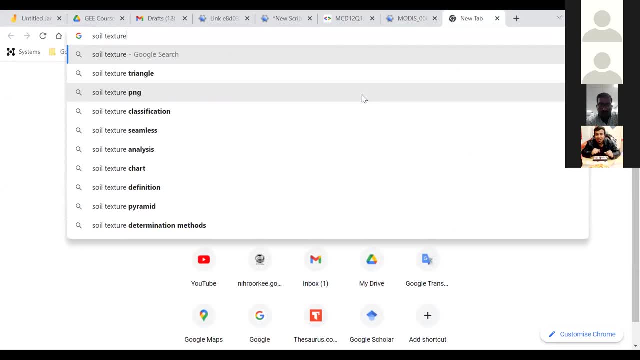 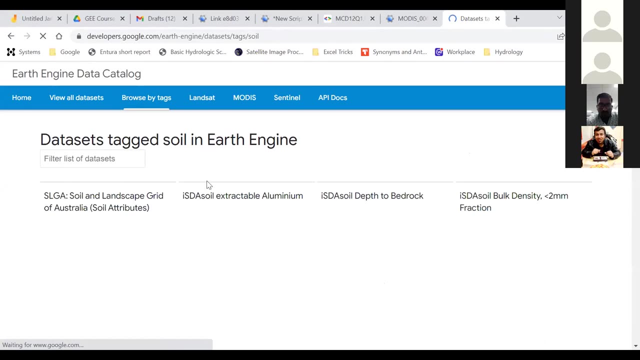 so, in order to explore the soil data set similarly, what we can do? we can simply type soil texture. we can simply type soil texture. we can simply type soil texture data if i open the data set tagged as soil, if i open the data set tagged as soil. 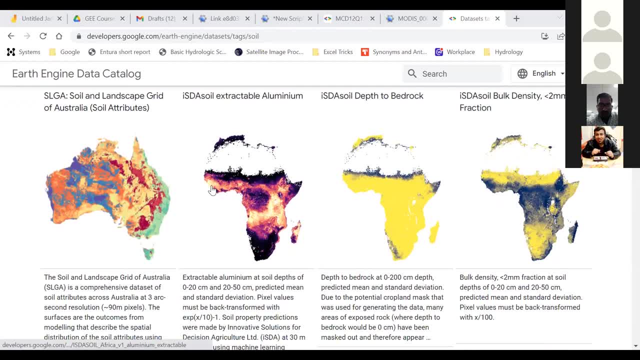 if i open the data set tagged as soil texture, texture, texture, so there are varieties of data, but there. so there are varieties of data but there. so there are varieties of data, but there are very only few data set related to. are very only few data set related to. 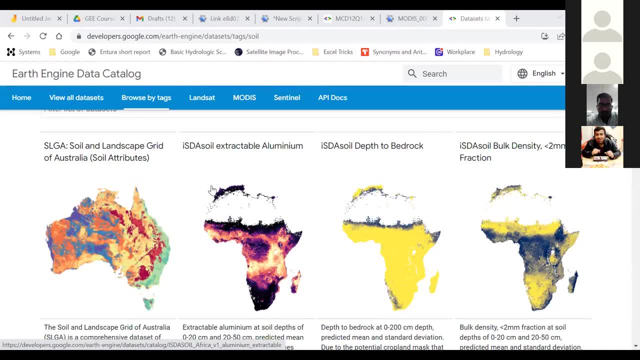 are very only few data set related to soil texture available for whole world. soil texture available for whole world. soil texture available for whole world or specifically for india. suppose these or specifically for india. suppose these or specifically for india. suppose these are the soil texture for us. are the soil texture for us? 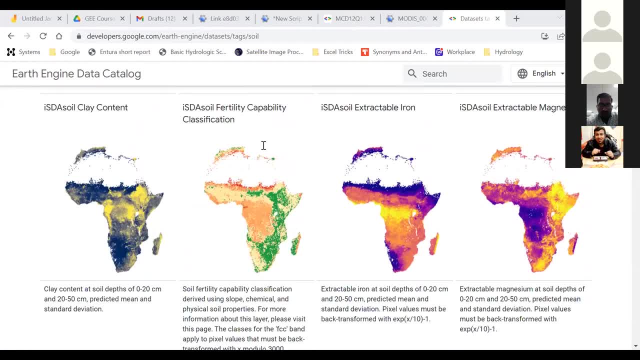 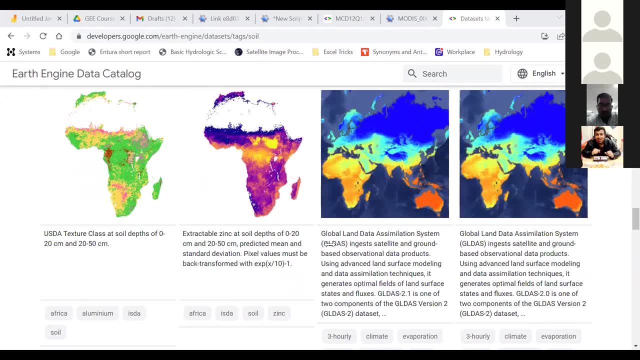 are the soil texture for us? philia only. these are for the africa only, philia only. these are for the africa only, philia only. these are for the africa only. so there is a uh soil data set. so there is a uh soil data set. so there is a uh soil data set, if i just 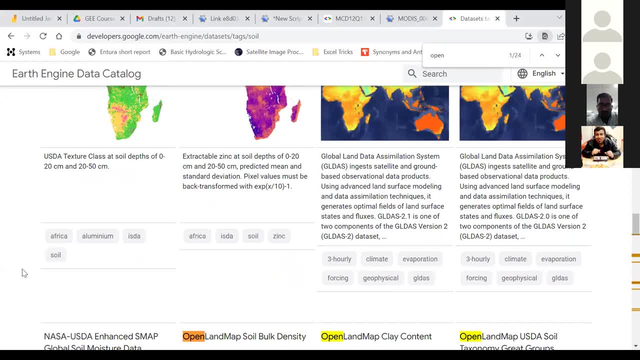 just simply type, simply type, simply type one one one land map, land map, land map. so so. so these are few data sets like open soil. these are few data sets like open soil. these are few data sets like open soil bulk density. open soil clay content. bulk density- open soil clay content. 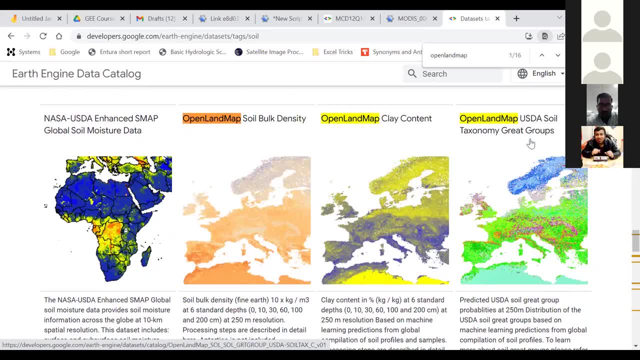 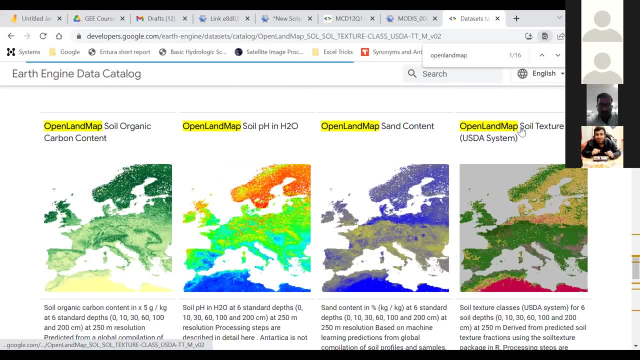 bulk density- open soil clay content. open bulk density- open soil clay content. open land map uh usga soil taxonomy- open land map uh usga soil taxonomy- open land map uh usga soil taxonomy. soil organic carbon content- soil ph. soil organic carbon content- soil ph. soil organic carbon content soil ph. soil texture data. if i open this, 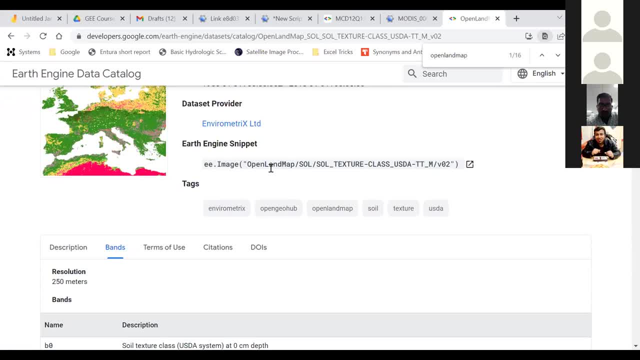 so these are the agency, the data set. so these are the agency, the data set. so these are the agency, the data set provider. and this is the earth index provider and this is the earth index provider and this is the earth index snippet, snippet, snippet. and here, in this image, this is the have. 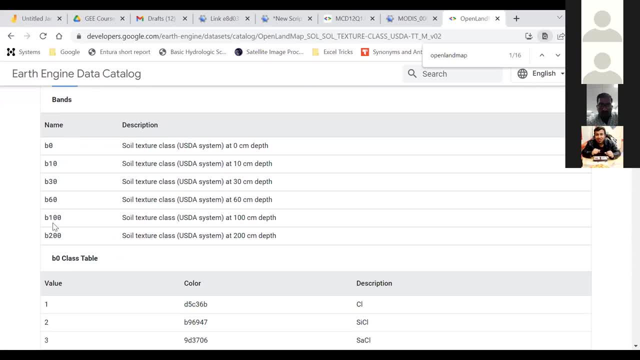 and here in this image, this is the have. and here in this image, this is the have. a resolution of 250 meters. a resolution of 250 meters, a resolution of 250 meters. they have five to six bands. b0 is soil. they have five to six bands b0 is soil. 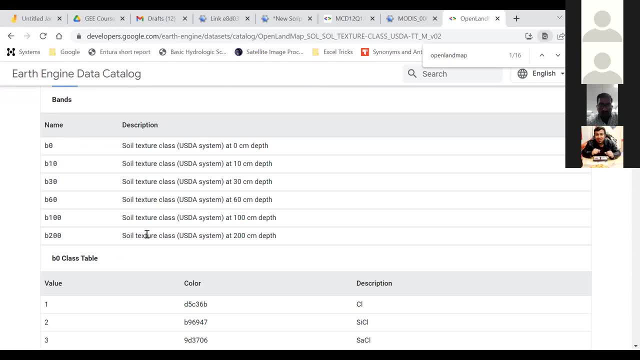 they have five to six bands: b0 is soil texture class at zero centimeter depth. texture class at zero centimeter depth. texture class at zero centimeter depth and b2 double zero is a full texture and b2 double zero is a full texture and b2- double zero is a full texture class at two double zero centimeter depth. 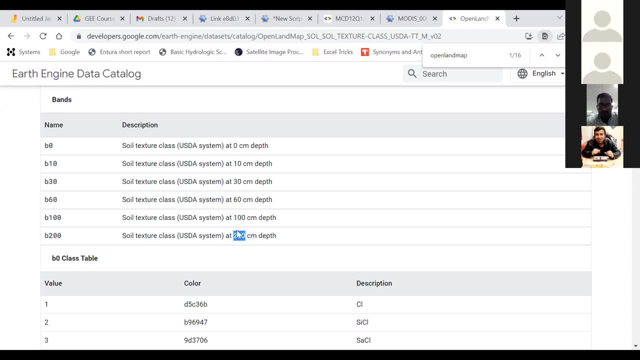 class at two double zero centimeter depth. class at two double zero centimeter depth. so if you are looking for different uh, so if you are looking for different uh, so if you are looking for different uh. soil classification for different level. soil classification for different level. soil classification for different level. you can get this data set, but the 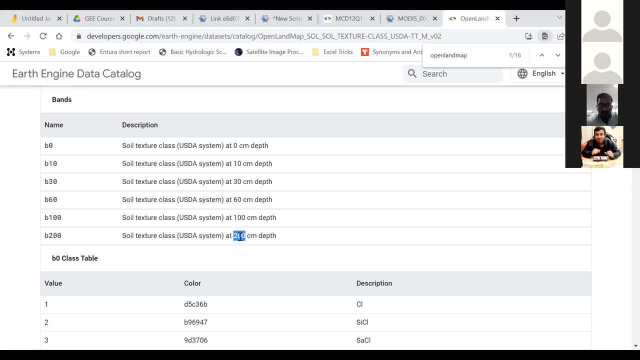 you can get this data set, but the you can get this data set, but the accuracy of these data set, specifically, accuracy of these data set, specifically, accuracy of these data set specifically in india, is not very good. why? because in india is not very good. why? because in india is not very good? why? because these data sets are. we have been 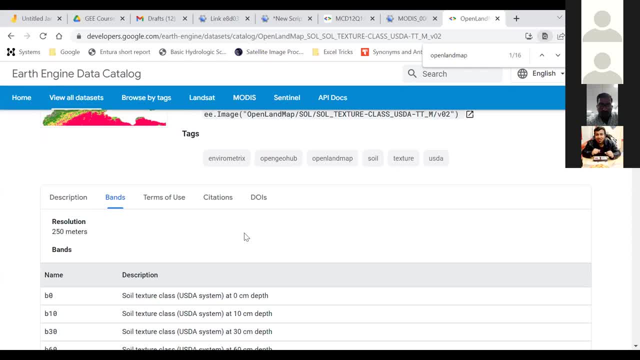 these data sets are, we have been. these data sets are, we have been prepared with the prepared, with the prepared, with the, with a very huge amount of ground survey, with a very huge amount of ground survey, with a very huge amount of ground survey and most of the ground survey samples. 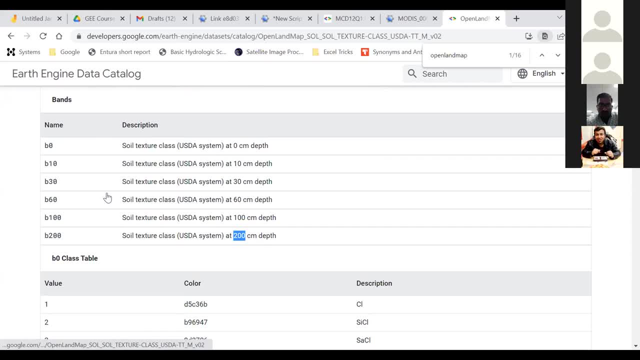 and most of the ground survey samples and most of the ground survey samples has been done, has been done, has been done specifically in their own region, that specifically in their own region, that specifically in their own region. that means european means european means european. so you cannot totally rely for the soil. 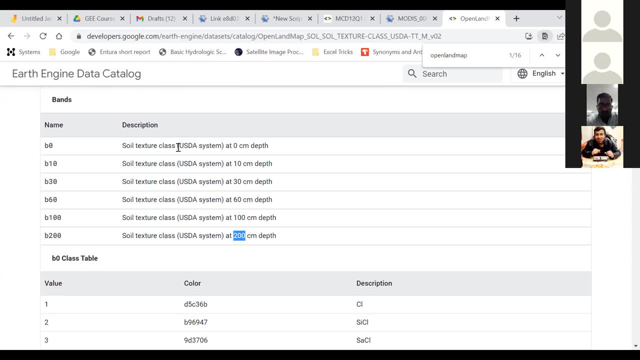 so you cannot totally rely for the soil, so you cannot totally rely for the soil texture for the lower region, but for the texture for the lower region, but for the texture for the lower region, but for the upper region. that means upper region, that means upper region, that means at this surface. you can use this data. 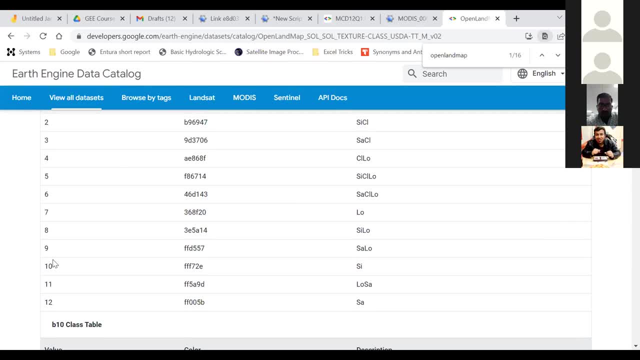 at this surface, you can use this data. at this surface you can use this data set set, set and they have a different classes up to and they have a different classes up to and they have a different classes up to class number 12. class number 12. 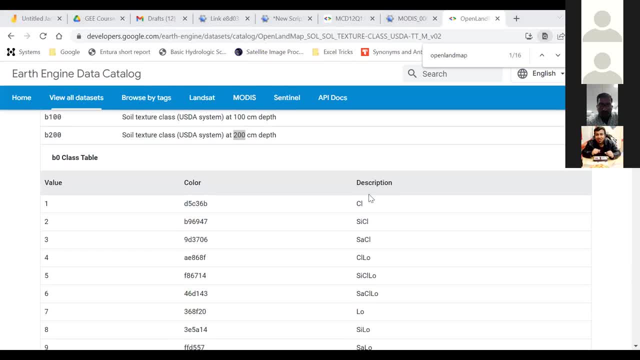 class number 12 and in the description they have written and in the description they have written and in the description they have written that class number one denotes cl. that class number one denotes cl. that class number one denotes cl means clay soil. class number five denotes means clay soil. class number five denotes: 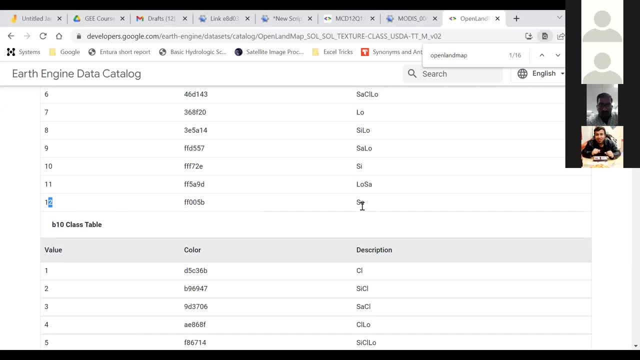 means clay soil. class number five denotes cell clay lomi and class number 12 denotes cell clay lomi and class number 12 denotes cell clay lomi and class number 12 denotes send sandy, send sandy, send sandy. so similarly you can convert this. so similarly you can convert this. 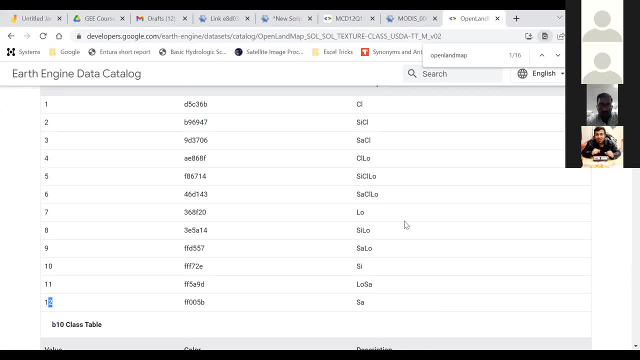 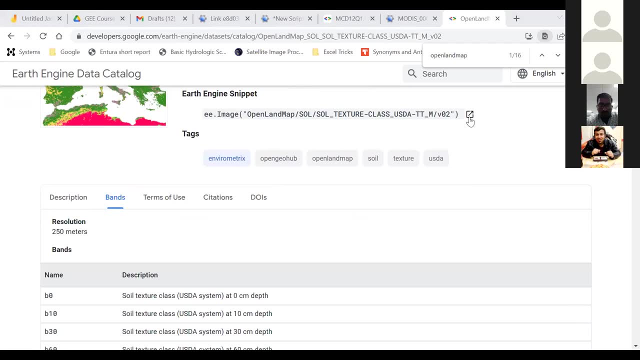 so, similarly, you can convert this classification into class abc, classification into class abc, classification into class abc. so, first of all, we will open this data. so, first of all, we will open this data. so, first of all, we will open this data set. by using this, now you will look how we. 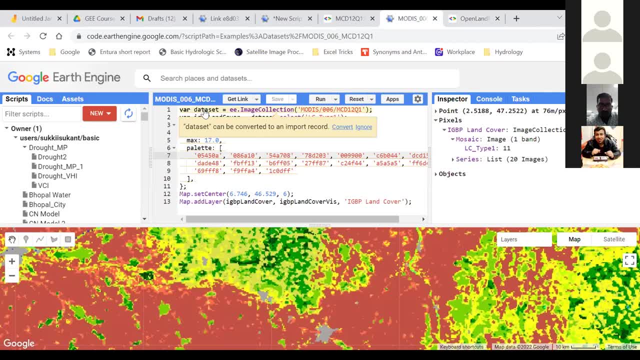 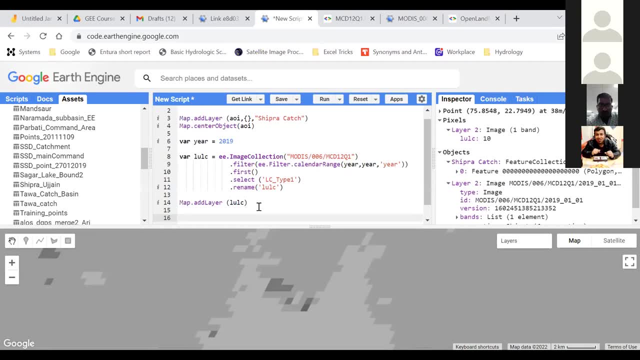 by using this now, you will look how we by using this now, you will look how we can can can use the similar. okay, now this is about the llc class. okay, now, this is about the llc class. okay, now we will open the soil data set variable. 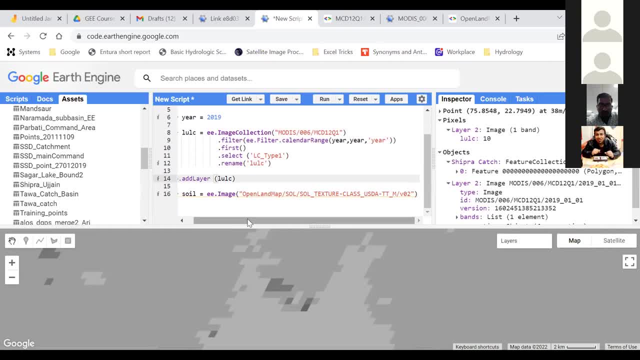 we will open the soil data set variable. we will open the soil data set variable: soil, soil, soil. we put the code: what we have copied now. we put the code: what we have copied now. we put the code: what we have copied now. this is not the image collection, this is 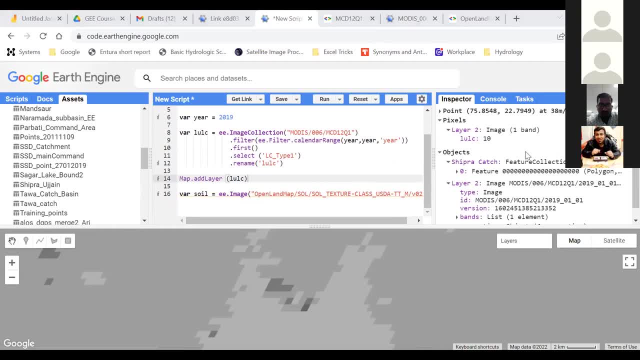 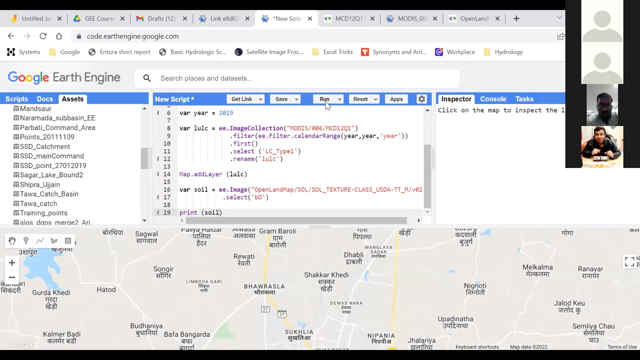 this is not the image collection. this is. this is not the image collection. this is a single image. a single image, a single image. okay, and? and we have to select a single band. that means b0, that means b0. and if i click print, see what will happen. 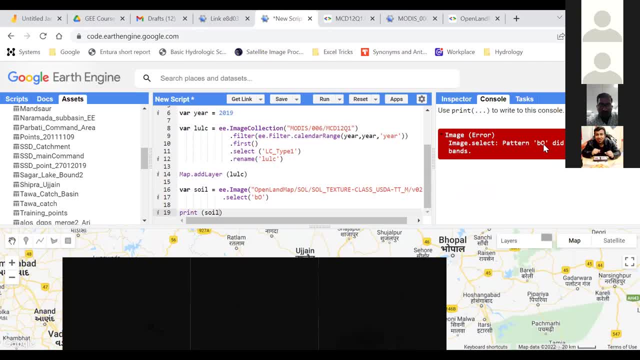 in the console there is an error. because in the console there is an error. because in the console there is an error. because it is written that it is written that it is written that b0 is not any band. uh, if i just b0 is not any band. uh, if i just. 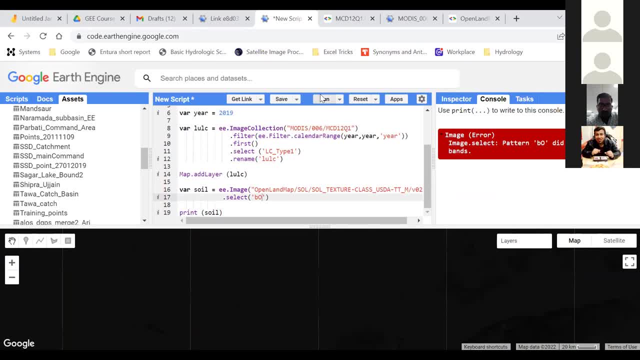 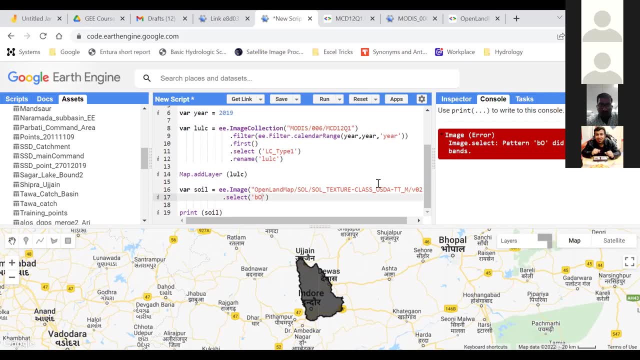 b0 is not any band. uh, if i just: it is not actually b0, it may be b. it is not actually b0, it may be b0. it is not actually b0, it may be b0. it is not actually b0, it may be b0. 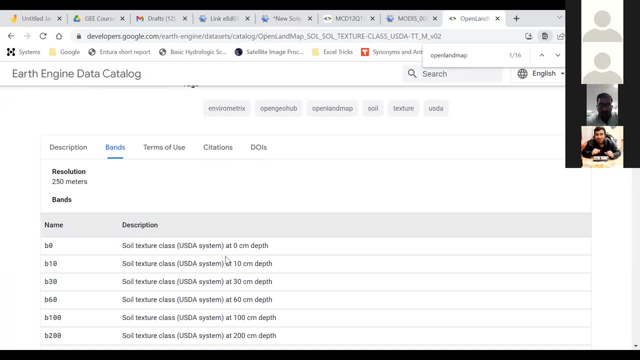 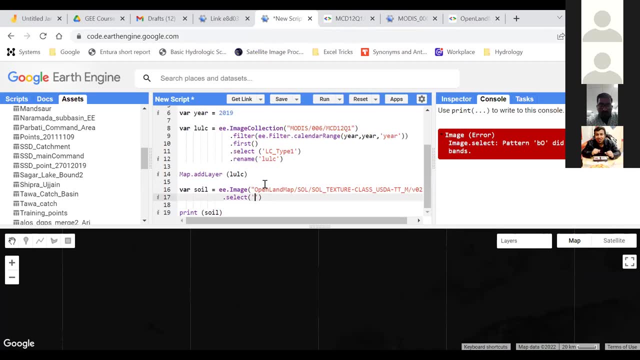 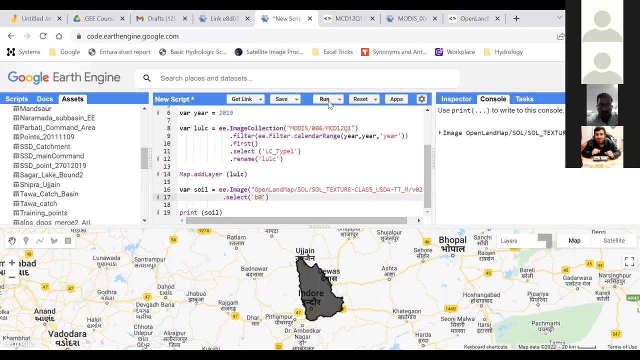 i guess using some wrong space. maybe i guess using some wrong space. maybe i guess using some wrong space, maybe or simply i just copy: it is b0, but initially i was typing bo. it is b0, but initially i was typing bo. it is b0, but initially i was typing bo. so now you can see there is a single map. 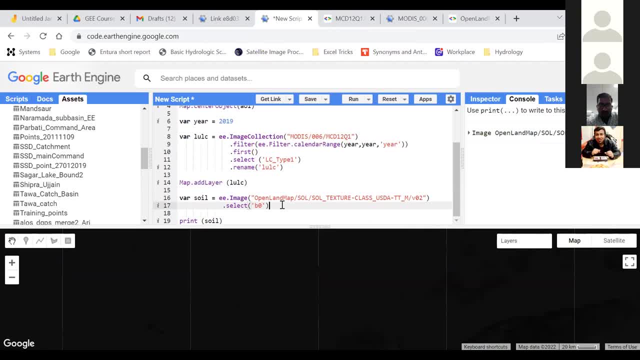 so now you can see there is a single map. so now you can see there is a single map. okay, okay, okay. of open land map, now what we can do. of open land map, now what we can do. of open land map, now what we can do. we can simply: 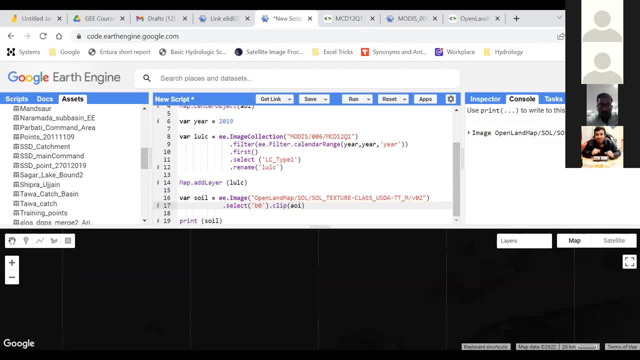 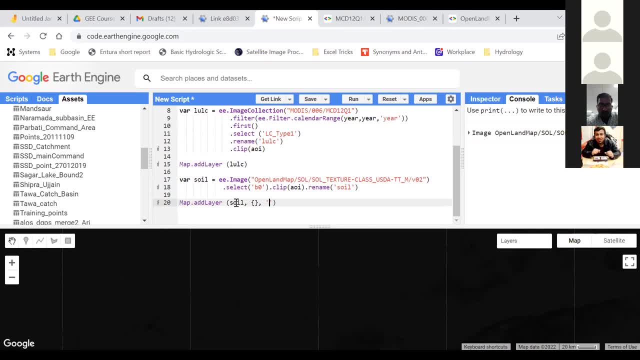 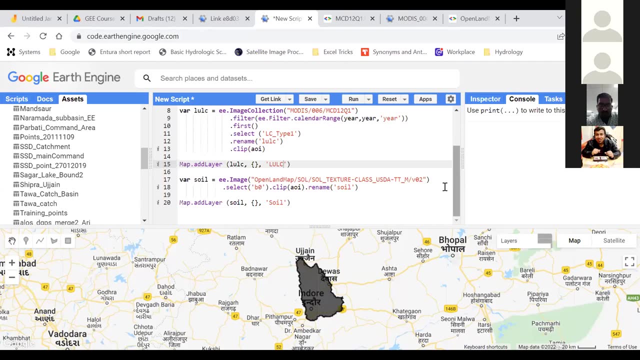 map. add layer map. add layer in which. in which. in which i just write this layer name as soil. i just write this layer name as soil, i just write this layer name as soil and in the lulc i will write now in the layer panel. we have three. 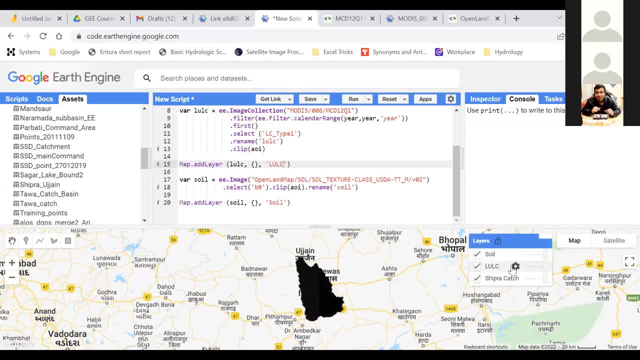 now in the layer panel we have three. now in the layer panel we have three layers. one is shaped like catchment, that layers. one is shaped like catchment, that layers. one is shaped like catchment, that means catchment boundary means catchment boundary means catchment boundary. we have lulc and we have soil, the color. we have lulc and we have soil the color. we have lulc and we have soil. the color. denotion is not very, denotion is not very. denotion is not very good. okay, just if these are just in good. okay, just if these are just in. 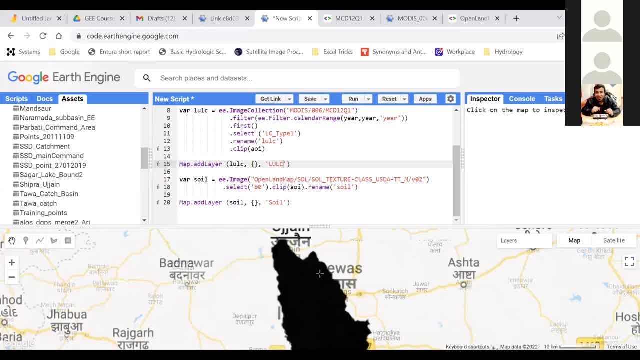 good, okay, just if these are just in black and white color, black and white color, black and white color. but if i click on the inspect tool and if, but if i click on the inspect tool and if, but if i click on the inspect tool and if i click anywhere on any pixel, 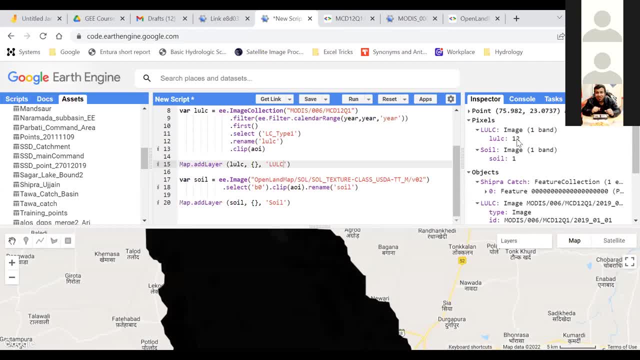 i click anywhere on any pixel. i click anywhere on any pixel, i can found that this particular pixel. i can found that this particular pixel. i can found that this particular pixel has a land use land cover of 12. has a land use land cover of 12. 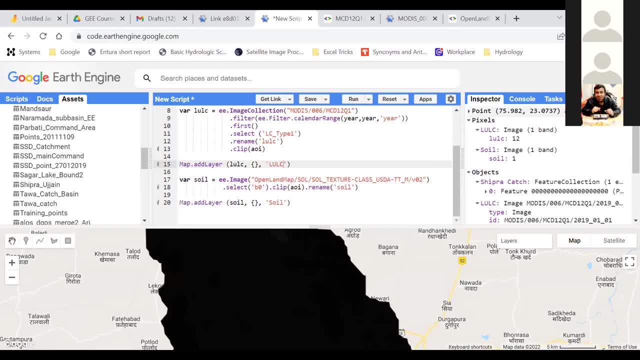 has a land use land cover of 12, has soil texture of one, has soil texture of one, has soil texture of one. so that means this area belongs to the. so that means this area belongs to the. so that means this area belongs to the crop plants. crop plants. 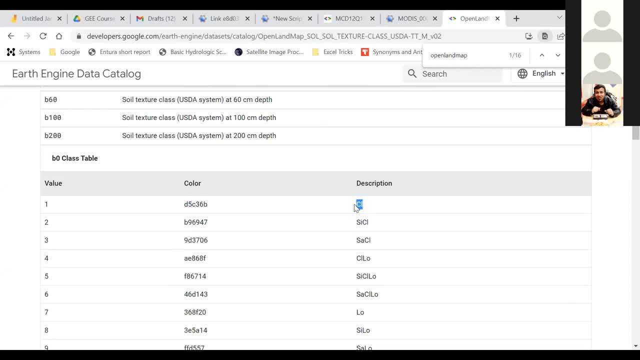 crop plants, and in the soil texture it belongs to, and in the soil texture it belongs to, and in the soil texture it belongs to, the, the, the clay. so now this information has been clay. so now this information has been clay. so now this information has been extracted. now the next. 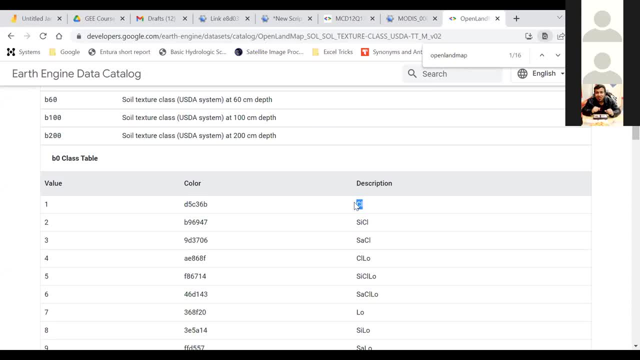 extracted now, the next extracted now. the next thing that we have to do is the convert thing that we have to do is the convert thing that we have to do is the convert this information into the, this information into the, this information into the curve number area, curve number that. 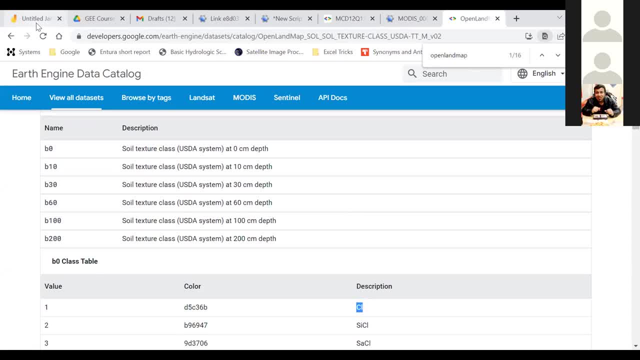 curve number, area, curve number. that curve number, area, curve number, that, if you remember in the slides, if you remember in the slides, if you remember in the slides, um, um, um, the curve number, the curve number, the curve number, uh has only four classes. that means, uh has only four classes. that means 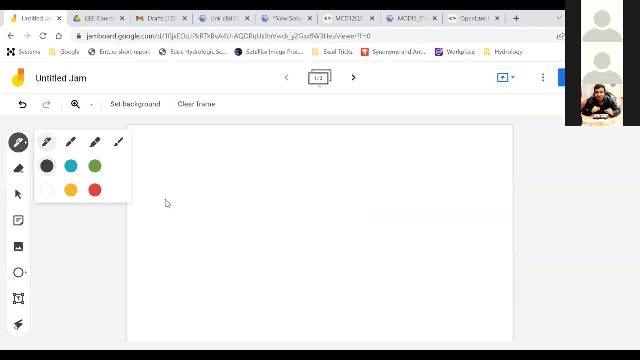 uh, has only four classes. that means class number. it means class a, b c. it means class a, b c. it means class a, b c. now, presently, we have a soil map. if now, presently, we have a soil map, if now, presently, we have a soil map, if suppose this is a raster. 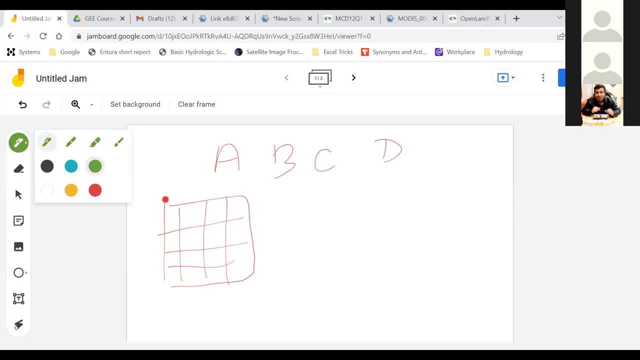 suppose this is a raster. suppose this is a raster, okay and okay and okay. and we have class number. uh, we have a. we have class number. uh, we have a, we have class number. uh, we have a roster of class number with the name 1. roster of class number with the name 1. 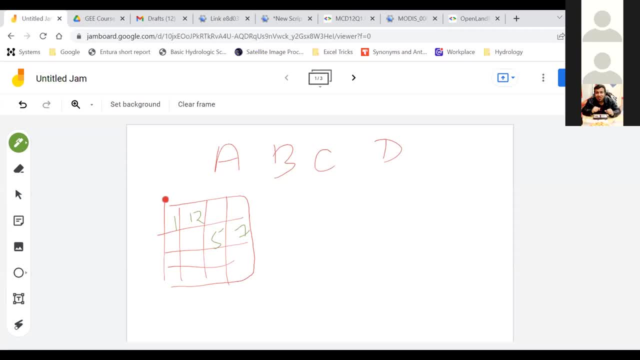 roster of class number with the name 1 to 12. either 1- 12 to 12, either 1- 12 to 12, either 1- 12, 5, 5, 5, 7, 8, etc, 7, 8, etc, 7, 8, etc. now what we have to do, 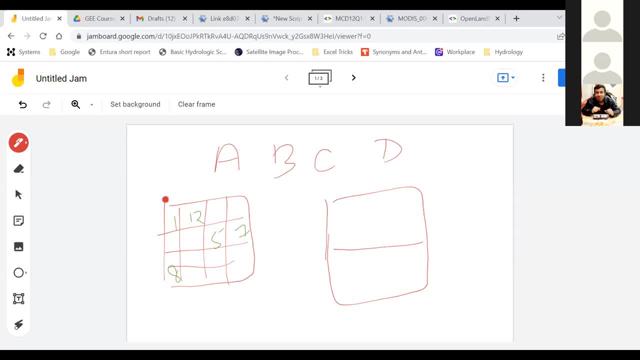 now what we have to do. now what we have to do, we have to convert this raster. we have to convert this raster. we have to convert this raster in this format: abcd, in this format abcd, in this format abcd. but raster cannot be in abcd format. 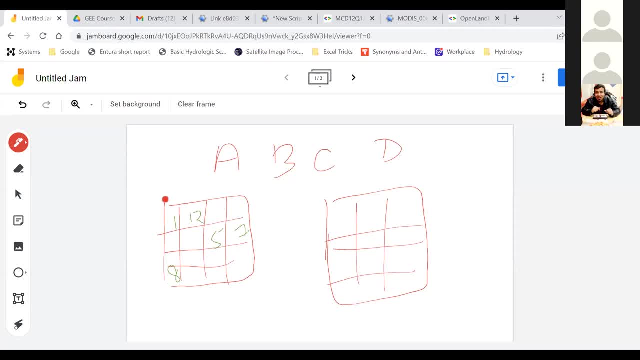 but raster cannot be in abcd format. but raster cannot be in abcd format. that means this cannot be, that means this cannot be. that means this cannot be um string. it has to be an integer or um string. it has to be an integer or um string. it has to be an integer or whole number. so what we are going to do, 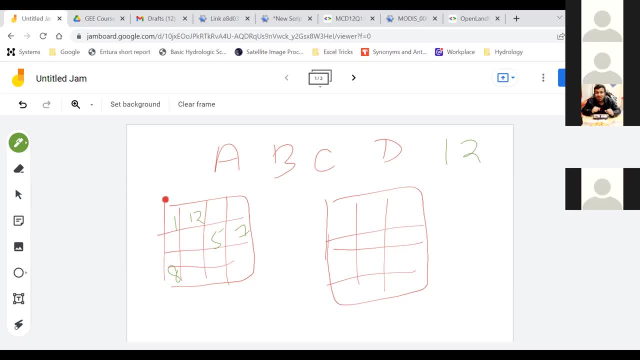 whole number. so what we are going to do: whole number. so what we are going to do: we are converting this abcd into one two. we are converting this abcd into one two. we are converting this abcd into one two, three, fours, three, fours, three fours, and the pixels actually can, uh, getting in. 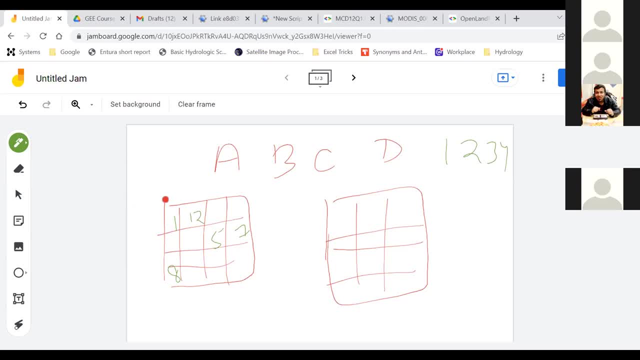 and the pixels actually can uh getting in and the pixels actually can uh getting in the domain of a. that means maybe one. or the domain of a. that means maybe one. or the domain of a. that means maybe one or five. we have to give the number as one. 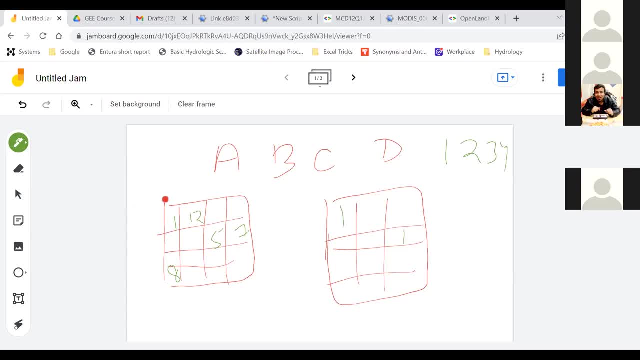 five we have to give the number as one. five we have to give the number as one. one or class number 12 is actually one, or class number 12 is actually one, or class number 12 is actually coming in the soil group b. then we have 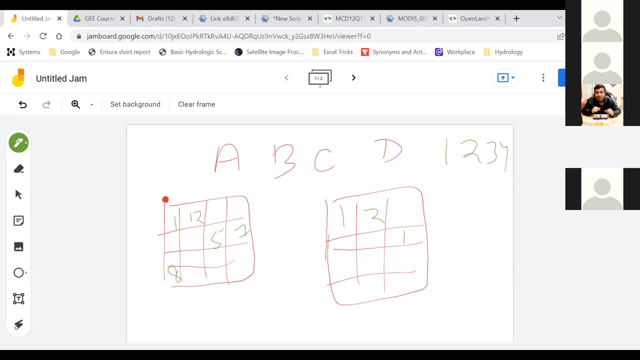 coming in the soil group b, then we have coming in the soil group b, then we have to denote as a, to denote as a. to denote as a two class number eight is actually coming. two class number eight is actually coming. two class number eight is actually coming in the soil group c. so we have to. 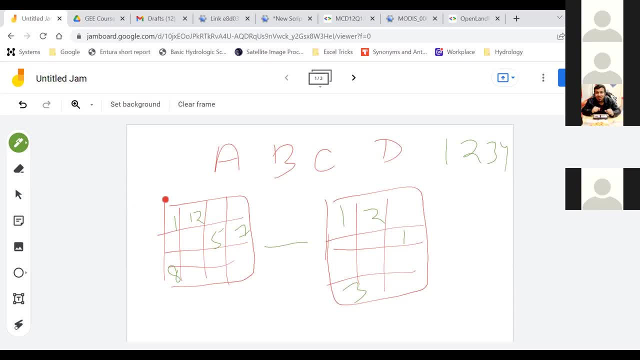 in the soil group c, so we have to in the soil group c, so we have to provide class number a. that provide class number a, that provide class number a. that, what we have to do, we have to convert, what we have to do, we have to convert. 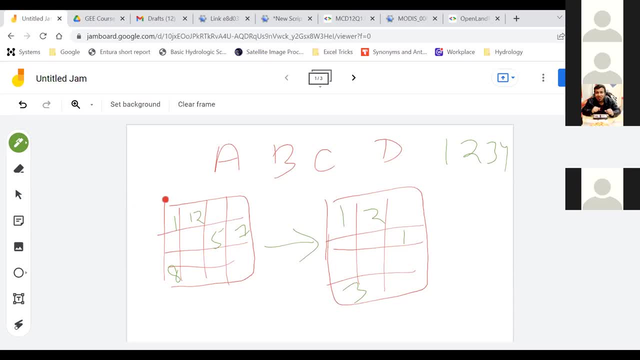 what we have to do. we have to convert this raster into this raster. that means this raster into this raster. that means this raster into this raster. that means we have to reclassify raster into a. we have to reclassify raster into a. we have to reclassify raster into a hydrologic soil condition and in order. 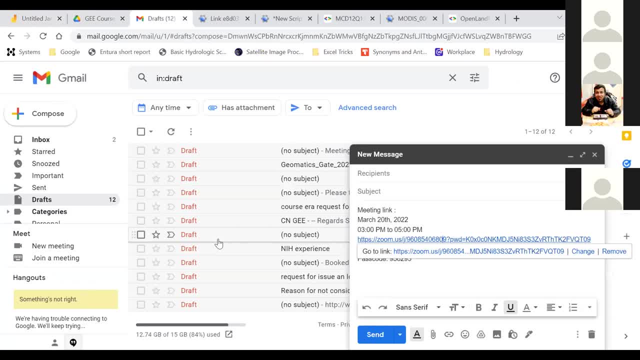 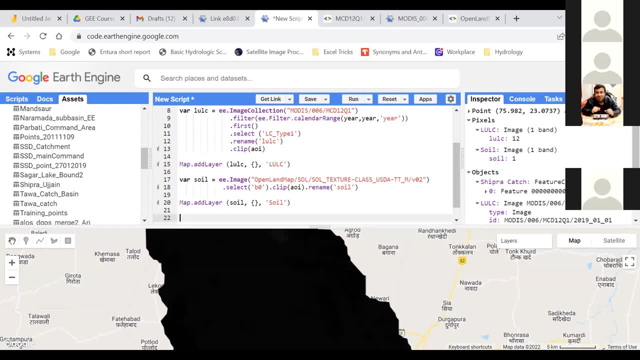 hydrologic soil condition and in order, hydrologic soil condition. and in order to do that, what we will do, there is a function in the first of all. there is a function in the first of all. there is a function in the first of all. we will create a variable. 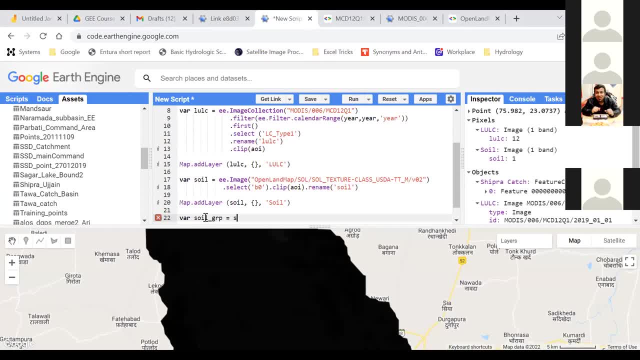 we will create a variable. we will create a variable. soil grp, that means soil group is equal. soil grp, that means soil group is equal. soil grp, that means soil group is equal to soil, because this is the soil and we to soil, because this is the soil and we. 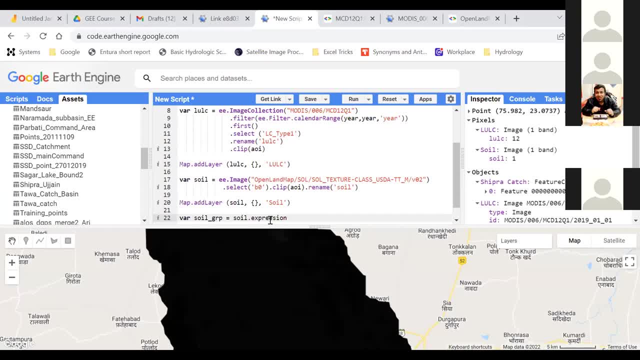 to soil, because this is the soil and we have to apply an expression. so now, as the spelling uh this uh line, so now, as the spelling uh this uh line, so now, as the spelling uh this uh line has been converted from black to green, has been converted from black to green. 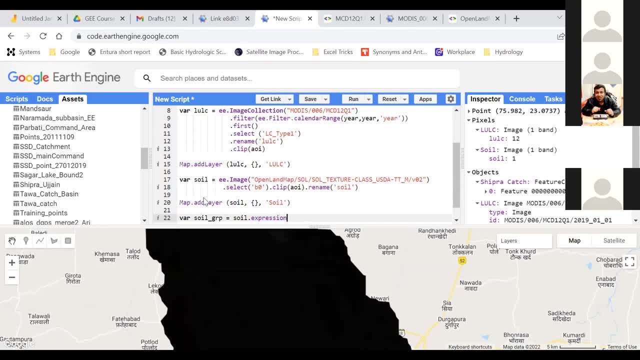 has been converted from black to green. so that means this is an available. so that means this is an available. so that means this is an available function in the earth engine. and if you function in the earth engine, and if you function in the earth engine and if you go to the dots, 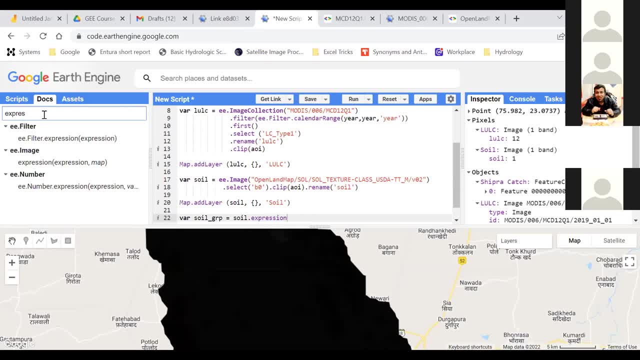 go to the dots, go to the dots and we search for the expression, and we search for the expression and we search for the expression so you can find the expression is in. so you can find the expression is in. so you can find the expression is in the filter, it is in the image and is in. 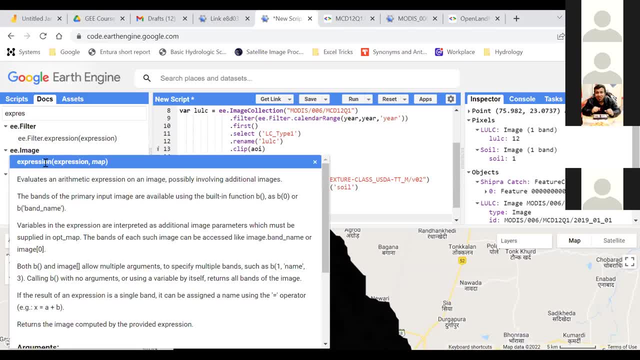 the filter. it is in the image and is in the filter. it is in the image and is in number, number, number. so we have to apply expression over an. so we have to apply expression over an. so we have to apply expression over an image if we click over this. 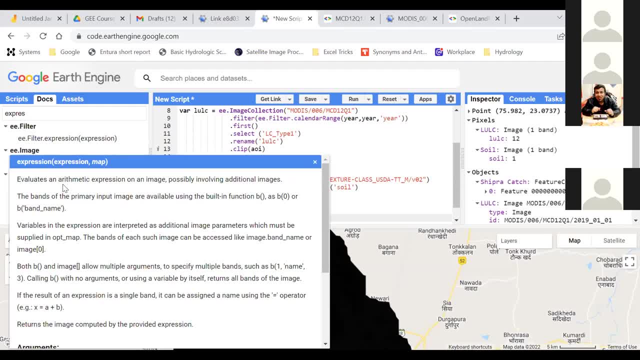 image, if we click over this image, if we click over this, so the details of this particular task, so the details of this particular task, so the details of this particular task is written over here. that it evaluates is written over here. that it evaluates is written over here that it evaluates an arithmetic expression. 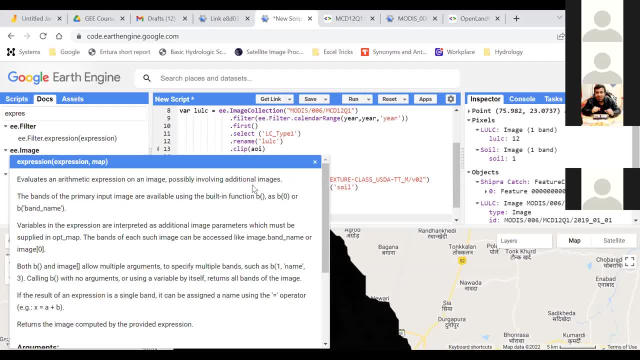 an arithmetic expression. an arithmetic expression on an image possibly involving additional. on an image possibly involving additional. on an image possibly involving additional images. images: images and how to access the different bands. you and how to access the different bands. you and how to access the different bands. you can extract the different band as. 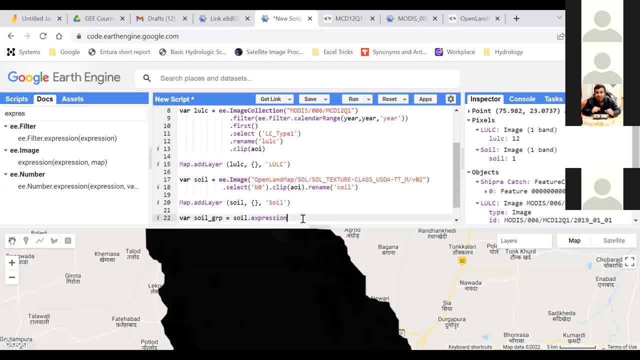 can extract the different band, as can extract the different band as b in the brackets. so let's see how it b in the brackets. so let's see how it b in the brackets. so let's see how it would work, would work, would work. so after writing soilexpression: 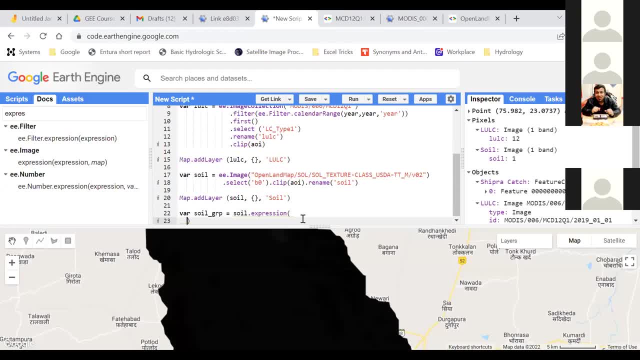 so, after writing soilexpression, so, after writing soilexpression, we have to just open and close the. we have to just open and close the. we have to just open and close the bracket, bracket, bracket. okay, in the inverted commas, we will. okay, in the inverted commas, we will. 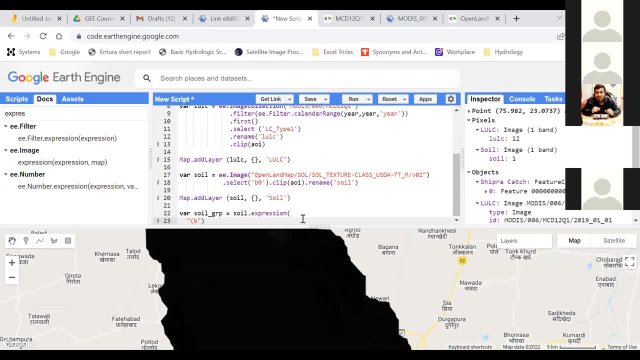 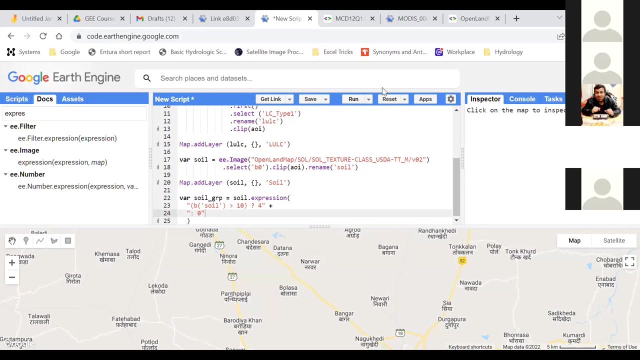 okay, in the inverted commas we will write greater than i'll just tell you what we are actually. i'll just tell you what we are actually. i'll just tell you what we are actually doing. okay, so let's just see that, uh, we are not. so let's just see that, uh, we are not. 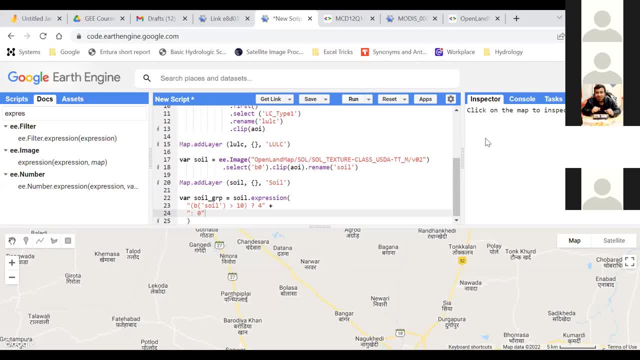 so let's just see that, uh, we are not creating any syntax error. so in the console panel, there is no. so. in the console panel, there is no. so in the console panel, there is no error. that means there is no syntax error. error: that means there is no syntax error. 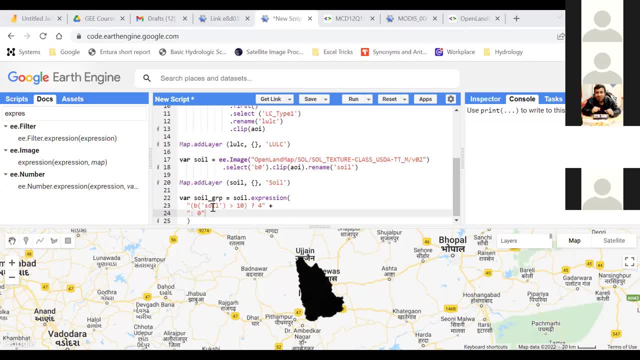 error. that means there is no syntax error. so what we are actually doing, so what we are actually doing, so what we are actually doing, so we are seeing that. so we are seeing that. so we are seeing that in the soil image. okay, we have uh in the soil image. okay, we have uh. 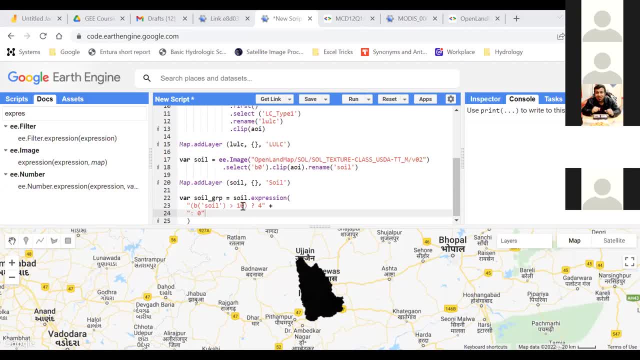 in the soil image. okay, we have, uh, integer values from 1 to 12.. so all integer values from 1 to 12.. so all integer values from 1 to 12.. so, all those integer values which is greater, those integer values which is greater. 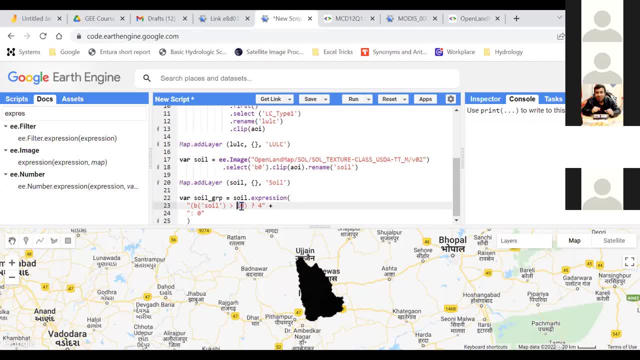 those integer values which is greater than 10. that means 11 and 12 than 10. that means 11 and 12 than 10. that means 11 and 12 will be converted into 4 will be converted into 4 will be converted into 4 and all the remaining pixels that are: 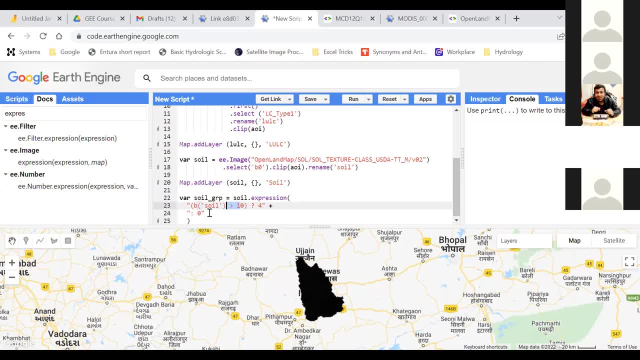 and all the remaining pixels that are, and all the remaining pixels that are having having having value other than this condition will be value other than this condition will be value other than this condition will be converted as converted as converted as zero. so, similarly, if i just uh. 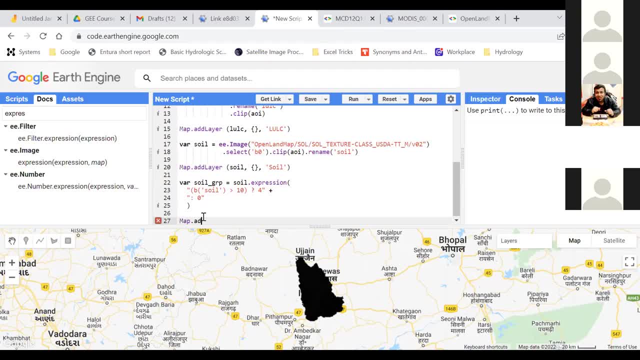 zero. so, similarly, if i just uh zero, so similarly, if i just uh: add this map, add this map. add this map. dot. add layer and type dot. add layer and type dot. add layer and type. if i just if i just if i just run script and let's see what are the 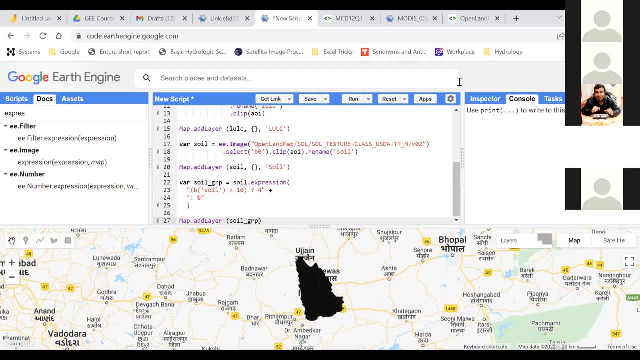 run script and let's see what are the run script and let's see what are the different things, different things, different things. we are actually getting if i click. we are actually getting if i click, we are actually getting, if i click anywhere on this particular pixels- any. 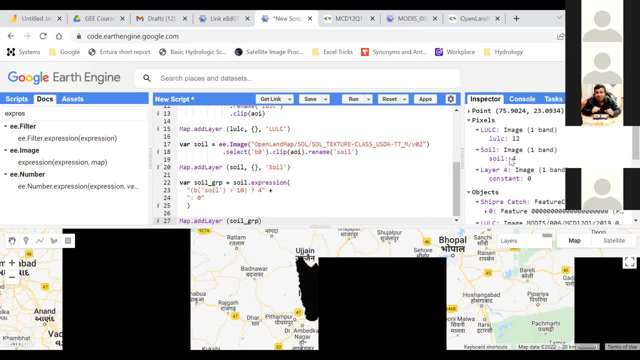 anywhere on this particular pixels, any. anywhere on this particular pixels, any pixel. so now, initially, the soil class is four. so now, initially the soil class is four. so now, initially the soil class is four, but in the final map the soil group this. but in the final map the soil group this. 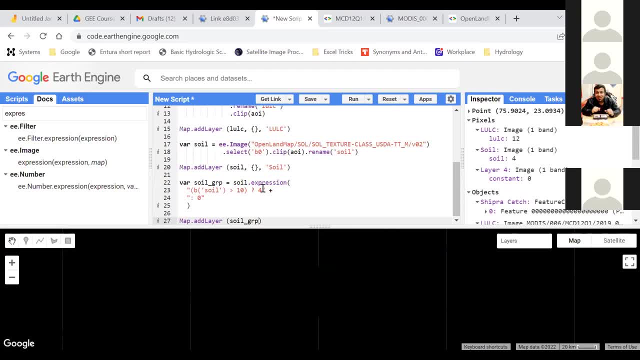 but in the final map, the soil group. this is soil class, is soil class, is soil class zero? why? because all the integers that zero. why? because all the integers that zero? why? because all the integers that are are are value. uh, other than this condition that value, uh, other than this condition that. 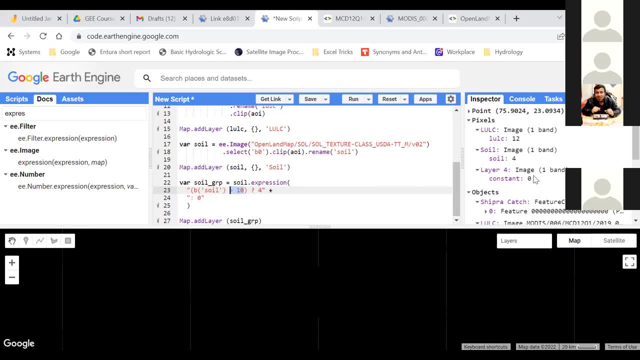 value. uh, other than this condition, that means less than 10 if we are denoting as means less than 10, if we are denoting as means less than 10, if we are denoting as zero, zero, zero. so what we have to do, if i just uh go to, 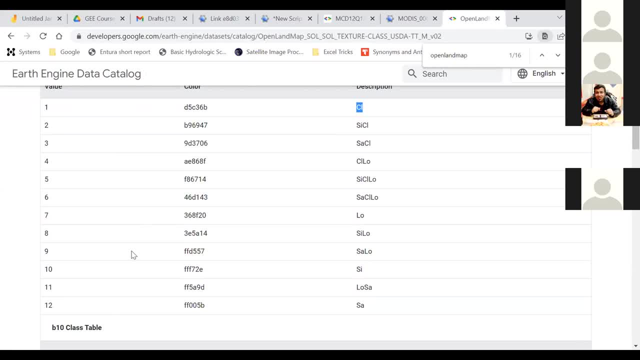 so what we have to do if i just uh go to, so what we have to do if i just uh go to the, the, the soil classification, so we can see there soil classification, so we can see there soil classification, so we can see there are 12 to 12 classes, so we have to on. 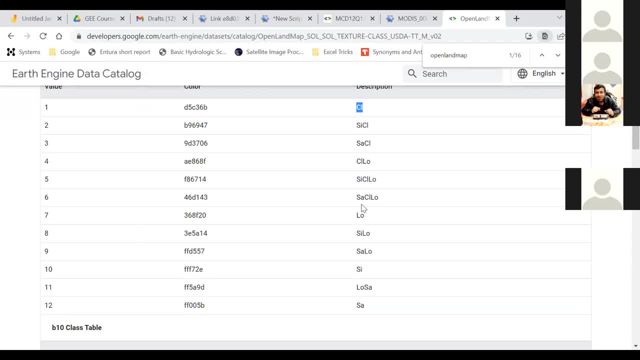 are 12 to 12 classes, so we have to. on are 12 to 12 classes, so we have to. on our hydraulic knowledge, knowledge using our hydraulic knowledge, knowledge using our hydraulic knowledge, knowledge using our hydraulic knowledge. we have to, our hydraulic knowledge, we have to. 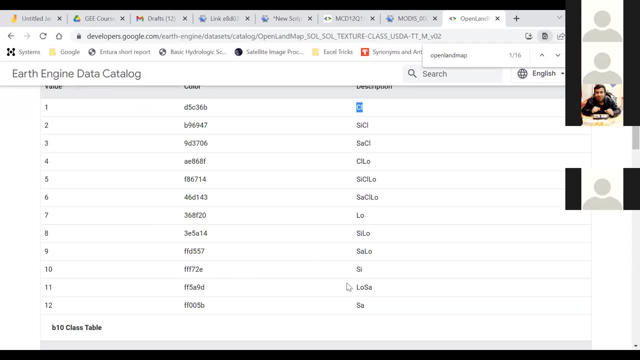 our hydraulic knowledge, we have to classify, classify, classify in different groups. for example, class in different groups. for example, class in different groups. for example, class number 11 and 12 will be in the soil. number 11 and 12 will be in the soil. number 11 and 12 will be in the soil group. 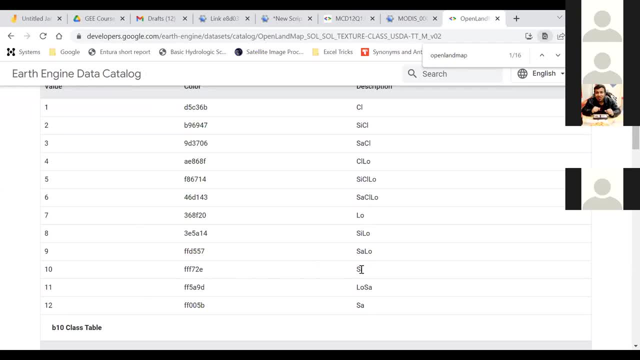 group group: class number: class number: class number six, seven, eight, nine and ten will be six, seven, eight, nine and ten will be six, seven, eight, nine and ten will be in soil group c and class number one in soil group c and class number one in soil group c and class number one will be in soil group a. 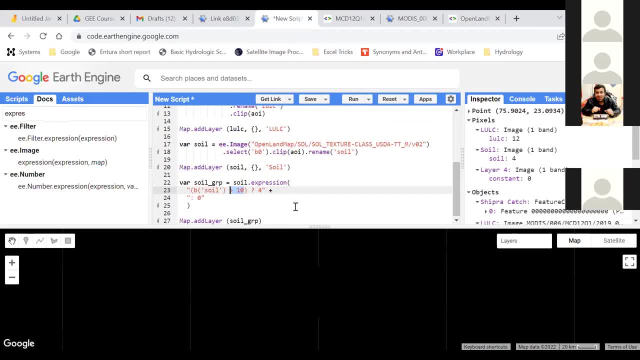 will be in soil group a will be in soil group a, so so. so, on that basis, on that basis, on that basis, we have to convert this equation, we have to convert this equation. we have to convert this equation according to our own. so i'm not, so, i'm not. 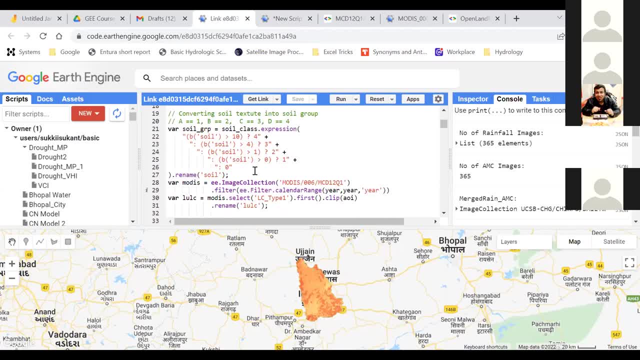 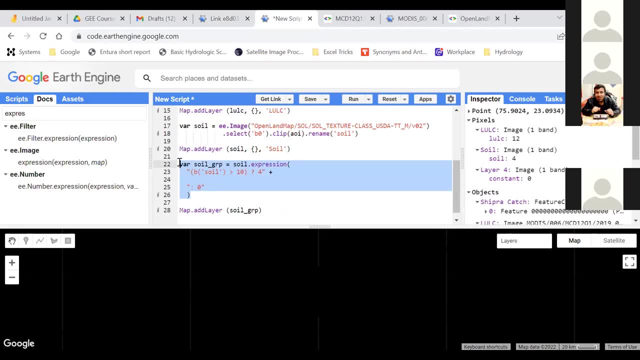 so i'm not, i'm writing each and everything. i. i'm writing each and everything. i. i'm writing each and everything. i just using, just using, just using the already written. so now what we are actually doing we are. so now what we are actually doing, we are. 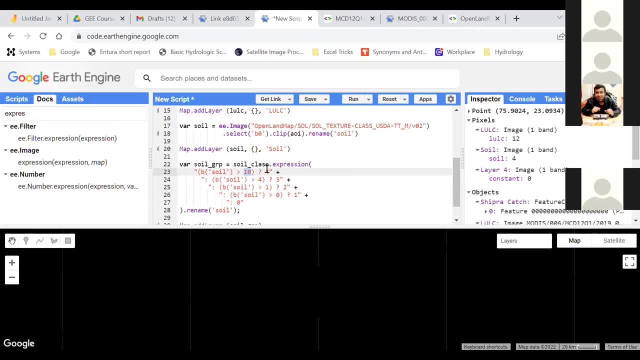 so now what we are actually doing. we are converting all the integer having value. converting all the integer having value. converting all the integer having value greater than 10 is in four. greater than 10 is in four. greater than 10 is in four. all the integer pixels having value. 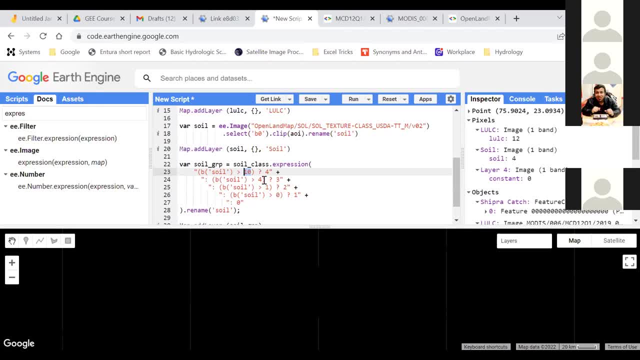 all the integer pixels having value. all the integer pixels having value between 10 to 4 is converted into 3. between 10 to 4 is converted into 3. between 10 to 4 is converted into 3. all the integer that has been value from. 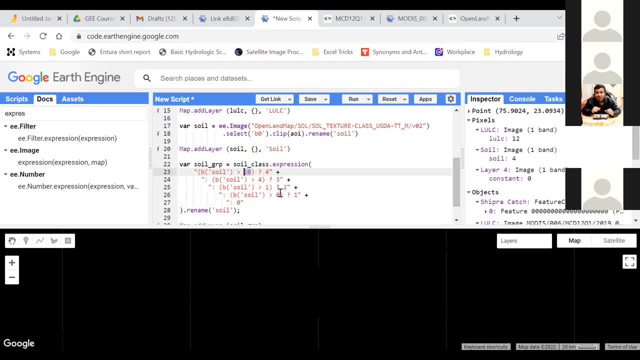 all the integer that has been value from. all the integer that has been value from 1 to 4 will be converted to 1 to 4. will be converted to 1 to 4. will be converted to all the integer that is having the value. 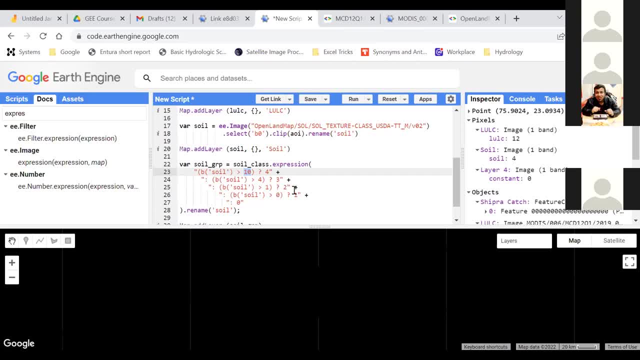 all the integer that is having the value, all the integer that is having the value of less than greater than zero, and one of less than greater than zero and one of less than greater than zero, and one that means one will be converted into one, that means one will be converted into one. 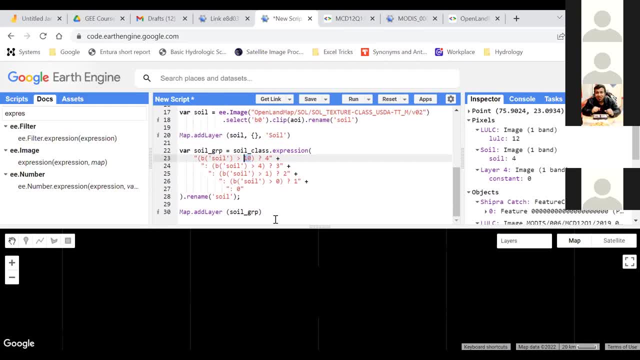 that means one will be converted into one and all the remaining pixel will be, and all the remaining pixel will be, and all the remaining pixel will be converted as you converted as you converted as you. and if we just, and if we just and if we just open uh, 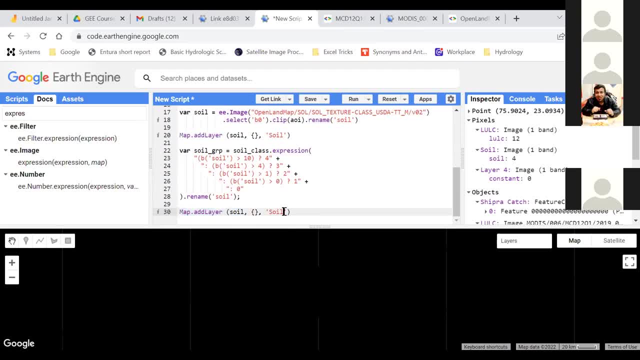 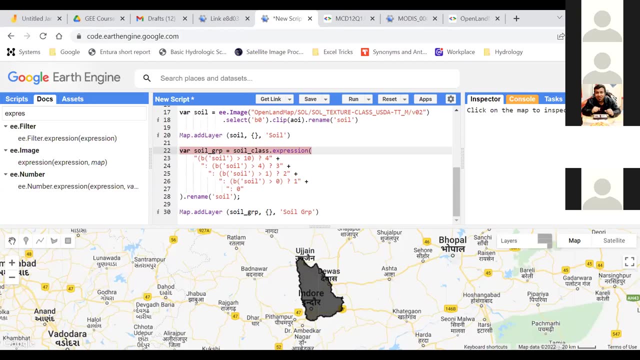 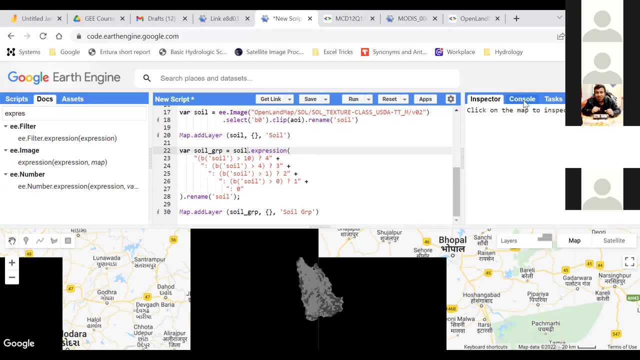 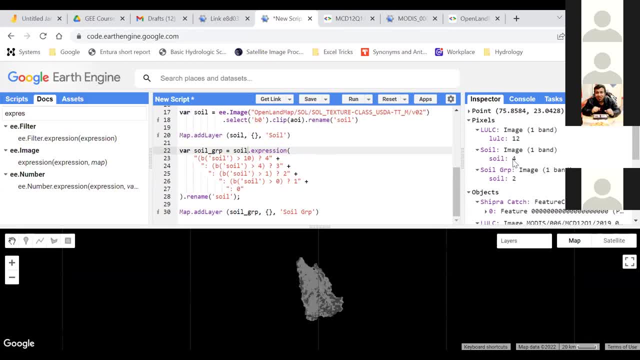 now, if i click on inspector tab and click on any pixel, on any pixel, on any pixel, i can found that the pixel value initially. i can found that the pixel value initially. i can found that the pixel value initially that has with the value of 4, now converted. 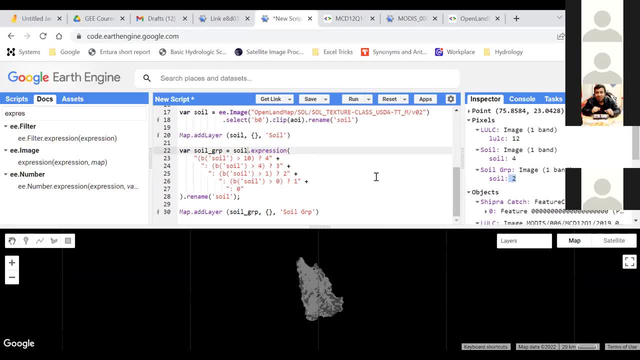 that has with the value of 4 now converted. that has with the value of 4 now converted into, into, into, into. so this is how we can convert our soil. so this is how we can convert our soil. so this is how we can convert our soil map from. 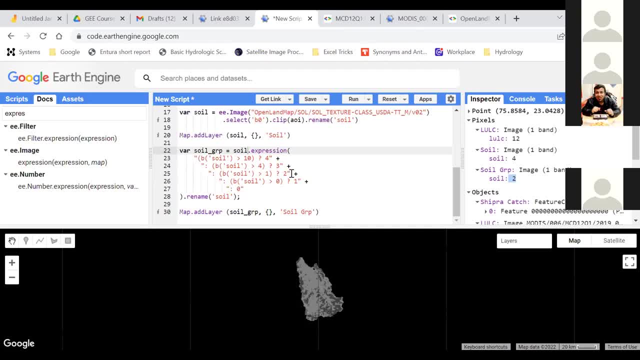 map from map, from their classification to our own, their classification to our own, their classification to our own classification. now, the next thing that we classification, now the next thing that we classification, now the next thing that we have to do, have to do, have to do, is up creating the curve number map. 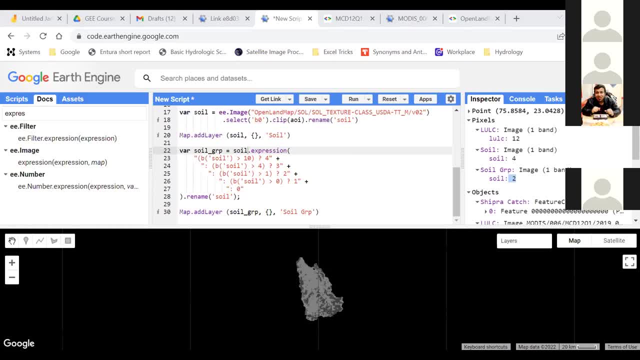 is up creating the curve number map is up creating the curve number map. so you know that current number map is. so you know that current number map is. so you know that current number map is. depend on two things, depend on two things. depend on two things: one is lulc and another is. 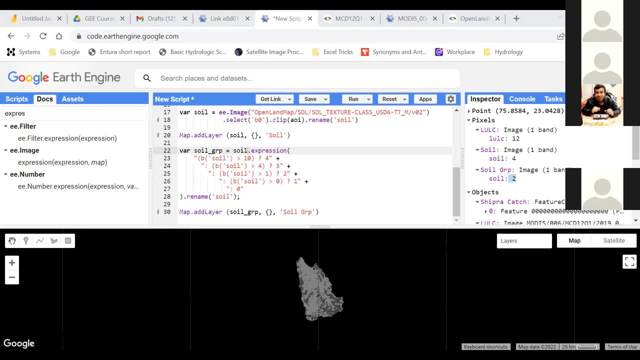 one is lulc and another is. one is lulc and another is uh uh uh. soil texture. so what we have to do, we soil texture. so what we have to do, we soil texture. so what we have to do, we have to create the combination of soil. 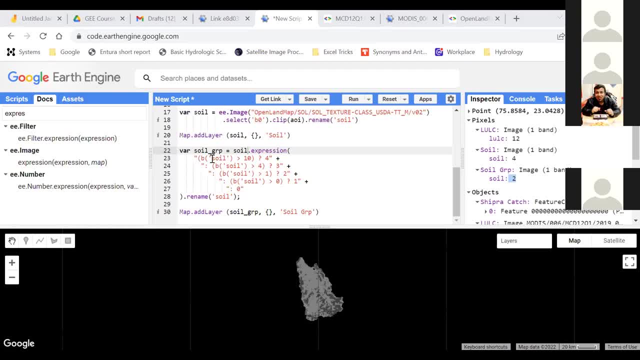 have to create the combination of soil, have to create the combination of soil and lulc, and we have to give this and lulc, and we have to give this and lulc, and we have to give this condition, condition, condition. yes, if the soil is 4 and the lulc is 12. yes, if the soil is 4 and the lulc is 12. yes, if the soil is 4 and the lulc is 12, then we have to assign a respective, then we have to assign a respective, then we have to assign a respective number, number. 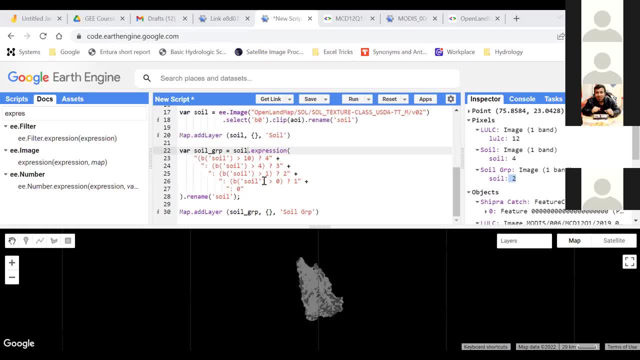 number. and if the soil is this and lulc this, and if the soil is this and lulc this, and if the soil is this and lulc this, then we have to assign this particular, then we have to assign this particular, then we have to assign this particular curve number. so for that basis, i'll just 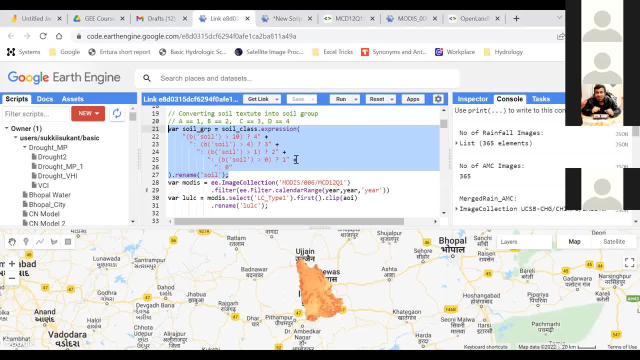 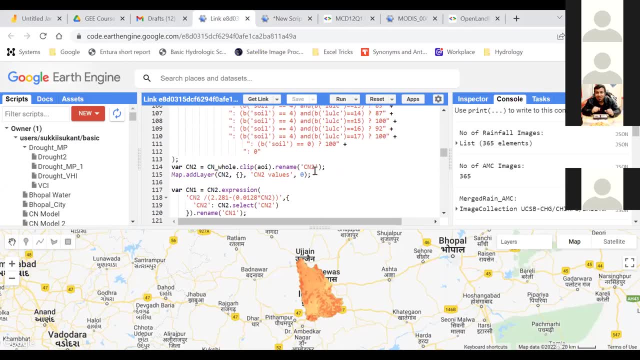 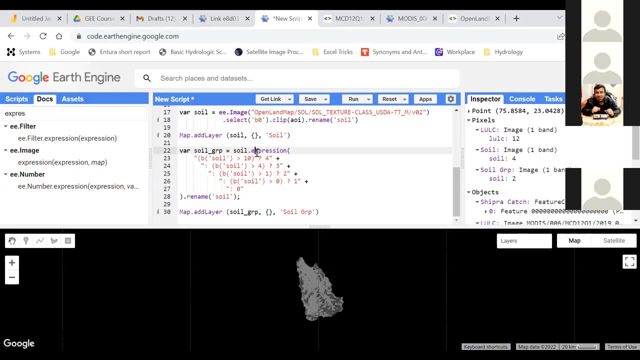 curve number. so for that basis i'll just curve number. so for that basis i'll just. because it is a very, because it is a very, because it is a very long code, i'll just copy the initial part, paste this over here and click run. paste this over here and click run. 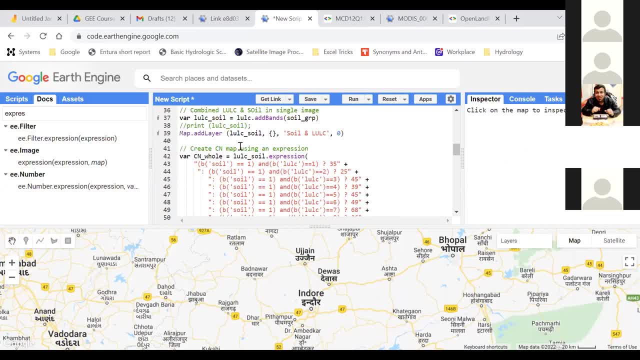 paste this over here and click run. and this is the script for. and this is the script for, and this is the script for converting the. creating the count number. converting the. creating the count number. converting the. creating the count number. map what we have done. map what we have done. 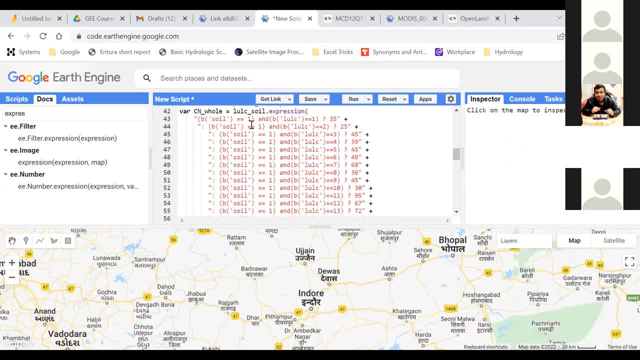 map what we have done. we have combined the soil and lulc into a. we have combined the soil and lulc into a. we have combined the soil and lulc into a single image and we have given the single image. and we have given the single image and we have given the condition that 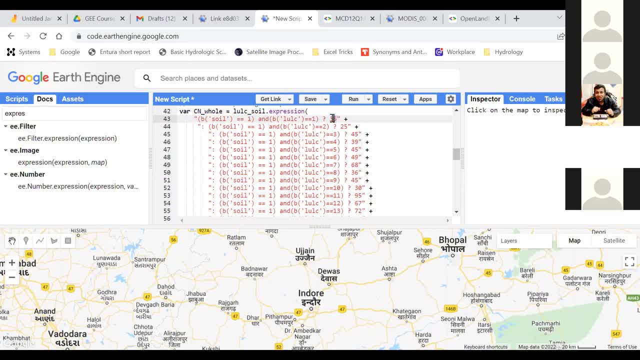 condition. that condition that if the soil is one and the lulc is one, if the soil is one and the lulc is one, if the soil is one and the lulc is one, gives the curve number as 35. gives the curve number as 35. 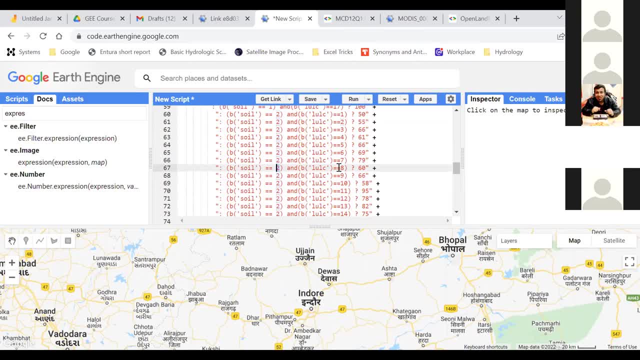 gives the curve number as 35 if the soil is two, and the curve number if the soil is two and the curve number if the soil is two and the curve number lulc is eight. give the come number as lulc is eight. give the come number as: 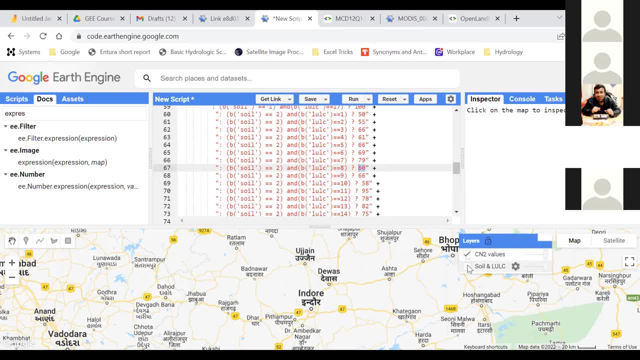 lulc is eight. give the come number as 60 and in the layer panel we can get the 60 and in the layer panel we can get the 60 and in the layer panel we can get the cn2 values, cn2 values, cn2 values and we have the lulc soil and lulc value. 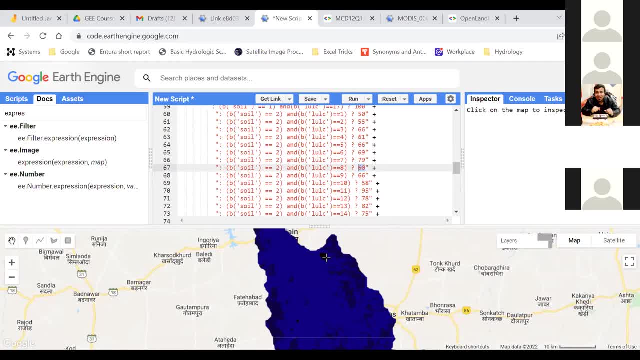 and we have the lulc soil and lulc value and we have the lulc soil and lulc value and we can inspect any of the and we can inspect any of the and we can inspect any of the particular pixel like this pixel. particular pixel like this pixel. 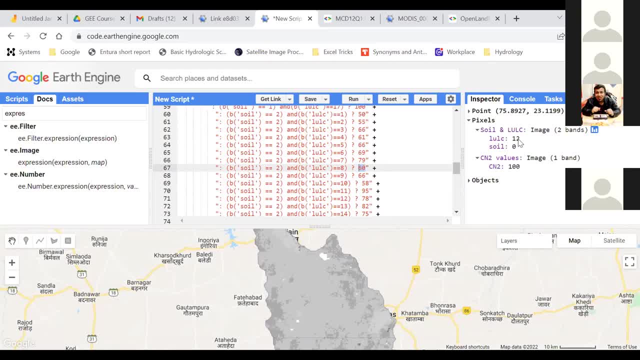 particular pixel like this pixel, so we can see this. this particular pixel, so we can see this. this particular pixel, so we can see this. this particular pixel has the lulc of 12 and soil is zero. that has the lulc of 12 and soil is zero. that. 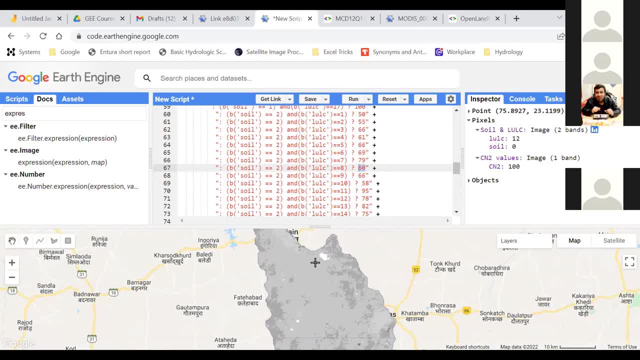 has the lulc of 12 and soil is zero. that means soil may be a water body. means soil may be a water body. means soil may be a water body. so it has a curve number of 12.. if i so, it has a curve number of 12.. if i 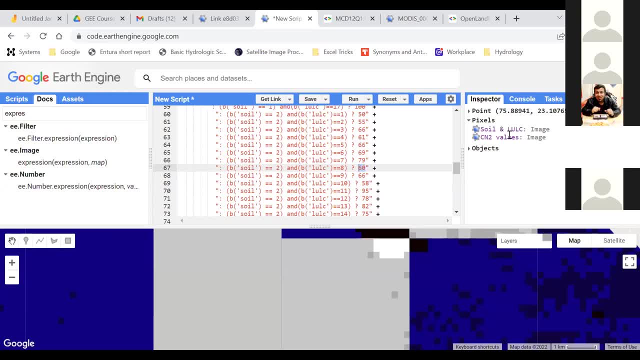 so it has a curve number of 12.. if i click on any one of the pixel over here, click on any one of the pixel over here. click on any one of the pixel over here. there the soil is, lulc is 12 and soil is. 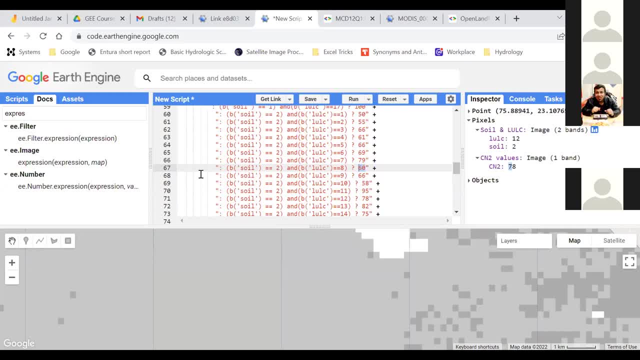 there, the soil is lulc is 12 and soil is there. the soil is lulc is 12 and soil is two, two, two. that's why we are getting curve number. that's why we are getting curve number. that's why we are getting curve number as 70.. 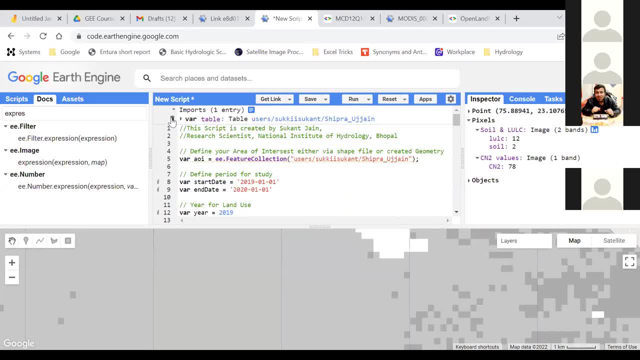 as 70.. as 70.. so what i'm going to do, i'm just uh, so what i'm going to do, i'm just uh, so what i'm going to do, i'm just uh, tell you how to share this code, so this. tell you how to share this code, so this. 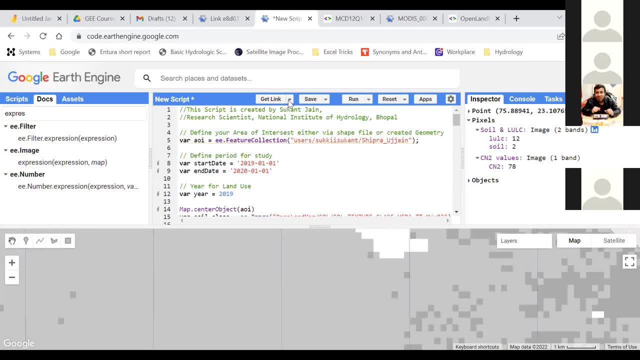 tell you how to share this code. so this is just a is just a is just a small segment. i'm just clicking get link, small segment. i'm just clicking get link, small segment. i'm just clicking get link. okay, copy this link and i'm pasting this. 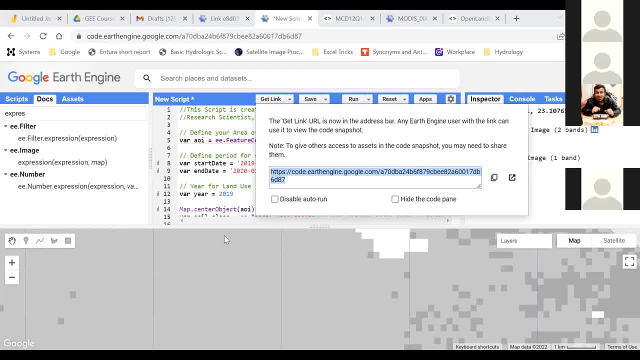 okay, copy this link and i'm pasting this. okay, copy this link and i'm pasting this in the chat box, in the chat box, in the chat box, and you can, and you can and you can explore, explore, explore this segment of this particular script, this segment of this particular script. 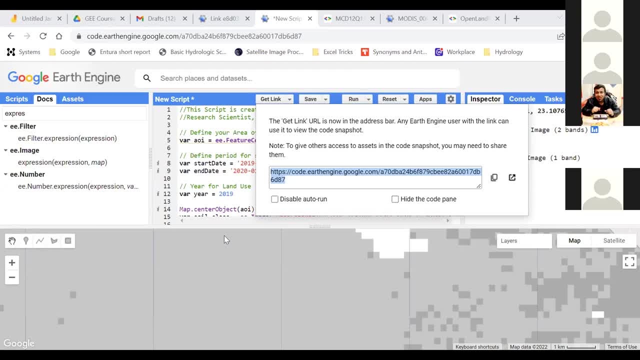 this segment of this particular script. you, just you, just you just open your chat box. click on this link. open your chat box. click on this link. open your chat box. click on this link. and if you have google earth indian and if you have google earth indian and if you have google earth indian account, uh, if you have registered google. 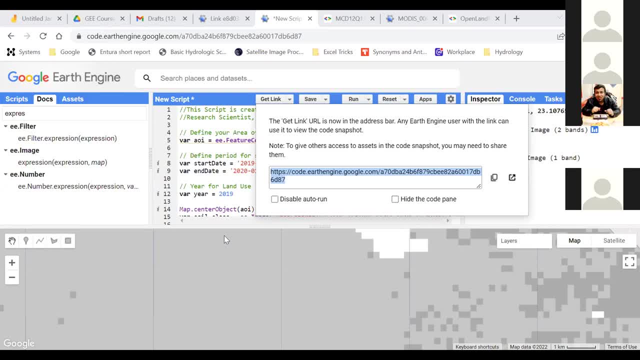 account, uh, if you have registered google account, uh, if you have registered google, then you can account, you will open. if i, then you can account, you will open. if i, then you can account, you will open. if i just just just copy this script, okay, copy this script, okay. 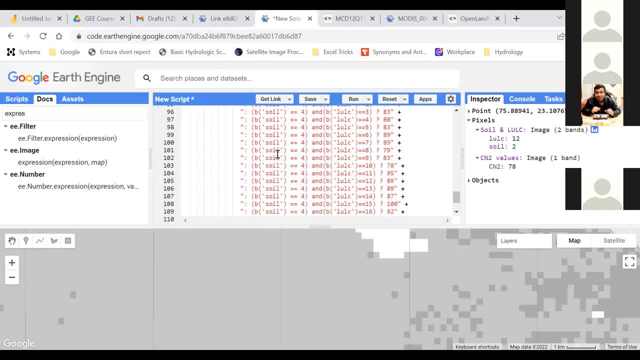 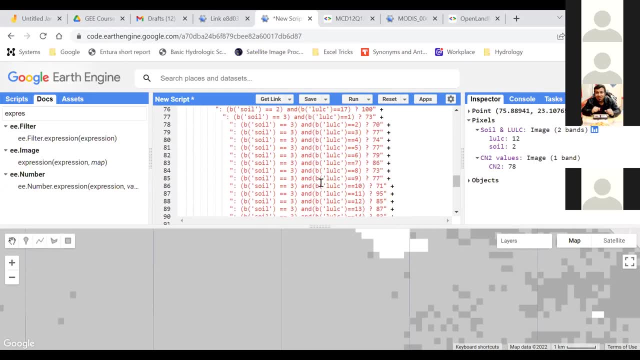 copy this script. okay, so you will open this particular. so you will open this particular, so you will open this particular script into your web browser. so just check the script and see uh, you. so just check the script and see uh, you. so just check the script and see uh, you don't need to go line by line, you just 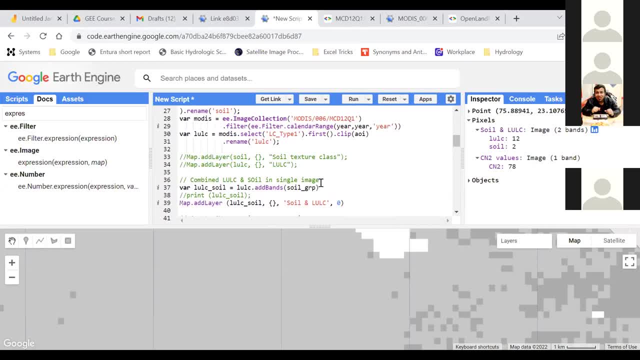 don't need to go line by line. you just don't need to go line by line. you just see how the things will work, see how the things will work, see how the things will work. okay, so, if i need to just change the, okay. so, if i need to just change the. 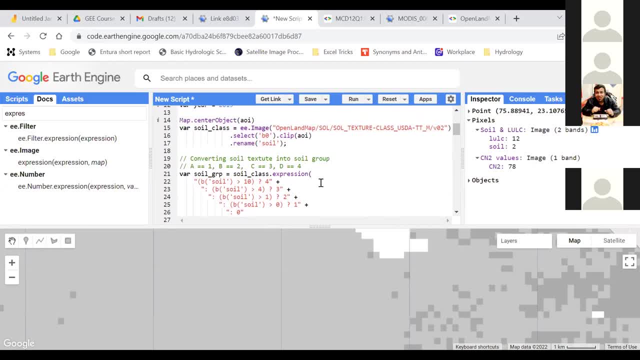 okay, so if i need to just change the lulc year from, either, for example, lulc year from, either, for example, lulc year from either, for example: uh. presently i'm using land use land cover. uh. presently i'm using land use land cover. uh. presently i'm using land use land cover year of 2019. i'm getting this data. 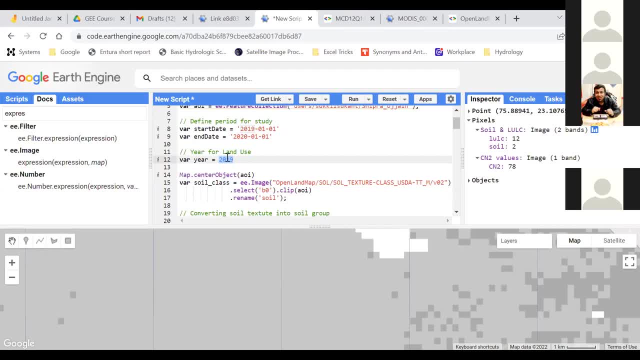 year of 2019: i'm getting this data. year of 2019: i'm getting this data. so if i want to change the year to 2019, so if i want to change the year to 2019, so if i want to change the year to 2019 to 2005, i don't need to write each and. 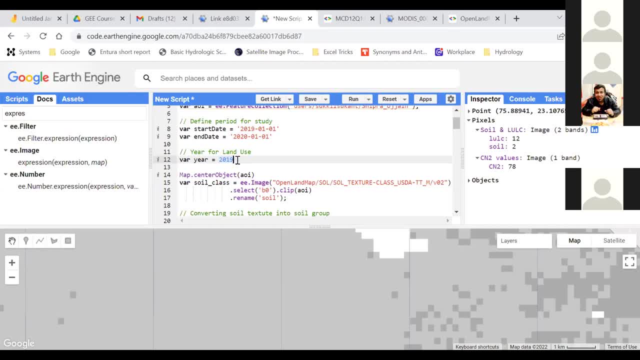 to 2005- i don't need to write each- and to 2005: i don't need to write each and every procedure. i don't need to download every procedure. i don't need to download every procedure, i don't need to download the dataset, i just need to change this. 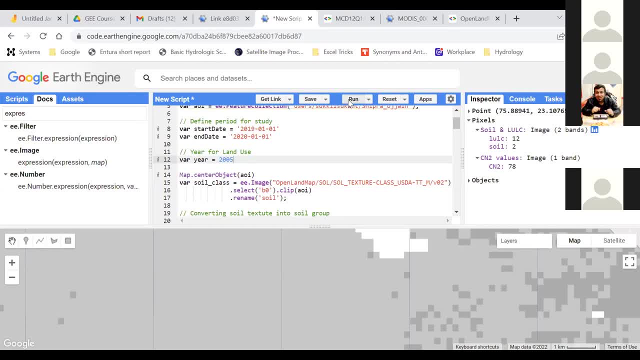 the dataset. i just need to change this, the dataset. i just need to change this value from 2019 to 2005, value from 2019 to 2005, value from 2019 to 2005, and run this script. and run this script. 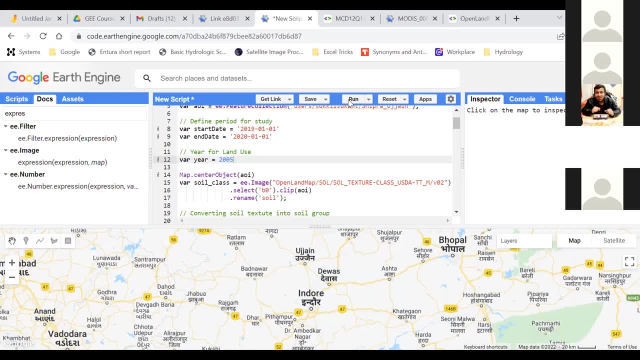 and run this script: now we will get the lulc of 2005. now we will get the lulc of 2005. now we will get the lulc of 2005. so this is how the, so this is how the. so this is how the cloud computational platform is very much. 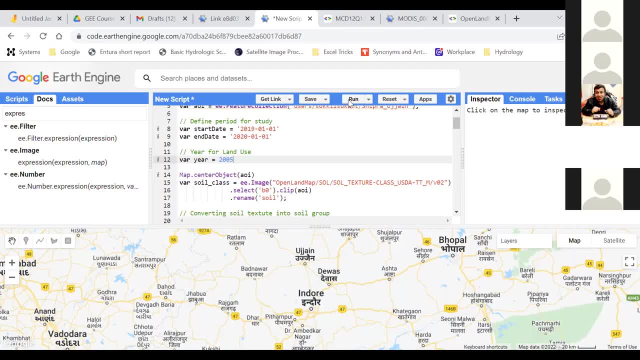 cloud computational platform is very much. cloud computational platform is very much useful that you don't need to useful, that you don't need to useful, that you don't need to follow each and every step again and follow each and every step again, and follow each and every step again and again. you can just change the variables. 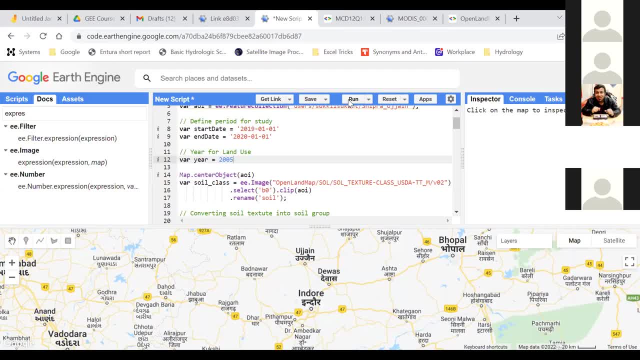 again, you can just change the variables. again, you can just change the variables: uh certain numbers, you can get your data. uh certain numbers. you can get your data. uh certain numbers. you can get your data set set set. so meanwhile, if there are any question, i. so meanwhile, if there are any question, i. 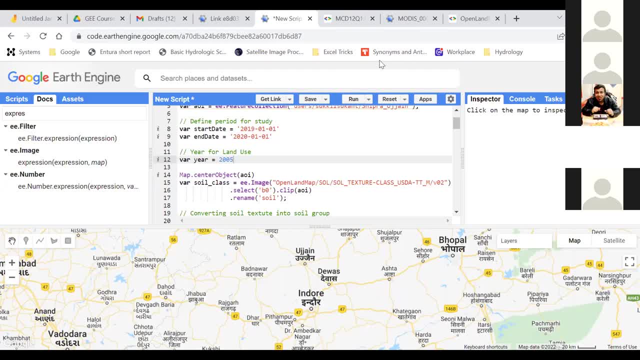 so meanwhile, if there are any question, i see can check box, so i think i think there are a few. so i think i think there are a few. so i think i think there are a few questions, questions, questions. so should we take them now, or do you want? 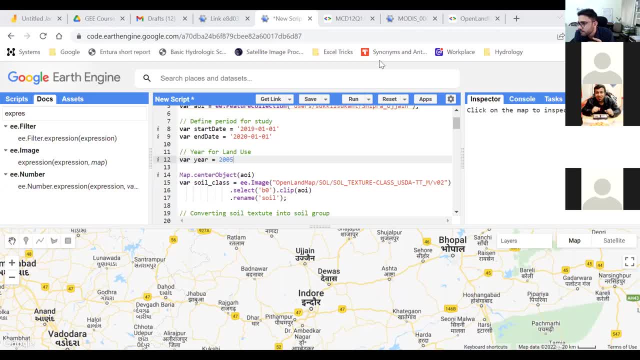 so should we take them now, or do you want? so, should we take them now, or do you want? yes, yes, we can take them now. if they are yes, yes, we can take them now. if they are yes, yes, we can take them now if they are relevant to up to this part. 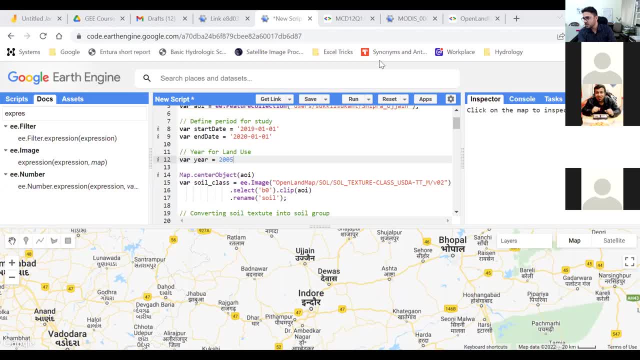 relevant to up to this part. relevant to up to this part, i will try to answer. or, if it is relevant, i will try to answer. or if it is relevant, i will try to answer. or if it is relevant, there are some general questions, but i. there are some general questions, but i. 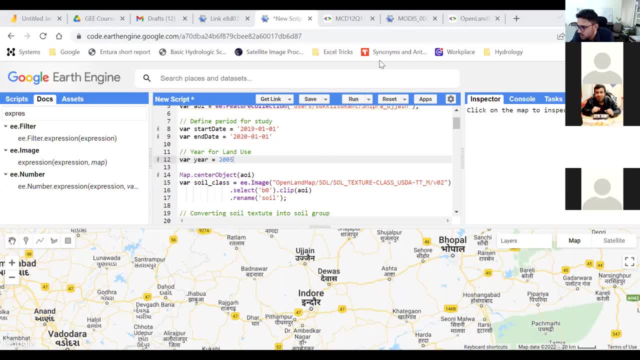 there are some general questions, but i will pick the ones which are relevant to. will pick the ones which are relevant to, will pick the ones which are relevant to what we discuss, what we discuss, what we discuss? uh, right now, i think there's one. uh, right now, i think there's one. 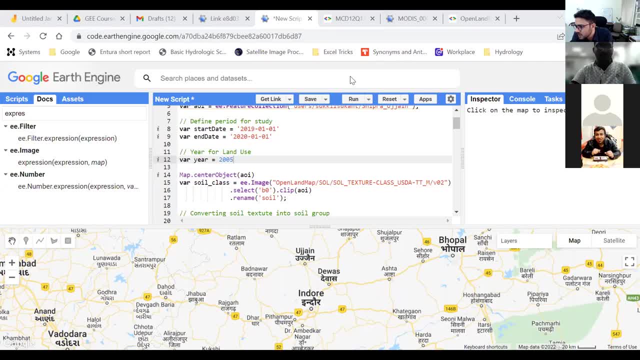 uh, right now i think there's one question which question which question which: how one can crop their own study area. how one can crop their own study area. how one can crop their own study area, any district or any state in google earth, any district or any state in google earth. 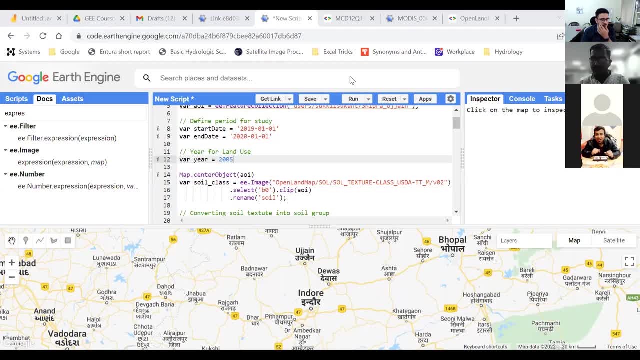 any district or any state in google earth engine engine engine: yes, uh so, uh, yes, uh, so, uh, yes, uh so uh. google earth engine doesn't provide any google earth engine. doesn't provide any. google earth engine doesn't provide any vector data set, or is there very few. 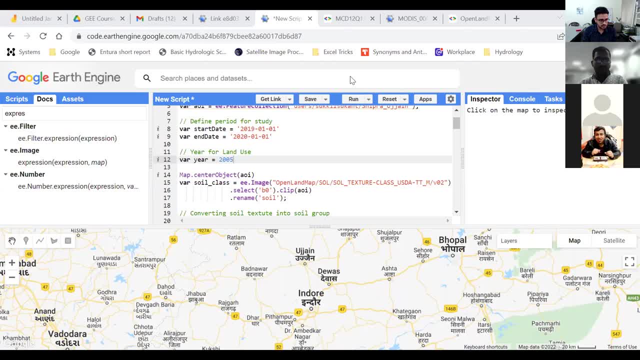 vector data set. or is there very few vector data set, or is there very few data but few of the user worldwide has data? but few of the user worldwide has data. but few of the user worldwide has ingested their own data set. so there is. ingested their own data set, so there is. 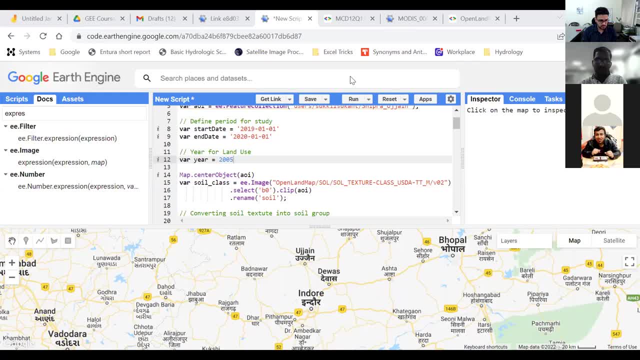 ingested their own data set. so there is a data set known as gaul, a data set known as gaul, a data set known as gaul- uh. in the end, i'm going to share the uh. in the end, i'm going to share the uh. in the end, i'm going to share the link: how to extract those data set. but 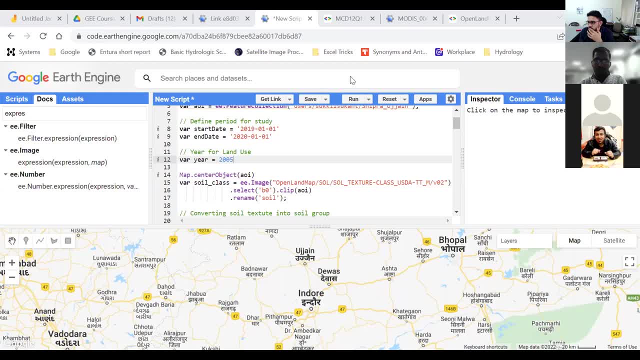 link how to extract those data set, but link how to extract those data set, but it is an international boundary. it is an international boundary. it is an international boundary which is not accepted. uh to indians. which is not accepted, uh to indians. which is not accepted, uh to indians. that means it is a. 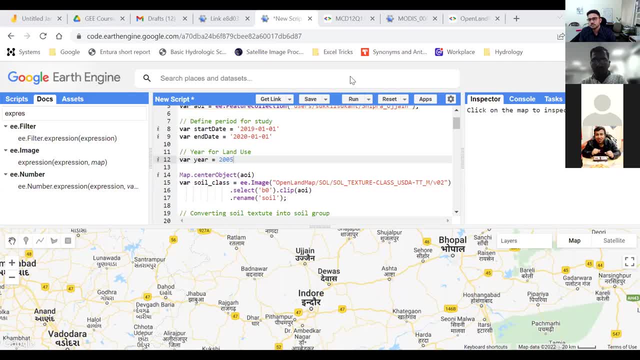 that means it is a. that means it is a uh incorrectly showing some international uh incorrectly showing some international uh incorrectly showing some international boundaries, boundaries, boundaries. so it is my advice: don't use that, what so? it is my advice, don't use that, what so? it is my advice, don't use that. what you can do. 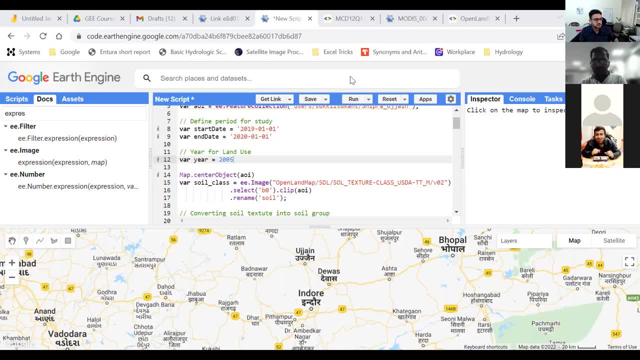 you can do. you can do if you are, if you are having your own, if you are, if you are having your own, if you are, if you are having your own shape file, either for your catchment area shape file, either for your catchment area shape file, either for your catchment area or for. 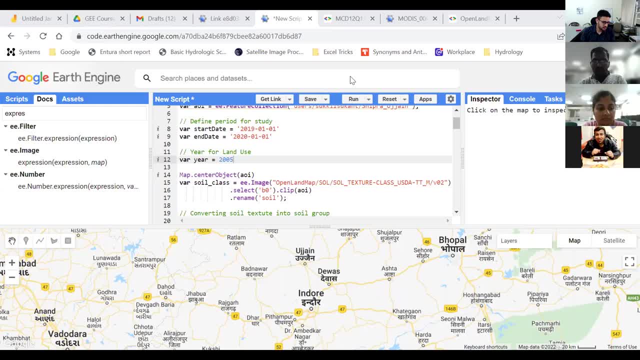 or for, or for your district or for your state. you can your district or for your state, you can your district or for your state, you can incorporate in those things, incorporate in those things, incorporate in those things. but it is all about the administrative, but it is all about the administrative. 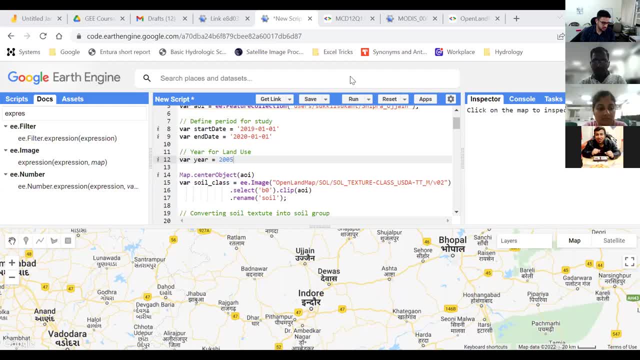 but it is all about the administrative boundaries. but if you are using any boundaries, but if you are using any boundaries, but if you are using any hydrological boundary, hydrological boundary, hydrological boundary, either the cashmint basin, then you have, either the cashmint basin, then you have. 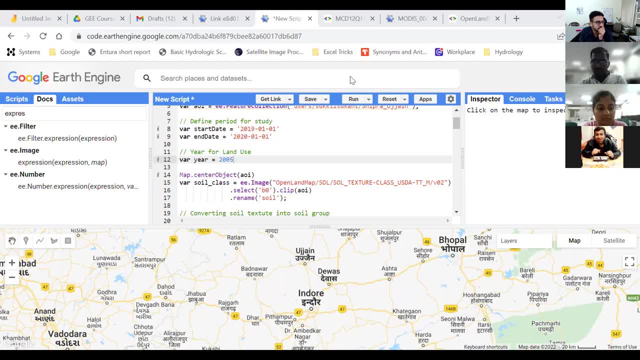 either the cashmint basin, then you have to delineate on your own. to delineate on your own, to delineate on your own either in the qgis or rgis or any other. either in the qgis or rgis or any other, either in the qgis or rgis or any other platform. 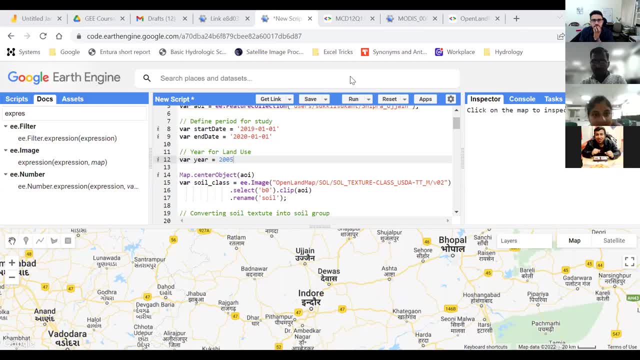 platform, platform and you can import those boundaries and you can import those boundaries and you can import those boundaries into the rg. perfect, uh, i hope the question is answered. there is one more question by pavan uh. there is one more question by pavan uh. there is one more question by pavan uh. who asked that? 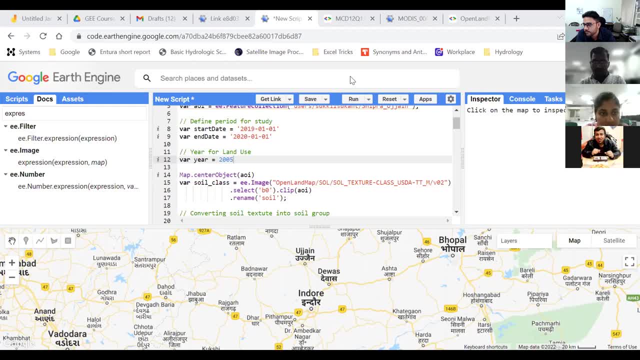 who asked that? who asked that? how can we see yearly change in lulc? how can we see yearly change in lulc? how can we see yearly change in lulc? yes, uh. so if you want to just see the, yes, uh. so if you want to just see the, 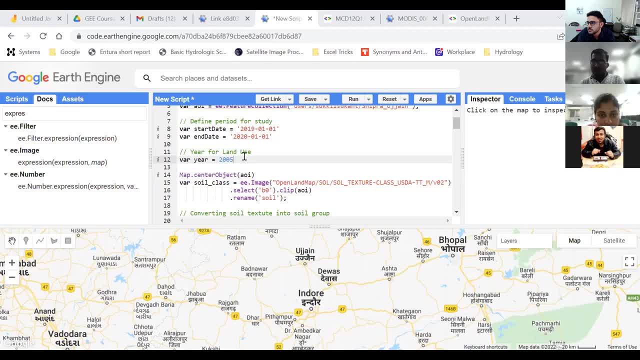 yes, uh, so if you want to just see the lulc chain, you can lulc chain, you can lulc chain. you can change this value like 2005 to 2015 and change this value like 2005 to 2015, and change this value like 2005 to 2015, and you can separately visualize the data. 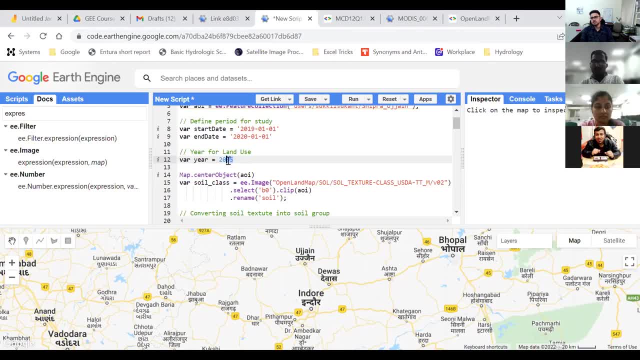 you can separately visualize the data. you can separately visualize the data. but if you want to analyze the uh, how? but if you want to analyze the uh, how? but if you want to analyze the uh, how much amount of much amount of much amount of uh classes has been converted from this? 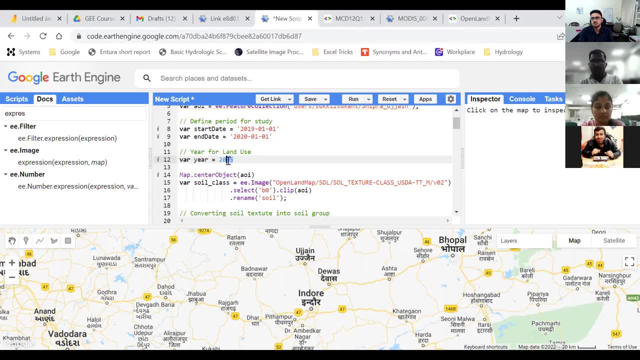 uh classes has been converted from this uh classes has been converted from this class to that class, class to that class, class to that class. so for that purpose, you need to uh write. so, for that purpose, you need to uh write. so, for that purpose, you need to uh write a code, a separate code of zonin. 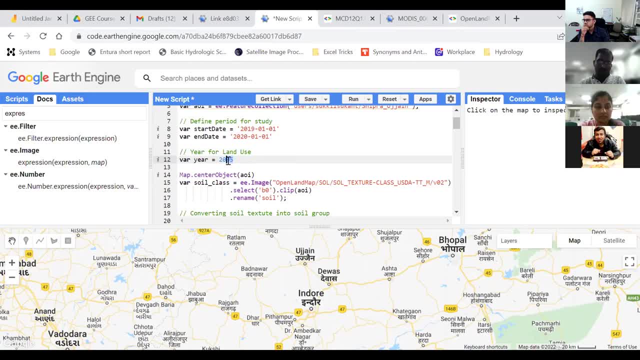 a code, a separate code of zonin, a code, a separate code of zonin statics in the earth engine, statics in the earth engine statics in the earth engine. uh, i will tell you in detail at the end. uh, i will tell you in detail at the end. 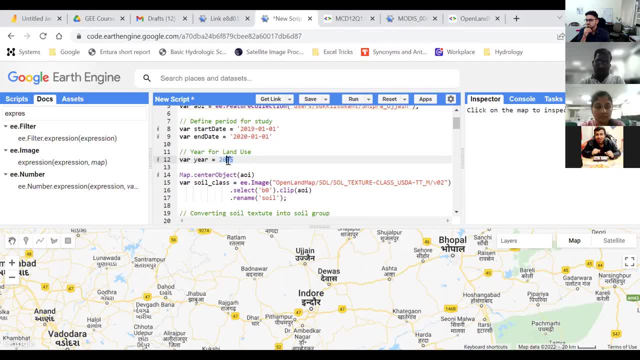 uh, i will tell you in detail at the end of the session. because at the end of the of the session, because at the end of the of the session, because at the end of the session we are preparing actually a chart session. we are preparing actually a chart. 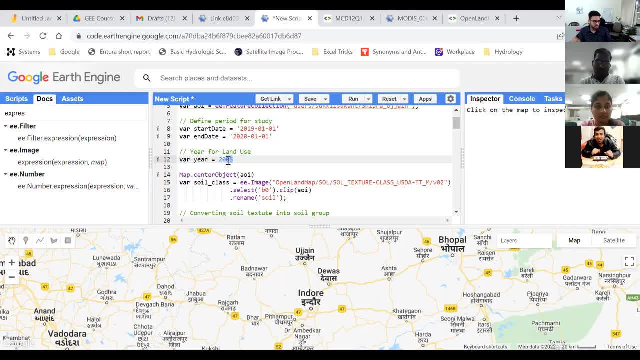 session. we are preparing actually a chart, so what this chart is actually doing. it so what this chart is actually doing. it so what this chart is actually doing: it is computing the average rainfall and is computing the average rainfall and is computing the average rainfall and average average. 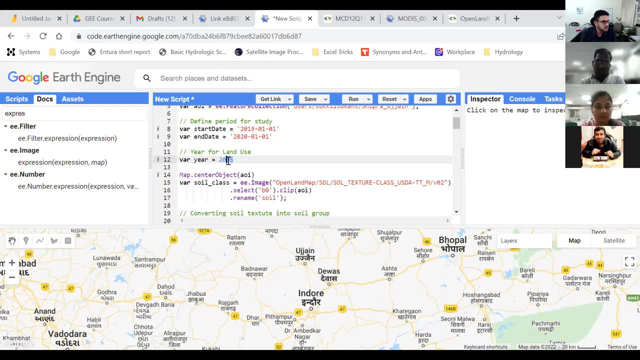 average runoff for your area. so you can use runoff for your area, so you can use runoff for your area, so you can use those similar charts for those similar charts, for those similar charts for land use. only so for that purpose you. land use, only so for that purpose, you. 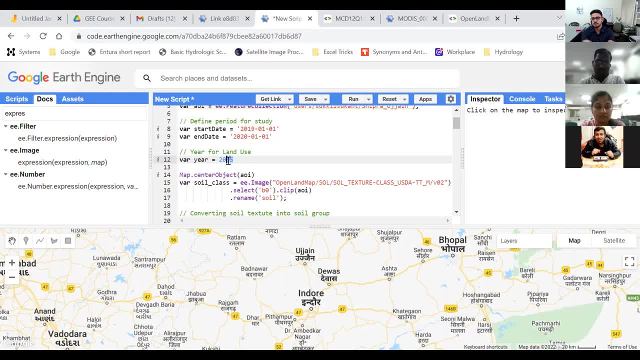 land use only so for that purpose you can create two charts, can create two charts. can create two charts: one from 2005- value will see, and from one from 2005- value will see. and from one from 2005- value will see and from 2015 values. 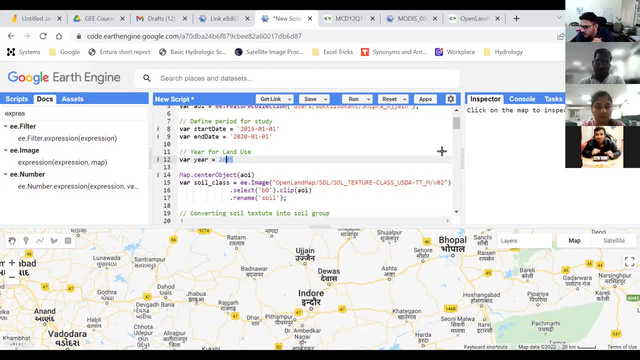 2015 values- 2015 values. i hope, uh, you get get things clear. i hope, uh, you get get things clear. i hope, uh, you get get things clear. yeah, we got thank you from pavan and yeah, we got thank you from pavan and yeah, we got thank you from pavan and jiraj. i think their questions are. 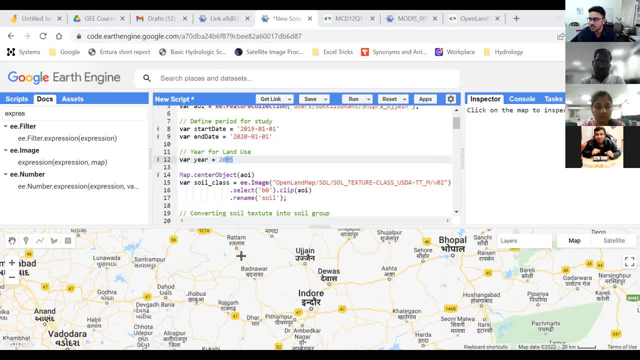 jiraj. i think their questions are jiraj. i think their questions are answered. so i think that's all there are answered. so i think that's all there are answered. so i think that's all. there are a couple of questions which are general. a couple of questions which are general. 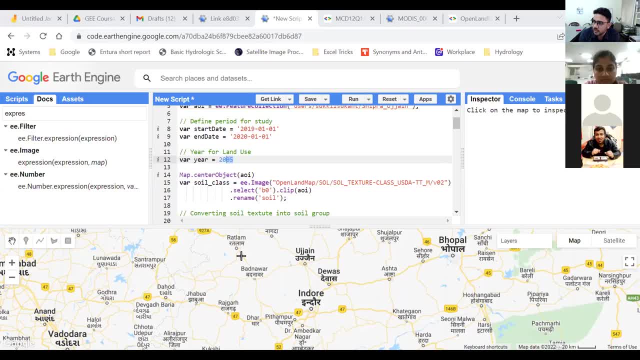 a couple of questions which are general in nature, so we'll take. probably we'll in nature, so we'll take. probably we'll in nature, so we'll take. probably we'll take in the end, take in the end, take in the end. excuse me, sir, can i ask a question? 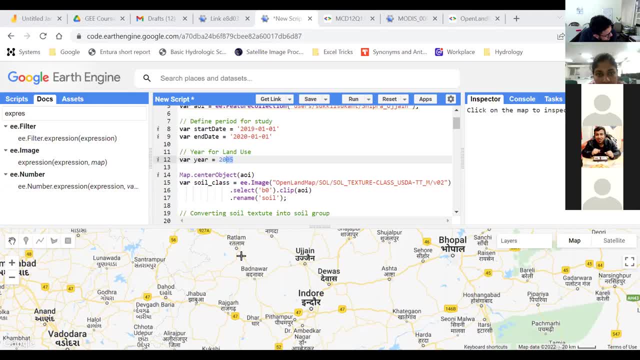 excuse me, sir, can i ask a question? excuse me, sir, can i ask a question? yes, sure uh, yeah uh. yes, sure uh, yeah uh. yes, sure uh, yeah uh, sukant. i just i was curious about the sukant. i just i was curious about the sukant. i just i was curious about the script which you just shared. so i just 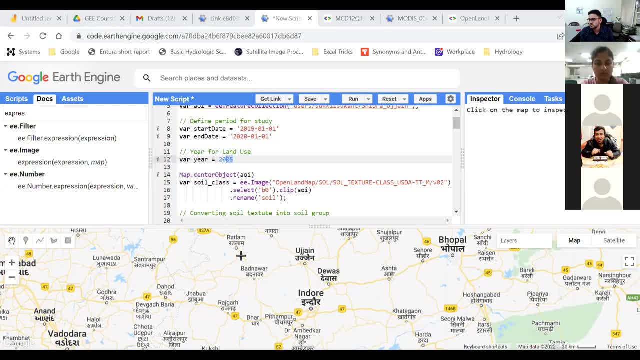 script which you just shared. so i just script which you just shared. so i just changed the, changed the changed the area of interest with my shape file for area of interest. with my shape file for area of interest. with my shape file for alaknanda: alaknanda. 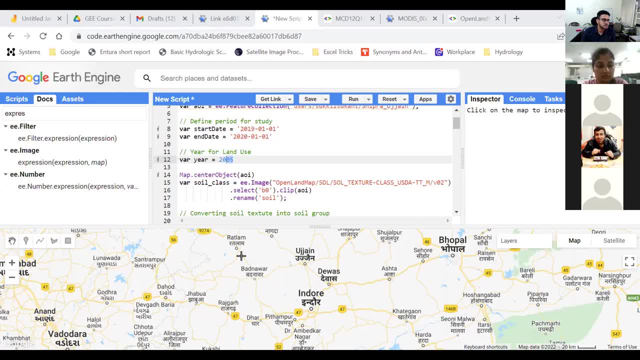 alaknanda watershed: okay, okay. so when once the watershed, okay, okay. so when once the watershed, okay, okay. so when once the script was run, so i was just checking script was run, so i was just checking script was run, so i was just checking the cn values, so i just observed that. 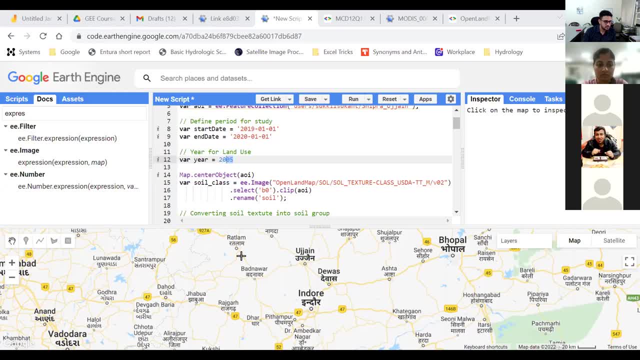 the cn values. so i just observed that the cn values. so i just observed that in the snow covered areas, the cm value in the snow covered areas, the cm value in the snow covered areas, the cm value is displaying as 100 is displaying as 100 is displaying as 100. but like this is like i was also. 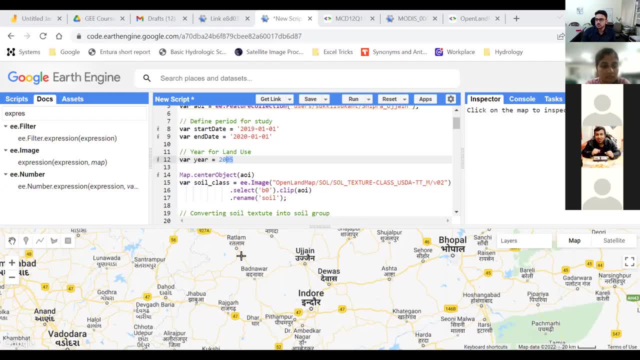 but like this is like i was also. but like this is like i was also curious about what to take the. i was curious about what to take the. i was curious about what to take the. i was preparing this map for my own study. preparing this map for my own study. 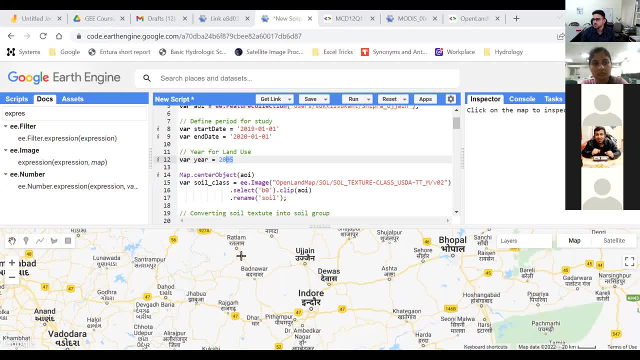 preparing this map for my own study before this. so i always have a doubt before this. so i always have a doubt before this. so i always have a doubt: what cn should we? what cn should we? what cn should we assign for snow areas? and i could not. 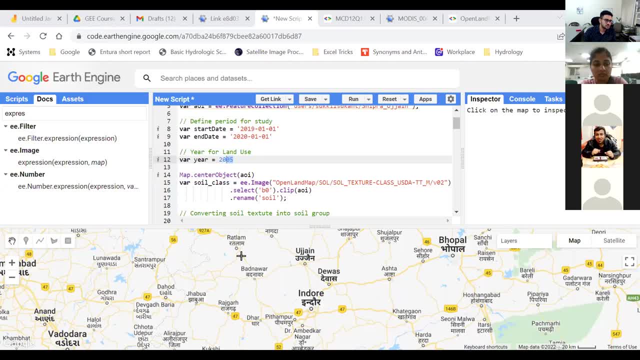 assign for snow areas and i could not assign for snow areas and i could not find a proper find, a proper find, a proper uh explanation in the literature also. so i uh explanation in the literature also. so i uh explanation in the literature also. so i just want to know: 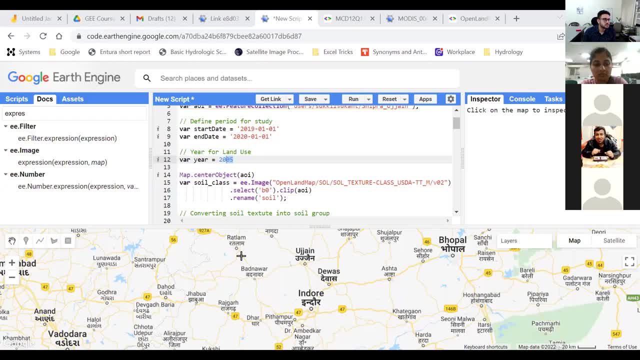 just want to know, just want to know: how did you like using your script? yes, how did you like using your script? yes, how did you like using your script? yes, it is showing hundreds. it is showing hundreds. it is showing hundreds, uh, so uh, thank you for asking putting. 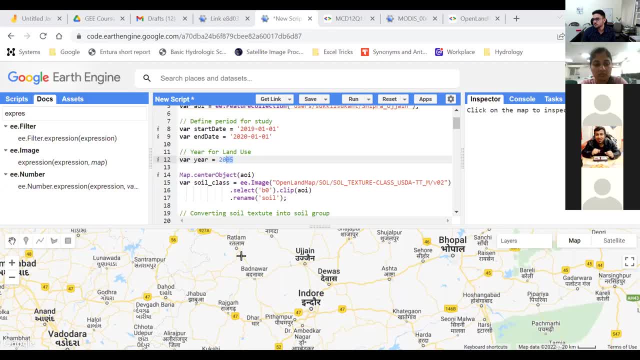 uh. so uh, thank you for asking putting uh. so uh, thank you for asking, putting this question. because this question, because this question, because, uh, there is a negative side of come. uh, there is a negative side of come. uh, there is a negative side of come. number technique is that. 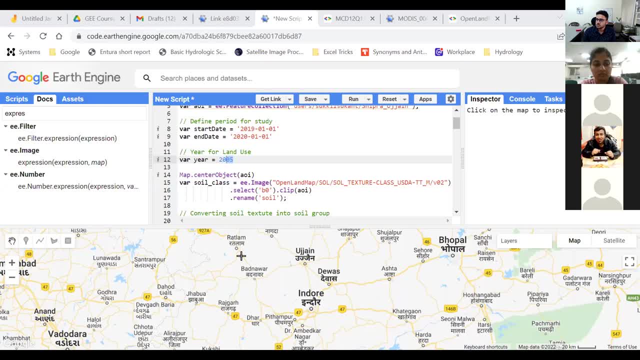 number technique. is that number technique? is that it is not advisable for snow area? yes, it is not advisable for snow area. yes, it is not advisable for snow area. yes, because i have uh used the many of the, because i have uh used the many of the, because i have uh used the many of the script. 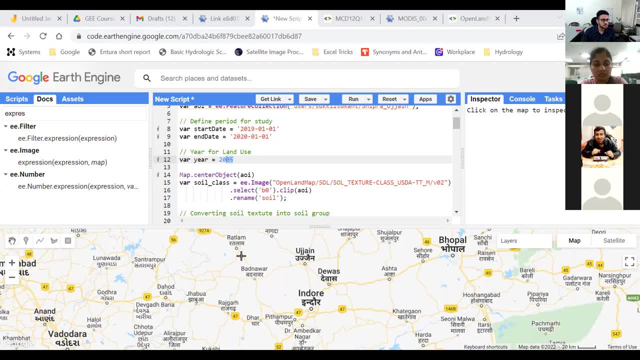 script, script literatures. so there is no definite cn literatures. so there is no definite cn literatures. so there is no definite cn number for number, for number for snow area. but if somehow you define some snow area, but if somehow you define some snow area, but if somehow you define some some curve number of snow area either. 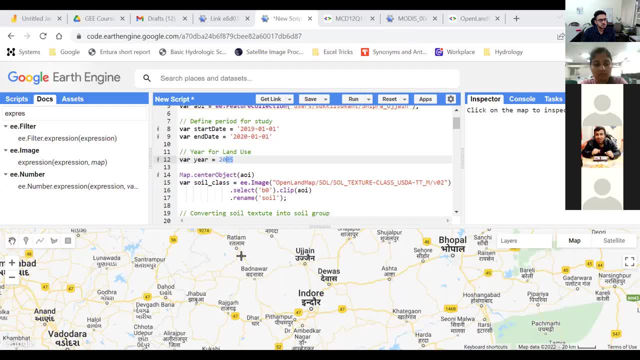 some curve number of snow area, either some curve number of snow area, either nearby 100 or nearby zero, but the nearby 100 or nearby zero, but the nearby 100 or nearby zero. but the conversion of uh, conversion of uh, conversion of uh, that snowfall into the runoff will be. 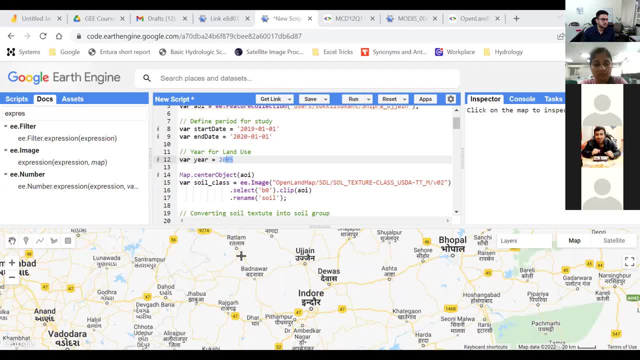 that snowfall into the runoff will be, that snowfall into the runoff will be inaccurate. why? because converting uh inaccurate. why because converting uh inaccurate? why? because converting uh snowfall into runoff will depend on. snowfall into runoff will depend on several factors, not only on the rainfall. 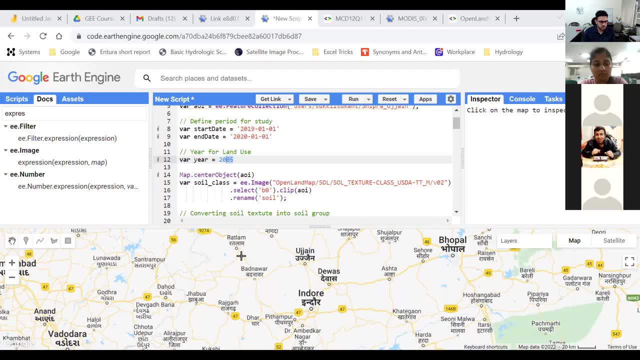 several factors not only on the rainfall. several factors not only on the rainfall. it will depend on the temperature it. it will depend on the temperature it. it will depend on the temperature. it will depend on the radiation inward and will depend on the radiation inward and will depend on the radiation inward and output region. 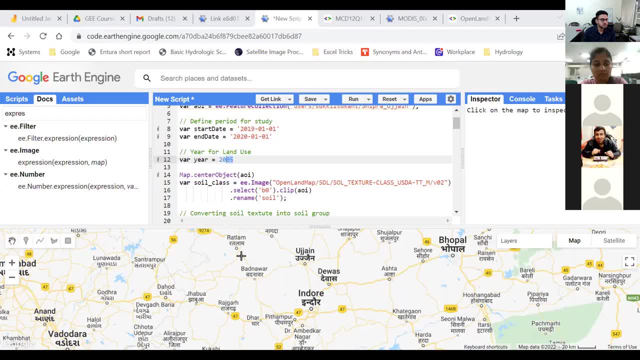 output region, output region. so that is why uh curve number technique. so that is why uh curve number technique. so that is why uh curve number technique totally depends on the rainfall, totally depends on the rainfall, totally depends on the rainfall elevation soil. so that's why, for hilly uh 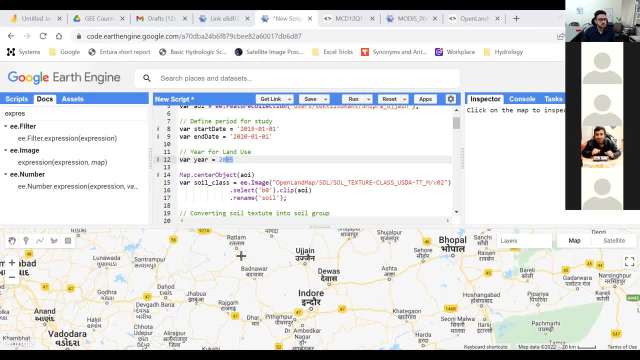 elevation soil. so that's why for hilly uh elevation soil. so that's why for hilly uh, for snowy part, for snowy part, for snowy part, curve number model is not suggested, curve number model is not suggested, curve number model is not suggested. so that's why you won't get easily the 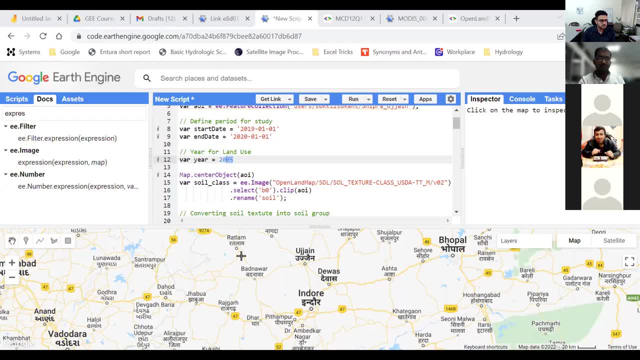 so that's why you won't get easily the. so that's why you won't get easily the curve number of snow area. curve number of snow area. curve number of snow area. but if, uh, if there are, if any, some. but if, uh, if there are, if any, some. 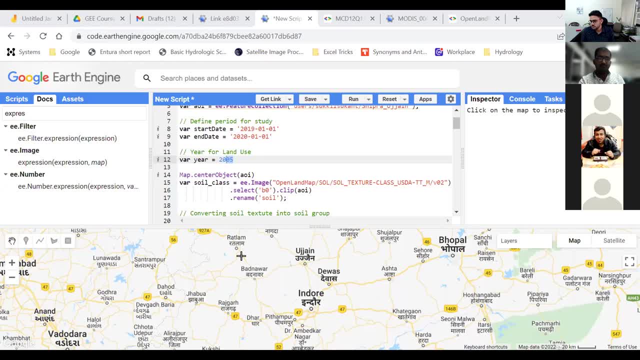 but if, uh, if there are, if any, some literature is there? literature is there? literature is there in which, uh, the conversion of count number, in which, uh, the conversion of count number, in which, uh, the conversion of count number runoff will be used as an input to some? 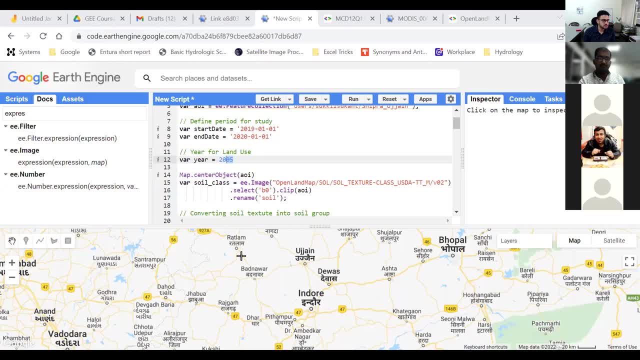 runoff will be used as an input to some runoff will be used as an input to some other model, other model, other model for a snow watershed. you can use that for a snow watershed. you can use that for a snow watershed. you can use that. okay, and one more thing i want to ask. 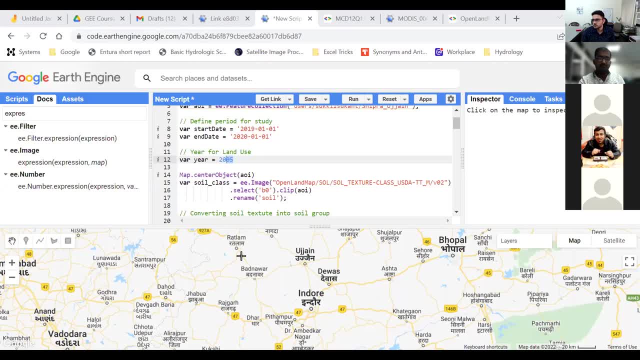 okay, and one more thing i want to ask, okay, and one more thing i want to ask, like, if, uh, like, if uh like, if uh for a snow like snow covered watershed, if for a snow like snow covered watershed, if for a snow like snow covered watershed, if we want to neglect those areas or 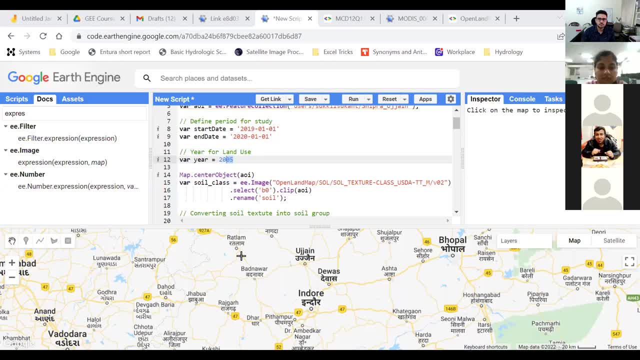 we want to neglect those areas, or we want to neglect those areas or ignore those areas. so what change should ignore those areas? so what change should ignore those areas? so what change should we make in the code? we make in the code we make in the code like, because we don't have a proper cn. 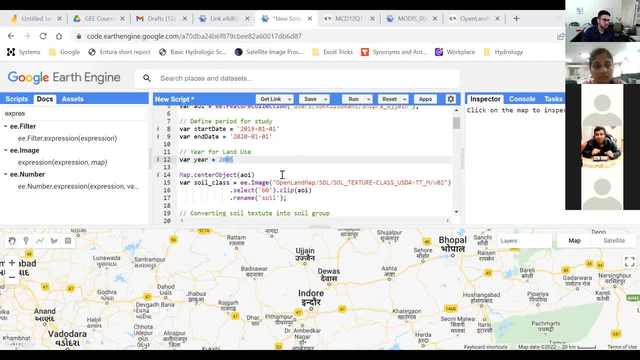 like because we don't have a proper cn, like because we don't have a proper cn. values for this: yes, yes. values for this: yes, yes. values for this, yes, yes. so what you can do: yes, so, if you go to. so, what you can do, yes, so if you go to. 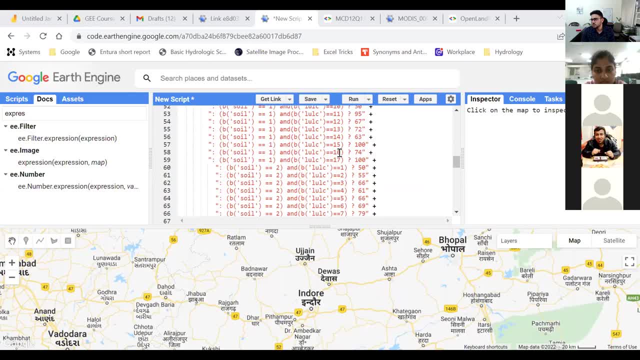 so what you can do, yes, so if you go to this code and if you suppose the lulc 16- this code, and if you suppose the lulc 16- this code, and if you suppose the lulc 16 is snow cover, yes, what you can do either. 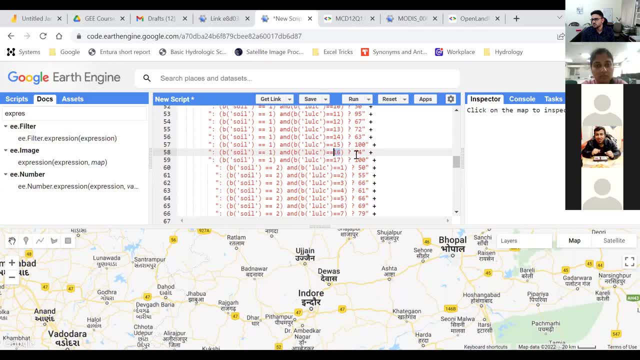 is snow cover. yes, what you can do. either is snow cover. yes, what you can do. either you can incorporate uh the lulc 16, as you can incorporate uh the lulc 16, as you can incorporate uh the lulc 16 as zero. okay, or 100. 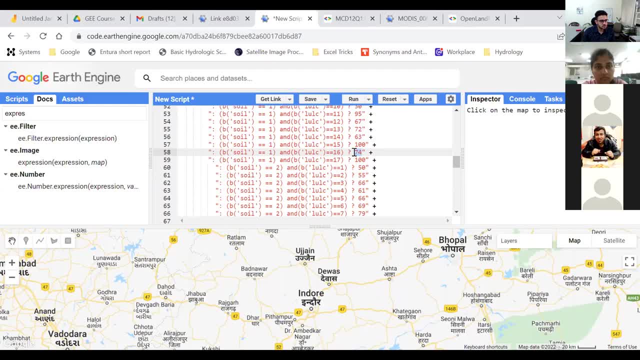 zero okay or 100. zero okay or 100, but please remember that if you go to zero, but please remember that if you go to zero, but please remember that if you go to zero, then the composite curve number will be. then the composite curve number will be: 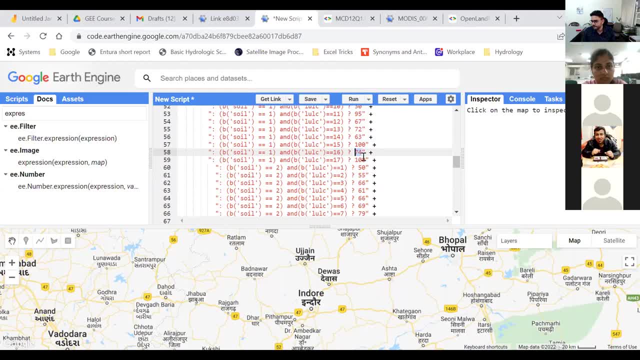 then the composite curve number will be fall down, fall down, fall down. yes. if you do the hundred, the composite: yes. if you do the hundred, the composite: yes. if you do the hundred, the composite curve number will give a higher value. curve number will give a higher value. 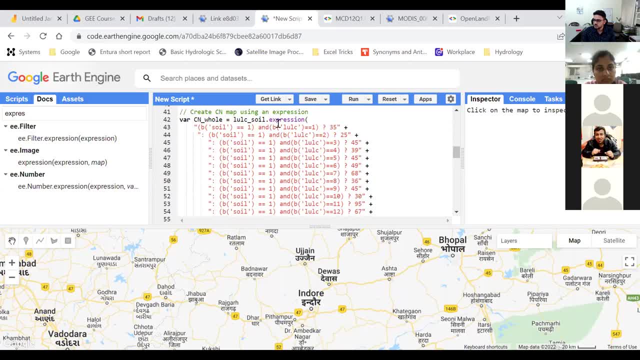 curve number will give a higher value. so what you can do, uh, you can simply uh. so what you can do, uh, you can simply uh. so what you can do, uh, you can simply uh, try, uh, try, uh, try uh. you can perform some hidden trial, that you can perform some hidden trial that. 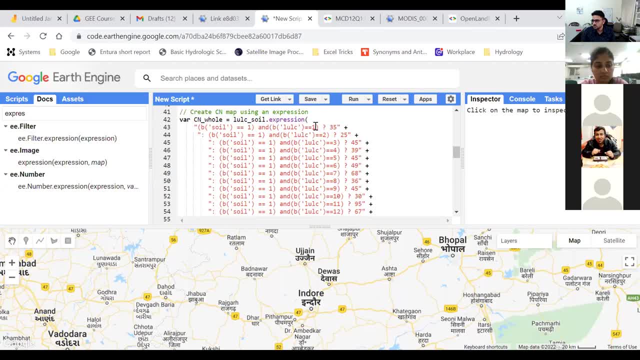 you can perform some hidden trial. that in the soil expression code you want to. in the soil expression code you want to. in the soil expression code you want to exclude, there is a command dot known as exclude. there is a command dot known as exclude. there is a command dot known as ged. 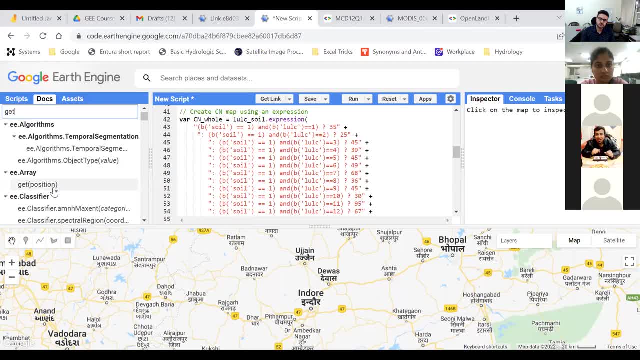 ged, ged if you go get, or greater than if you go get, or greater than if you go get, or greater than i'm forgetting, actually, i'm forgetting, actually, i'm forgetting actually, wait a minute, wait a minute. okay, so there is a command gt in the. okay, so there is a command gt in the. 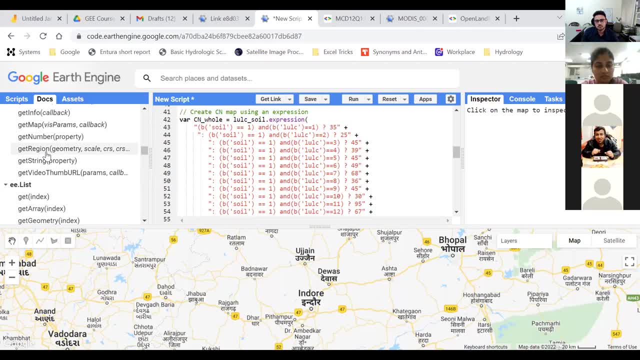 okay, so there is a command gt in the image collection and in the image which image collection and in the image which image collection and in the image which will tell you uh through which you can, will tell you uh through which you can, will tell you uh through which you can tell the. 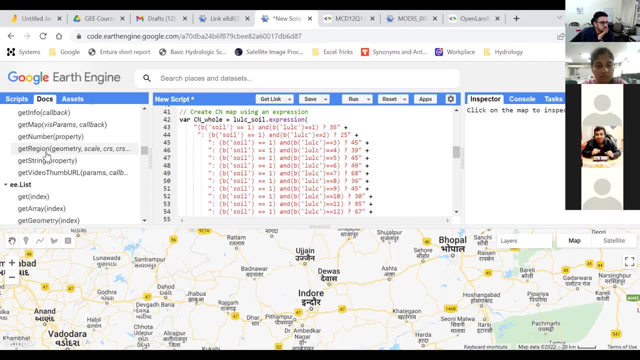 tell the tell the system that take only those pixels, which system that take only those pixels, which system that take only those pixels which having value greater than this or lower, having value greater than this or lower, having value greater than this or lower than this. so what we'll do, it will mosaic. 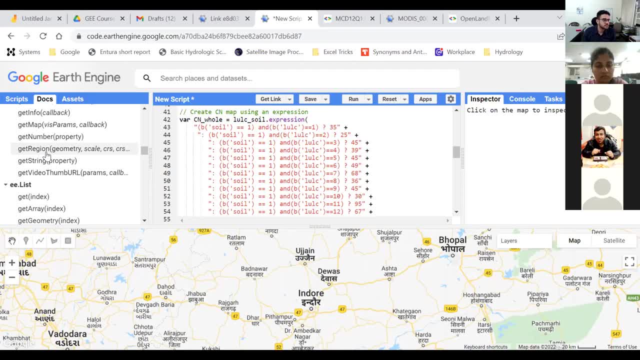 than this. so what we'll do, it will mosaic than this. so what we'll do, it will mosaic out all those unwanted pixels. after that, out all those unwanted pixels. after that, out all those unwanted pixels. after that, you can perform the lulc classification. you can perform the lulc classification. 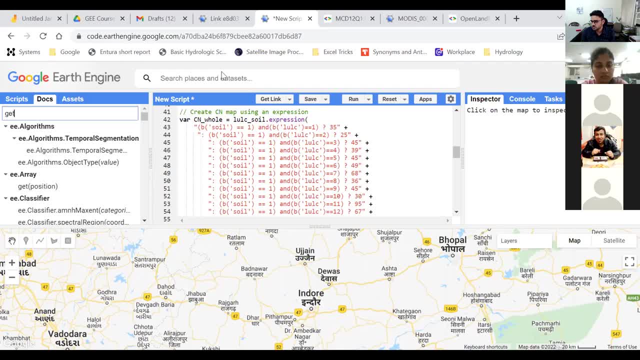 you can perform the lulc classification. okay, okay, okay, okay, thank you. so we can proceed further. so we can proceed further. so we can proceed further. yeah, if you uh, yeah, if you uh, yeah, if you uh. questions, we have the questions, but i questions, we have the questions, but i. 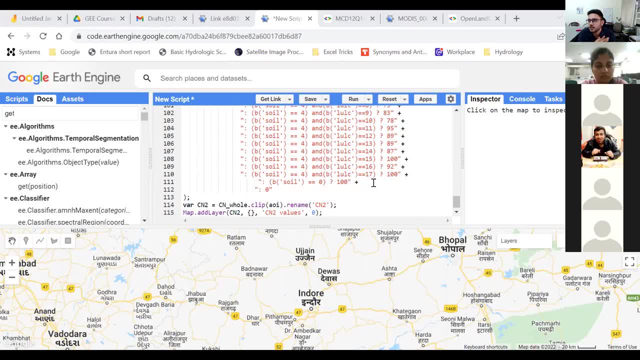 questions. we have the questions, but i would say uh, would say uh, would say uh, actually i mean uh in by this code. we actually i mean uh in. by this code, we actually i mean uh in. by this code we can incorporate the temperature data, can incorporate the temperature data. 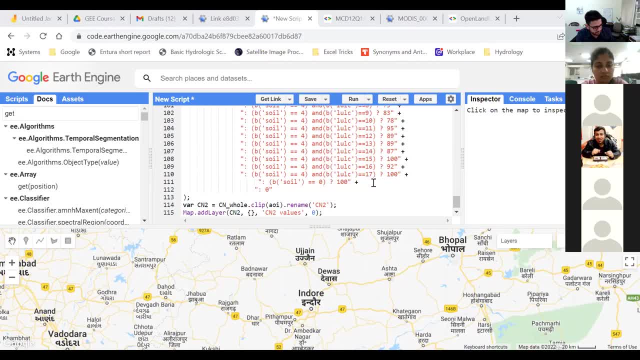 can incorporate the temperature data, so uh, the count number doesn't import in. so uh, the count number doesn't import in, so uh, the count number doesn't import in. uh, incorporate the? uh the temperature. uh, incorporate the? uh the temperature. uh, incorporate the? uh the temperature into their formula. but if you come up 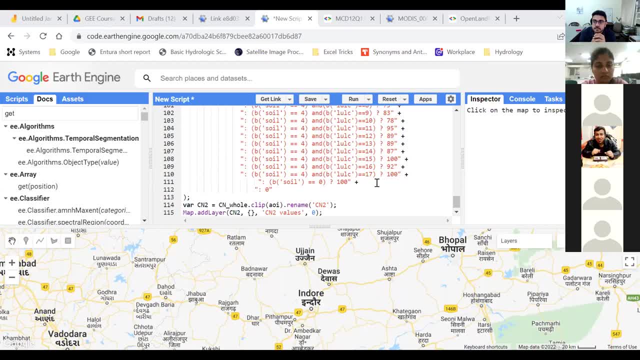 into their formula. but if you come up into their formula, but if you come up any new literature, any new literature, any new literature which is utilizing the temperature, which is utilizing the temperature, which is utilizing the temperature, incorporating in with the lulc and soil, incorporating in with the lulc and soil. 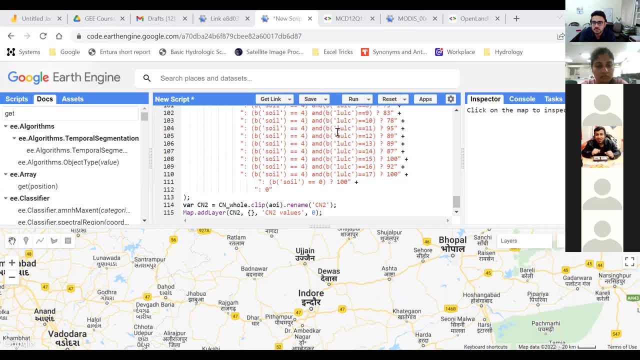 incorporating in with the lulc and soil. you can always have the temperature data. you can always have the temperature data. you can always have the temperature data because, because, because earth engine have lots of temperature, earth engine have lots of temperature, earth engine have lots of temperature data maximum. 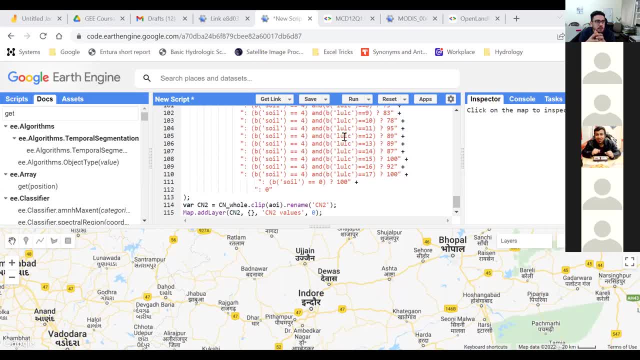 data: maximum data maximum like glds, flds and other data. noah data like glds, flds and other data. noah data like glds, flds and other data. noah data site is also there. you can utilize. your site is also there. you can utilize your. 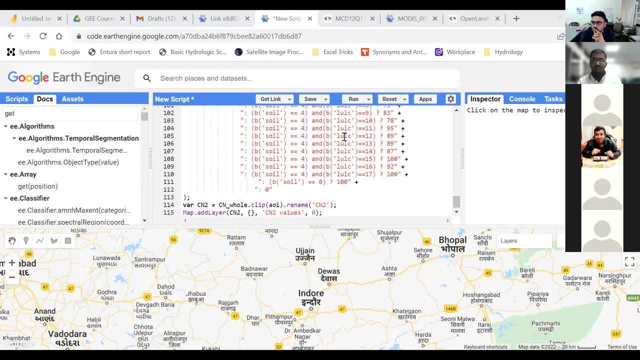 site is also there. you can utilize your data because i mean here in, i mean i'm data, because i mean here in. i mean i'm data because i mean here in, i mean i'm staying in punjab, staying in punjab, staying in punjab. so here there will be some amount of snow. 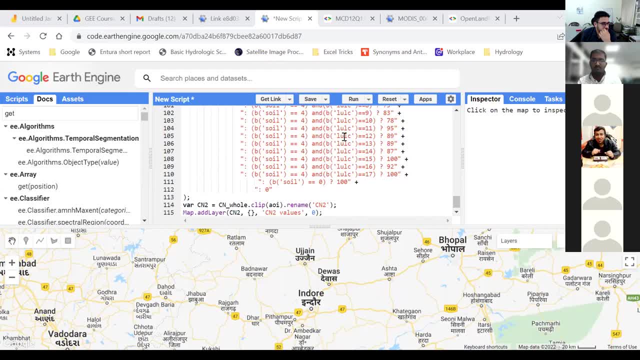 so here there will be some amount of snow. so here there will be some amount of snow cover. i mean if temperature decreases cover. i mean if temperature decreases cover. i mean if temperature decreases, then we can consider it as a snowfall, then we can consider it as a snowfall. 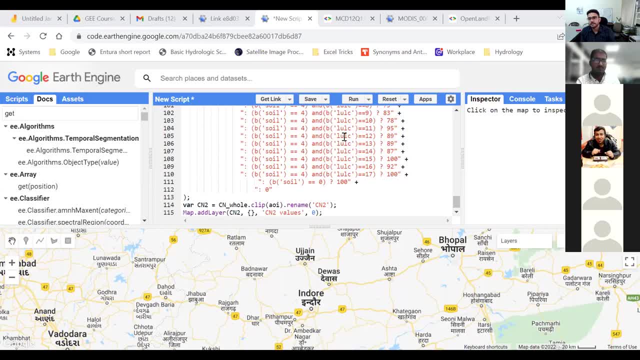 then we can consider it as a snowfall temperature increases, then it's temperature increases, then it's temperature increases, then it's considered just more enough, like that, considered just more enough, like that, considered just more enough, like that. so it is my personal advice, um, so it is my personal advice, um. 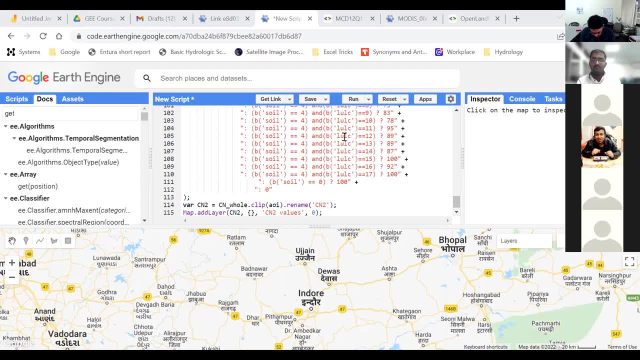 so it is my personal advice, um, as an hydrologist, that if you are using as an hydrologist that, if you are using as an hydrologist that, if you are using any uh, any uh, any uh, doing modeling for a snow cover area, yeah, 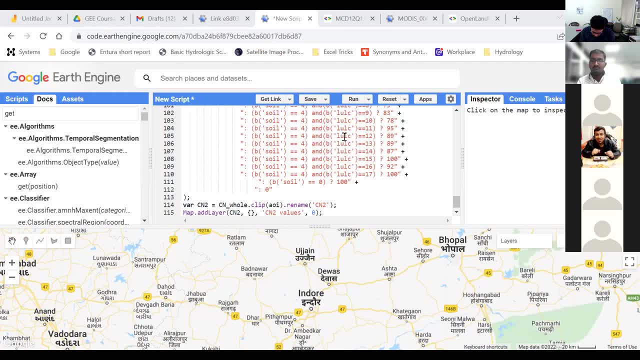 doing modeling for a snow cover area? yeah, doing modeling for a snow cover area? yeah, yeah, i mean we are doing. i mean then, yeah, i mean we are doing. i mean then, yeah, i mean we are doing. i mean, then, don't use the current number method. don't use the current number method. 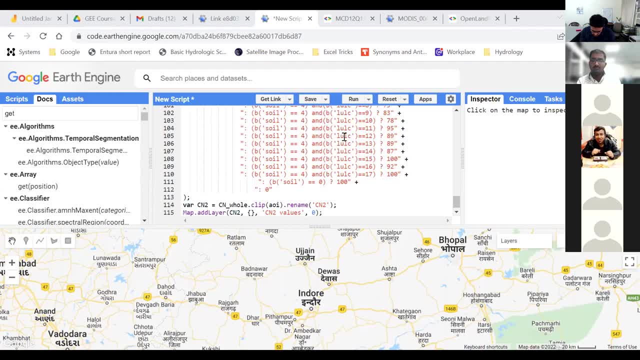 don't use the current number method, either use some what we can say, either use some what we can say, either use some what we can say, physical balance approach, either from physical balance approach, either from physical balance approach, either from big model, big model, big model, swat model, or maybe hms is there, so you 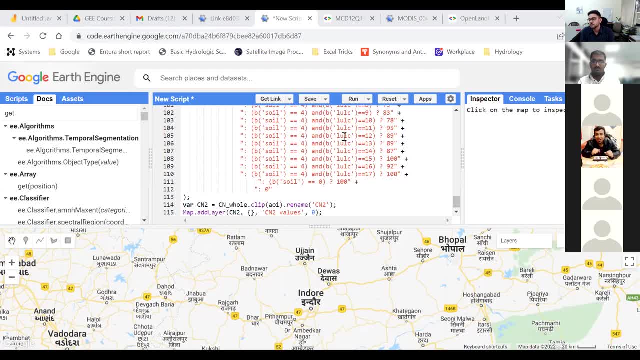 swat model or maybe hms is there. so you swat model or maybe hms is there, so you have to go with some advanced model or have to go with some advanced model, or have to go with some advanced model or there's no fed model. is there snow mod? 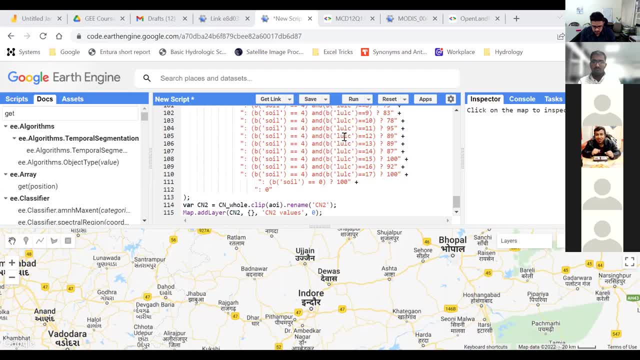 there's no fed model. is there snow mod? there's no fed model. is there snow mod model? is there, you can go with that model. is there, you can go with that model? is there, you can go with that model? not the curve number. okay, it is carbon number model, i mean. 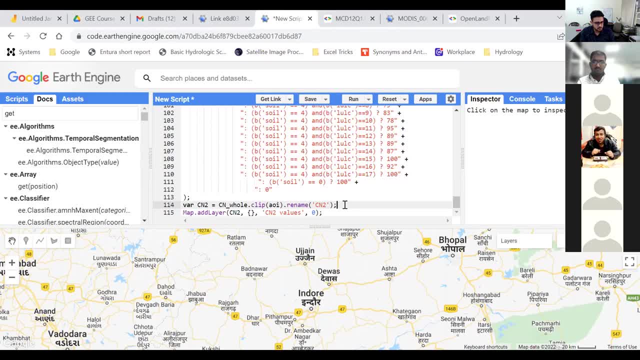 okay, it is carbon number model. i mean: okay, it is carbon number model. i mean only based upon the carbon number. yes, it only based upon the carbon number. yes, it only based upon the carbon number. yes, it is only based on the common one. okay, so is only based on the common one. okay so. 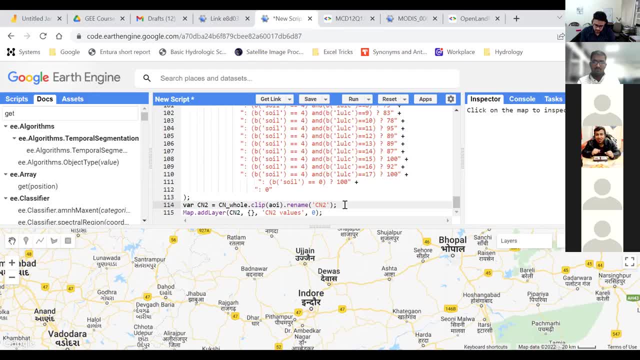 is only based on the common one. okay, so you can explore anything because see. you can explore anything because see. you can explore anything because see, either if you are adopting any type of either, if you are adopting any type of either, if you are adopting any type of model, any type of equation. 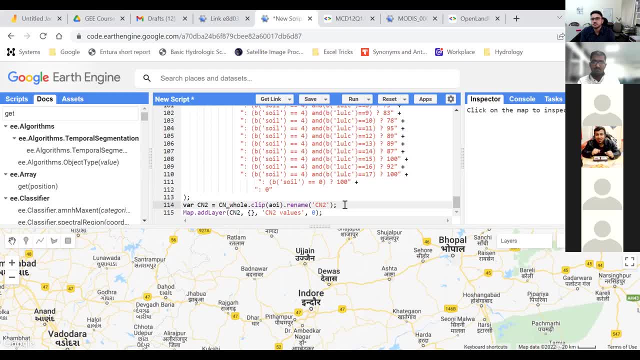 model, any type of equation model, any type of equation, you will require certain type of inputs. you will require certain type of inputs. you will require certain type of inputs if you are able to incorporate those, if you are able to incorporate those, if you are able to incorporate those equations in the earth engine, you can. 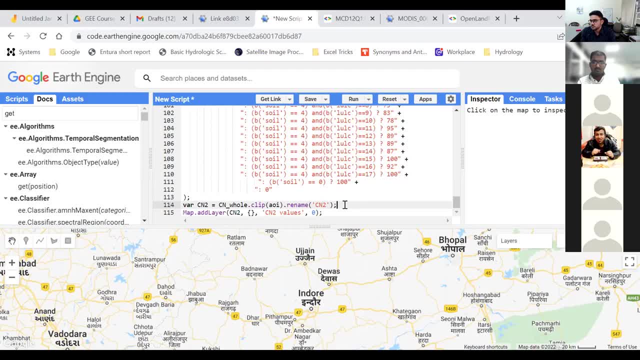 equations in the earth engine. you can equations in the earth engine. you can develop your own model, develop your own model, develop your own model. that means a cloud-based model. so that means a cloud-based model. so that means a cloud-based model. so presently, i have developed the curve. 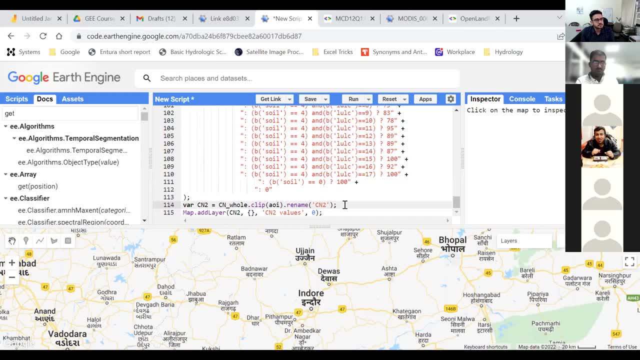 presently i have developed the curve. presently i have developed the curve number model, because it is a very number model, because it is a very number model, because it is a very simplistic approach. if you come up very simplistic approach, if you come up very simplistic approach, if you come up very new algorithm, you can incorporate your 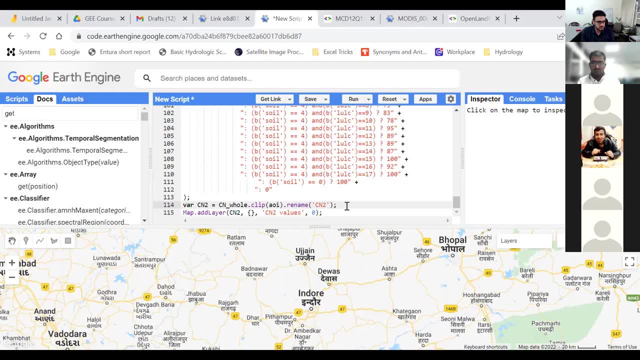 new algorithm. you can incorporate your new algorithm. you can incorporate your own in the earth engine, own in the earth engine, own in the earth engine, because all you need is the data set and because all you need is the data set, and because all you need is the data set and the formula. 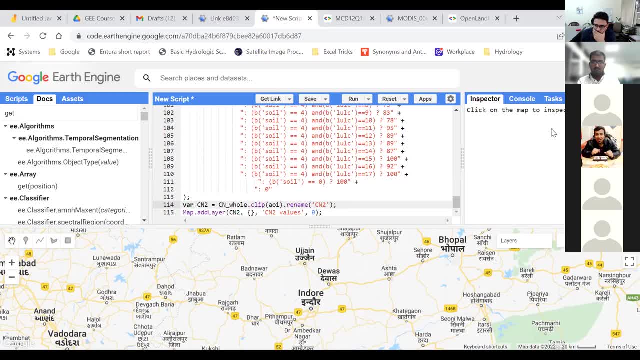 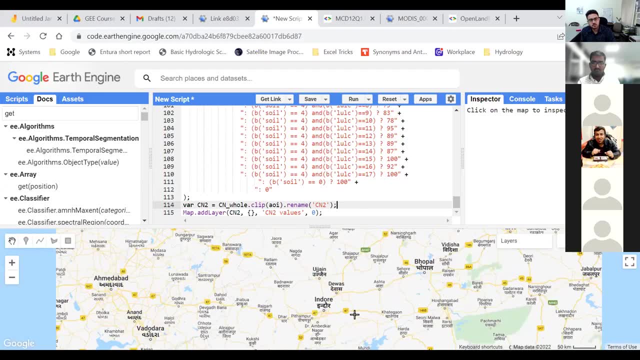 the formula, the formula nothing. so uh, so, uh, so uh. we will just quickly go to the next part. we will just quickly go to the next part. we will just quickly go to the next part of the session. that means of the session. that means of the session. that means now we have created the term number map. 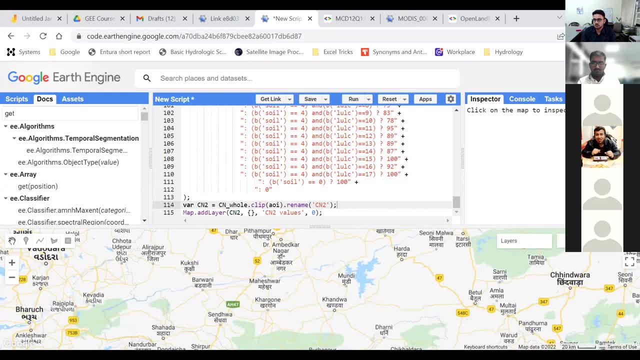 now we have created the term number map. now we have created the term number map. now, the next thing that we have to uh now, the next thing that we have to uh now, the next thing that we have to uh, look, it is the antecedent moisture. 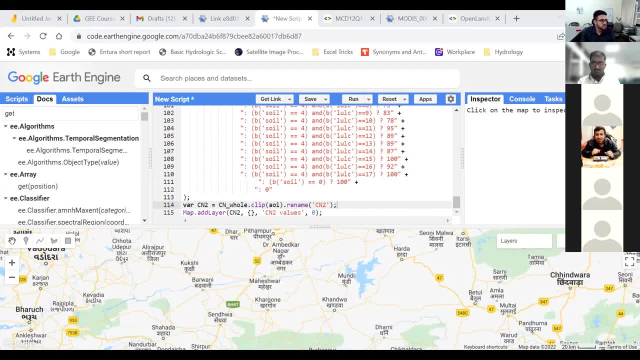 look, it is the antecedent moisture. look, it is the antecedent moisture condition. so what is actually antecedent condition? so what is actually antecedent condition? so what is actually antecedent moisture condition that i've told you, moisture condition that i've told you. 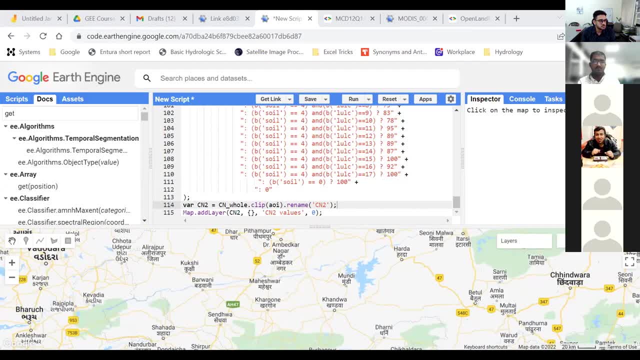 moisture condition that i've told you that, that that if the rainfall is um, if the rainfall is um, if the rainfall is um, having certain amount of rainfall is having certain amount of rainfall, is having certain amount of rainfall is there from past 13 days or from past uh. 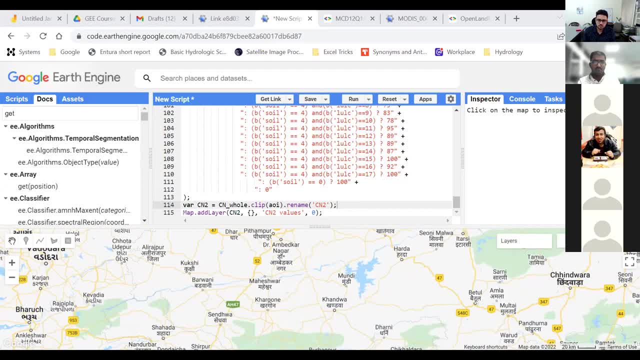 there from past 13 days or from past. uh, there from past 13 days or from past. uh, sorry, sorry, sorry, from past five days. if the certain amount from past five days, if the certain amount from past five days, if the certain amount of rainfall is there, then it is come. 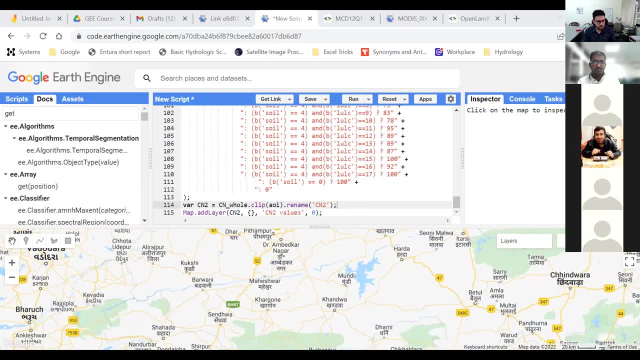 of rainfall. is there, then it is come of rainfall. is there, then it is come under the amc1, amc2 and amc3. under the amc1, amc2 and amc3. under the amc1, amc2 and amc3. okay, and if the amc is changing from 2: 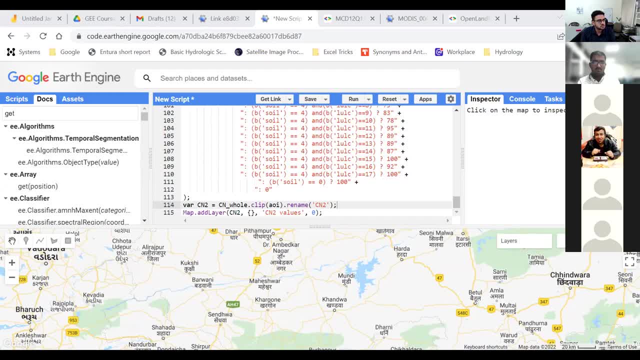 okay. and if the amc is changing from 2, okay. and if the amc is changing from 2 to 3 or 2 to 1, then the curve number to 3 or 2 to 1, then the curve number to 3 or 2 to 1, then the curve number, corresponding curve number will change. 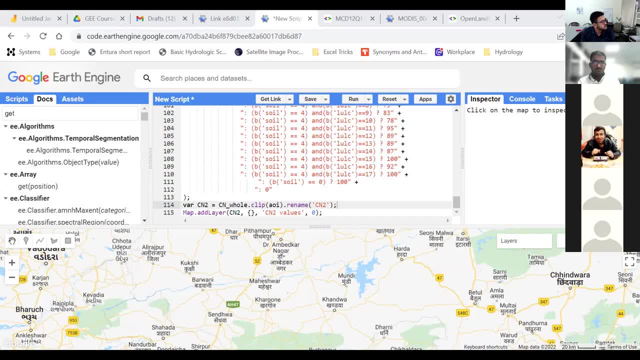 corresponding curve number will change, corresponding curve number will change. and for that purpose, and for that purpose, and for that purpose, first of all, we have to analyze the first of all, we have to analyze the first of all, we have to analyze the rainfall data set. so, if you go to the 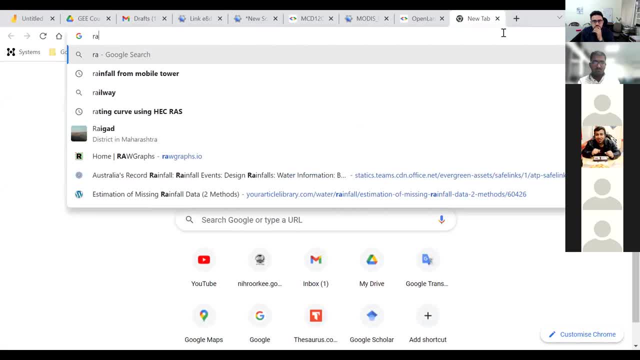 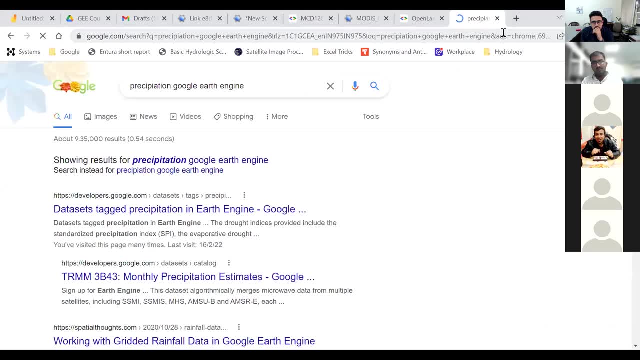 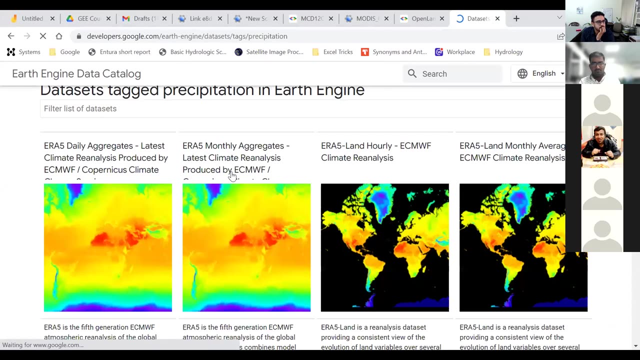 rainfall data set. so if you go to the rainfall data set, so if you go to the google again and search for google again, and search for google again and search for precipitation in google earth engine, okay, so you can get an amount of five maybe. so you can get an amount of five, maybe. 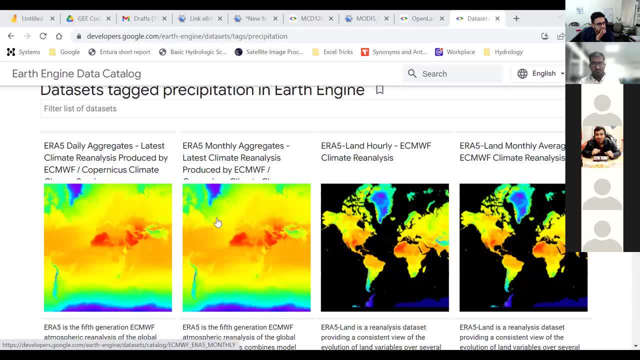 so you can get an amount of five, maybe six to seven type of data set, which is six to seven type of data set which is six to seven. type of data set which is useful for rainfall. so presently i have useful for rainfall. so presently i have useful for rainfall. so presently i have used a chirp data set. 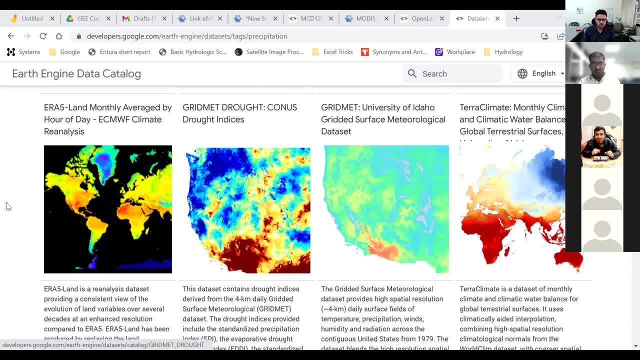 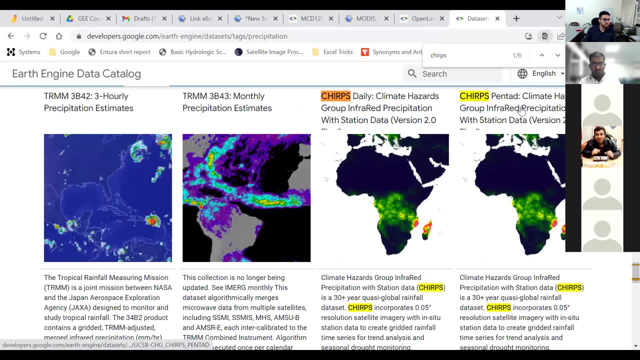 used a chirp data set. used a chirp data set. chirps daily. okay, okay, okay. chirp daily is available. just pentad is. chirp daily is available. just pentad is. chirp daily is available. just pentad is available. available. available if you click on this chirps daily data. 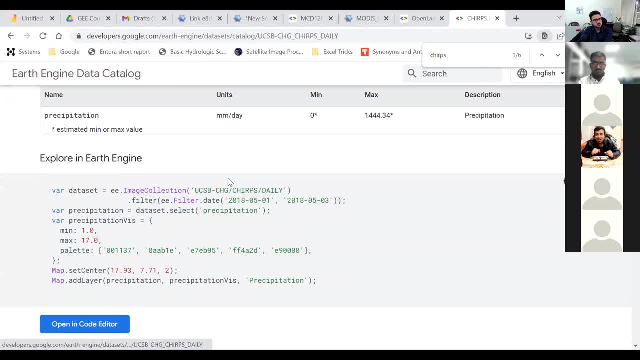 if you click on this chirps daily data. if you click on this chirps daily data site, it provides the rainfall in mm site. it provides the rainfall in mm site. it provides the rainfall in mm- the daily rainfall- and you can access the daily rainfall and you can access. 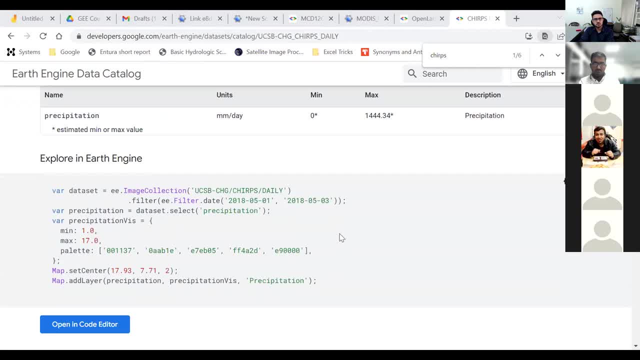 the daily rainfall and you can access this code, or if you want to access this code. or if you want to access this code, or if you want to access for a particular, so i'll just open this for a particular. so i'll just open this for a particular. so i'll just open this data set. 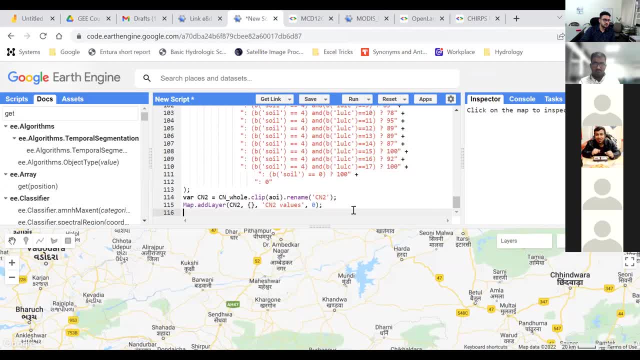 data set. data set: okay, and so i have actually utilizing the. so i have actually utilizing the, so i have actually utilizing the data data. data: data set from first of may 2018 to data set from first of may 2018 to data set from first of may 2018 to third of may 2018. 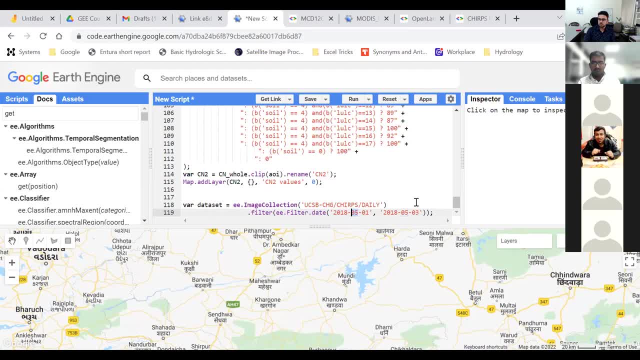 third of may 2018, third of may 2018, so so, so by 2018, can you hold for a one minute? i just, yeah sure, i think that would be fine. yeah sure, i think that would be fine. yeah sure, i think that would be fine. 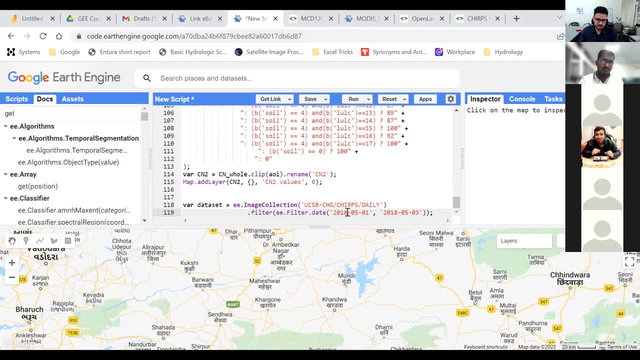 so sorry for the glitch, so here, uh, we so sorry for the glitch, so here uh, we so sorry for the glitch, so here, uh, we can write the date. either we can write, can write the date. either we can write the date here, or can write the date here, or or. 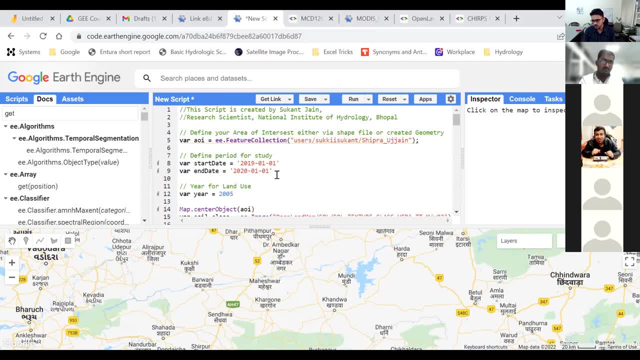 can write the date here, or. or we can actually define the date initially. we can actually define the date initially. we can actually define the date initially. uh in the initial part of the code. so for uh in the initial part of the code. so for uh in the initial part of the code. so, for example, if we have defined the period of 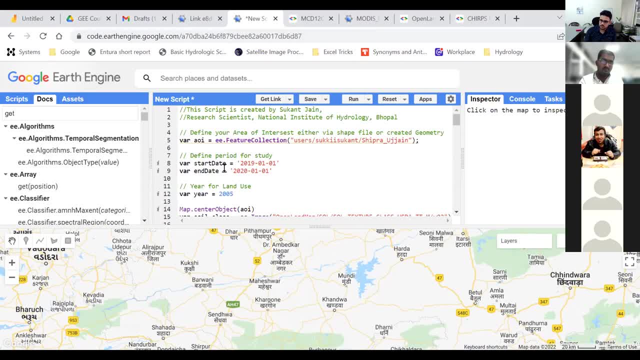 example, if we have defined the period of example, if we have defined the period of study at start date 2019 and end date study at start date 2019 and end date study at start date 2019 and end date 2020, so we can use this variable into. 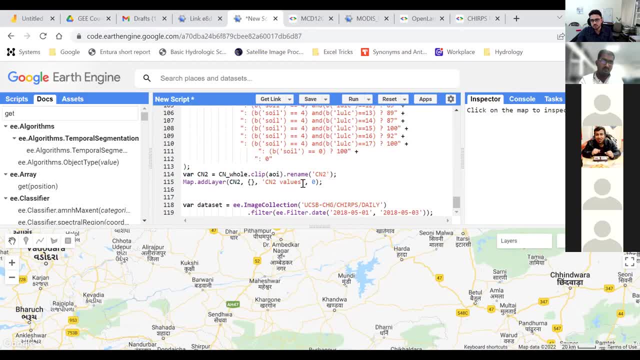 2020, so we can use this variable into 2020, so we can use this variable into our rainfall data set, our rainfall data set, our rainfall data set, start date, start date, start date. and we will put and we will put, and we will put the start date over here and we will. 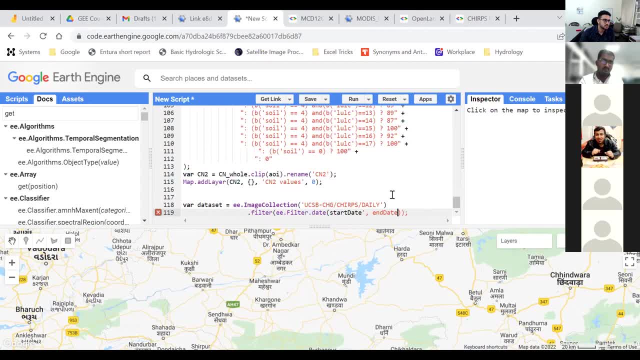 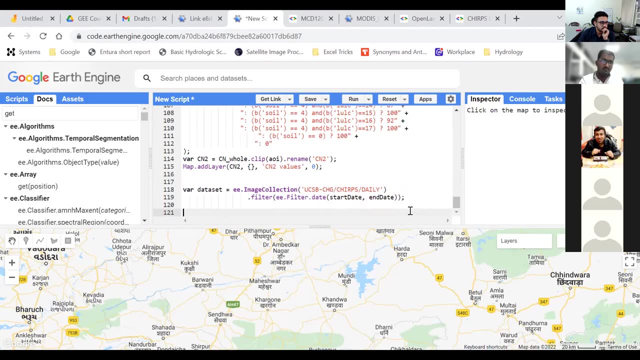 the start date over here and we will the start date over here and we will put it over here. and if i just print this data set, let's see what has actually happened in. let's see what has actually happened in. let's see what has actually happened in the. 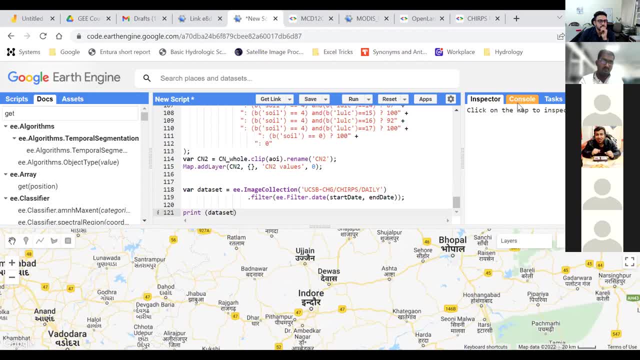 the the console panel. so now they have printed 365 image. why so now they have printed 365 image? why so now they have printed 365 image? why? because it is a daily data set and we because it is a daily data set and we because it is a daily data set and we have actually utilizing 365. 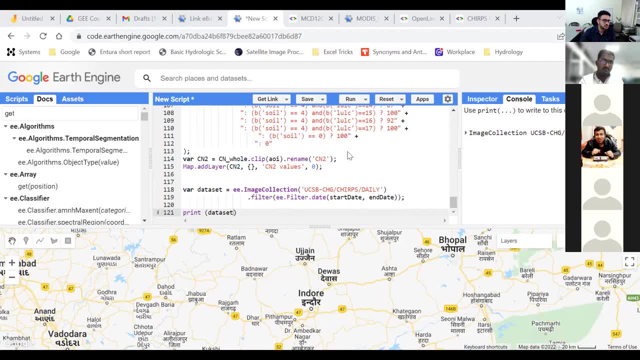 have actually utilizing 365, have actually utilizing 365 images, images, images. so now, after that, we have to calculate. so now, after that, we have to calculate. so now, after that, we have to calculate the amc condition. so for that purpose, we are actually uh. so for that purpose, we are actually uh. 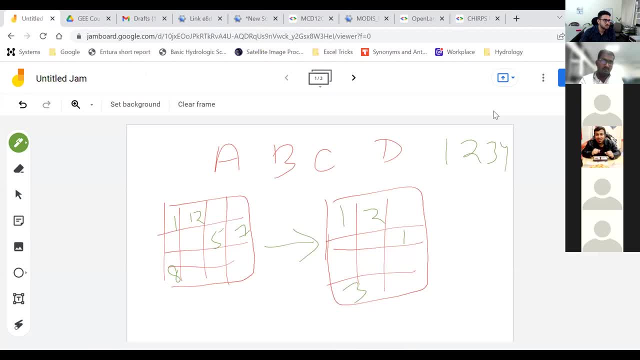 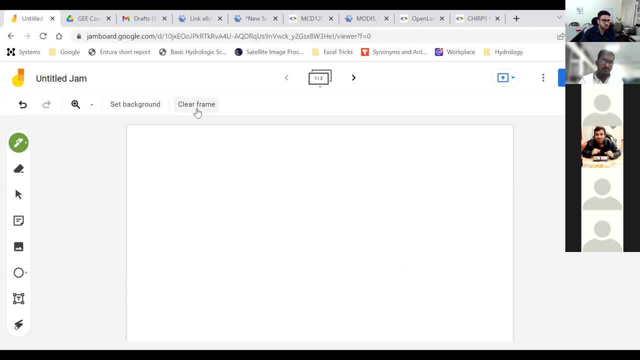 you use some programming language like python and java, so you have come up with python and java. so you have come up with python and java. so you have come up with a term loop, but in the a term loop, but in the a term loop, but in the earth engine javascript. 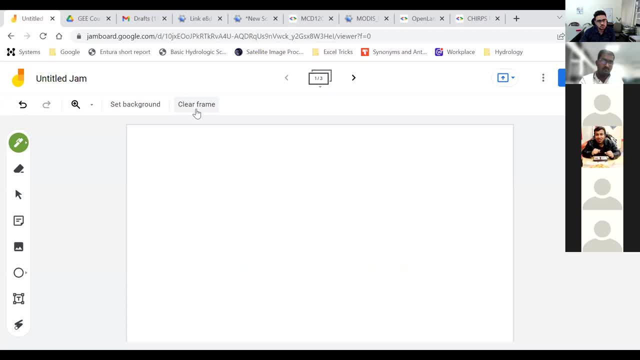 earth engine javascript. earth engine javascript. in their documents, they have generally in their documents, they have generally in their documents. they have generally suggested that don't use the loop, suggested that don't use the loop, suggested that don't use the loop because loop will actually hang. uh will. 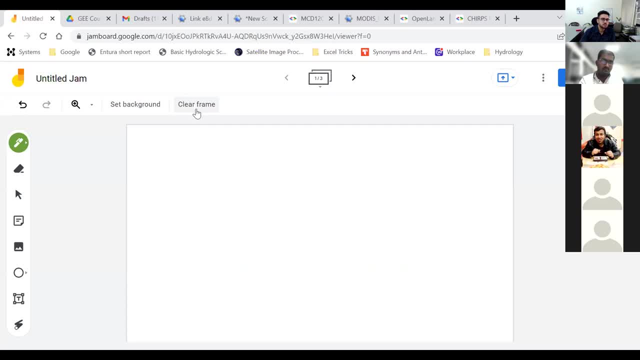 because loop will actually hang, uh will. because loop will actually hang, uh will result in hacking your code. result in hacking your code. result in hacking your code. and will uh not properly uh work and will uh not properly uh work and will uh not properly uh work can be done. so, what we can do, uh in. 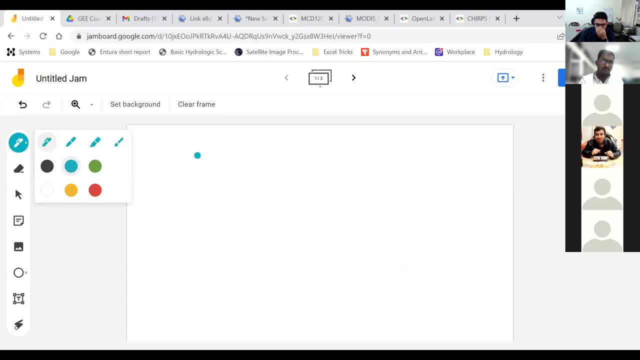 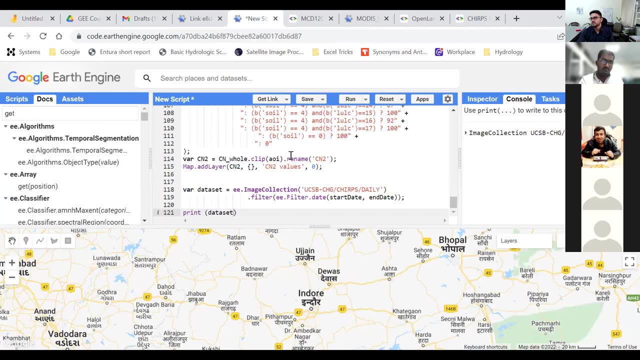 can be done. so what we can do, uh, in can be done. so what we can do, uh, in order to order, to order, to achieve this thing, we have to convert the achieve this thing. we have to convert the achieve this thing, we have to convert the image collection. okay, i just 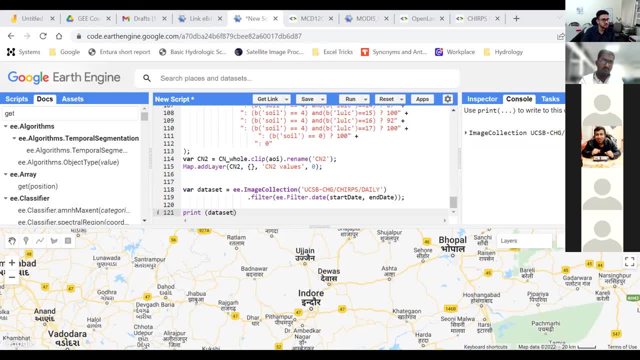 we have to convert this image collection. we have to convert this image collection. we have to convert this image collection into the list of images, into the list of images, into the list of images, and we can apply the functions if i open. and we can apply the functions if i open. 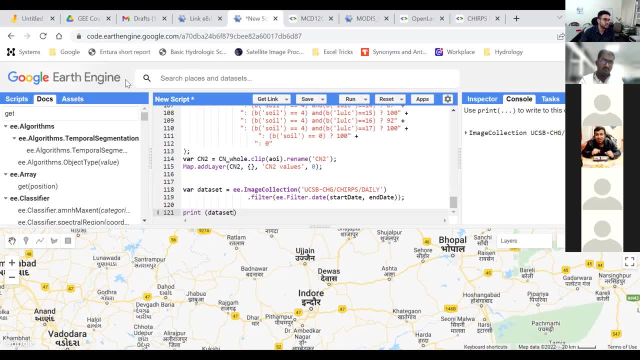 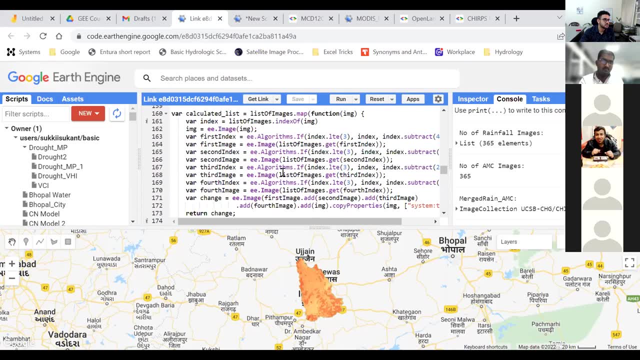 and we can apply the functions if i open the previous code, the previous code, the previous code. so after that, these are the rainfall. so after that, these are the rainfall. so after that, these are the rainfall. data, what we are going to do. data, what we are going to do. 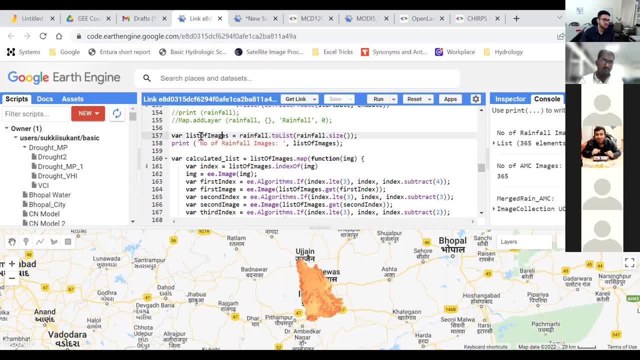 data. what we are going to do, we are going to convert the image. we are going to convert the image, we are going to convert the image collection to the list of images collection, to the list of images collection, to the list of images, because converting from image collect to 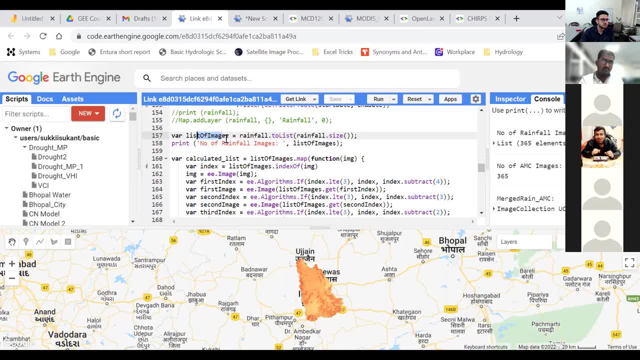 because converting from image collect to, because converting from image collect to list of images, list of images, list of images, we can actually access the previous five. we can actually access the previous five. we can actually access the previous five. day images also. day images also. day images also. and after that we have uh. 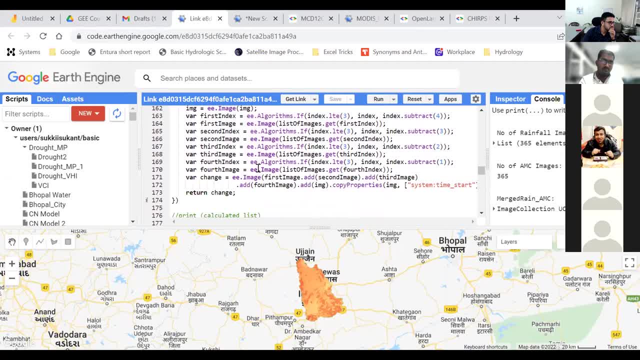 and after that we have uh, and after that we have uh. create an algorithm through which, if the create an algorithm through which, if the create an algorithm through which, if the image, that sum of that particular image, image, that sum of that particular image, image, that sum of that particular image is lesser than uh 13. 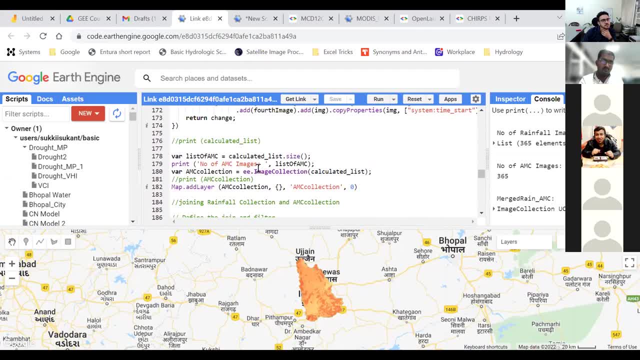 is lesser than uh 13 is lesser than uh 13. if i open this, if the letter than 13, if i open this, if the letter than 13, if i open this, if the letter than 13, then it will take amc condition 1 if it. 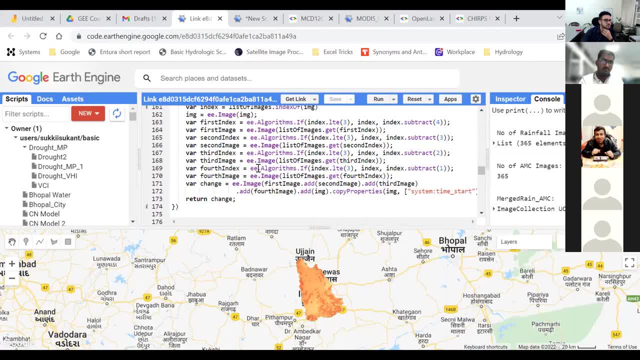 then it will take amc condition 1. if it, then it will take amc condition 1. if it is between 13 mm to 28 mm, it will take. is between 13 mm to 28 mm, it will take. is between 13 mm to 28 mm, it will take as amc condition 2. and if it is more. 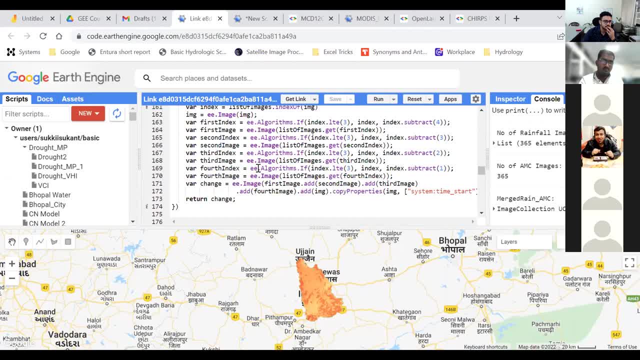 as amc condition 2 and if it is more as amc condition 2. and if it is more than 28 mm, then it will take emc. than 28 mm, then it will take emc. than 28 mm, then it will take emc condition 3 and after the 3mc condition. 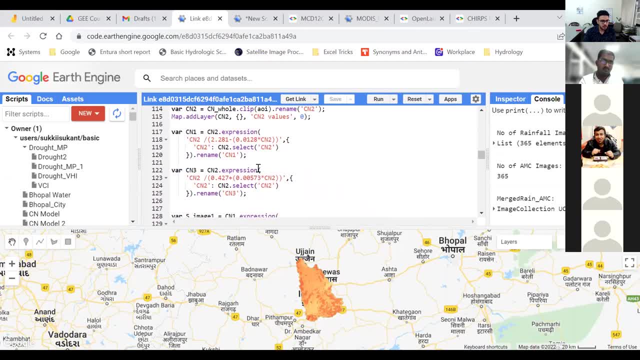 condition 3 and after the 3mc condition: condition 3 and after the 3mc condition: the, the, the. we will get the three curve number and we will get the three curve number and we will get the three curve number and the, the curve number two, and come number. 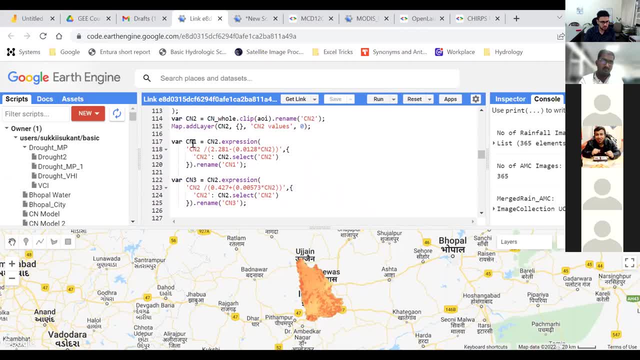 the, the curve number two and come number. the, the curve number two and come number three will be depend on the curve number three will be depend on the curve number three will be depend on the curve number. two value, two value, two value, so we have can create the curve number. 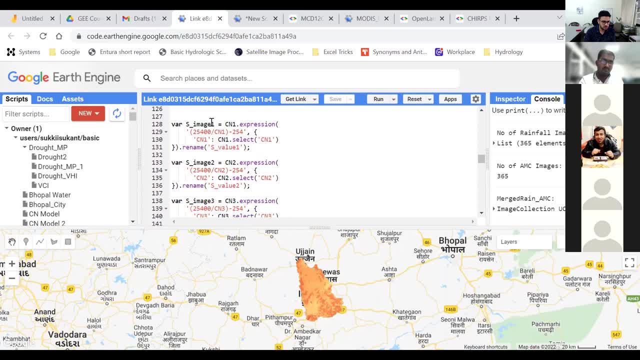 so we have can create the curve number. so we have can create the curve number one and come number three one and come number three one and come number three. and accordingly we have created s image and accordingly we have created s image and accordingly we have created s image for first come number. 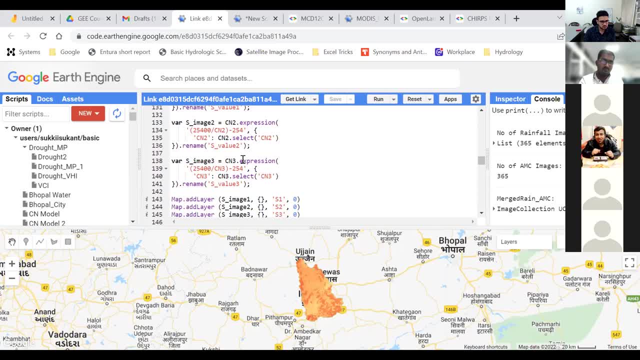 for first come number. for first come number. s image for second curve number and s s image for second curve number and s s image for second curve number and s image for third curve number. image for third curve number. image for third curve number. and. after utilizing all of this information, 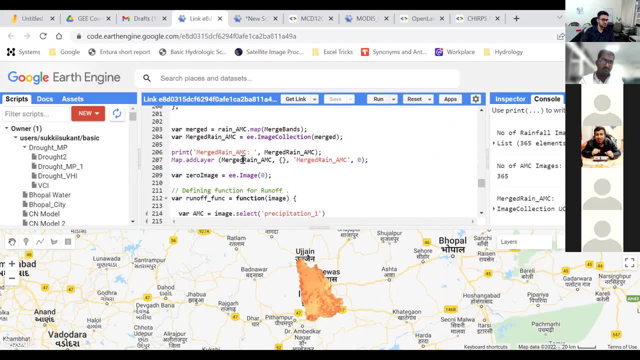 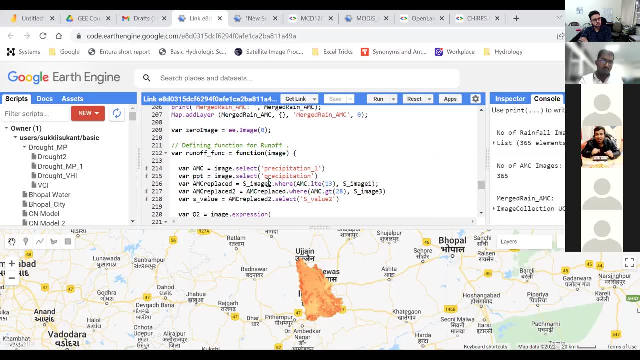 and after utilizing all of this information, and after utilizing all of this information, we have get the final runoff. that means what we have done. uh, runoff, that means what we have done. uh, runoff, that means what we have done. uh, we have defined a function that, if s, 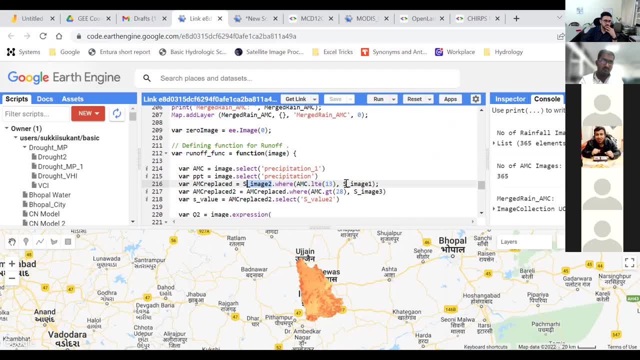 we have defined a function that if s. we have defined a function that if s. image 2: if amc is less than 13, image 2: if amc is less than 13, image 2: if amc is less than 13, then then, 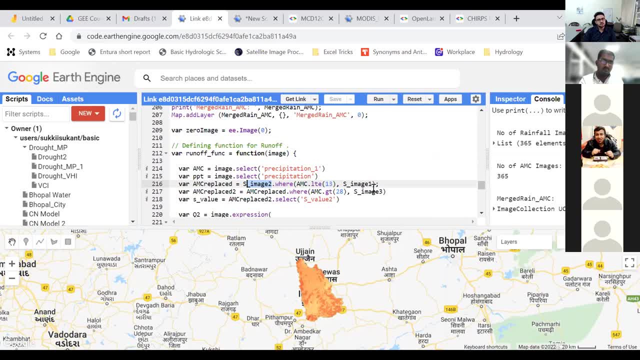 then, if it will use s image 1 and if it is, if it will use s image 1 and if it is, if it will use s image 1 and if it is greater than 28, it will utilize the s. greater than 28, it will utilize the s. 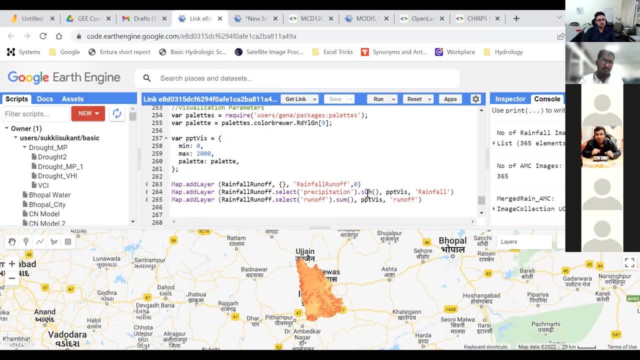 greater than 28, it will utilize the s image 3 and afterward image 3 and afterward image 3 and afterward. we have created the chart which i was. we have created the chart which i was. we have created the chart which i was telling you, telling you. 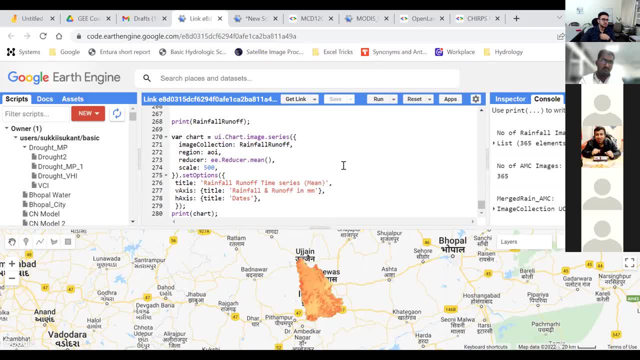 telling you: see, i'm not good in every very detail of see, i'm not good in every very detail of see, i'm not good in every very detail of this code because it will take a huge this code, because it will take a huge this code, because it will take a huge week. 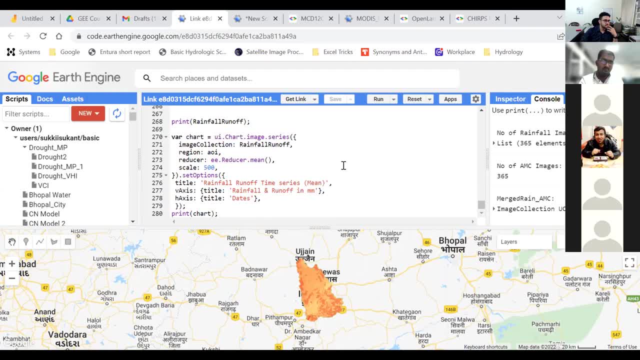 week week, a whole week in defining each and every. a whole week in defining each and every, a whole week in defining each and every. uh, what we can say what we have done, uh, what we can say what we have done, uh, what we can say what we have done, because i have taken more than 10 days to 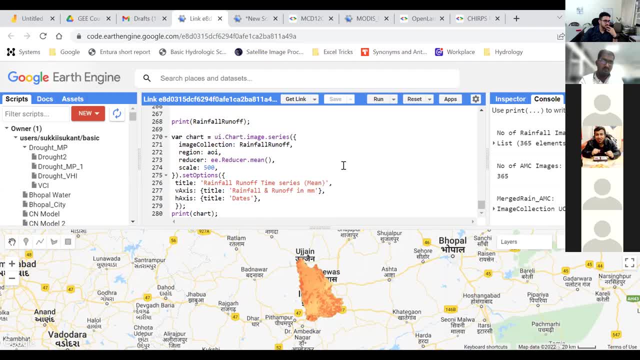 because i have taken more than 10 days to, because i have taken more than 10 days to develop so, develop so, develop so. but you can get very much insight of all, but you can get very much insight of all, but you can get very much insight of all the things that we have done here. so 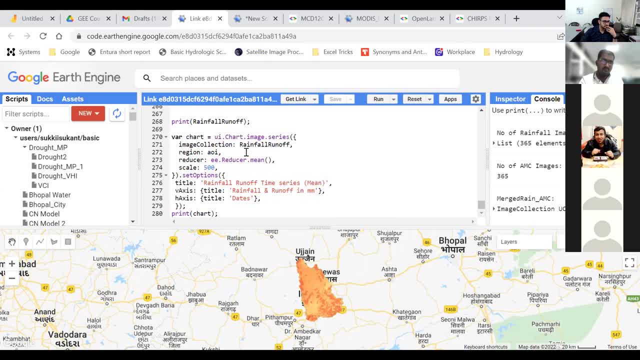 the things that we have done here. so the things that we have done here. so, after getting the image collection of, after getting the image collection of, after getting the image collection of this rainfall runoff, we have created a this rainfall runoff. we have created a this rainfall runoff. we have created a chart. 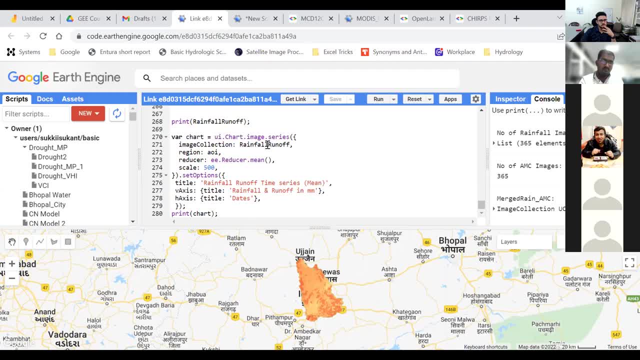 chart chart. that means which utilize uh that ui dot. that means which utilize uh that ui dot. that means which utilize uh that ui dot. chart dot image series and convert the chart dot image series. and convert the chart dot image series and convert the image collection into the spatial mean. 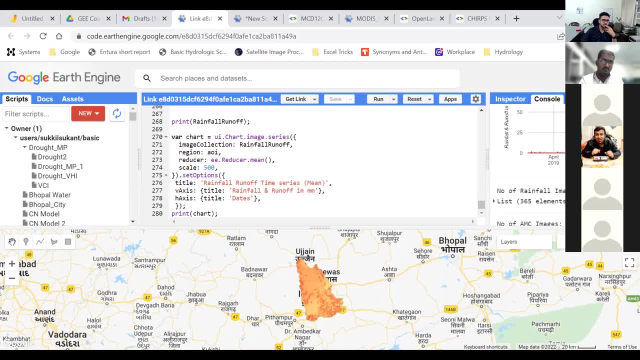 image collection into the spatial mean, image collection into the spatial mean, and provide the chart into the this, and provide the chart into the this and provide the chart into the this particular form, particular form, particular form. so so, so, as i told you that each and every detail, 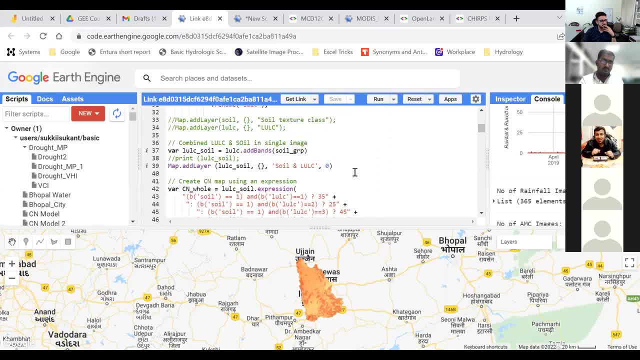 as i told you that each and every detail, as i told you that each and every detail could not be tell, but could not be tell, but could not be tell. but i'm just going to share this code with. i'm just going to share this code with. 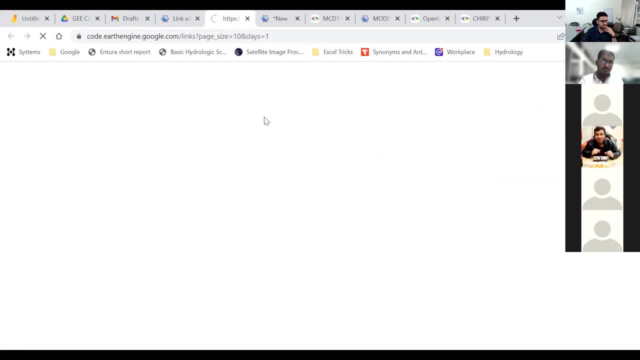 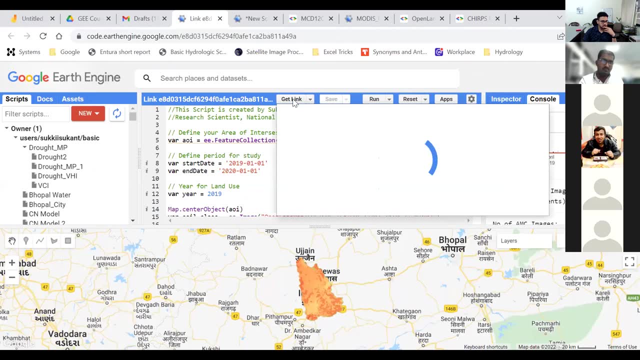 i'm just going to share this code with you, you, you, just by clicking this, uh, just by clicking this, uh, just by clicking this, uh, sorry, get link, get link, get link. copy. and i'm pasting this in the chat box: copy. and i'm pasting this in the chat box: 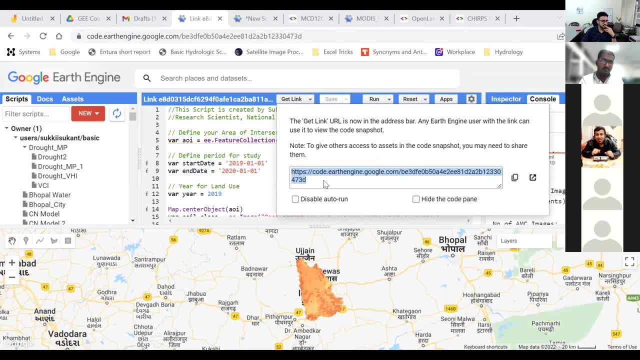 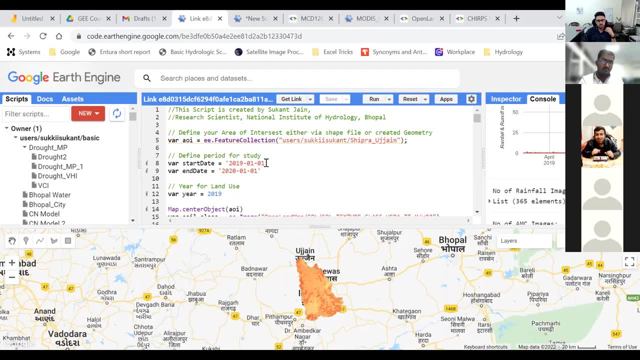 copy and i'm pasting this in the chat box so you can access this code and what you so you can access this code and what you so you can access this code and what you can do. can do. can do simply. uh, you can change your study. 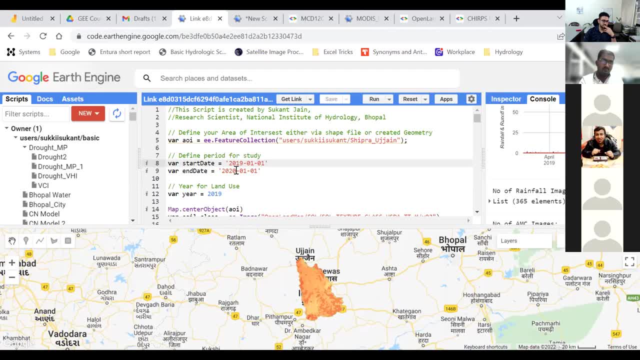 simply, uh, you can change your study. simply, uh, you can change your study period: either 2019- 2020 period, either 2019- 2020 period, either 2019- 2020, or from 2005 to 2006, but please make. or from 2005 to 2006, but please make. 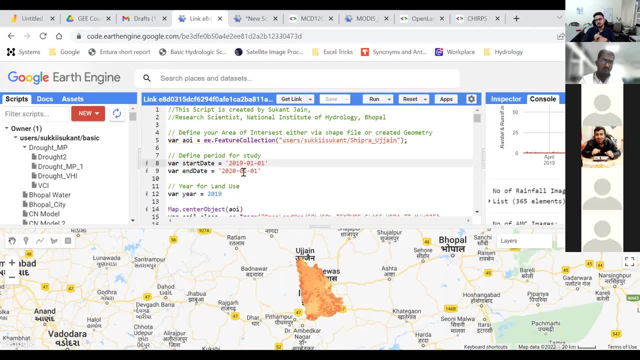 or from 2005 to 2006, but please make sure that it should not be more than two, sure that it should not be more than two, sure that it should not be more than two years, because it will years, because it will years, because it will, uh, certainly hang. that means it will. 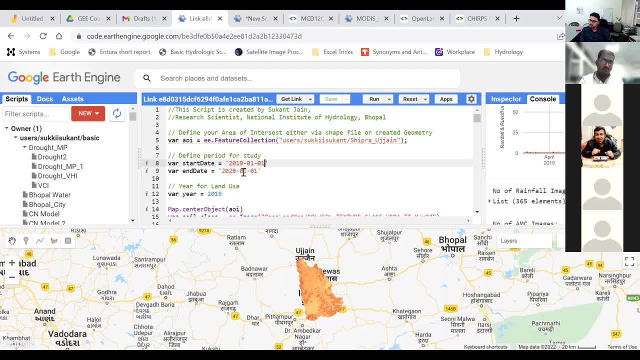 uh certainly hang. that means it will uh certainly hang. that means it will take two to three minutes or more than take two to three minutes, or more than take two to three minutes, or more than two to three minutes in two to three minutes, in two to three minutes. in generating the result, what you can do, 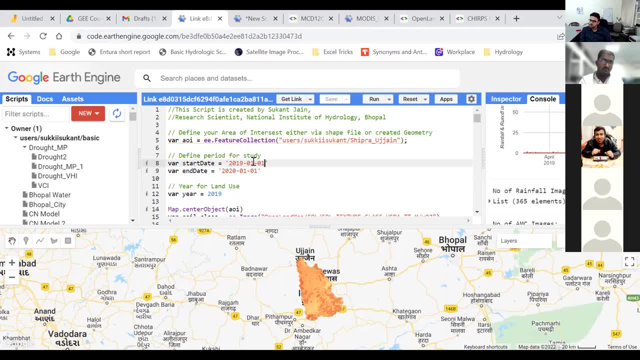 generating the result, what you can do, generating the result, what you can do. you can create two, two years. you can create two, two years. you can create two, two years. if you want to demo, if you want to demo, if you want to demo model, for 10 years you can run the model. model for 10 years. you can run the model model for 10 years. you can run the model five times for two- two years, five times for two, two years, five times for two, two years- and you can combine those data set into. and you can combine those data set into. 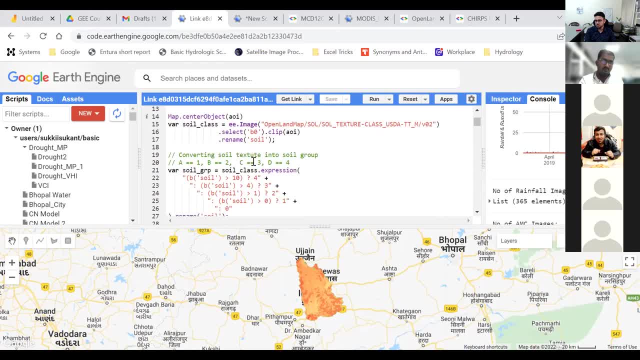 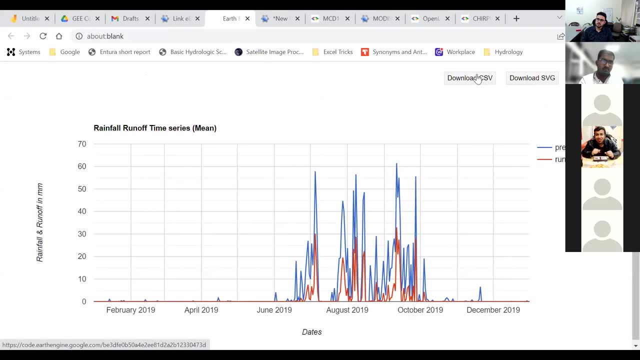 and you can combine those data set into excel or any other spreadsheet. and if i just open this into the new tab and if i just open this into the new tab, and if i just open this into the new tab and if i download the csv and if i download the csv. 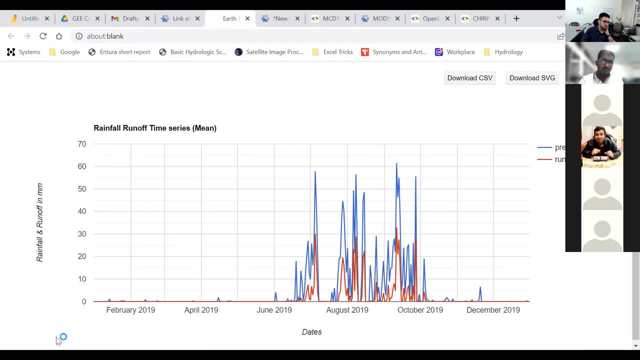 and if i download the csv and open the csv into the microsoft excel and open the csv into the microsoft excel and open the csv into the microsoft excel or in any other spreadsheet format, so we get the uh in the one column, we. so we get the uh in the one column, we. 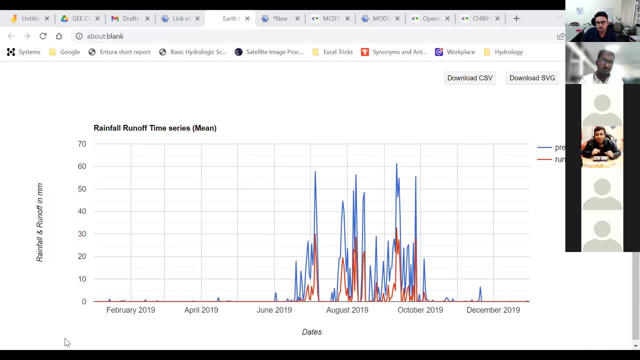 so we get the uh in the one column, we get the date, get the date, get the date in this format: january 1 2019. then we in this format: january 1 2019. then we in this format: january 1 2019. then we got the precipitation. 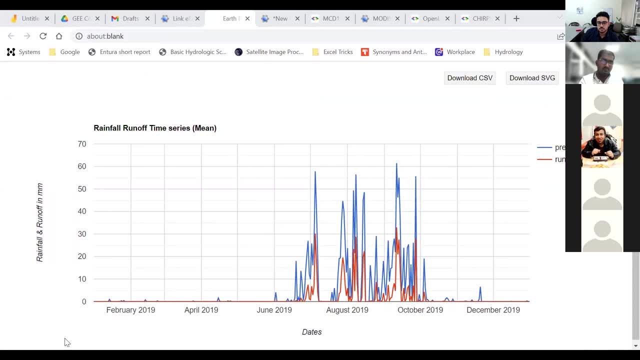 got the precipitation, got the precipitation in the mm, then we got the in the mm, then we got the in the mm, then we got the precipitation runoff in the mm and you can plot the runoff in the mm. and you can plot the runoff in the mm and you can plot the graph over here also. 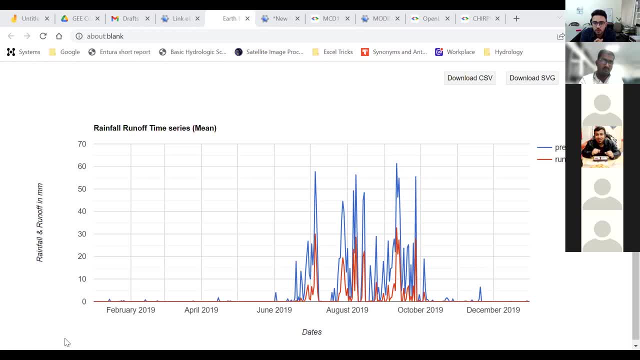 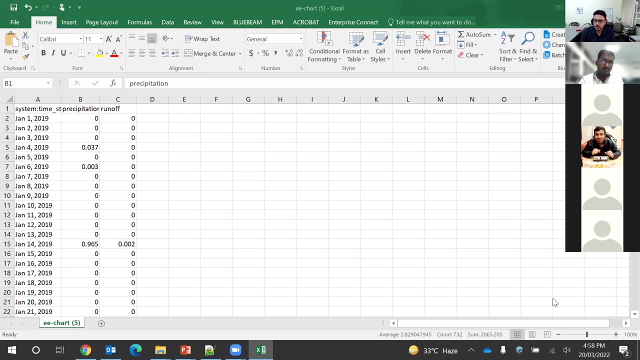 graph over here also. graph over here also, and you can. you are only sharing this and you can. you are only sharing this and you can. you are only sharing this chrome windows. okay, okay, sorry, sorry, thank you, sir. it's fine, okay, so, after opening the csv. it's fine, okay, so, after opening the csv. it's fine. okay. so after opening the csv file, you can see in the one column we file. you can see in the one column we file. you can see in the one column. we have got the date in the one column. we have got the date in the one column. we 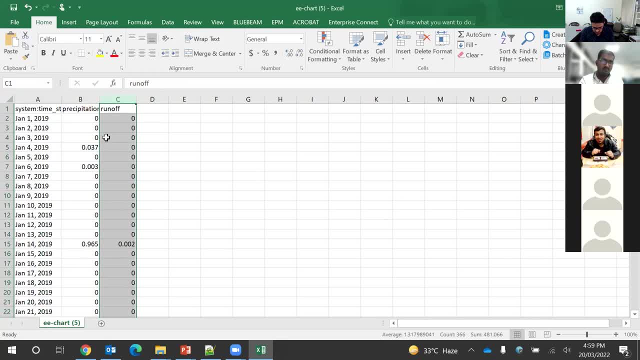 have got the date. in the one column we have got the precipitation, have got the precipitation, have got the precipitation. and in the third and in the third and in the third column we have got the rainfall. so if column we have got the rainfall, so if column we have got the rainfall. so if you download two, two years separately, 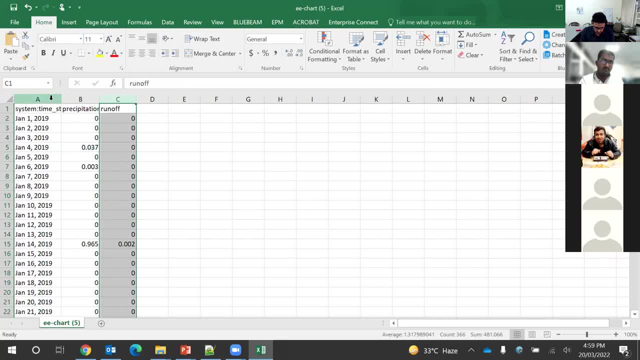 you download two two years separately. you download two two years separately. you can just combine those data site. you can just combine those data site. you can just combine those data site, either upward and downward, and you can either upward and downward, and you can either upward and downward, and you can plot the chart here also, and you can. 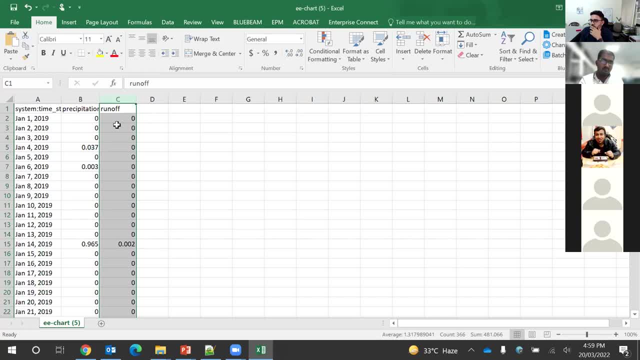 plot the chart here also. and you can plot the chart here also. and you can utilize this runoff in. some utilize this runoff. in some utilize this runoff in some other software or another modeling other software or another modeling other software or another modeling techniques to perform this, techniques to perform this. 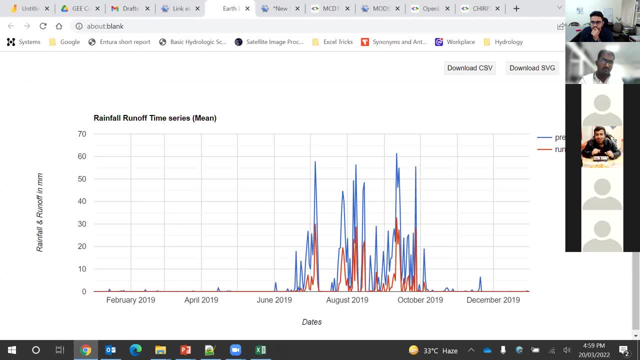 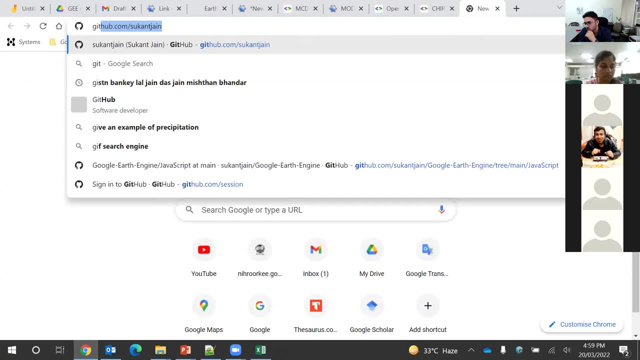 techniques to perform this calculation. so, uh, you can access this code by this link. you can access this code by this link. you can access this code by this link also. or you can access by the github also, or you can access by the github also, or you can access by the github link because it is already published. 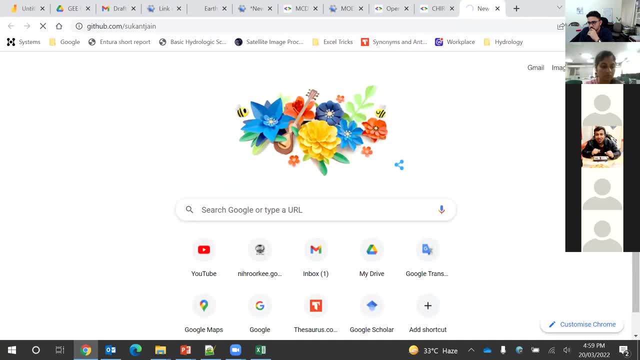 link because it is already published. link because it is already published. so if you go to the githubcom, so if you go to the githubcom, so if you go to the githubcom, uh, uh, uh, so you can get not only this, but uh, so you can get not only this, but uh. 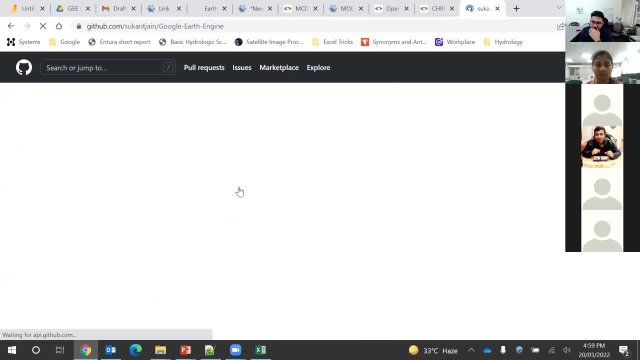 so you can get not only this but, uh, if you, if you, if you open the repository of google earth, open the repository of google earth, open the repository of google earth, engine, engine, engine. so i have put only few of the codes, so i have put only few of the codes. 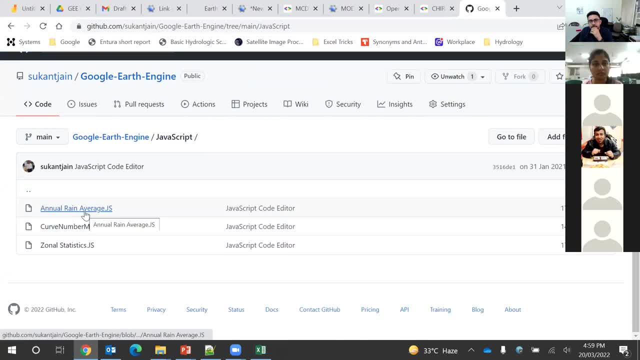 so i have put only few of the codes, like if you go to the javascript. like if you go to the javascript like actual main average. so in the ppt i like actual main average. so in the ppt i like actual main average. so in the ppt i have shown you how to get the. 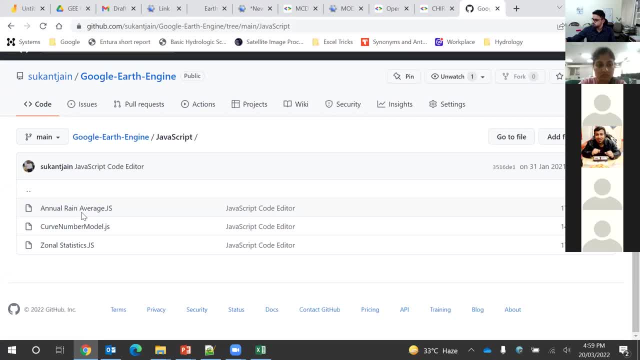 have shown you how to get the have shown you how to get the average amount of annual average average amount of annual average. average amount of annual average precipitation for whole area. you can precipitation for whole area. you can precipitation for whole area. you can open this, use this script. you can use. 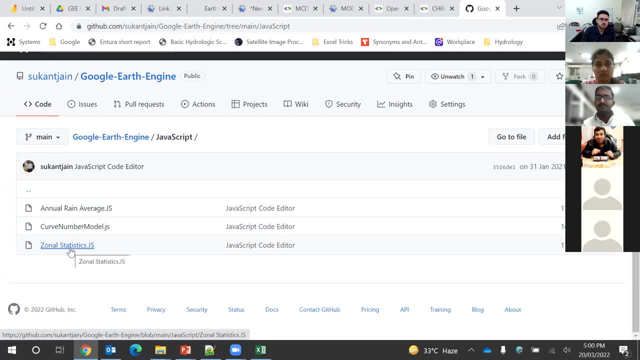 open this, use this script. you can use. open this, use this script. you can use the curve number model which i've shown, the curve number model which i've shown, the curve number model which i've shown you now, you, now, you, now. you can perform these only stats which: 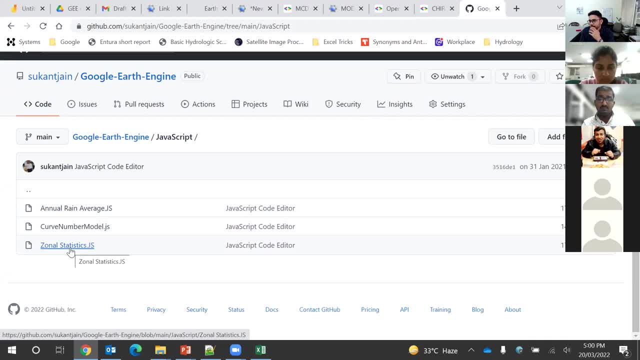 you can perform. these only stats which you can perform, these only stats which are. a participant was asking about the are. a participant was asking about the are. a participant was asking about the land use land cover chain pattern. you land use land cover chain pattern. you land use land cover chain pattern. you can use this and if you are very much, 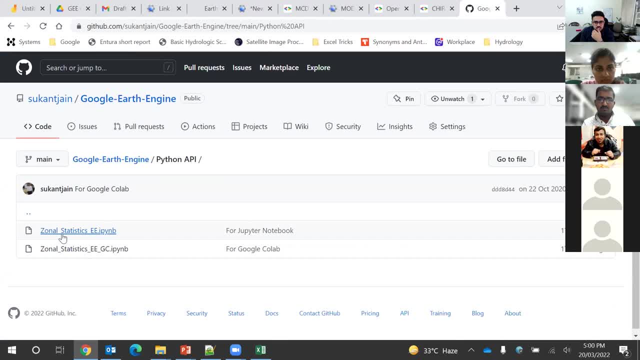 can use this and if you are very much, can use this. and if you are very much familiar with the python, you can go to familiar with the python. you can go to familiar with the python, you can go to the python api. and i have written a few. 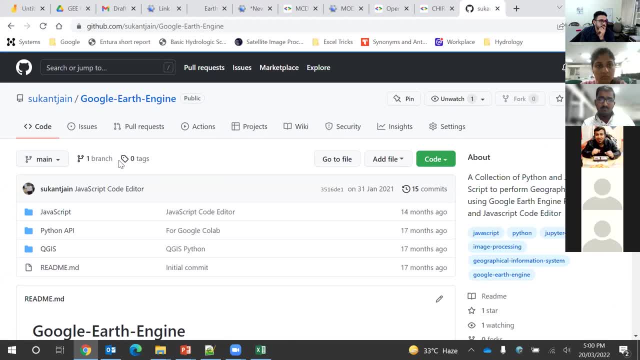 the python api and i have written a few the python api and i have written a few of these cryptos and other things of these cryptos and other things of these cryptos and other things which you can access with this also, which you can access with this also. 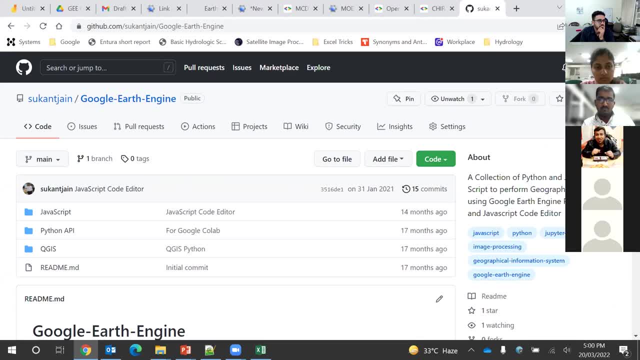 which you can access with this also, and a paper in the current science i and a paper in the current science i and a paper in the current science. i. think a link has been shared to you also. think a link has been shared to you also. think a link has been shared to you also, if not. 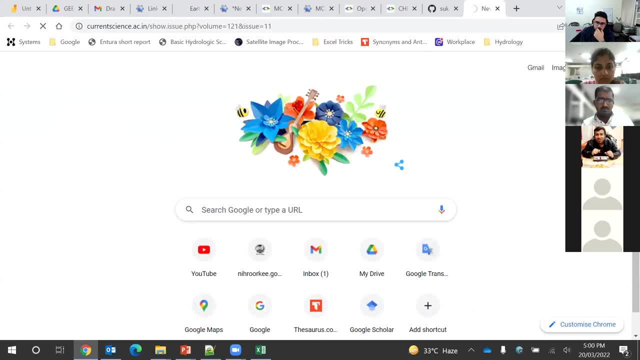 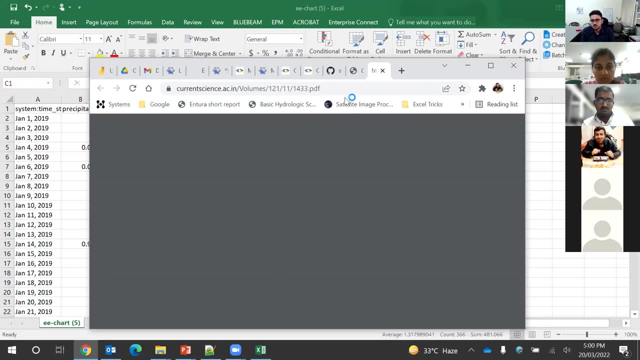 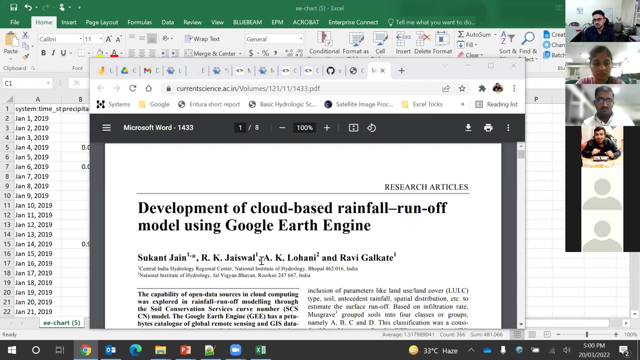 if not. if not, i will try to. so the details of this model can be so the details of this model can be. so the details of this model can be find out. you can find out in this. find out. you can find out in this. find out. you can find out in this link also. 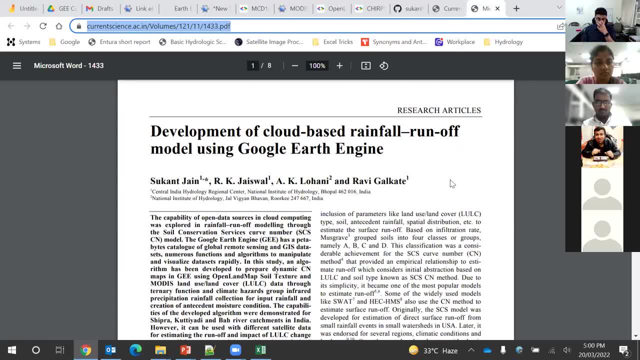 link also. link also: you can explore this and if you found any, you can explore this. and if you found any, you can explore this. and if you found any, encounter any problem or encounter any problem, or encounter any problem, or uh, it is my advice or my suggestion that 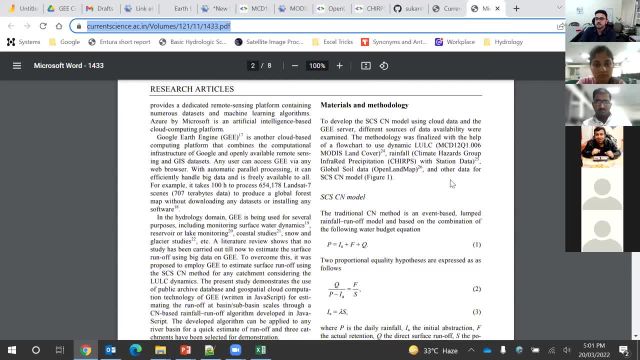 uh, it is my advice or my suggestion that, uh, it is my advice or my suggestion that, uh, you should do modeling for your own. uh, you should do modeling for your own. uh, you should do modeling for your own area and you can compare the result with area and you can compare the result with. 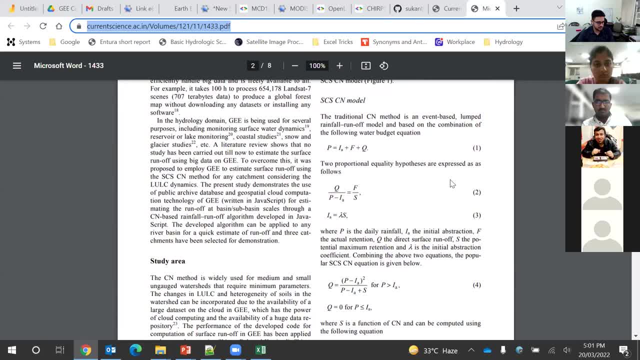 area and you can compare the result with a gnd site data site or with the compare a gnd site data site, or with the compare a gnd site data site or with the compare with archer model, because i've compared with archer model, because i've compared. 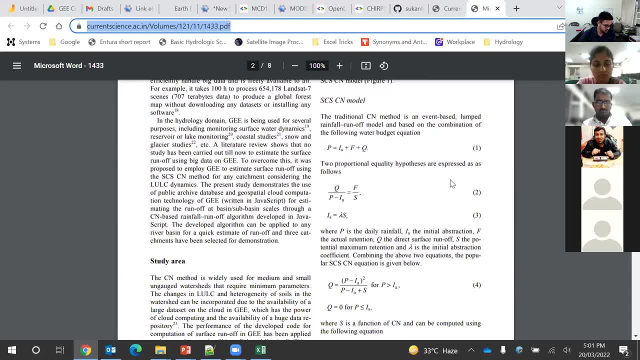 with archer model, because i've compared this model with a sort output or with a, this model with a sort output or with a, this model with a sort output or with a gnd site data, and it is giving quite good gnd site data and it is giving quite good. 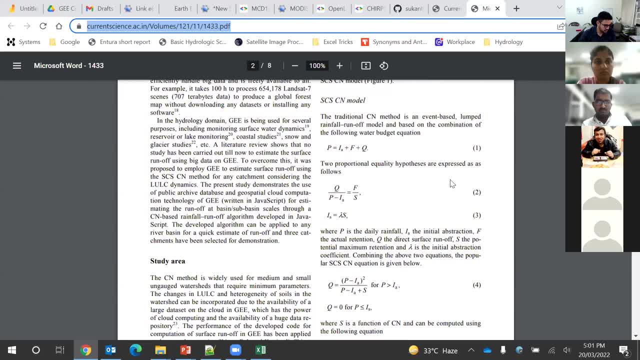 gnd site data and it is giving quite good result for the monthly, not for the daily, result for the monthly, not for the daily, result for the monthly, not for the daily, because our curve number application, because our curve number application, because our curve number application does not apply the routing techniques. so 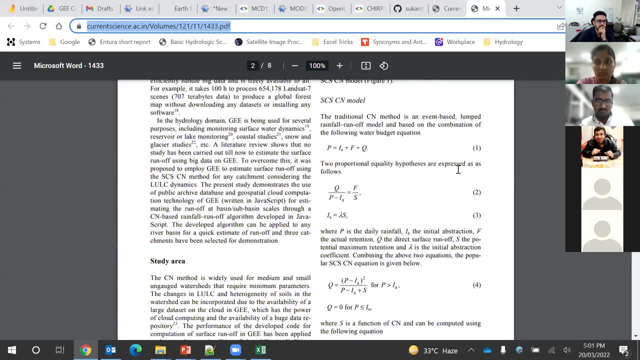 does not apply the routing techniques, so does not apply the routing techniques. so that's why, on the monthly basis on the, that's why on the monthly basis on the, that's why, on the monthly basis on the smaller watershed, it is giving the good. smaller watershed, it is giving the good. 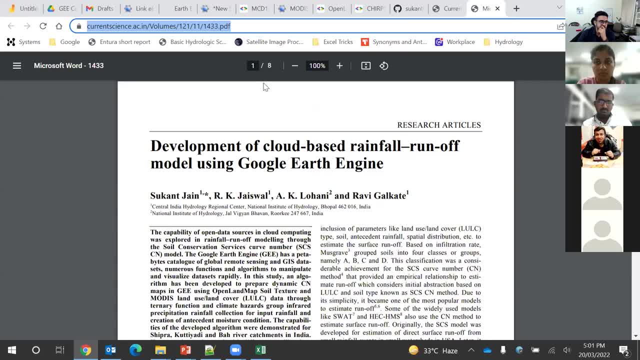 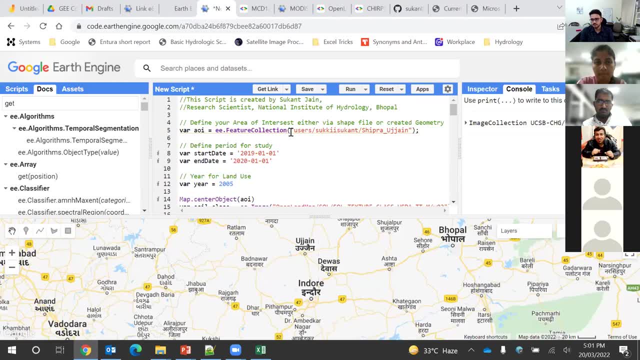 smaller watershed. it is giving the good result. so i think this is from my side, so i think this is from my side, so i think this is from my side of this whole uh, of this whole uh, of this whole uh, term number technology. so, if are any, 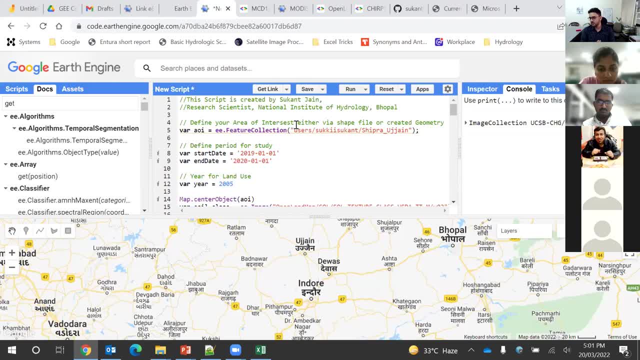 term number technology. so if are any term number technology. so if are any doubts any question, doubts any question, doubts any question. yeah, so i think we have uh two, three. yeah, so, i think we have uh two, three. yeah, so i think we have uh two, three questions that we left. there are a few. 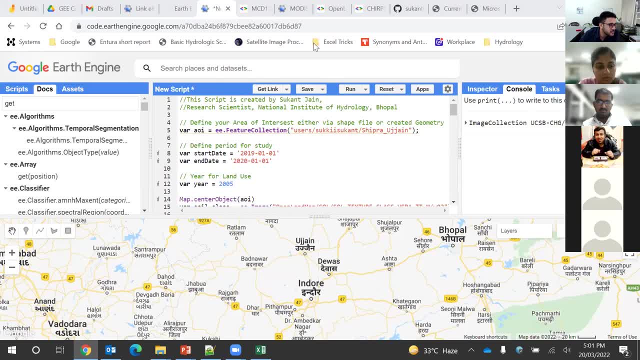 questions that we left. there are a few questions that we left. there are a few more questions coming in, more questions coming in, more questions coming in. so i'll go with the very first question. so i'll go with the very first question. so i'll go with the very first question, which was asked by ashu chaudhary. 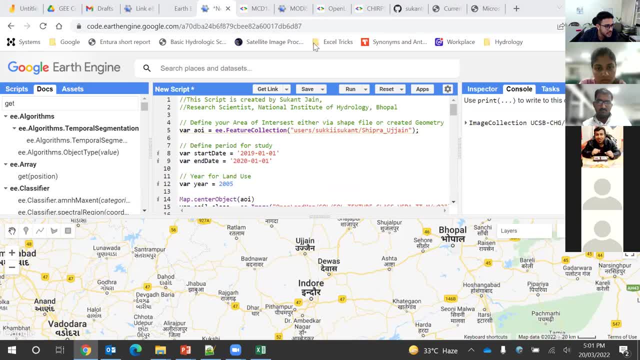 which was asked by ashu chaudhary. which was asked by ashu chaudhary. who asked that? what is the resolution? who asked that? what is the resolution? who asked that? what is the resolution? slash area pixel: we get slash area pixel. we get slash area pixel. we get the optimum information too. 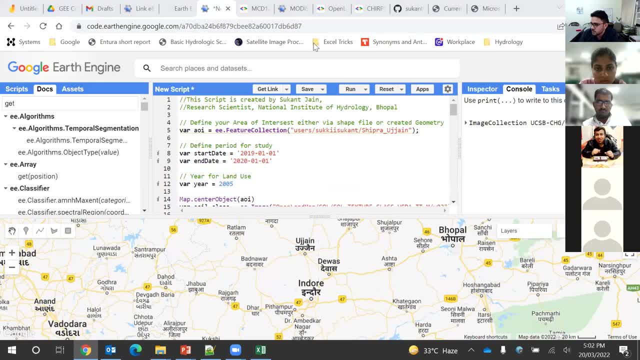 the optimum information too. the optimum information too? no, i'm not very sure what it means. no, i'm not very sure what it means. no, i'm not very sure what it means. if you can, yeah, hello um. if you can, yeah, hello um. if you can, yeah, hello um. thank you, it's very nice presentation, uh. 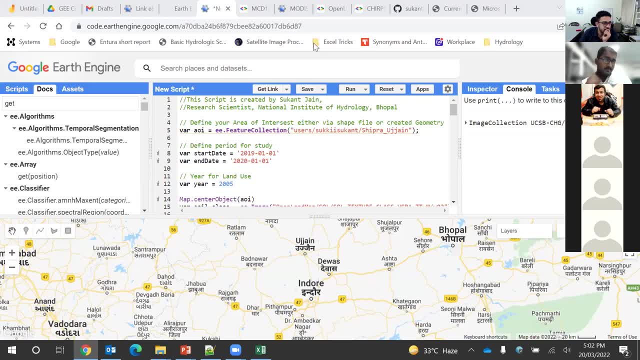 thank you, it's very nice presentation. uh, thank you, it's very nice presentation. uh, i'm actually very uh new to this field. i'm actually very uh new to this field. i'm actually very uh new to this field. but i understood, but i understood, but i understood most of the things. so my questions are: 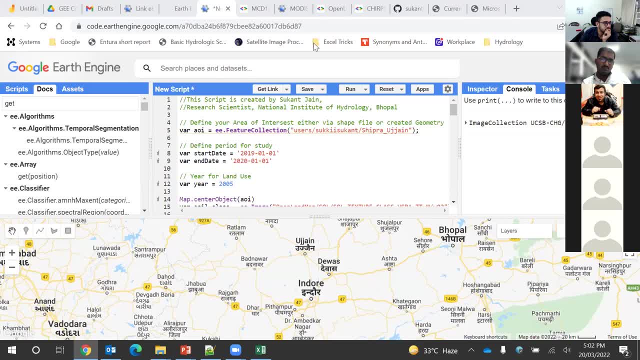 most of the things. so my questions are most of the things. so my questions are very basic. that very basic, that very basic. that when you start analyzing, you need to. when you start analyzing, you need to. when you start analyzing, you need to think about what pixel size you are. 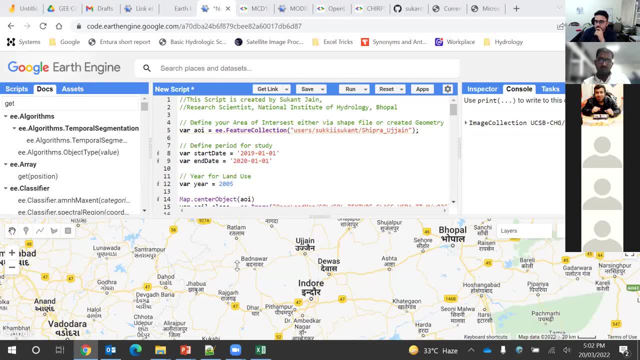 think about what pixel size you are, think about what pixel size you are targeting, targeting, targeting, so um how google earth gives us like so, um, how google earth gives us like so, um, how google earth gives us like the optimum uh information about the optimum uh information about. yeah, so please, uh, i got your question. 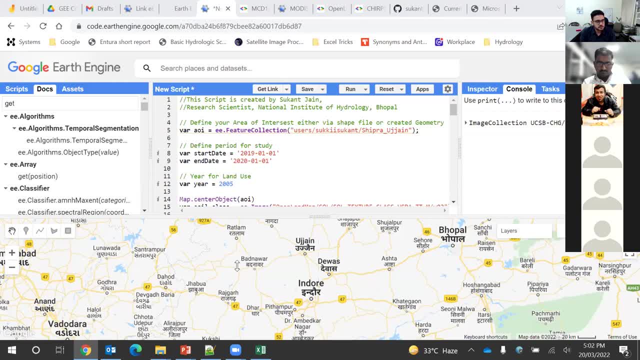 yeah, so, please, uh, i got your question. yeah, so, please, uh, i got your question. so see, as i told you that google, so see, as i told you that google, so see, as i told you that google is just a platform- okay, it doesn't- is just a platform. okay, it doesn't. 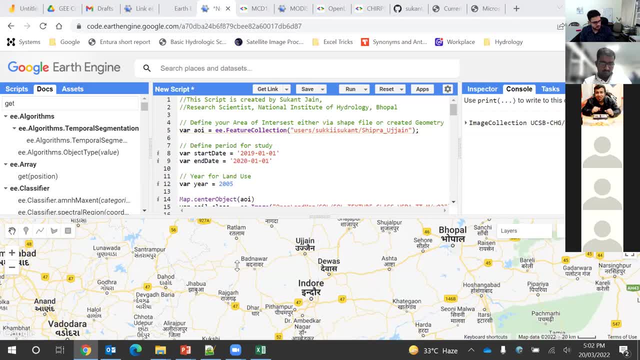 is just a platform. okay, it doesn't provide you your. provide you your. provide you your their own data set. it will provide you their own data set. it will provide you their own data set. it will provide you modest data set. it will provide you modest data set. it will provide you. 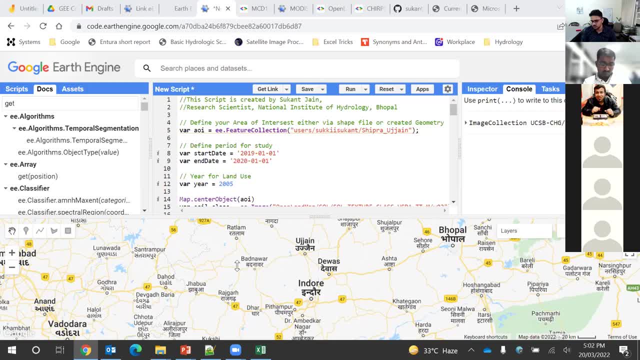 modest data set. it will provide you landsat data set. it will provide you landsat data set. it will provide you landsat data set. it will provide you sentinel data set. sentinel data set, sentinel data set. okay, so, whatever resolution: the data. okay, so, whatever resolution: the data. 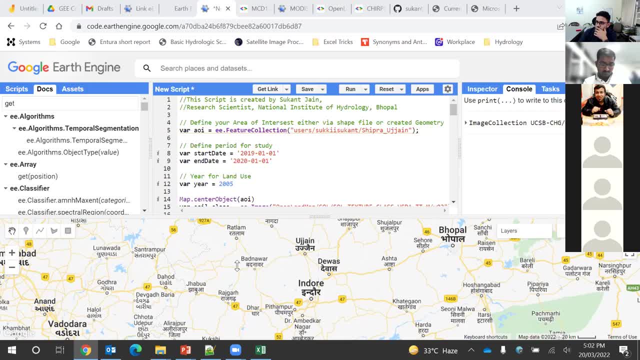 okay. so whatever resolution, the data set that we have present the free and set that we have present the free and set that we have present the free and open source sentinel data is the optimum open source sentinel data is the optimum open source sentinel data is the optimum resolution, like 10 meter resolution is. 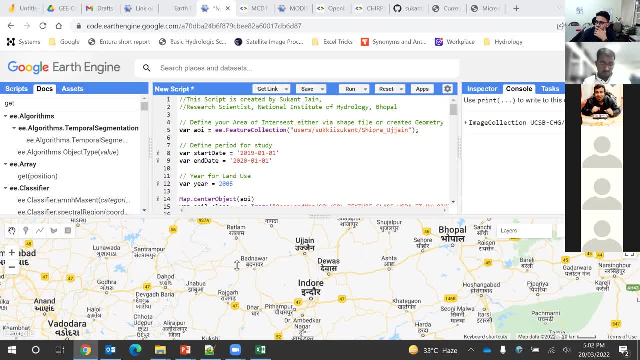 resolution like 10 meter resolution is. resolution like 10 meter resolution is here. so if you use those data set in here, so if you use those data set in here, so if you use those data set in preparing the lulc, you will get the 10. 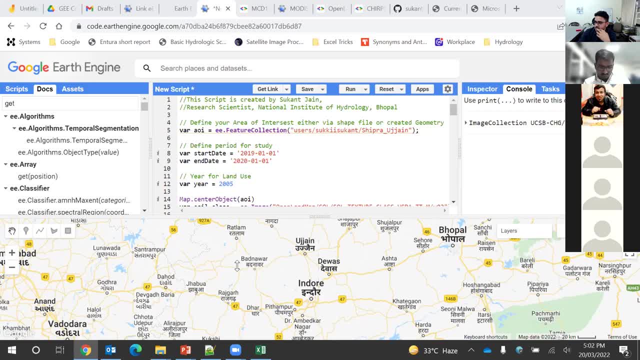 preparing the lulc, you will get the 10. preparing the lulc, you will get the 10. meter resolution result. meter resolution result. meter resolution result. but if you use the model data set which, but if you use the model data set which, but if you use the model data set which i've used in my present case, you will get. 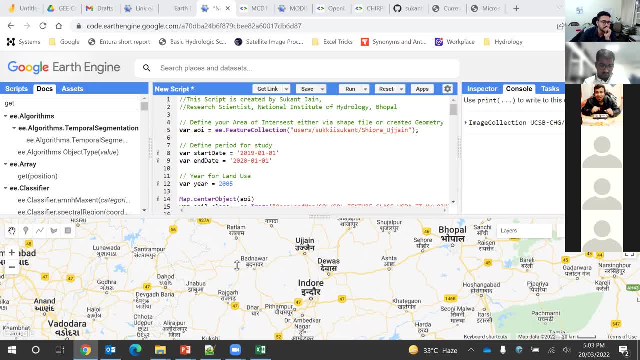 i've used in my present case, you will get. i've used in my present case, you will get the 500 meter resolution. so it is the 500 meter resolution. so it is the 500 meter resolution. so it is totally different. suppose if you have totally different, suppose if you have. 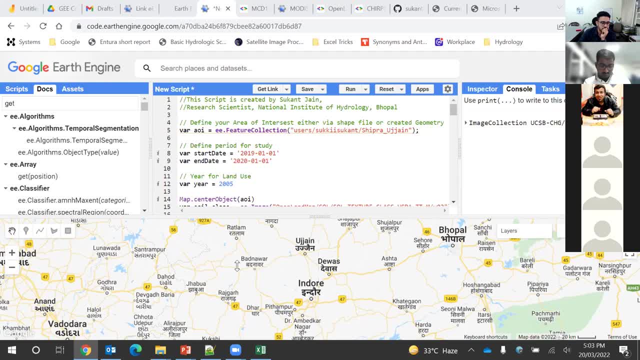 totally different. suppose, if you have your own data set of cartosite of, maybe your own data set of cartosite of, maybe your own data set of cartosite of maybe one or two meter, you can adjust your own one or two meter, you can adjust your own. 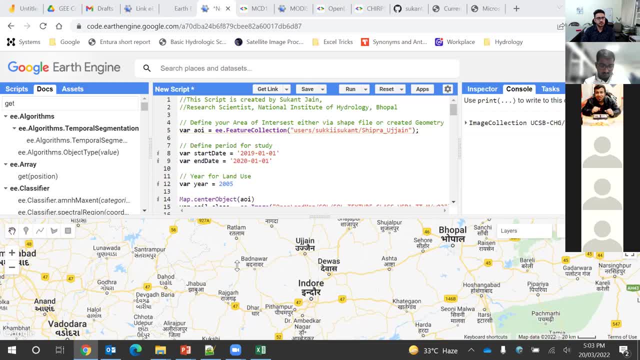 one or two meter, you can adjust your own data set into the earth engine and you data set into the earth engine and you data set into the earth engine and you apply your model there also apply your model there, also apply your model there also on the data set which we are using. so 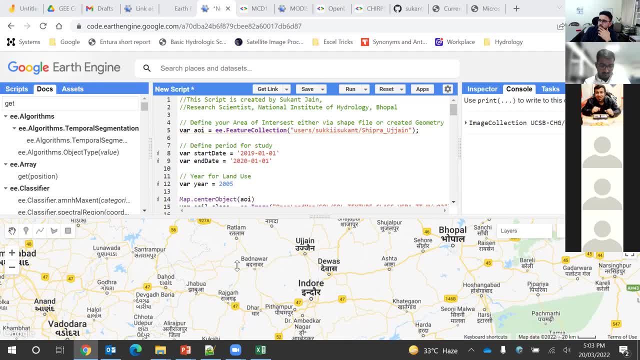 on the data set which we are using. so, on the data set which we are using. so the follow-up question is that, okay, we. the follow-up question is that, okay, we. the follow-up question is that, okay, we can club it, can club it, can club it, okay, uh. so, in order to formulate that we: 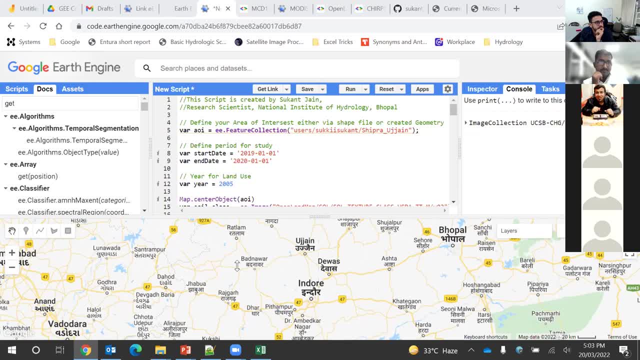 okay, uh. so in order to formulate that, we okay, uh. so in order to formulate that, we need to need to need to formulate it in the format of google earth. formulate it in the format of google earth. formulate it in the format of google earth. yes, yes, yes, yes. 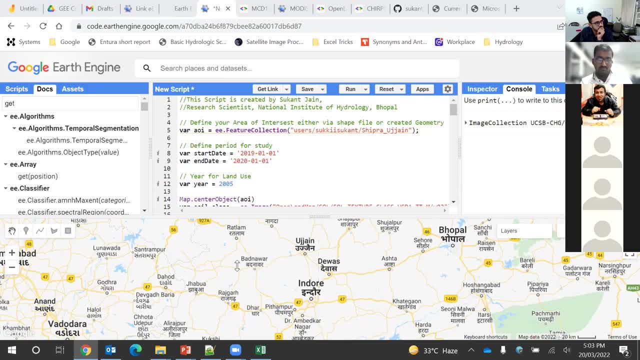 yes, yes, the google earth engine. uh supports only the google earth engine. uh supports only the google earth engine. uh supports only two data set: raster and vector. two data set: raster and vector. two data set: raster and vector. raster in the form of image collection or raster in the form of image collection, or. 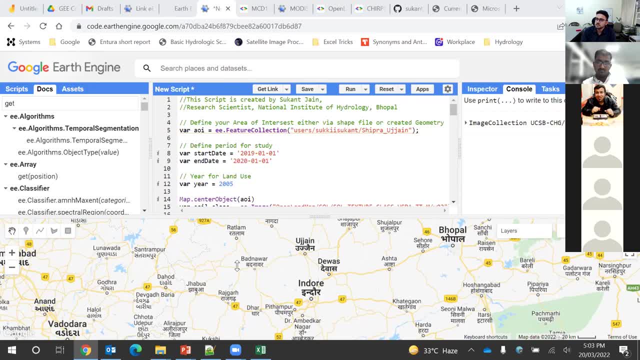 raster in the form of image collection or image image image, so you can ingest your image. either in so you can ingest your image, either in so you can ingest your image, either in the tiff format, or if the tiff format, or if the tiff format, or if images, you can create the image. 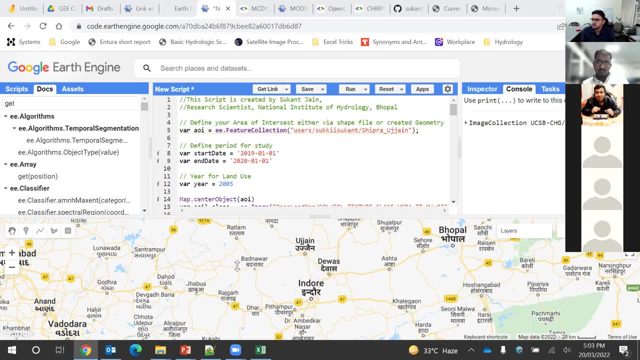 images. you can create the image images, you can create the image collection and ingest in that collection and ingest in that collection and ingest in that. so, in order to do that, do i need to? so? in order to do that, do i need to? so? in order to do that, do i need to have more information about this image? 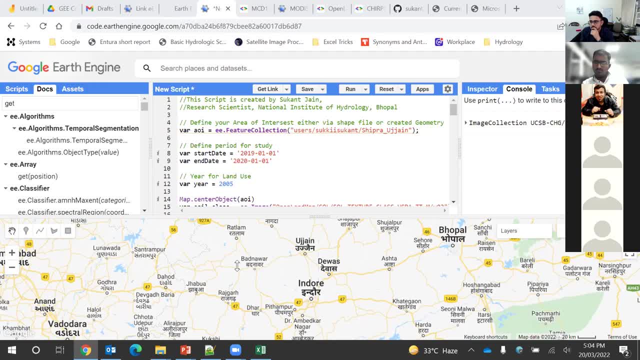 have more information about this image. have more information about this image. uh the resolution, the. uh the resolution, the. uh the resolution, the the image studies, the no, no, no, no you. the image studies, the no, no, no, no you. the image studies the no, no, no, no, you. you don't need to have very detailed. 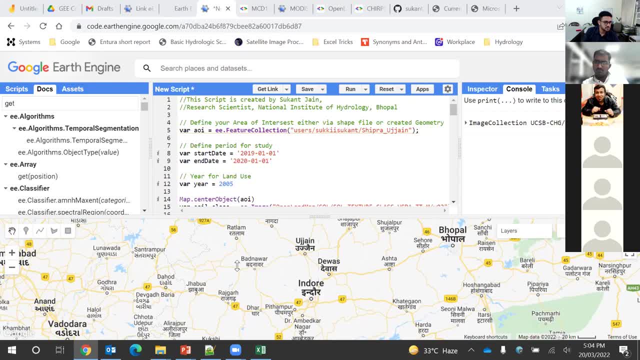 you don't need to have very detailed- you don't need to have very detailed knowledge of image classification. you knowledge of image classification, you knowledge of image classification. you just need to know about your own data, just need to know about your own data. just need to know about your own data. that's it. okay, the only thing here. you. 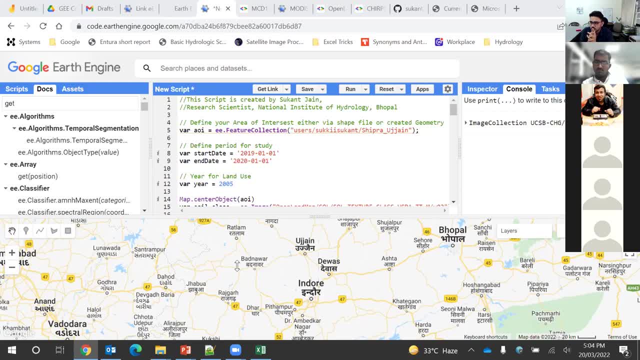 that's it okay, the only thing here. you- that's it okay, the only thing here- you- have a plant information about your own. have a plant information about your own. have a plant information about your own data data data. okay, thank you so much. thank you okay. thank you so much, thank you. 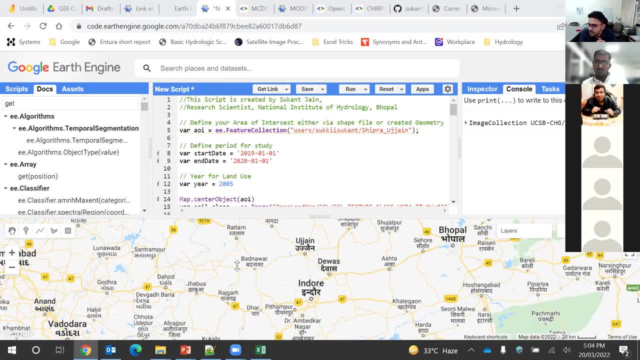 okay, thank you so much, thank you, thank you and thank you, shukant. so we'll go to thank you and thank you, shukant. so we'll go to thank you and thank you, shukant. so we'll go to the next question, which is by yes. 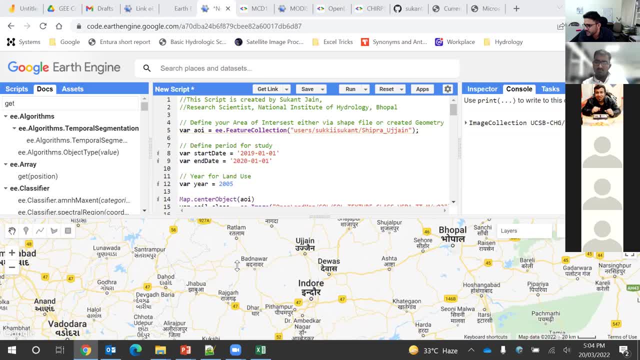 the next question which is by yes. the next question which is by yes. who is asking that? can we add our soil? who is asking that? can we add our soil? who is asking that? can we add our soil texture image as a raster file, and then texture image as a raster file, and then: 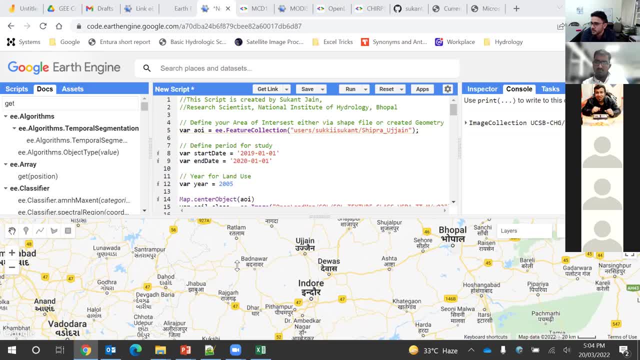 texture image as a raster file and then extract the curve number from it. is it extract the curve number from it? is it extract the curve number from it? is it possible or not possible or not possible or not? yes, you can extract uh. yes, you can extract uh. 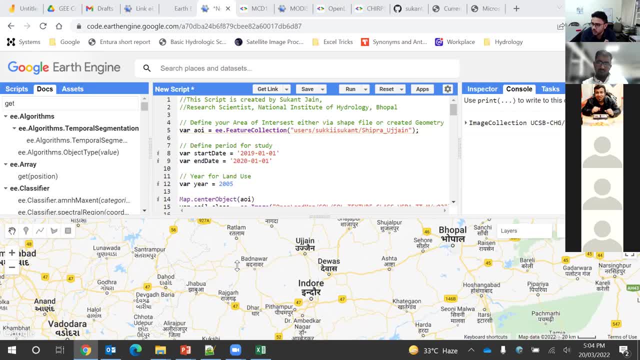 yes, you can extract. uh, you can. uh, you can. uh, you can uh. want to use their own soil texture? yes, want to use their own soil texture. yes, want to use their own soil texture. yes, you can add your own and you can convert. you can add your own and you can convert. 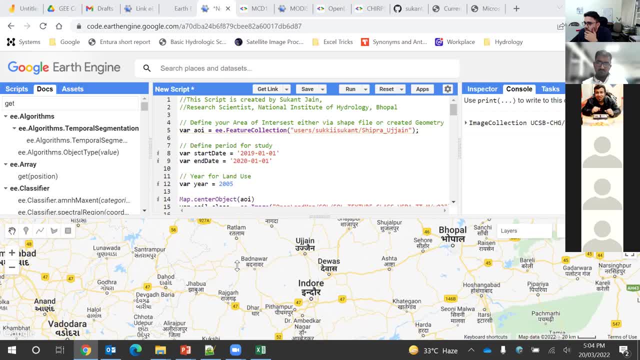 you can add your own and you can convert the curve number according to that one. so there's a question by so. there's a question by so. there's a question by nathan singh, who is asking that in the. nathan singh, who is asking that in the? 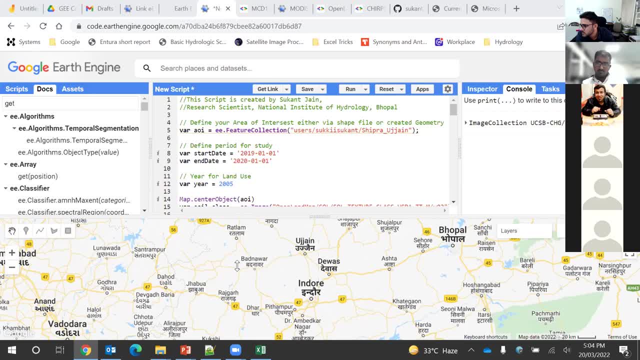 nathan singh who is asking that in the ppt you had shown the ppt, you had shown the ppt. you had shown the number of formulas for cn number. number of formulas for cn number. number of formulas for cn number. number. conversion from two to three and two. number conversion from two to three and two. number conversion from two to three and two to one to one to one. can you throw some light how these uh. can you throw some light how these uh, can you throw some light how these uh formulas were developed based on the? 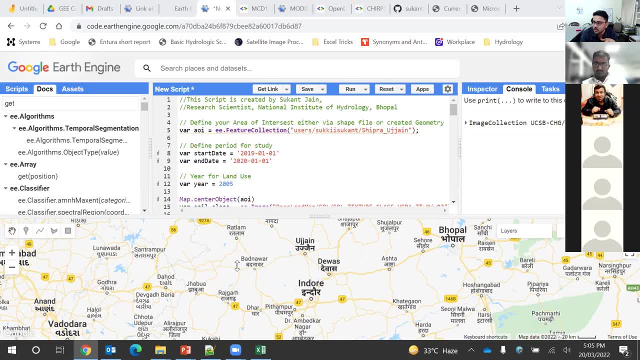 formulas were developed based on. the formulas were developed based on the intelligent moisture condition, and are intelligent moisture condition and are intelligent moisture condition, and are this formula empirical, this formula empirical, this formula empirical, uh, i think, which is very basic, uh, i think which is very basic, uh, i think which is very basic. nathan, you can find the answer to this. 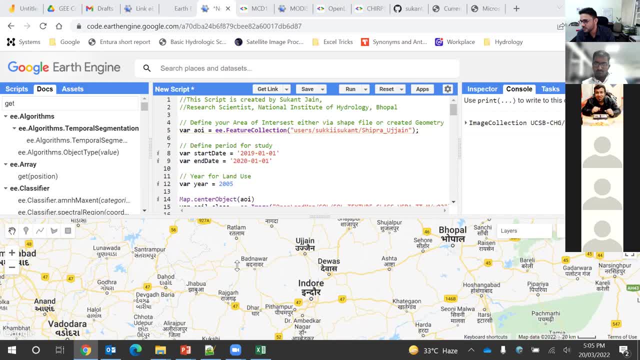 nathan. you can find the answer to this, nathan. you can find the answer to this question in any of the hydrology books. question in any of the hydrology books. question in any of the hydrology books. but still, if you want, but still, if you want. 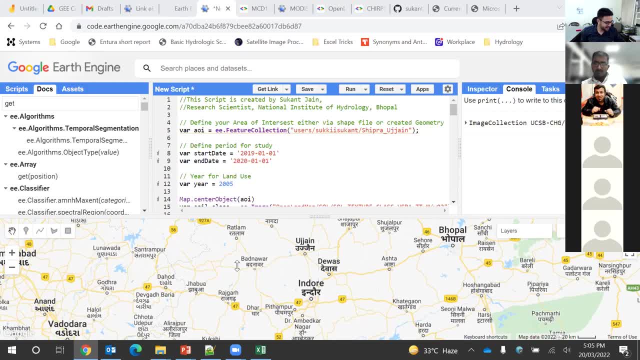 but still, if you want just yes, the just yes, the just yes, the. you have said right that it is a very. you have said right that it is a very. you have said right that it is a very basic thing. that uh basic thing, that uh basic thing, that uh, if you go to the very basic uh book of 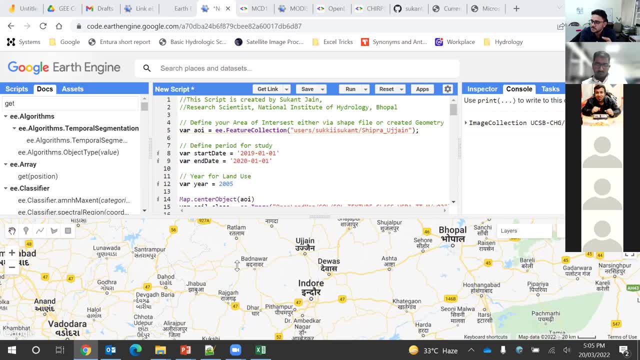 if you go to the very basic uh book of, if you go to the very basic uh book of subramanian, subramanian, subramanian, subramani, of hydrology, so they have a very of hydrology, so they have a very of hydrology. so they have a very detailed description and how the 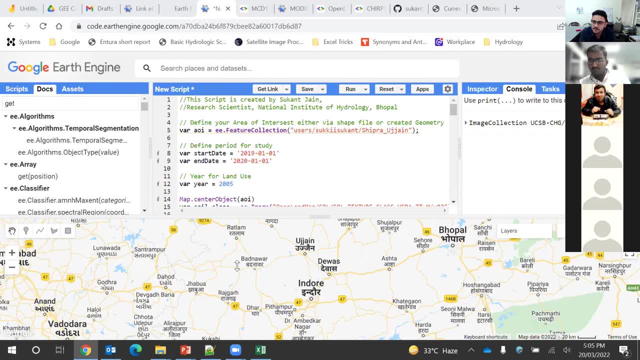 detailed description and how the detailed description and how the anti-serum moisture condition is anti-serum moisture condition, is anti-serum moisture condition is actually actually actually affecting the runoff in the current, affecting the runoff in the current, affecting the runoff in the current number method and how. 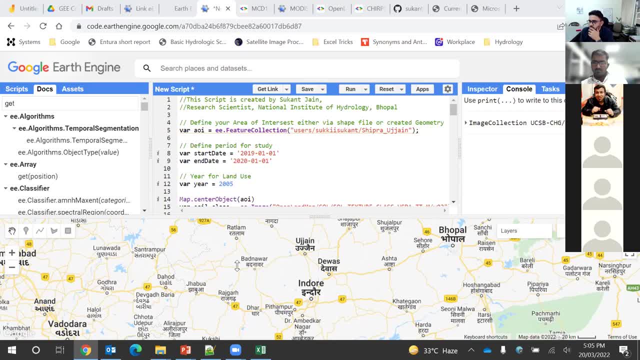 number method and how. number method and how we can use the amc condition in different. we can use the amc condition in different. we can use the amc condition in different: defining different. defining different. defining different: curve number. suppose if we have uh amc curve number. suppose if we have uh amc. 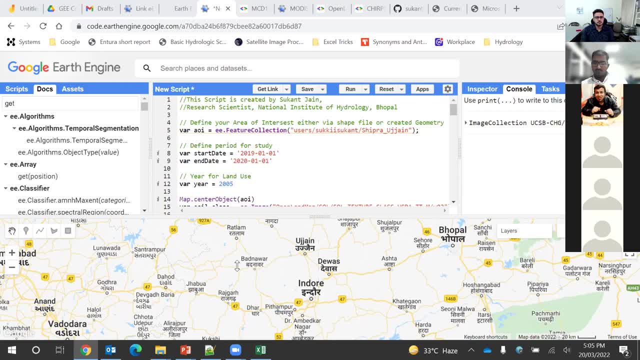 curve number. suppose if we have uh amc, very dry amc, then of course the curve very dry amc, then of course the curve very dry amc, then of course the curve number have to be on the lower side number have to be on the lower side. 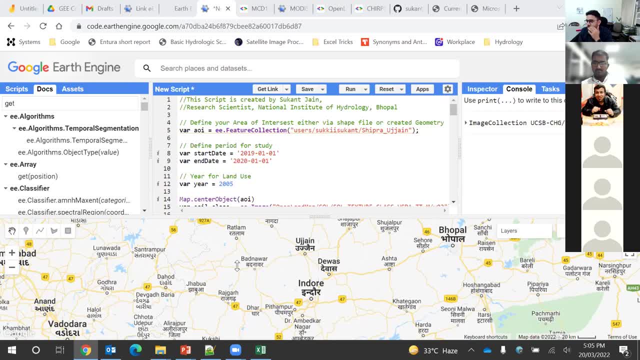 number have to be on the lower side. so so, so, on the different uh, as i've told you, the. on the different uh, as i've told you, the on the different uh, as i've told you, the ppt, that ppt, that ppt, that not only one, but different researchers. 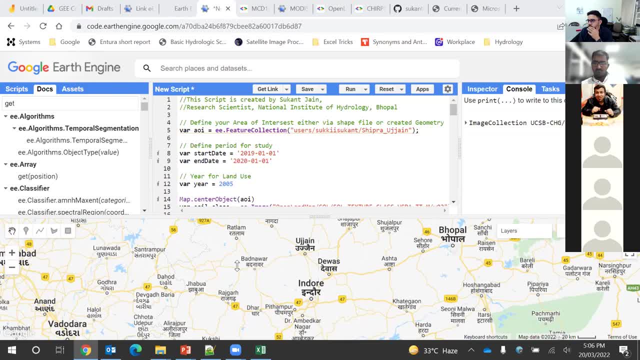 not only one, but different researchers. not only one, but different researchers have come up with the different formulas. have come up with the different formulas. have come up with the different formulas for amc one and three. so you can apply for amc one and three, so you can apply. 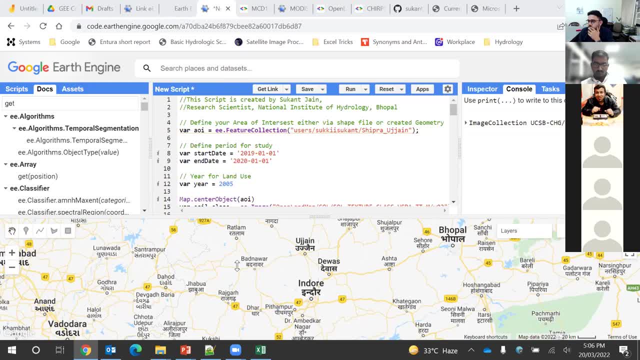 for amc one and three. so you can apply, or you can hit and trial for your own, or you can hit and trial for your own, or you can hit and trial for your own area. but the most widely used is the area. but the most widely used is the. 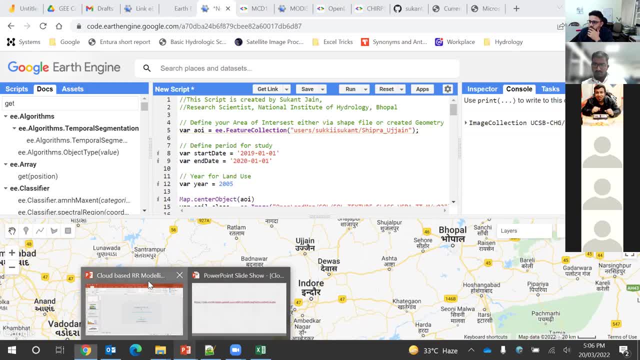 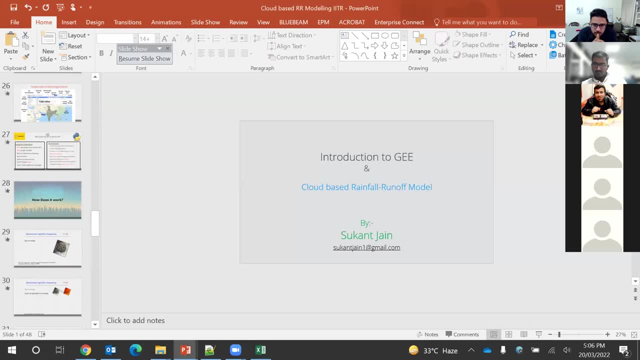 area, but the most widely used is the uh formula which has uh. i have shown you uh formula which has uh. i have shown you uh formula which has uh. i have shown you- i don't remember its name. these are basically empirical formulas. these are basically empirical formulas. 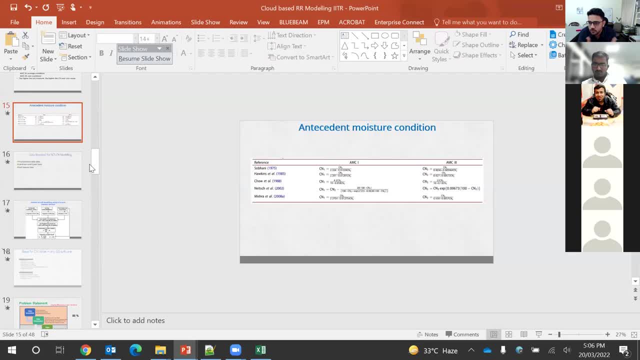 these are basically empirical formulas which are available almost in all the which are available almost in all the which are available almost in all the engineering hydrology books. so the hawkins is generally used formula. the hawkins is generally used formula. the hawkins is generally used formula which is found in the. 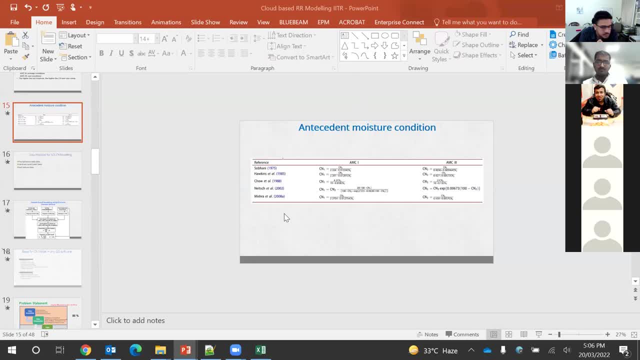 which is found in the, which is found in the my name book birth rate or other, my name book birth rate or other my name book birth rate or other related research has been developed on. a related research has been developed on. a related research has been developed on a certain. 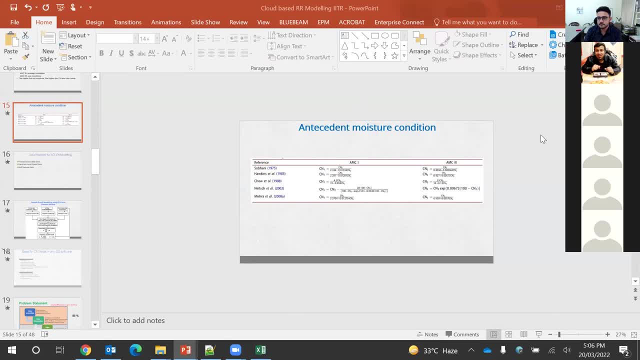 certain, certain, certain, so you can explore your own area, so you can explore your own area, so you can explore your own area: research publications and research publications, and research publications, and you can do the analysis on that area. you can do the analysis on that area. you can do the analysis on that area also. 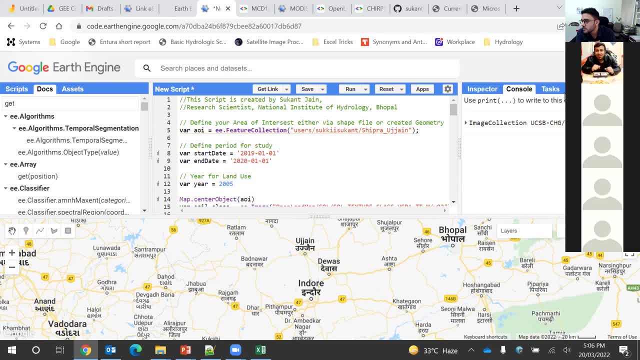 also also perfect. thank you. uh, we have an perfect thank you. uh, we have an perfect thank you. uh. we have an interesting question from pavan. who is interesting question from pavan. who is interesting question from pavan, who is asking that: how can we represent the? 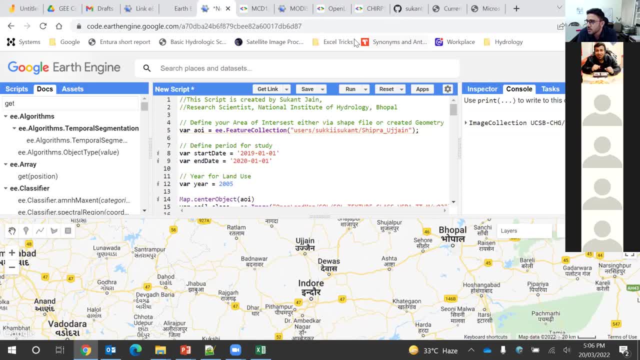 asking that? how can we represent the asking that? how can we represent the spatial change in precipitation, or lulc? spatial change in precipitation, or lulc. spatial change in precipitation, or lulc, along with the temporal change in one tip, along with the temporal change in one tip? 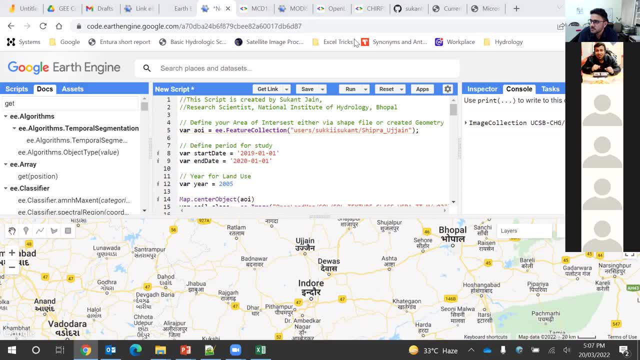 along with the temporal change in one tip file file. so we want to show temporal as well as so. we want to show temporal as well as so. we want to show temporal as well as spatial changes in either presentation, spatial changes in either presentation, spatial changes in either presentation or lulc, but in one single t file. 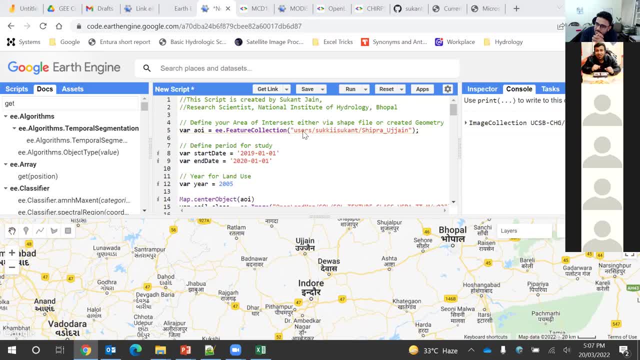 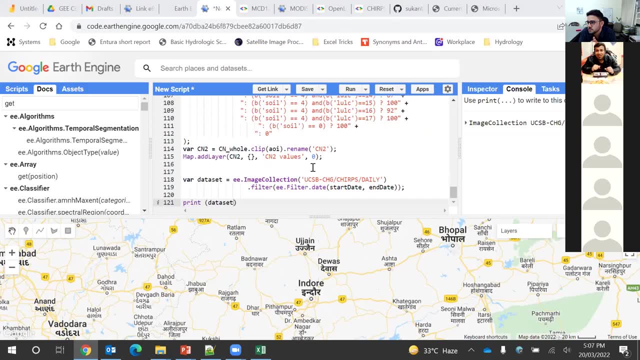 or lulc, but in one single t file, or lulc, but in one single t file. okay, so, um, okay so, um, okay, so, um, i'll just, i'll just, i'll just show you the code. so if you want to prepare a map of a, so if you want to prepare a map of a, 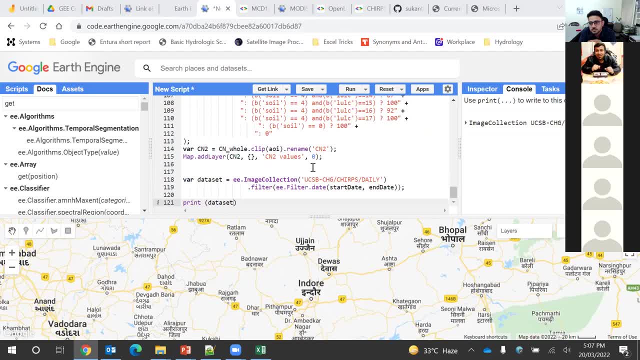 so if you want to prepare a map of a maybe precipitation, so either it has to maybe precipitation, so either it has to maybe precipitation, so either it has to be a single day precipitation or a sum of be a single day precipitation or a sum of be a single day precipitation or a sum of precipitation. 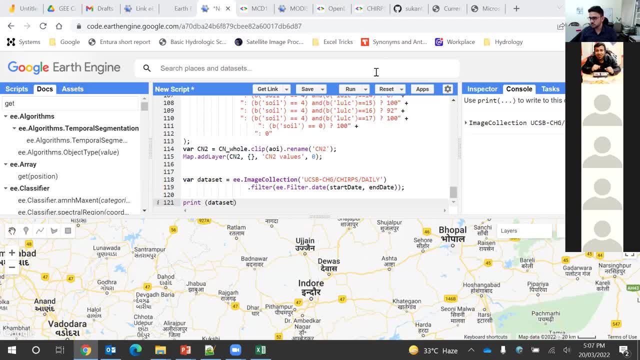 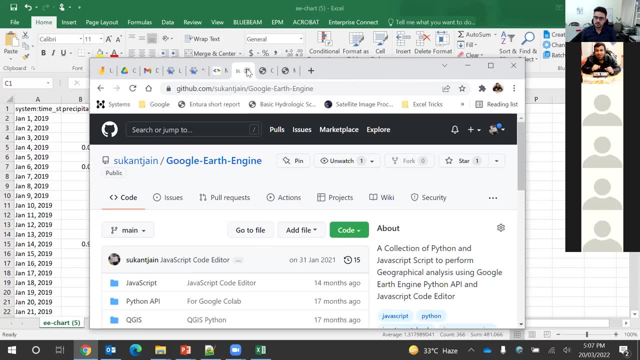 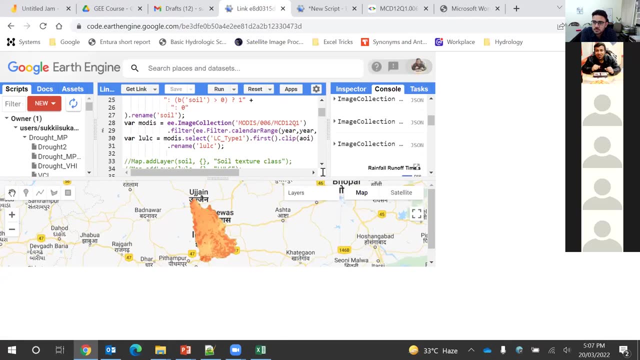 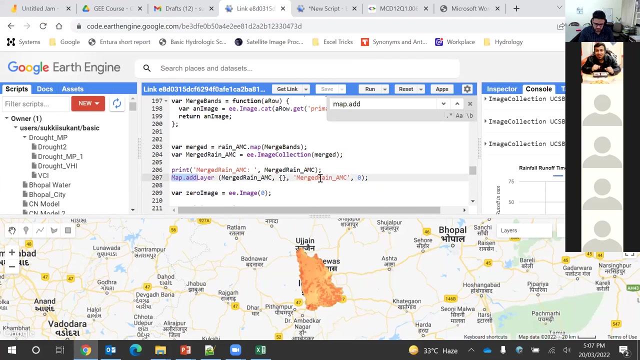 precipitation, precipitation. okay, so what you can do, i'll just now you can see that i have prepared. now you can see that i have prepared. now you can see that i have prepared. this search: okay, okay, okay. so here you can see this. we have added. so here you can see this, we have added. 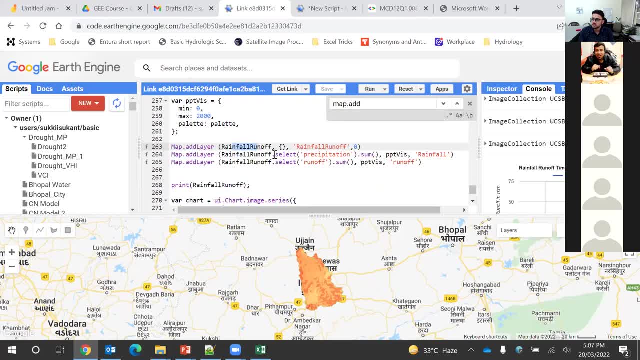 so here you can see this. we have added three maps. one is rainfall runoff. three maps: one is rainfall runoff. three maps: one is rainfall runoff, one is rainfall runoff- selecting the one is rainfall runoff, selecting the one is rainfall runoff. selecting the precipitation. and we have used the sum. 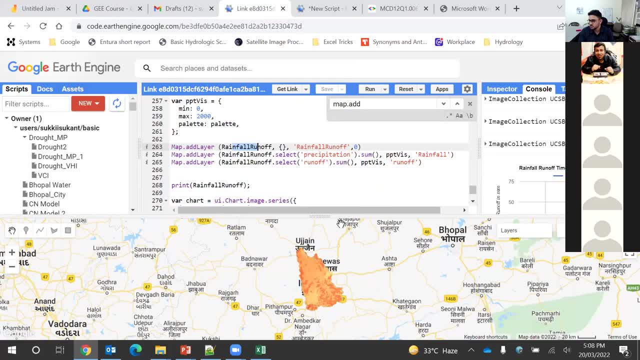 precipitation and we have used the sum. precipitation and we have used the sum. so what we are doing, we are displaying. so what we are doing, we are displaying. so what we are doing, we are displaying the map of the map, of the map, of some map. okay, so if you want to see the 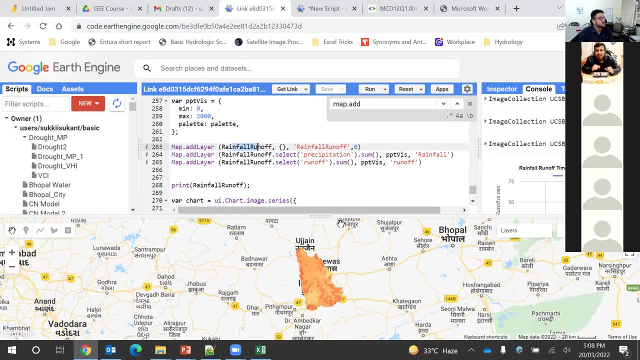 some map. okay, so if you want to see the some map, okay. so if you want to see the change, change, change in the sub map. what you can do there is in the sub map. what you can do there is in the sub map. what you can do there is an option of. 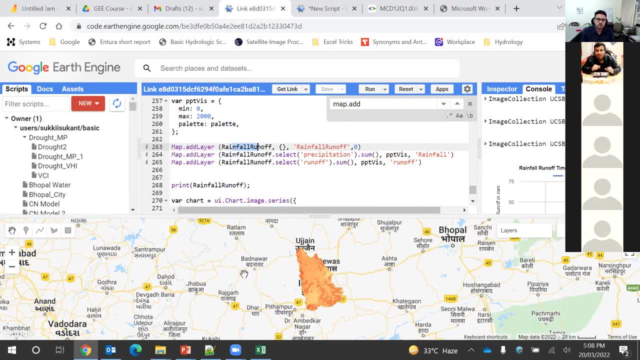 an option of an option of the slider chain. that means you can the slider chain. that means you can the slider chain. that means you can actually actually actually slide this map and see the chain, slide this map and see the chain, slide this map and see the chain detection. 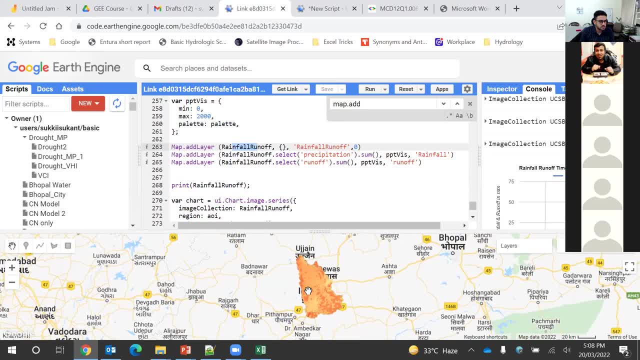 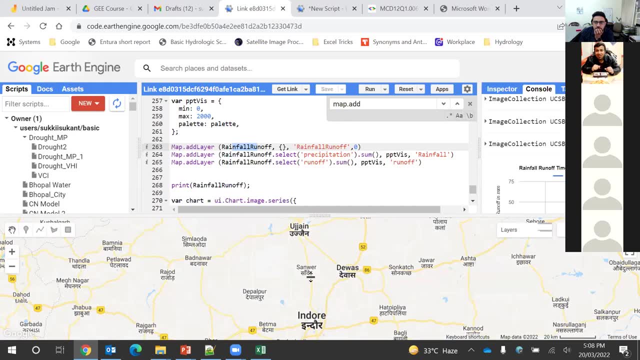 detection, detection. but it is not advisable for the runoff, but it is not advisable for the runoff, but it is not advisable for the runoff. sorry rainfall, runoff modeling. sorry rainfall, runoff modeling. sorry rainfall, runoff modeling. why? because we actually see the why. because we actually see the why, because we actually see the temporal variation. but still, if you 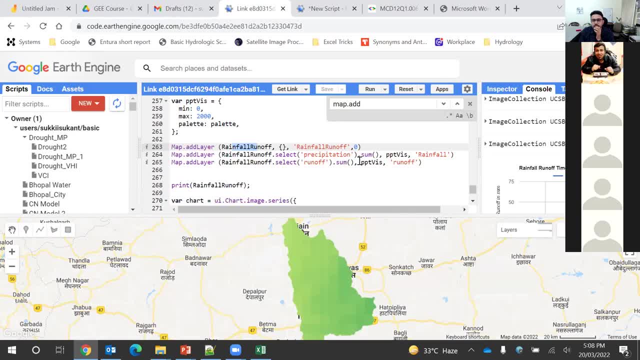 temporal variation. but still, if you temporal variation, but still, if you want to go for the spatial variation, want to go for the spatial variation, want to go for the spatial variation, what you can do, you can create your sun. what you can do, you can create your sun. 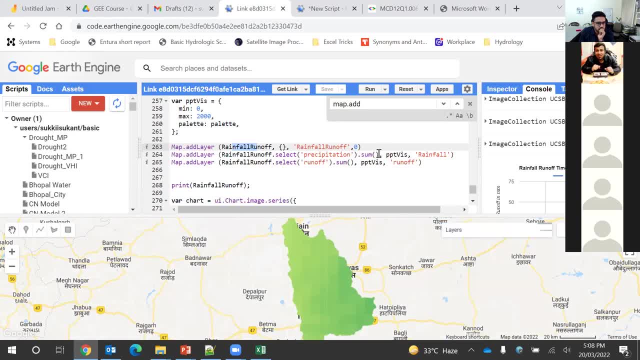 what you can create your sun map for your area and you can change the map for your area and you can change the map for your area and you can change the palettes. for example, i have used the palettes. for example, i have used the palettes. for example, i have used the palettes ppt with this one in which the 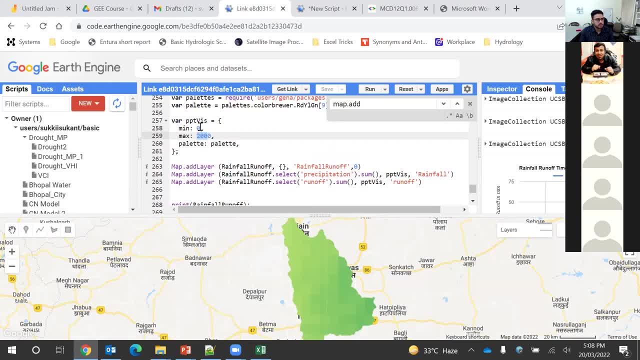 palettes ppt with this one in which the palettes ppt with this one in which the maximum value is zero and the minimum maximum value is zero and the minimum maximum value is zero and the minimum maximum value is 2000 and the minimum maximum value is 2000 and the minimum. 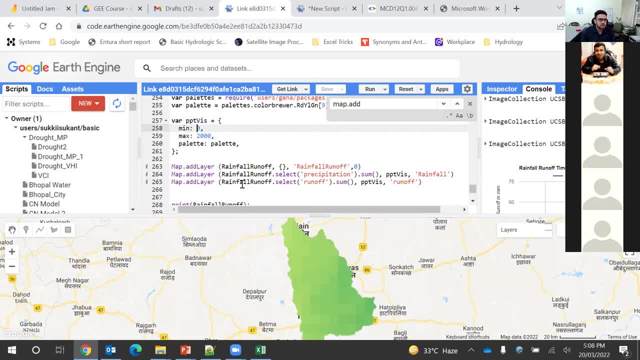 maximum value is 2000 and the minimum value is to zero. so that's why it is value is to zero. so that's why it is value is to zero, so that's why it is producing this type of wizard, producing this type of wizard, producing this type of wizard. but if i change, if i narrow down this, 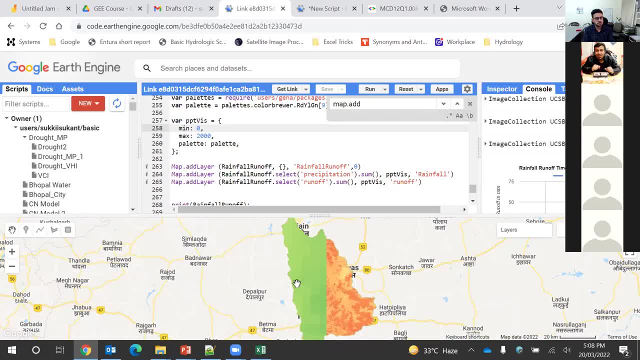 but if i change, if i narrow down this, but if i change, if i narrow down this- pixels minimum maximum- what we can do. we pixels minimum maximum, what we can do. we pixels minimum maximum, what we can do- we can analyze more effectively how the can analyze more effectively how the 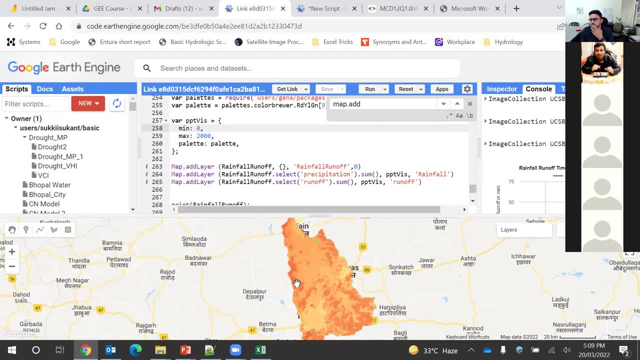 can analyze more effectively how the things are the values are changing from things. are the values are changing from things? are the values are changing from different area? or the third thing you can do, you can. or the third thing you can do, you can. or the third thing you can do, you can download this tiff file into your 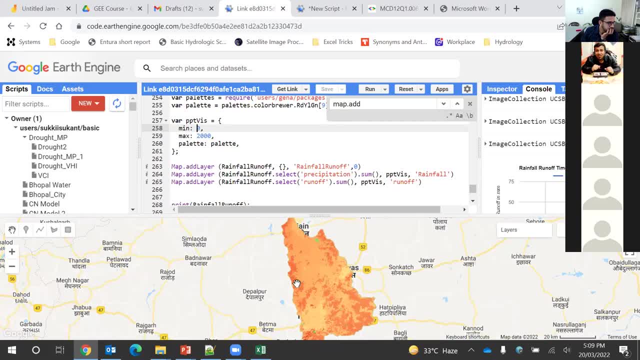 download this tiff file into your. download this tiff file into your local drive and you can always explore local drive and you can always explore local drive and you can always explore these special uh, what we can say, these special uh, what we can say, these special uh, what we can say. prepare a nice map and publish in your 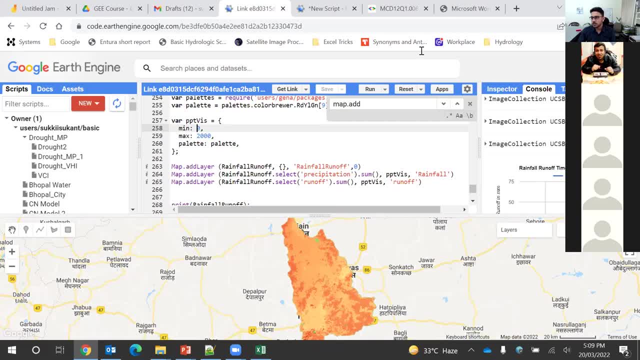 prepare a nice map and publish in your. prepare a nice map and publish in your report, or etc. i think, uh, yes, i think that was, i think that was, i think that was wonderful, wonderful, wonderful it was. i think this reminded me of one, it was. i think this reminded me of one. 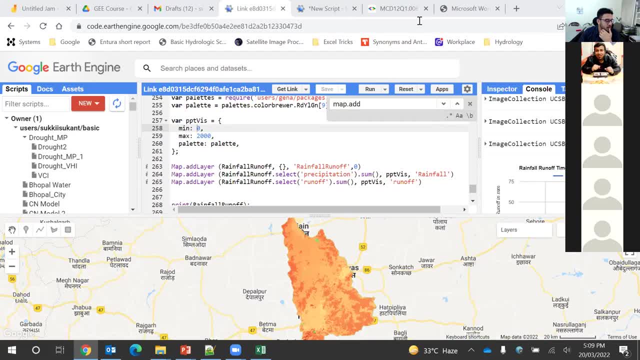 it was. i think this reminded me of one work which i did a couple of years back, work which i did a couple of years back, work which i did a couple of years back using uh google earth engine, and i'll using uh google earth engine and i'll. 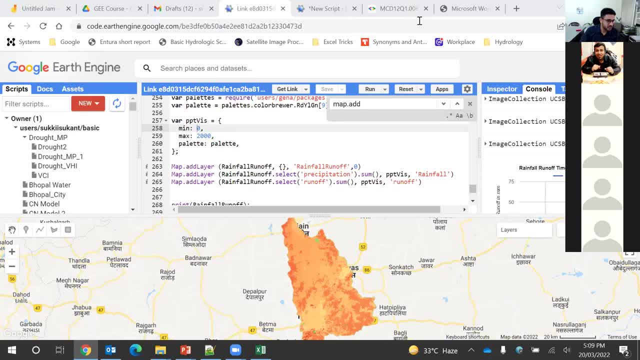 using uh google earth engine and i'll quickly share it with the participants, quickly share it with the participants, quickly share it with the participants so that, so that, so that they can uh see what there are different, they can uh see what there are different, they can uh see what there are different things that we can. google earth engine. 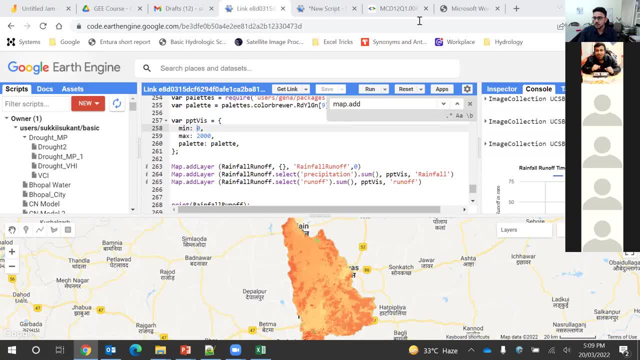 things that we can google earth engine. things that we can google earth engine. let me quickly share my screen. let me quickly share my screen. let me quickly share my screen. so this will stop your screen. so just so, this will stop your screen. so just so, this will stop your screen. so just give me a minute, okay, okay, no problem. 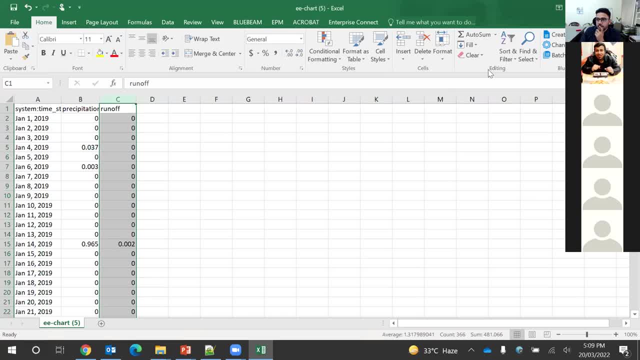 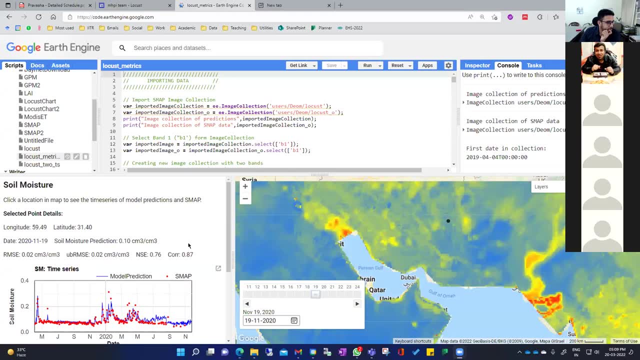 give me a minute, okay, okay, no problem. give me a minute, okay, okay, no problem, okay. so this is so, this is so. this is right, right, right. i hope you can see my screen right. i hope you can see my screen right. i hope you can see my screen right. so google earth engine also allows you to. 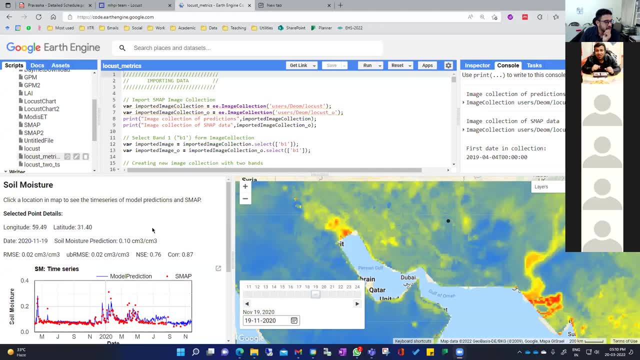 so google earth engine also allows you to. so google earth engine also allows you to make something called apps. they call it make something called apps. they call it make something called apps. they call it earth engine apps- earth engine apps, which can be integrated in any website. which can be integrated in any website. 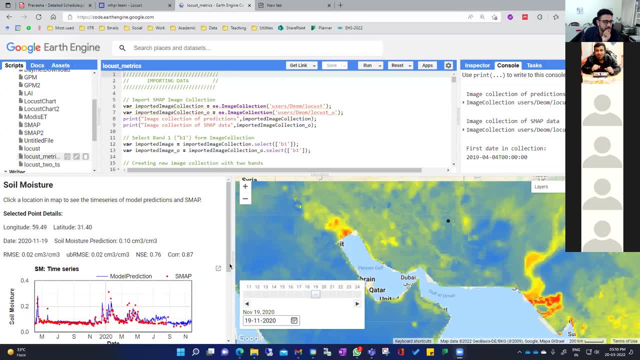 which can be integrated in any website or with any of the, or with any of the or with any of the different tools: online tools, which are different tools. online tools, which are different tools. online tools which are available and their available and their available and their sliders. that shukant was just talking. 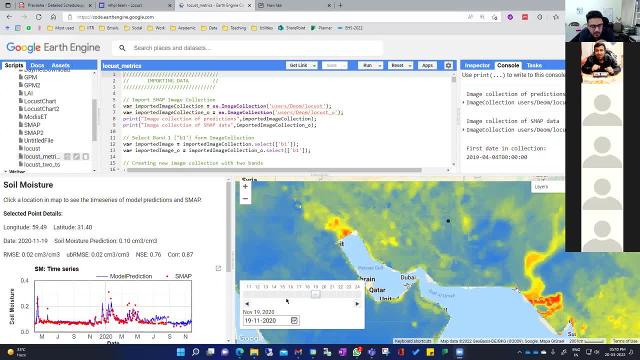 sliders that shukant was just talking, sliders that shukant was just talking about that. we can add these sliders about that. we can add these sliders about that. we can add these sliders wherein we can change the dates we can, wherein we can change the dates we can. 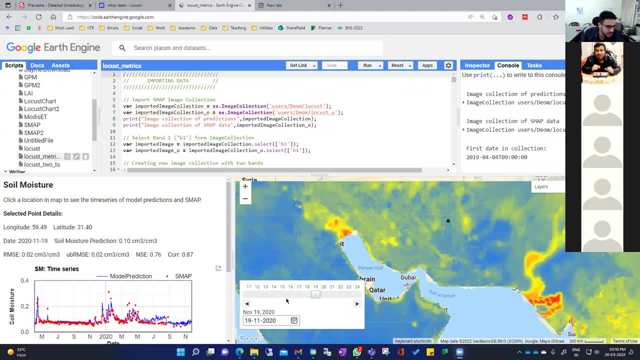 wherein we can change the dates, we can change the time, and then we can show change the time, and then we can show change the time and then we can show different uh rasters. so here what we did- different uh rasters. so here what we did- different uh rasters. so here what we did. we created this one: soil moisture. 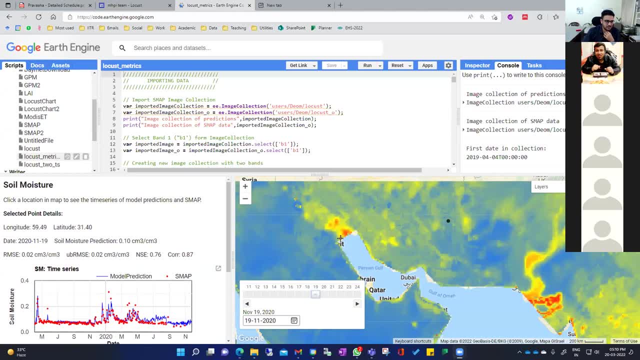 we created this one soil moisture. we created this one soil moisture forecasting tool which was for some forecasting tool, which was for some forecasting tool, which was for some middle east, middle east, middle east part and some parts of the part and some parts of the part and some parts of the south asia. 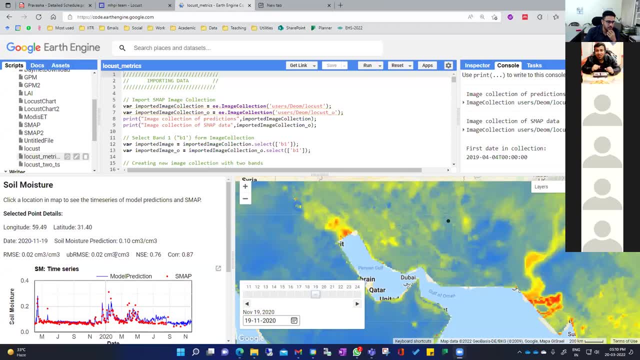 south asia, south asia, and in the backend, we had a deep learning and in the backend, we had a deep learning and in the backend we had a deep learning code which was working, which was making code which was working, which was making code which was working, which was making predictions: forecasts of soil moisture. 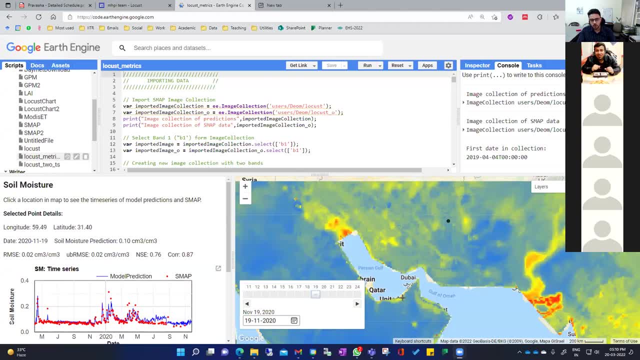 predictions: forecasts of soil moisture. predictions: forecasts of soil moisture over next 16 days. and those were over next 16 days and those were over next 16 days and those were automatically shown over this google. automatically shown over this google. automatically shown over this google earth engine app. 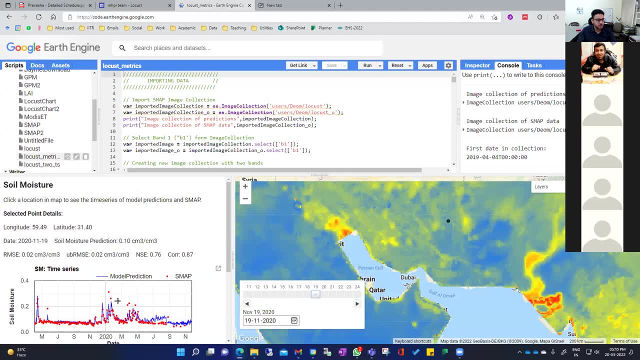 earth engine app. earth engine app- selected point on this map. it also further selected point on this map. it also further selected point on this map. it also further shows the shows: the shows the uh time series of the soil moisture at. uh time series of the soil moisture at. 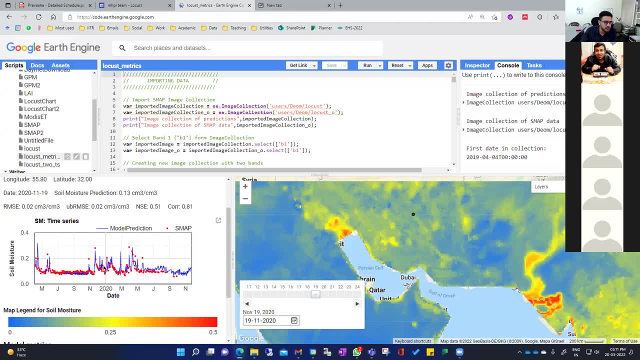 uh, time series of the soil moisture at that particular point and, as you see, i that particular point and, as you see, i that particular point and, as you see, i clicked on a different point and it clicked on a different point, and it clicked on a different point and it started generating the map for the 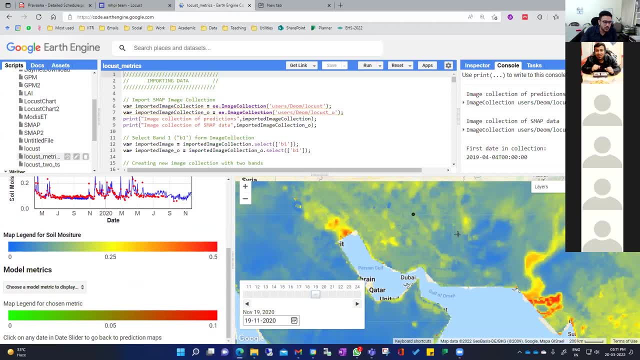 started generating the map for the, started generating the map for the different point. different point, different point, and then there is legend which shows, and then there is legend which shows, and then there is legend which shows this color, this color, this color schemes, and further you can choose. 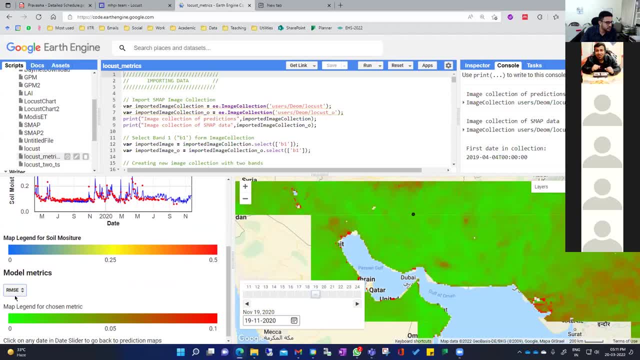 schemes, and further you can choose schemes, and further you can choose different different schemes, and further you can choose different colors that we had, and then colors that we had, and then colors that we had, and then, from this time, uh, slider, i can change. from this time, uh, slider, i can change. 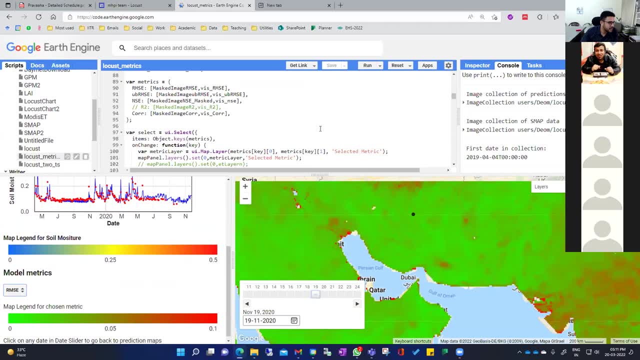 from this time. uh, slider, i can change the dates, the dates, the dates, although this code is very long, you can. although this code is very long, you can, although this code is very long, you can try some of the day, but the main. try some of the day, but the main. 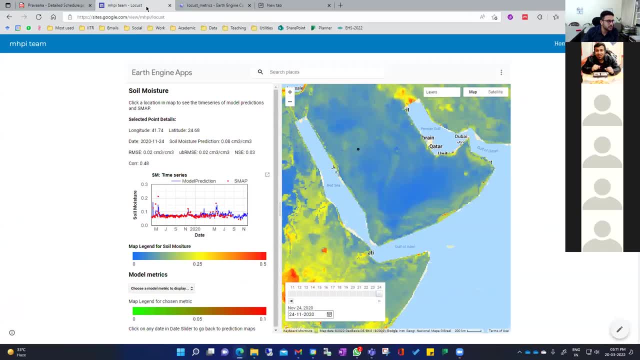 try some of the day, but the main advantage that we have, that we can advantage that we have that we can advantage that we have that we can integrate this with some other website, integrate this with some other website, integrate this with some other website. for example, this is a google. 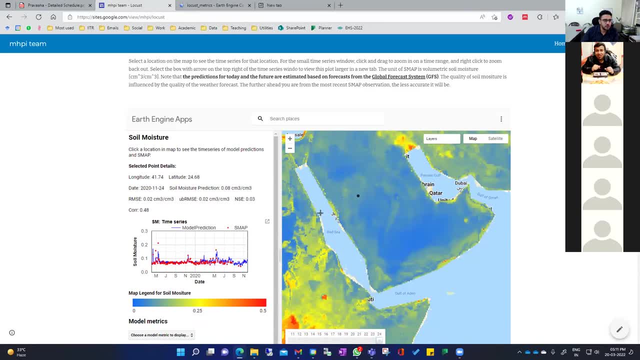 for example, this is a google. for example, this is a google- uh google website where we integrated uh google website, where we integrated uh google website, where we integrated this code. now, you will not look at what this code now, you will not look at what this code now, you will not look at what we wrote, but you will simply see this. 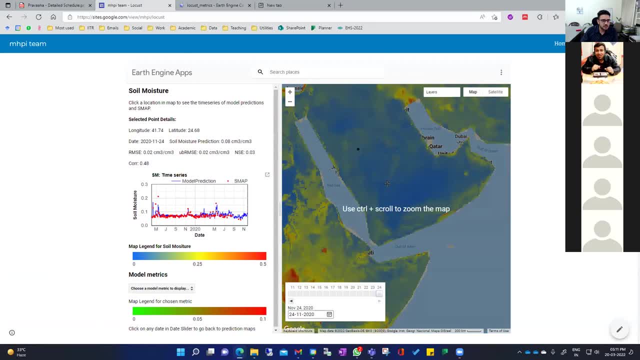 we wrote, but you will simply see this. we wrote, but you will simply see this, which will be updated automatically. which will be updated automatically, which will be updated automatically every day, every day, every day, and then by just scrolling here like a, and then by just scrolling here like a, 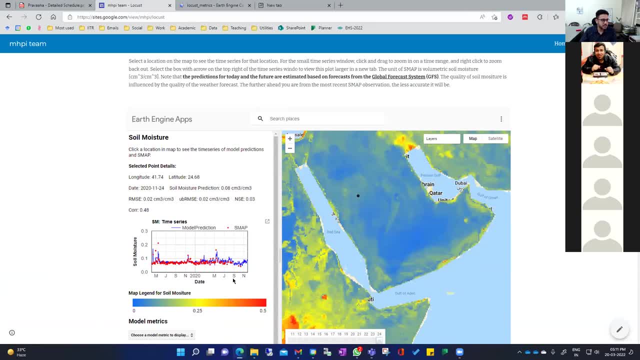 and then by just scrolling here, like a google map, you can google map. you can google map. you can show your results. you can show the show, your results. you can show the show, your results. you can show the forecast. in this case, we were showing forecast. in this case, we were showing. 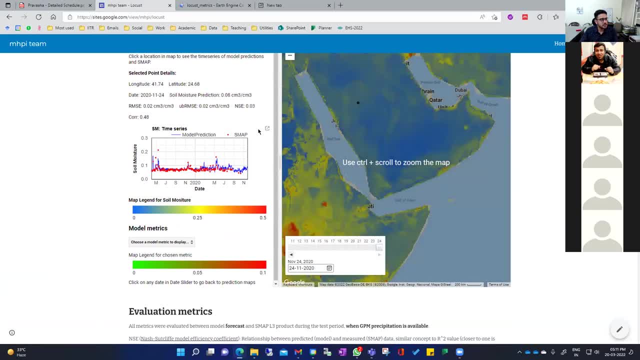 forecast. in this case, we were showing the forecast, the forecast, the forecast. you can also integrate these charts. you can also integrate these charts. you can also integrate these charts which can be exported, as you can told us, which can be exported, as you can told us which can be exported, as you can told us, we can export it to csb. we can further. 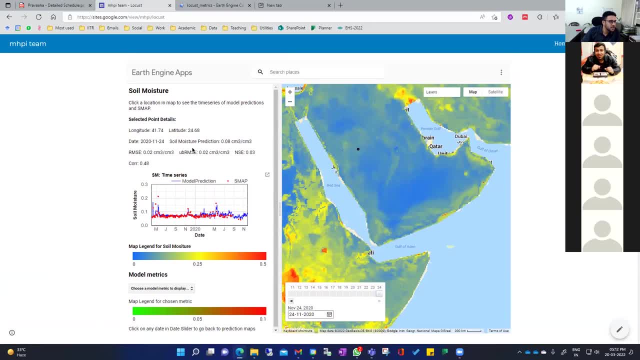 we can export it to csb. we can further. we can export it to csb. we can further add different elements. for example, here: add different elements. for example here, add different elements. for example: here we are, i think, showing the values of. we are, i think, showing the values of. 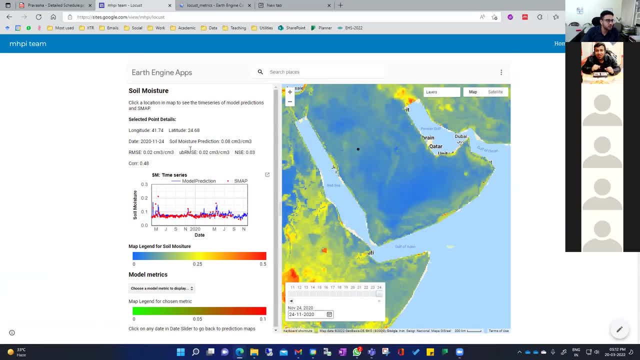 we are, i think, showing the values of rudman's care at different points. if we rudman's care at different points, if we rudman's care at different points, if we click somewhere at some other point, it click somewhere at some other point. it click somewhere at some other point. it will update it. 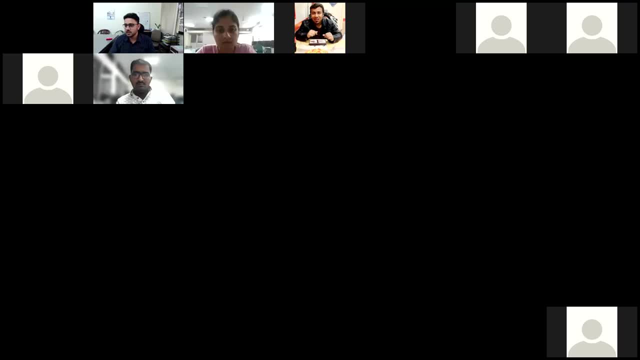 will update it, will update it. so those kind of things are also possible. so those kind of things are also possible. so those kind of things are also possible with google earth engine, and i would with google earth engine, and i would with google earth engine and i would, uh, encourage all the participants to. 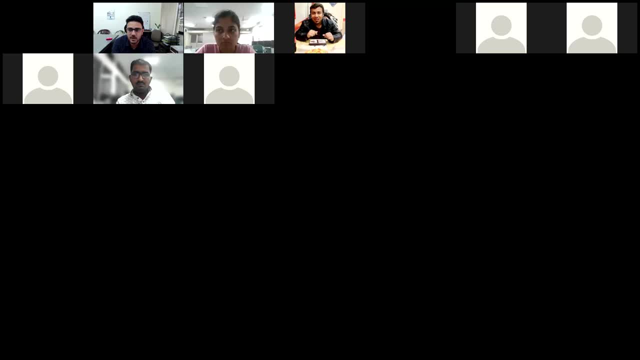 uh, encourage all the participants to uh, encourage all the participants to explore it further, because this is a kind, explore it further. because this is a kind, explore it further because this is a kind of new revolution in this field. where of new revolution in this field. where of new revolution in this field where google, we can use google's resources. 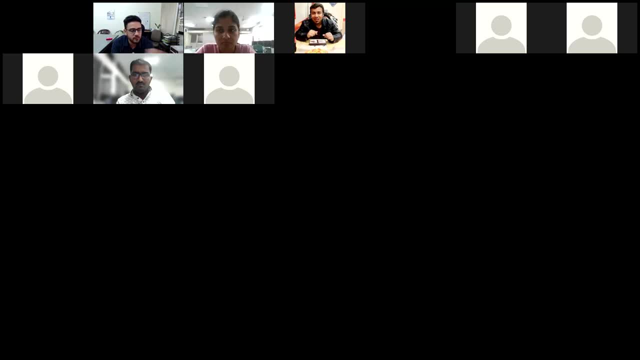 google, we can use google's resources, google, we can use google's resources, their storage, their computation, and we their storage, their computation, and we their storage, their computation, and we can produce these kind of tools, which can produce these kind of tools, which can produce these kind of tools, which will be very helpful. 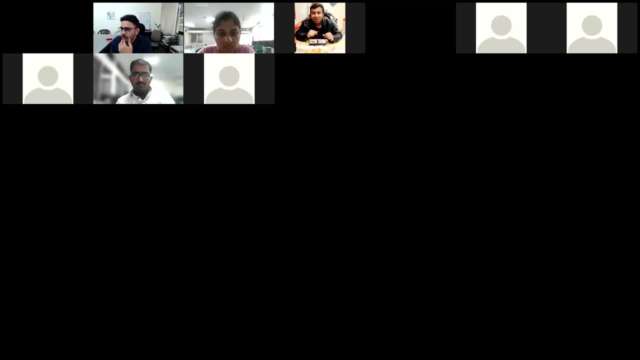 will be very helpful, will be very helpful. so, coming back to the question and so coming back to the question, and so coming back to the question and answer: uh, we have a couple of more answer. uh, we have a couple of more answer. uh, we have a couple of more questions. 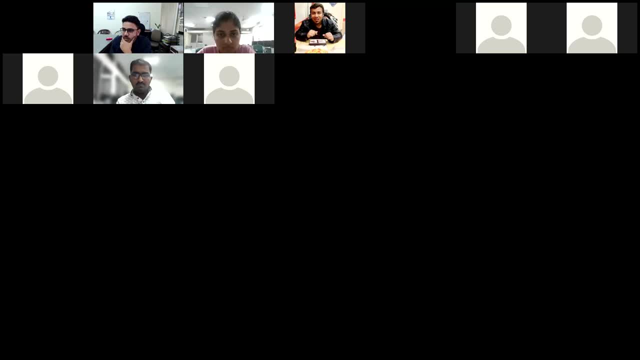 questions, questions. uh, there's one question by anand who is uh. there's one question by anand who is uh. there's one question by anand who is asking that. is it possible to develop asking that? is it possible to develop asking that? is it possible to develop distributed rainfall random model or? 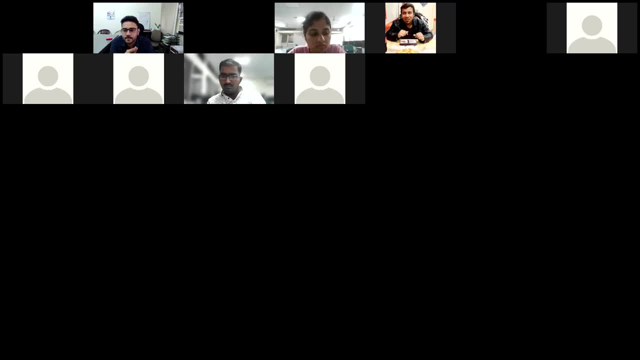 distributed rainfall- random model. or distributed rainfall- random model, or only semi-distributed models, only semi-distributed models, only semi-distributed models. so, as i told you that, so, as i told you that, so as i told you that it is actually preparing the curve number, it is actually preparing the curve number. 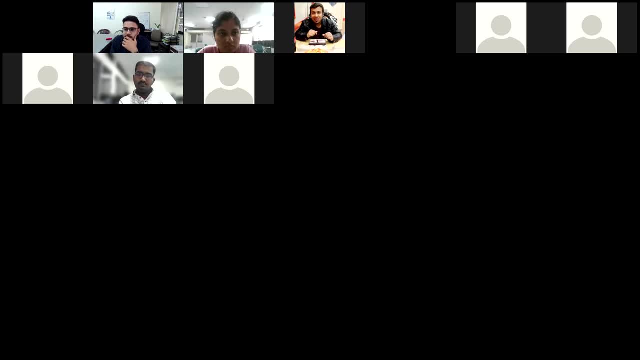 it is actually preparing the curve number on the pixel basis. so on the pixel basis, so on the pixel basis. so in hindi, in hindi, in hindi: okay because uh all the models that we okay, because, uh all the models that we okay, because, uh all the models that we have that either in hack hms. 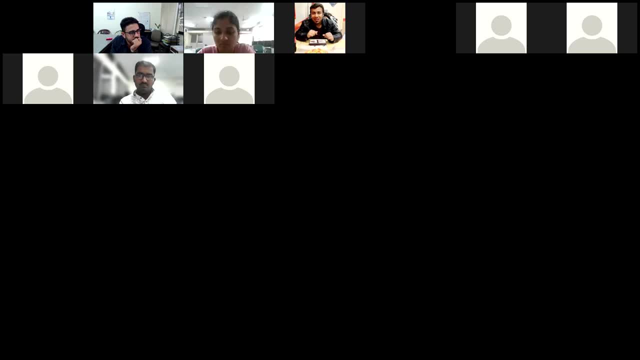 have that either in hack hms. have that either in hack hms. so what is doing? it is basically deriving. so what is doing? it is basically deriving. so what is doing? it is basically deriving the curve number on the subbasins. the curve number on the subbasins. 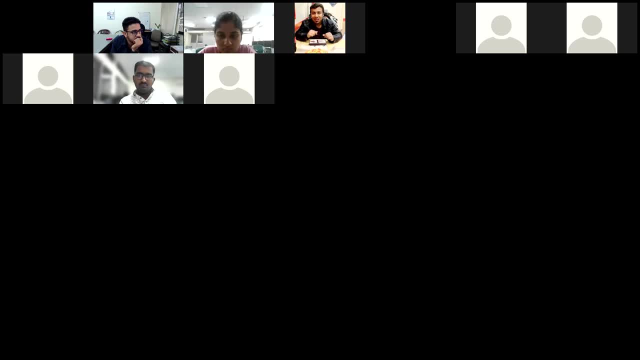 the curve number on the subbasins. sword model is also doing that thing. sword model is also doing that thing. sword model is also doing that thing, also in the vic model. we are actually also in the vic model. we are actually also in the vic model. we are actually preparing the grid of maybe one kilometer. 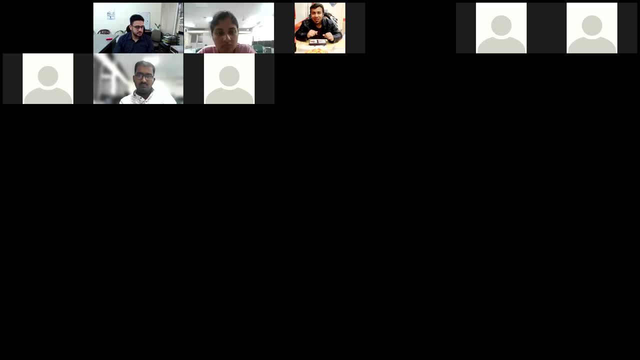 preparing the grid of maybe one kilometer, preparing the grid of maybe one kilometer or two kilometer, or two kilometer or two kilometer. uh, not, uh, lesser than that will be. uh, not, uh, lesser than that will be, uh, not, uh, lesser than that will be, created some problem in developing the. 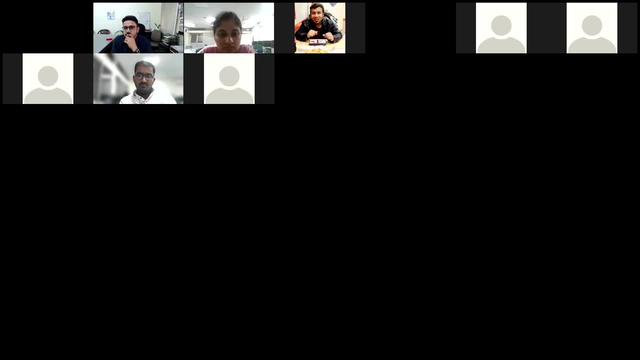 created some problem in developing the created some problem in developing the model. so i don't think so. there is model, so i don't think so. there is model, so i don't think so. there is anything which provide the curve number, anything which provide the curve number. 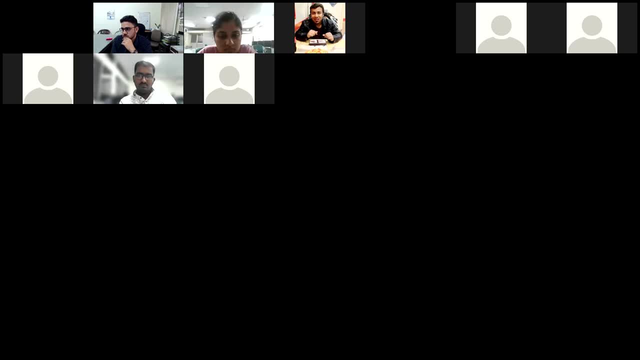 anything which provide the curve number, the model with at the pixel level, and it the model with at the pixel level and it the model with at the pixel level, and it is totally depend on the user data set, is totally depend on the user data set. is totally depend on the user data set. if you use the sentinel data, you will get. 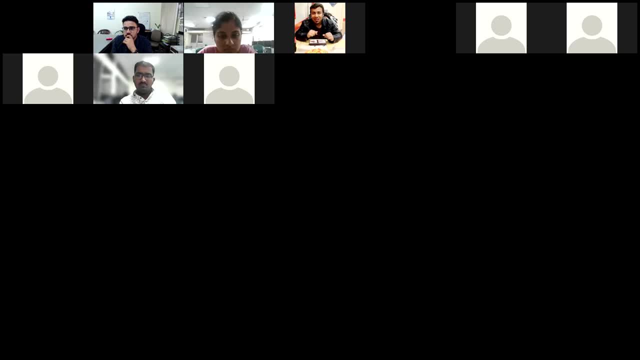 if you use the sentinel data, you will get. if you use the sentinel data, you will get the curve number at the 10 meter, the curve number at the 10 meter, the curve number at the 10 meter resolution, resolution resolution. so you can get the curve number at that. 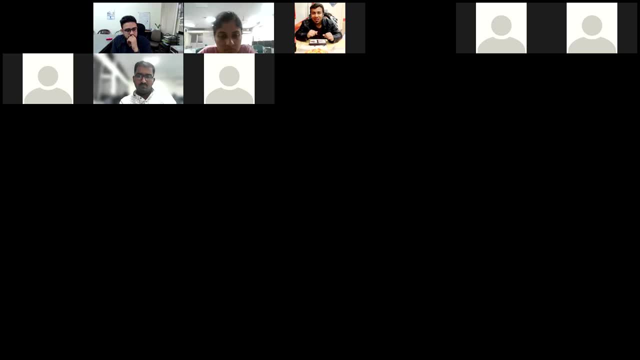 so you can get the curve number at that. so you can get the curve number at that level. also totally depend on the level, also totally depend on the level, also totally depend on the whatever the data you are using actually, whatever the data you are using actually, whatever the data you are using, actually great. so there's another question, uh. 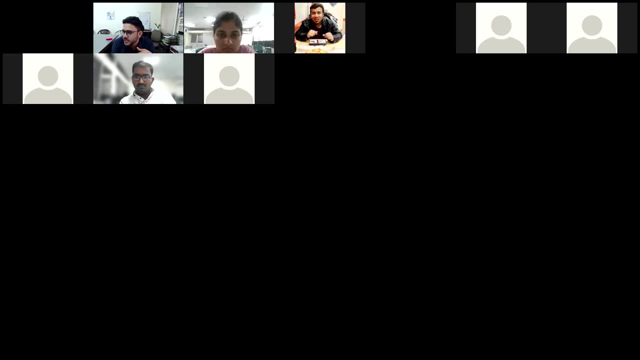 great, so there's another question. uh, great, so there's another question. uh, which is by? which is by? which is by? ganga nagri, who asked that my study area. ganga nagri, who asked that my study area. ganga nagri, who asked that my study area is less. i mean, i think he's referring to 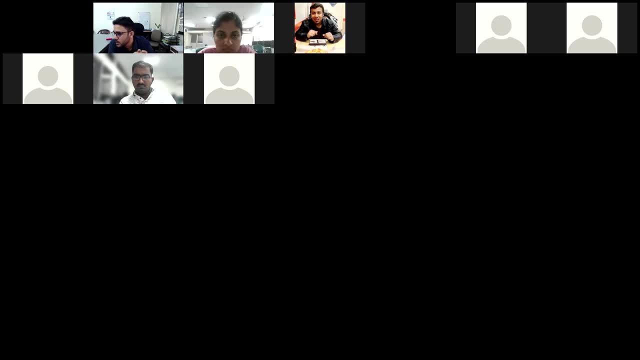 is less. i mean i think he's referring to is less. i mean i think he's referring to that his study area is small, so that his study area is small, so that his study area is small, so he's unable to classify lulc using. he's unable to classify lulc using. 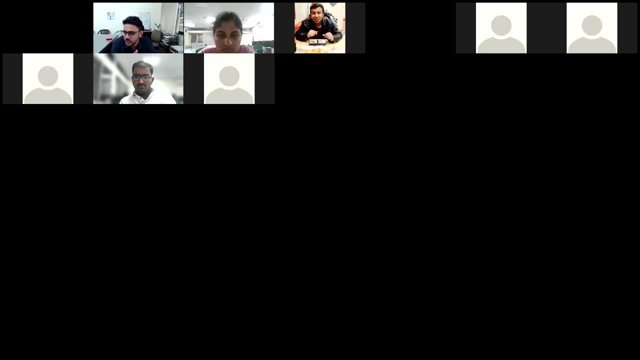 he's unable to classify lulc using google earth engine. so is there any google earth engine? so is there any google earth engine? so is there any method to do this classification for method, to do this classification for method, to do this classification for smaller areas, smaller areas? 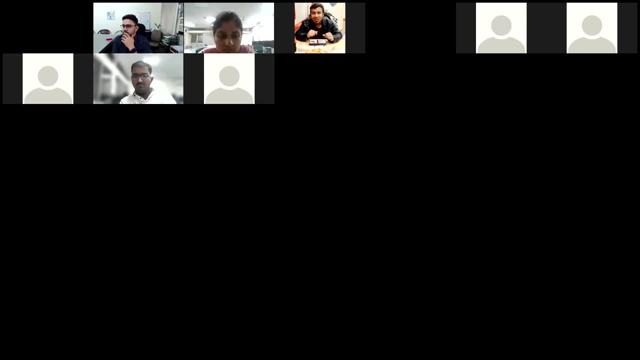 smaller areas. yes, there is a very uh. yes, there is a very uh. yes, there is a very uh, very good and very advanced machine. very good and very advanced machine, very good and very advanced machine. learning algorithms are there to classify learning algorithms are there to classify learning algorithms are there to classify, uh, your study area and if your study. 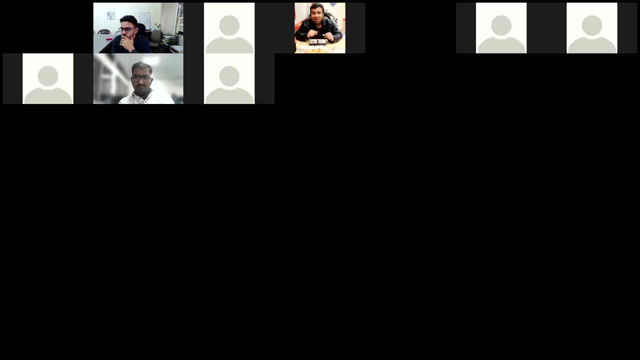 uh your study area and if your study uh your study area and if your study area is small, you can use the sentinel area is small. you can use the sentinel area is small. you can use the sentinel. two data set which has a 10 meter. two data set which has a 10 meter. 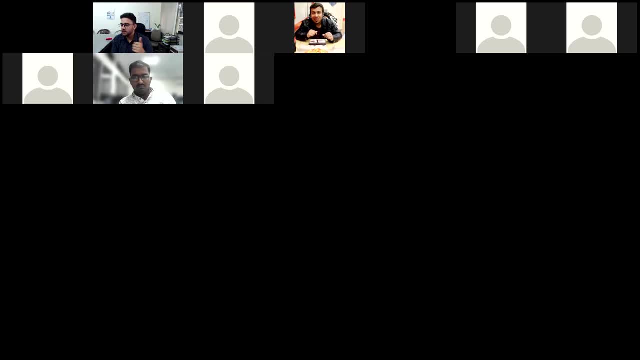 two data set which has a 10 meter uh hydrological model, uh hydrological model, uh hydrological model and there was a hand raised. i sorry i and there was a hand raised. i sorry i and there was a hand raised. i sorry i missed it. and then now i cannot see who. 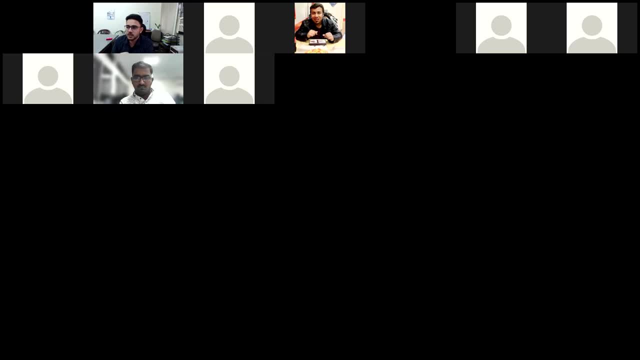 missed it and then now i cannot see who missed it and then now i cannot see who was it. so was it? so was it? so? if there is someone who wants to interact, if there is someone who wants to interact, if there is someone who wants to interact with shukant, please, 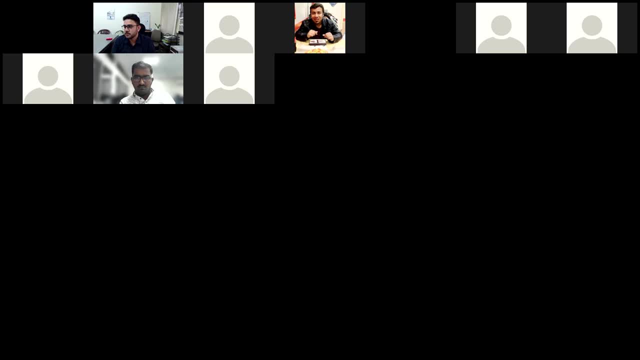 with shukant please. with shukant, please go ahead. okay, so we have another question. uh, okay, so we have another question. uh, okay, so we have another question. uh, shukant from bhanu parmar who is asking? shukant from bhanu parmar, who is asking? 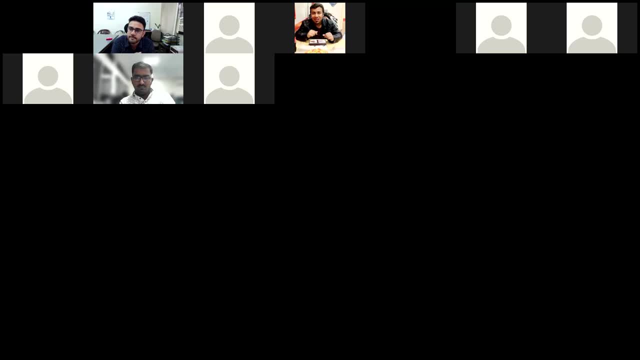 shukant from bhanu parmar who is asking that: can we use station data that? can we use station data that? can we use station data? uh, yes, bhanu, you can use the station. uh yes, bhanu, you can use the station. uh yes, bhanu, you can use the station. rainfall data into the oxygen. but 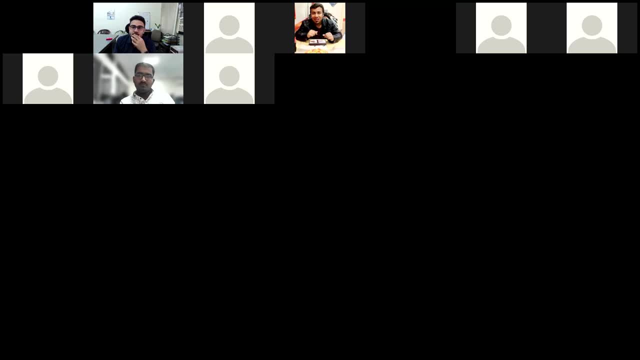 rainfall data into the oxygen. but rainfall data into the oxygen. but the conversion from station the, the conversion from station the, the conversion from station the excel data into the raster data is quite. excel data into the raster data is quite. excel data into the raster data is quite crumblesome. because 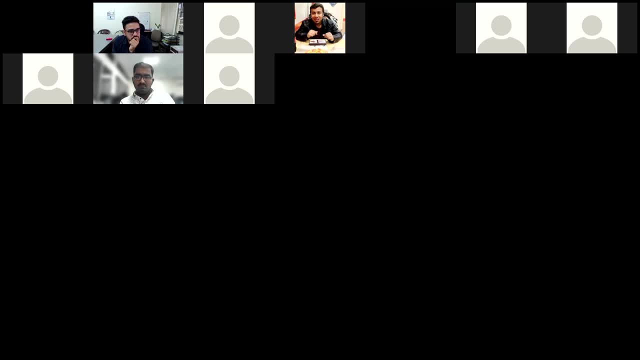 crumblesome because crumblesome because you have to convert first into the net. you have to convert first into the net. you have to convert first into the net cdf format, then in the net cdf format, cdf format, then in the net cdf format. 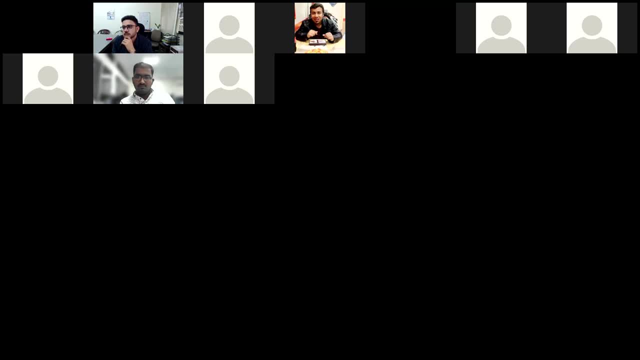 cdf format, then in the net cdf format you have to convert the geotiff, you have to convert the geotiff. you have to convert the geotiff. then in the geotiff the 365 geotiff for, then in the geotiff the 365 geotiff for. 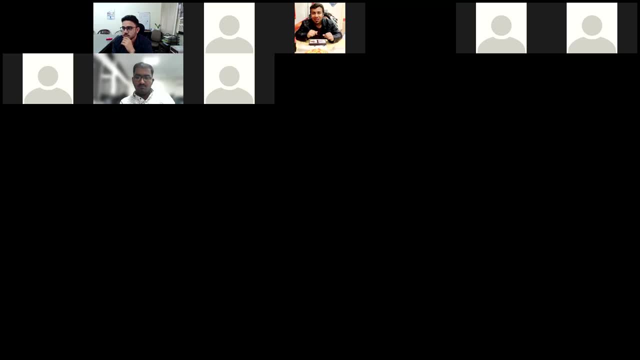 then in the geotiff, the 365 geotiff for a, a a single year. so you have to create n single year. so you have to create n single year, so you have to create n number of geotiffs, number of geotiffs, number of geotiffs. then only you can upload. but the good. 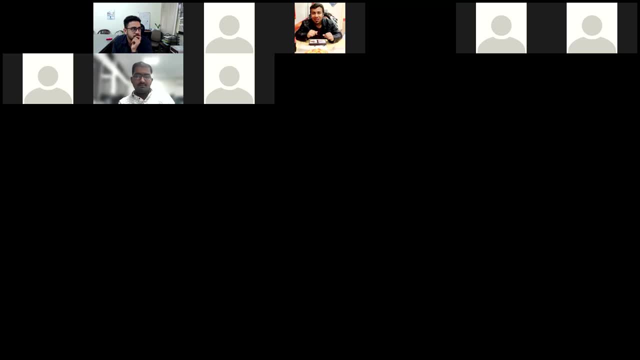 then only you can upload. but the good, then only you can upload. but the good thing is that if you are able to explore thing is that if you are able to explore thing is that if you are able to explore the python api of the earth engine, the python api of the earth engine, 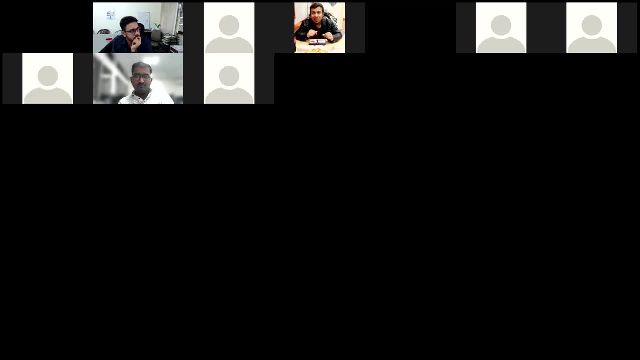 the python api of the earth engine, then it is going to be very easy for you, then it is going to be very easy for you. then it is going to be very easy for you. just you have to convert the curve, just you have to convert the curve. 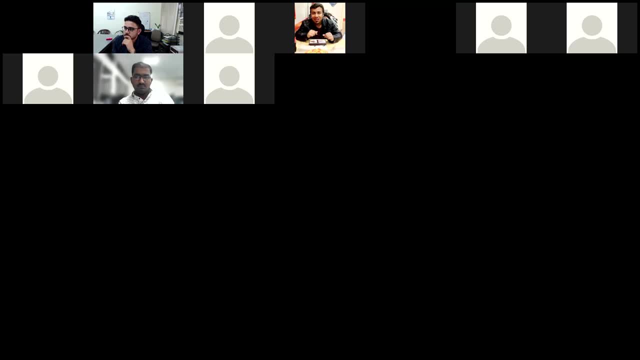 just, you have to convert the curve number number, number and bring that into your local geo. and bring that into your local geo. and bring that into your local geo: pandas data frame. pandas data frame, pandas data frame. and you can call the excel file of the. and you can call the excel file of the. 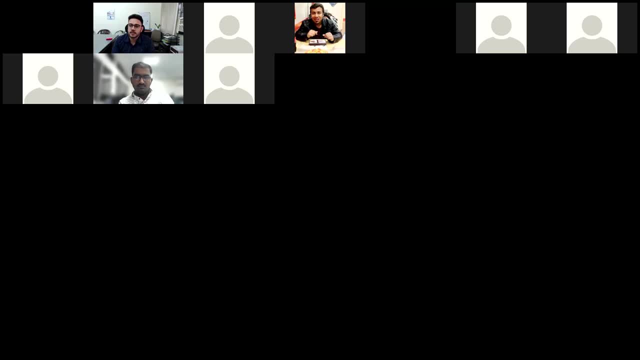 and you can call the excel file of the station data and you can club those two station data and you can club those two station data and you can club those two data set into your local machine, data set into your local machine, data set into your local machine. and then the thing is going to be very 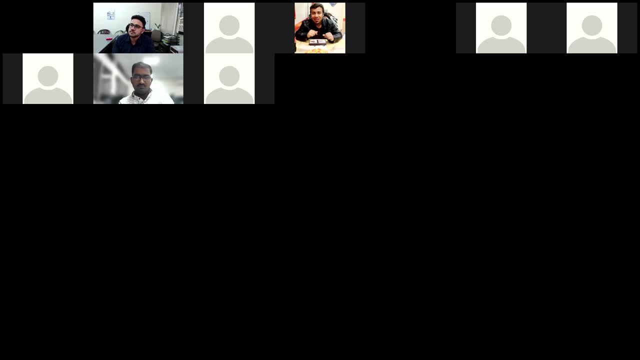 and then the thing is going to be very, and then the thing is going to be very much easy. that's why i've told you at much easy. that's why i've told you at much easy, that's why i've told you at the presentation that, as for a starter, 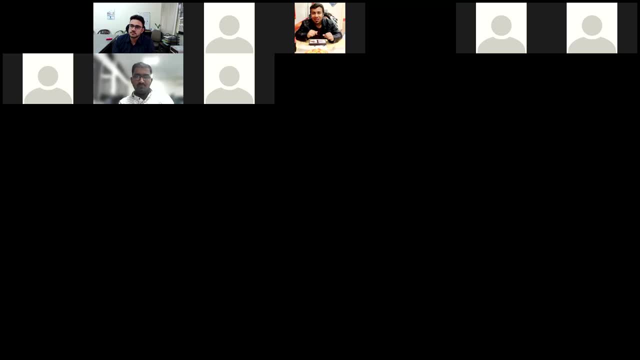 the presentation, that, as for a starter, the presentation, that, as for a starter, you have to stick into the javascript, you have to stick into the javascript, you have to stick into the javascript, but once you get very much familiar with, but once you get very much familiar with, 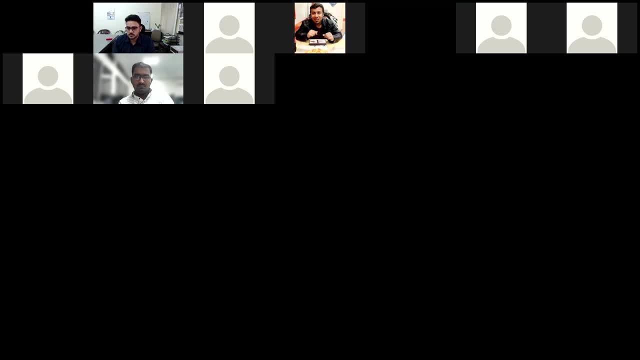 but once you get very much familiar with earth engine the data sets then you can earth engine the data sets, then you can earth engine the data sets, then you can easily switch to the python. and once you easily switch to the python, and once you easily switch to the python and once you switch to the python, 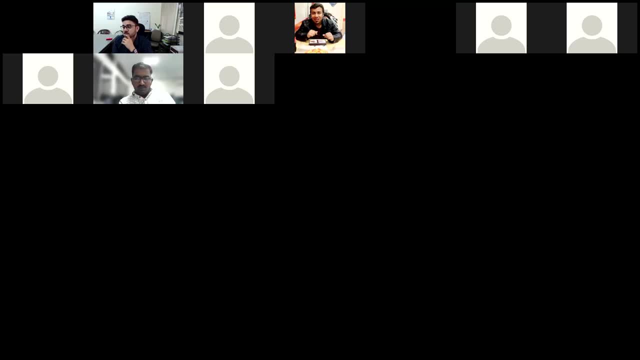 switch to the python. switch to the python uh. a new varieties of scope or new uh, a new varieties of scope or new uh, a new varieties of scope or new scope of things will be open for you. i think i answer the question. i think i answer the question. 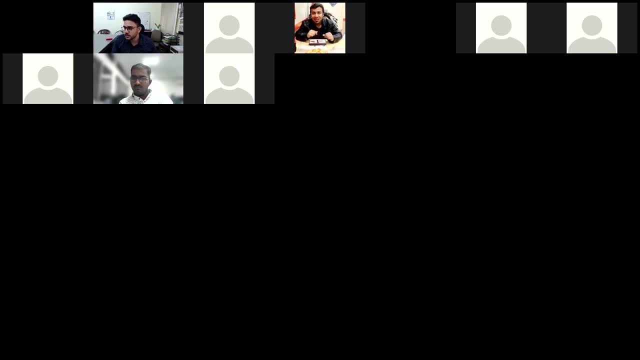 i think i answer the question according to my operating knowledge. according to my operating knowledge, according to my operating knowledge: yeah, i think that is great and i see we. yeah, i think that is great and i see we. yeah, i think that is great. and i see we have one more question coming in from. 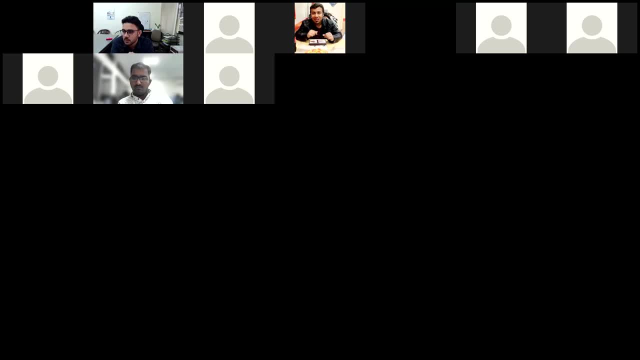 have one more question coming in from. have one more question coming in from: anand. do you want to ask it yourself, or anand do you want to ask it yourself or anand do you want to ask it yourself or do you want to? do you want to? 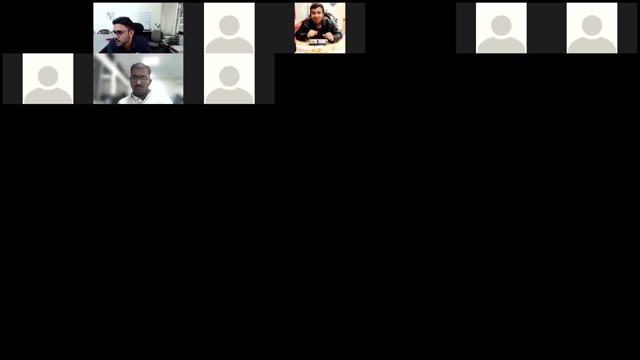 do you want to me to read it out? hello, hello, hello, hello, hello, hello, yes, yes, yes, yeah, i am asking that. can we use google? yeah, i am asking that. can we use google? yeah, i am asking that. can we use google or khanjin for prediction of lulc change? 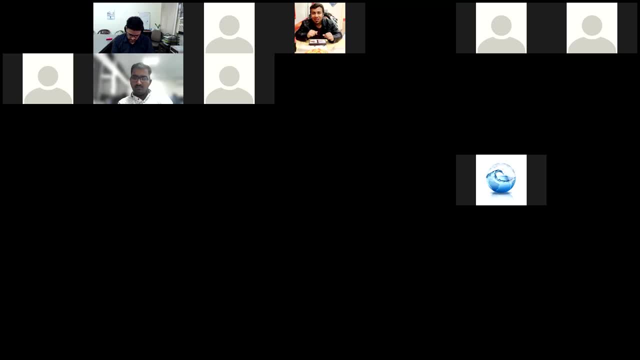 or khanjin for prediction of lulc change or khanjin for prediction of lulc change for future. for future. for future based on the past history of lulc or based on the past history of lulc or based on the past history of lulc or based on changes. 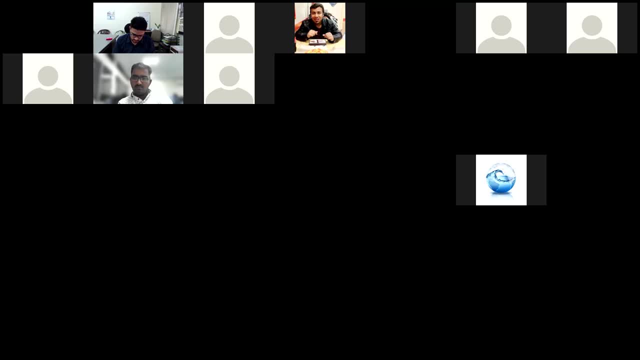 based on changes. based on changes: yes, anand. presently i don't know about yes, anand. presently i don't know about. yes, anand. presently i don't know about any algorithm that do this task, any algorithm that do this task, any algorithm that do this task, um, but i think there is a model, um. i 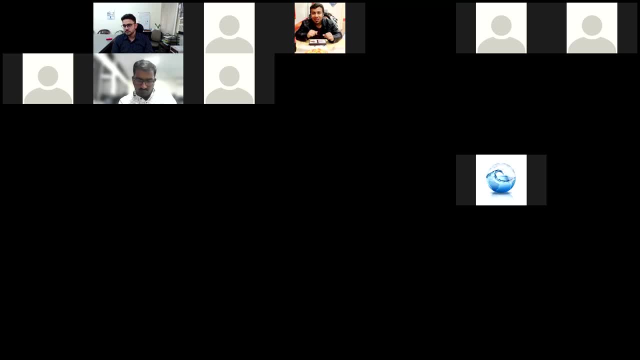 um, but i think there is a model um, i, um, but i think there is a model um- i don't remember its name- which do this, don't remember its name, which do this, don't remember its name- which do this task on a desktop. this is a desktop. 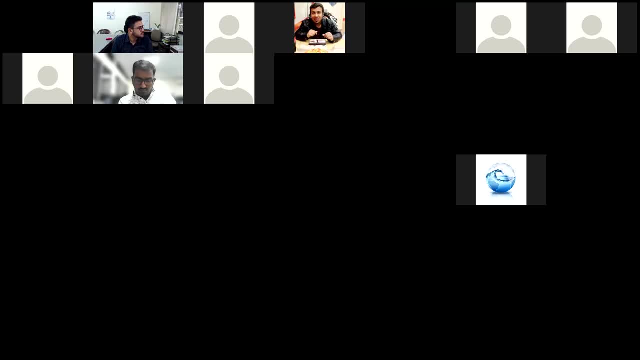 task on a desktop. this is a desktop task on a desktop. this is a desktop based, model based, model based model which incorporates the older lulc and which incorporates the older lulc and which incorporates the older lulc and gives the newer lulc the prediction loc. 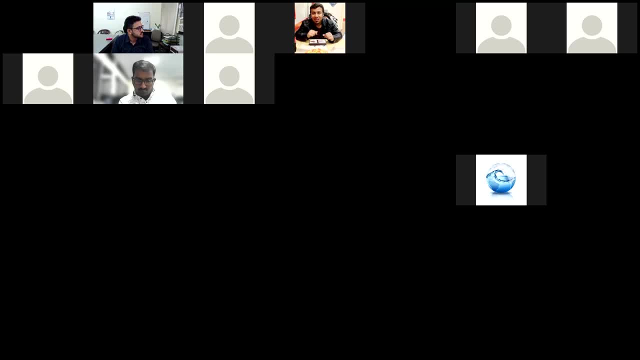 gives the newer lulc the prediction loc, gives the newer lulc the prediction loc. and if you are able to, and if you are able to, and if you are able to, incorporate the equations of those, incorporate the equations of those, incorporate the equations of those models into the earth engine. 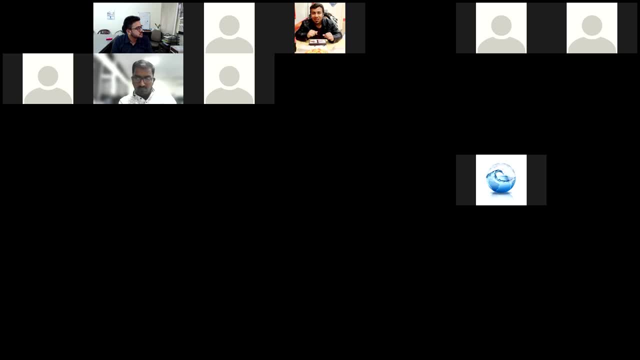 models into the earth engine, models into the earth engine, then only you can do this, then only you can do this, then only you can do this, or if in fact you can use some machine, or if in fact you can use some machine, or if in fact you can use some machine learning, calculations are there. 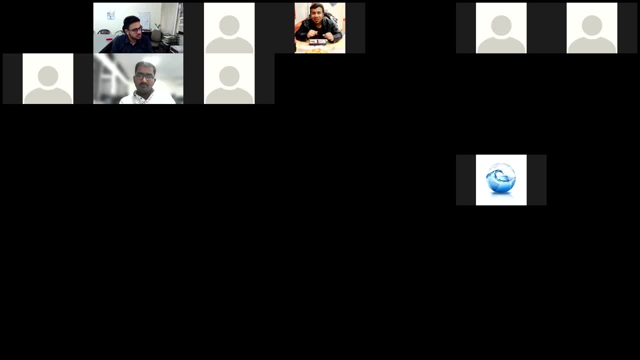 learning calculations. are there learning calculations? are there? uh to uh give the historical time series. uh to uh give the historical time series. uh to uh give the historical time series of lulc as an of lulc, as an of lulc as an inputs and get the latest time series. but 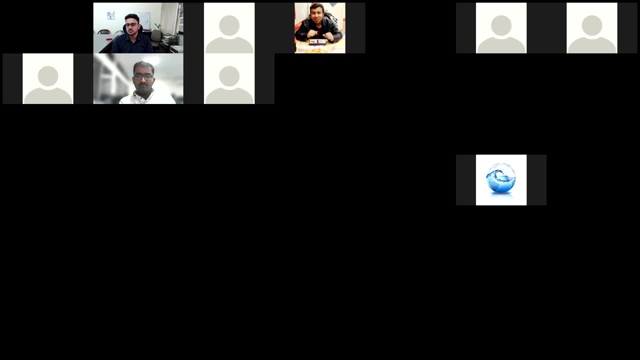 inputs and get the latest time series. but inputs and get the latest time series, but, uh, i don't know how the things will. uh, i don't know how the things will. uh, i don't know how the things will, but you have to go to some. but you have to go to some. 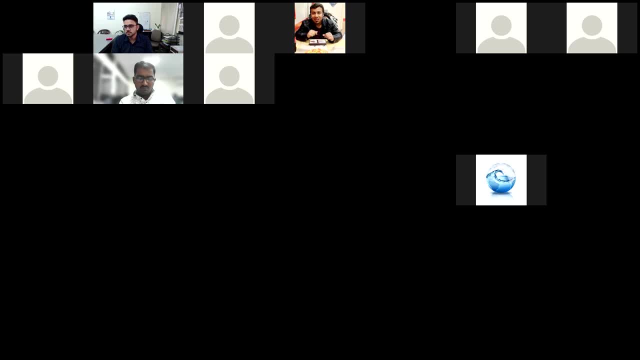 but you have to go to some what we can say to some literature, that what we can say to some literature, that what we can say to some literature that someone has done it, but yes, someone has done it. but yes, someone has done it. but yes, if the equation is there, if the 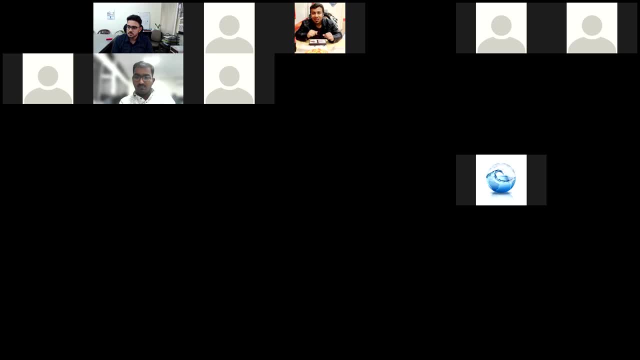 if the equation is there, if the, if the equation is there, if the algorithms there, then you can develop algorithms there. then you can develop algorithms there, then you can develop your own, your own, your own. okay, thank you so much. okay, thank you so much. okay, thank you so much. and yes, i think gagan deep has. and yes, i think gagan deep has. and yes, i think gagan deep has mentioned in the chat markov chain, mentioned in the chat markov chain, mentioned in the chat markov chain. modeling is one of the way in which we modeling is one of the way in which we. 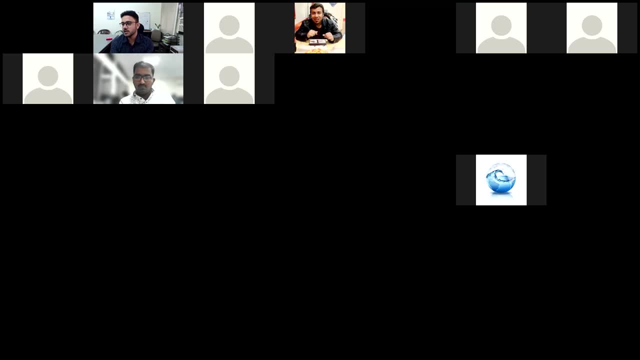 modeling is one of the way in which we can yes from the lulc prediction and i can yes from the lulc prediction and i can yes from the lulc prediction and i think there are many other well think. there are many other well think there are many other well established methods nowadays. 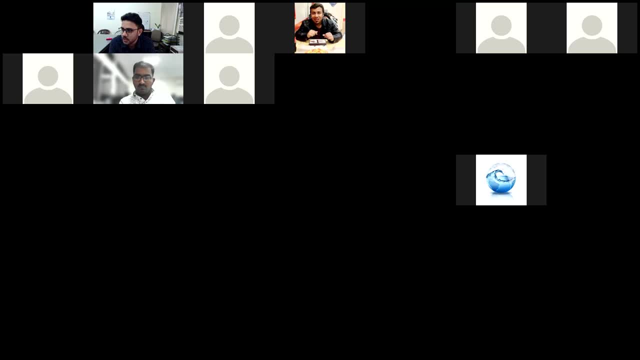 established methods nowadays, established methods nowadays which can be used for lulc prediction, which can be used for lulc prediction, which can be used for lulc prediction. the question is that, whether we can do. the question is that, whether we can do. the question is that whether we can do that on google earth engine or not. 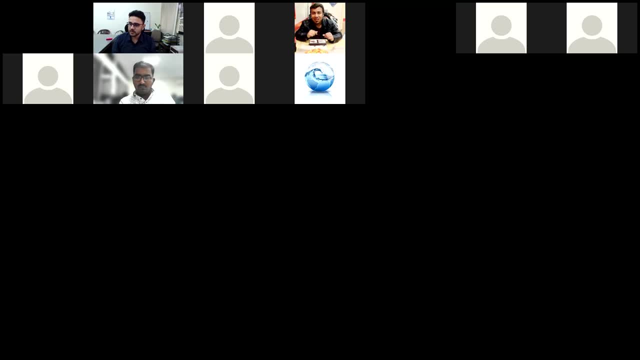 that on google earth engine or not. that on google earth engine or not would obviously depend on your coding. would obviously depend on your coding, would obviously depend on your coding skills and the capabilities that google skills and the capabilities that google skills and the capabilities that google earth engine offers. 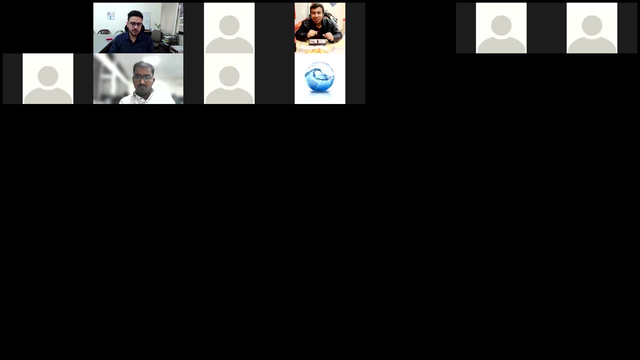 earth engine offers. earth engine offers. so i think we do not have any further. so i think we do not have any further, so i think we do not have any further questions. and we are already questions, and we are already questions, and we are already 20 minutes past our scheduled time. so 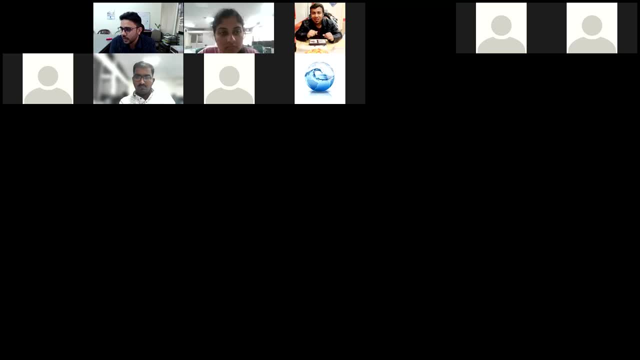 20 minutes past our scheduled time. so 20 minutes past our scheduled time. so we'll stop here, uh, and i would again. we'll stop here, uh, and i would again. we'll stop here, uh, and i would again. thank uh shukant. thank you very much for. 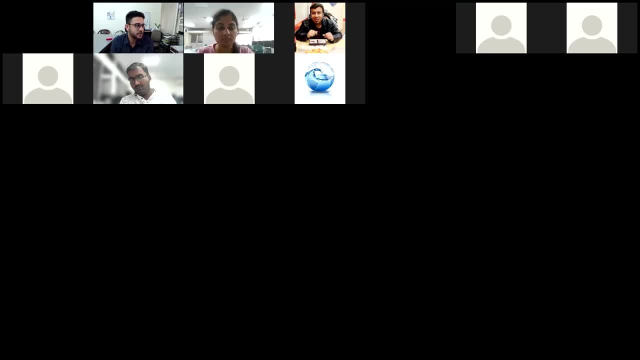 thank uh shukant. thank you very much for thank uh shukant, thank you very much for your valuable time. uh for this great your valuable time. uh for this great, your valuable time. uh for this great hands-on and the demonstration on google. hands-on and the demonstration on google. 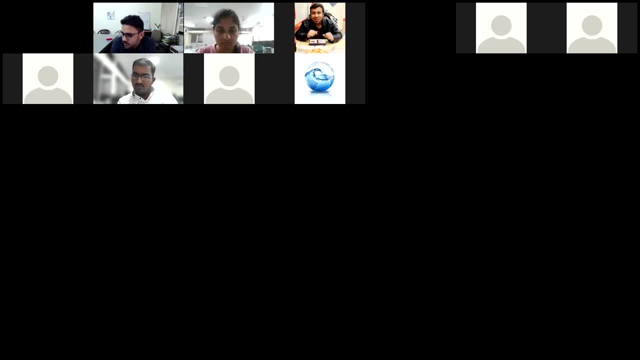 hands-on and the demonstration on google earth engine and i'm sure earth engine and i'm sure earth engine and i'm sure it will be very helpful for all the. it will be very helpful for all the, it will be very helpful for all the student participants in their research. 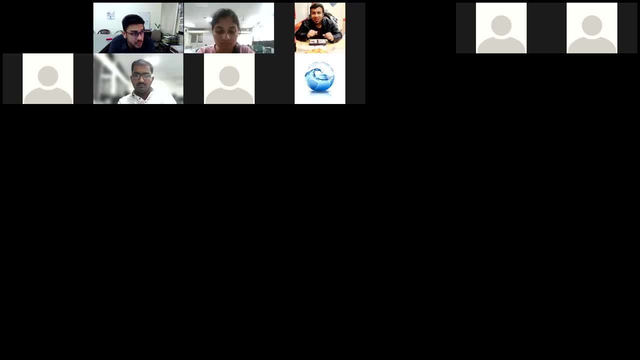 student participants in their research, student participants in their research work, work, work. google earth engine has already, uh, google earth engine has already uh. google earth engine has already uh provided us a lot of data sets which we provided us a lot of data sets which we provided us a lot of data sets which we cannot download on our computers. but 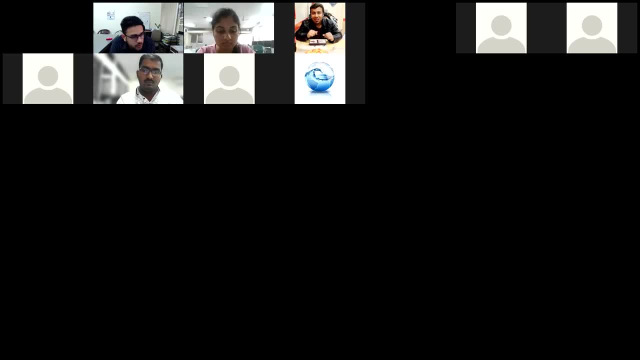 cannot download on our computers, but cannot download on our computers. but there you can analyze terabytes of data. there you can analyze terabytes of data. there you can analyze terabytes of data sets without having to download even sets, without having to download even sets, without having to download even single megabyte of data onto your 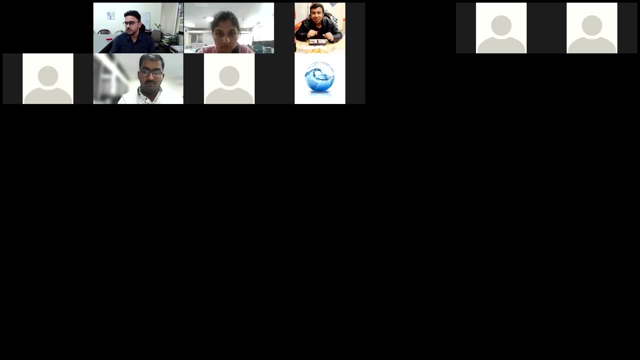 single megabyte of data onto your single megabyte of data onto your computer, computer, computer. so i'm sure your talk and demonstration, so i'm sure your talk and demonstration, so i'm sure your talk and demonstration will be uh very much helpful to the will be uh very much helpful to the. 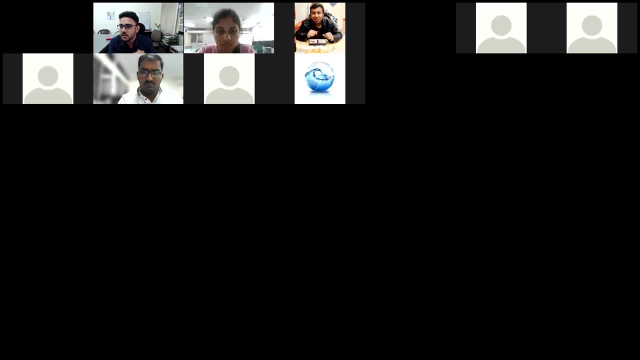 will be uh very much helpful to the students. one thing i want to ask: we had students. one thing i want to ask: we had students. one thing i want to ask: we had many uh questions in the chat. uh, many uh questions in the chat. uh many uh questions in the chat uh regarding sharing of this recording. so 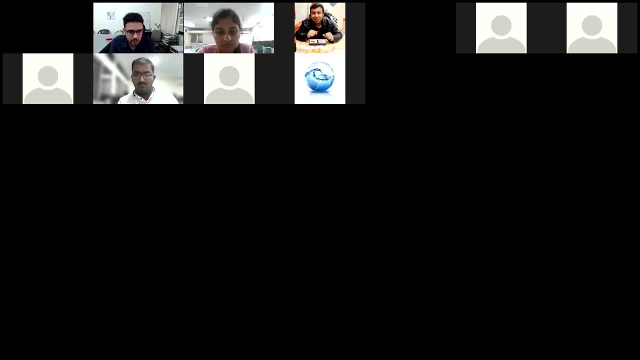 regarding sharing of this recording. so, regarding sharing of this recording. so if it is fine with you, can we, if it is fine with you, can we, if it is fine with you, can we? uh provide the recording of this session? uh provide the recording of this session. uh provide the recording of this session to the participants. 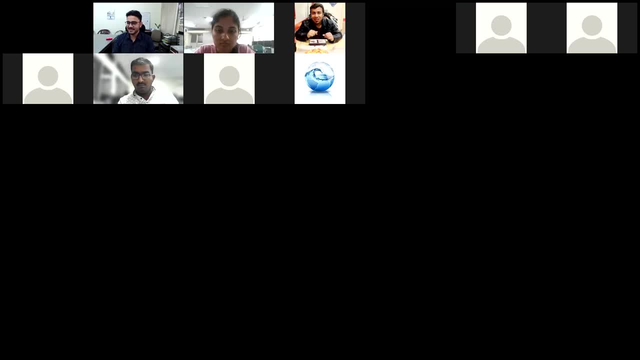 uh, yes, uh, there is no problem for my side. uh, yes, uh, there is no problem for my side. uh, yes, uh, there is no problem for my side. uh, you can, uh, you can uh, you can share this, or in fact, uh, share this, or in fact, uh. 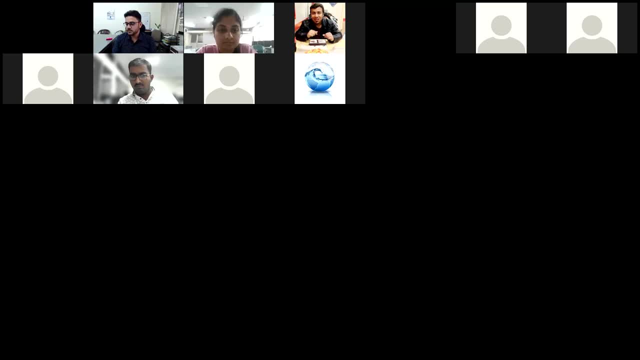 share this, or, in fact, uh, i think you have already shared your code. i think you have already shared your code. i think you have already shared your code, which is wonderful. i think, yes, yes, you, which is wonderful. i think, yes, yes, you, which is wonderful. i think, yes, yes, you get, the code is available in the public. 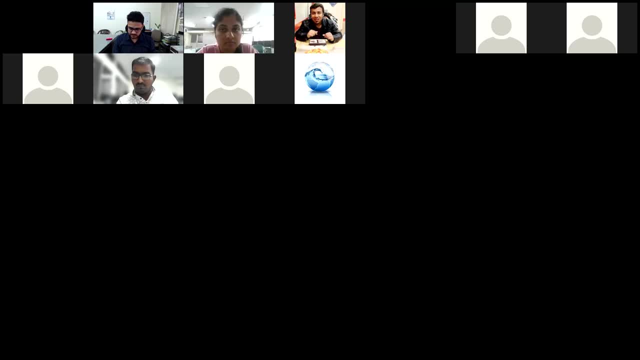 get the code is available in the public. get the code is available in the public domain. the good thing about this earth domain, the good thing about this earth domain, the good thing about this earth engine, is that most of the developers engine is that most of the developers. 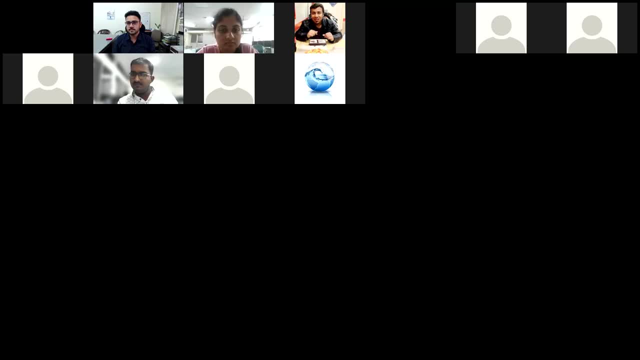 engine is that most of the developers are actually uh sharing their uh are actually uh sharing their uh are actually uh sharing their uh. research work in the open source domain, research work in the open source domain, research work in the open source domain. so, yes, my all the works, most of my works. so, yes, my all the works, most of my works. so, yes, my all the works, most of my works are in the open source domain. you can are in the open source domain. you can are in the open source domain. you can access my github account and through. access my github account and through. 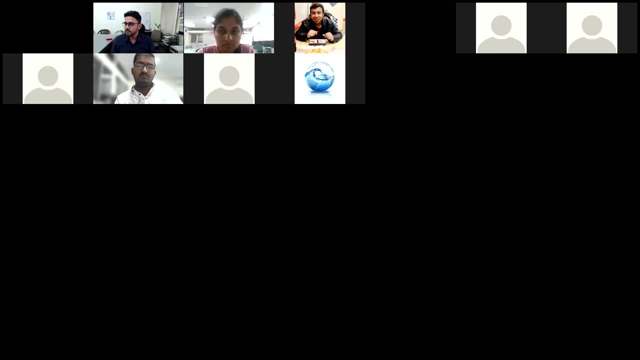 access my github account and, through github account, you can get to my youtube github account. you can get to my youtube github account. you can get to my youtube channel, through which there are some channel through which there are some channel through which there are some tutorials related to qgis and robert. 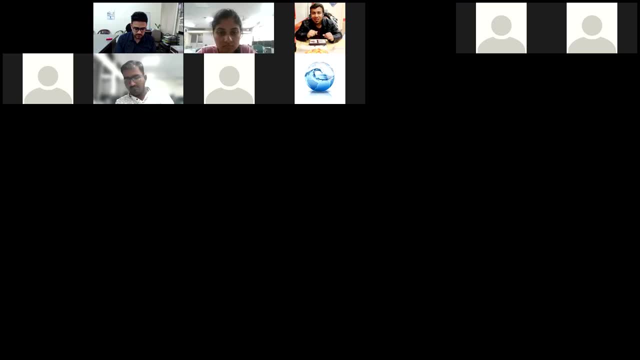 tutorials related to qgis and robert. tutorials related to qgis and robert engine. you can always access this and i engine you can always access this and i engine you can always access this and i will try, will try, will try, uh the uh to share this uh train and 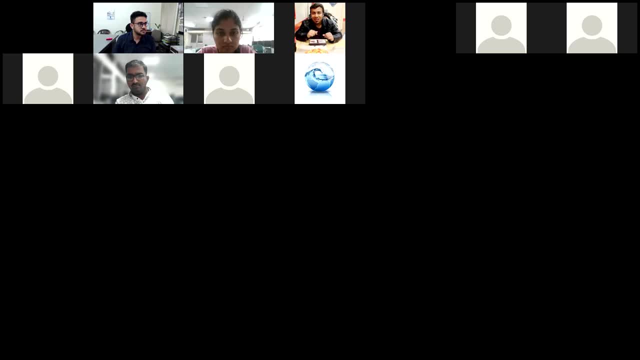 uh the uh to share this uh train and uh the uh to share this uh train. and this recording, this recording, this recording uh to all the participants also. uh, to all the participants also. uh, to all the participants also. or the anirudh, the coordinator, uh will. 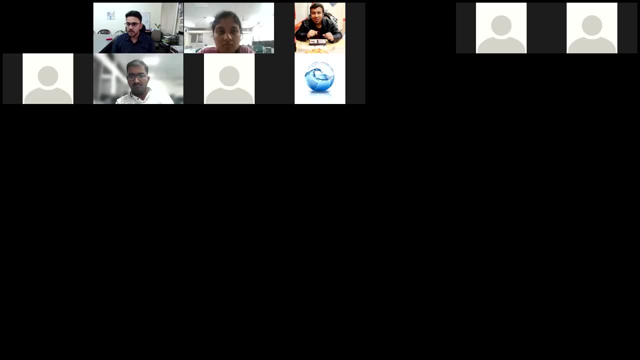 or the anirudh the coordinator uh will, or the anirudh, the coordinator uh will be be be sharing, the sharing, the sharing, the. yes, anirudh can, yes, anirudh can, yes, anirudh can interact with you later on, and then we 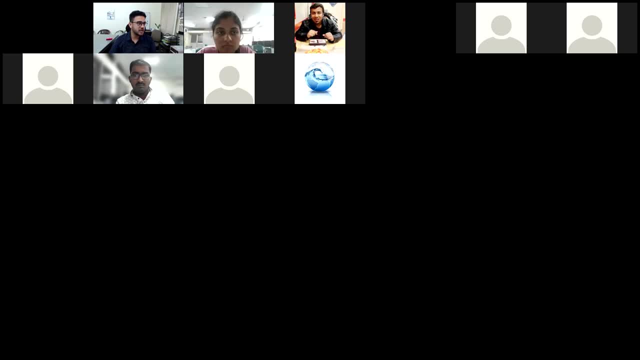 interact with you later on, and then we interact with you later on, and then we can discuss on how to share, can discuss on how to share, can discuss on how to share in the meanwhile. i just pasted the link in the meanwhile. i just pasted the link. 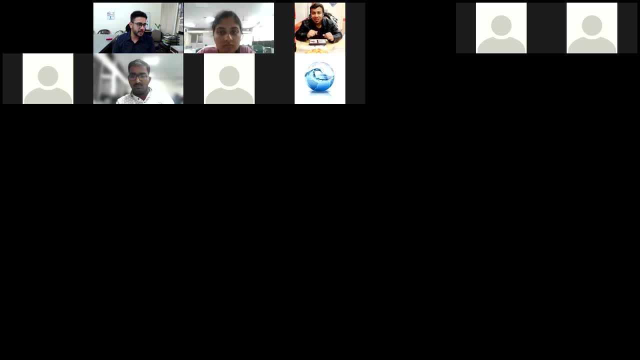 in the meanwhile i just pasted the link to shukan's github page. so participants to shukan's github page, so participants to shukan's github page, so participants can visit that page and they can can visit that page and they can can visit that page and they can look at all the public domain codes. 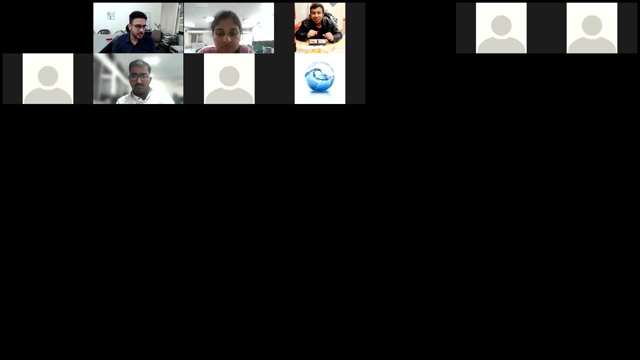 look at all the public domain codes. look at all the public domain codes which are shared by shukant and which are shared by shukant and which are shared by shukant, and probably they can use them and they can. probably they can use them and they can. 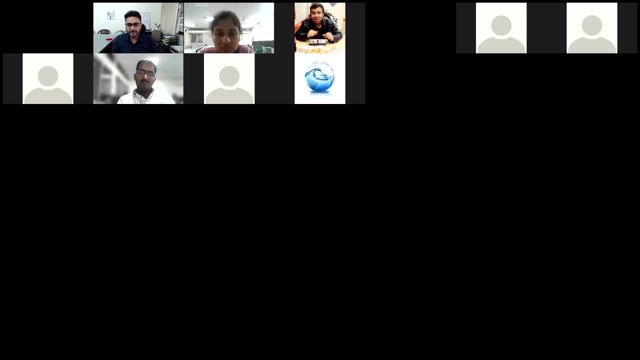 probably they can use them and they can interact further, interact further, interact further. you can suggest to improve uh all the you can suggest to improve uh all the you can suggest to improve uh all. the participants are requested to. participants are requested to. participants are requested to suggest me that how the 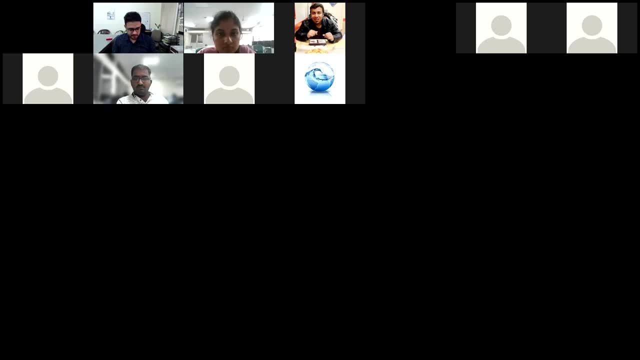 suggest me that, how the suggest me that how the, the open source sharing platform can be the open source sharing platform can be the open source sharing platform can be improved, improved, improved so that more followers will be there, so that more followers will be there, so that more followers will be there, yeah. 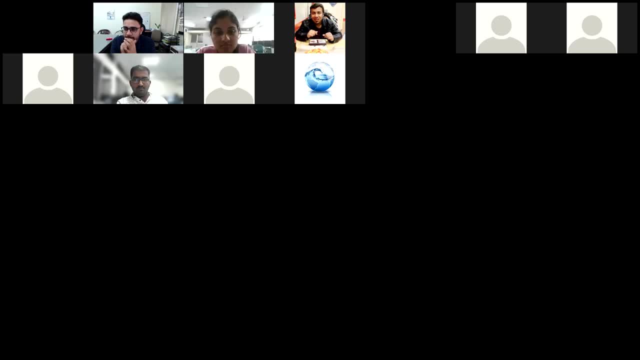 yeah, yeah, i would like to thank the uh. i would like to thank the uh. i would like to thank the uh prava team and dr ashutosh and all the prava team and dr ashutosh and all the prava team and dr ashutosh and all the student coordinator and hod. 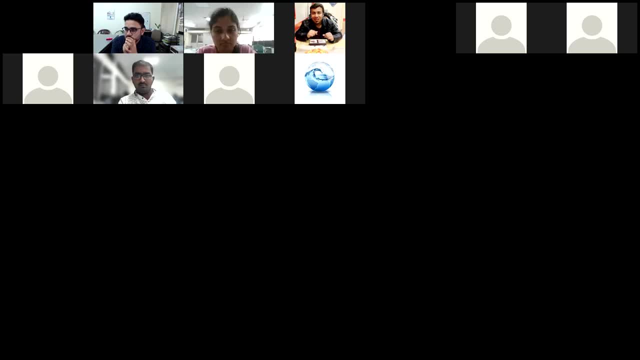 student coordinator and hod. student coordinator and hod for organizing uh this event, because it for organizing uh this event, because it for organizing uh this event, because it is very much, is very much, is very much useful uh to use this technology and the useful uh to use this technology and the. 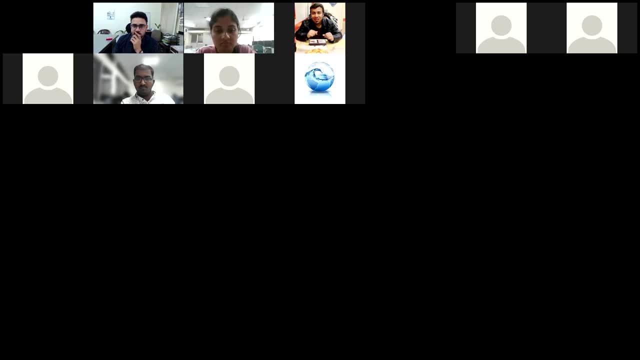 useful, uh, to use this technology and the participant has to understand. the google participant has to understand. the google participant has to understand. the google engine is just a tool. engine is just a tool. engine is just a tool and it has to be linked to your and it has to be linked to your. 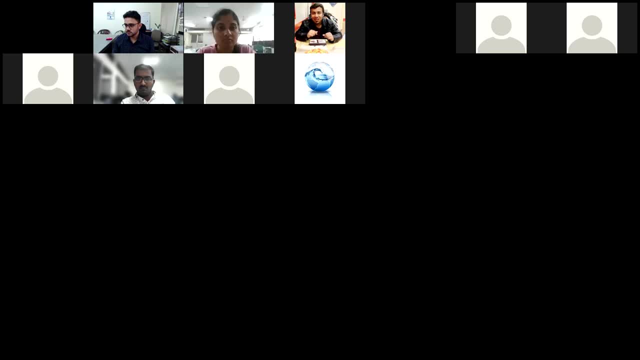 and it has to be linked to your imagination. okay, it has to be linked to imagination. okay, it has to be linked to imagination. okay, it has to be linked to your own perseverance. how to utilize your own perseverance? how to utilize your own perseverance, how to utilize this tool. 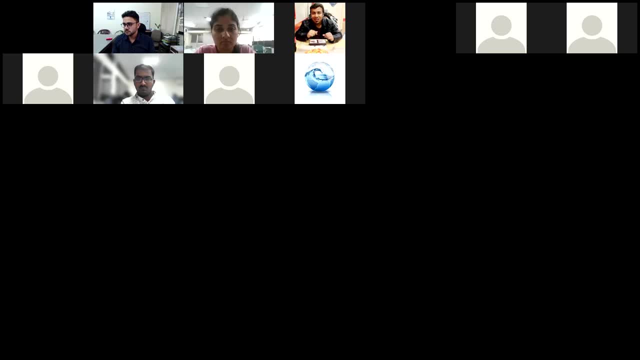 this tool, this tool in exploring n number of things? yes, so, as shushant mentioned, there are. yes, so, as shushant mentioned, there are. yes, so, as shushant mentioned, there are many possibilities, even many possibilities, even many possibilities, even, uh, many of the things on google earth. 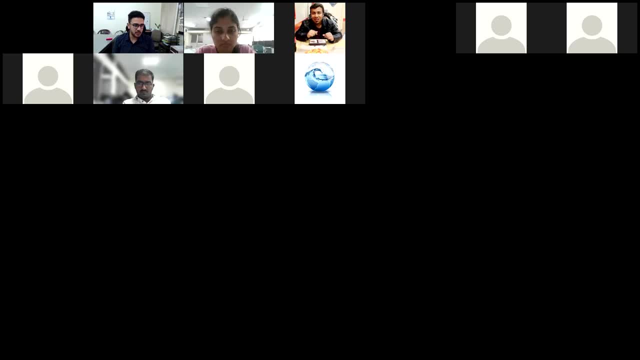 uh, many of the things on google earth, uh, many of the things on google earth engine are not engine, are not engine, are not fully explored yet. so there's a lot of fully explored yet. so there's a lot of fully explored yet. so there's a lot of possibility. 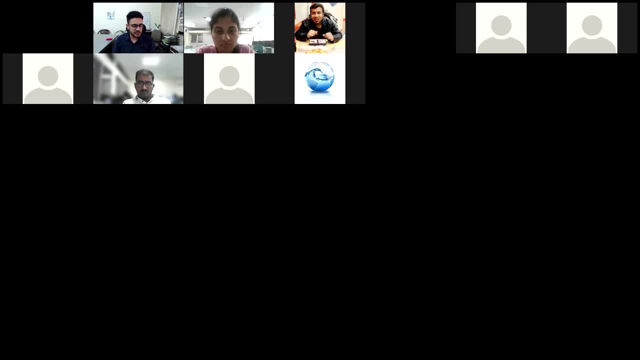 possibility. possibility that students can do many innovative, that students can do many innovative, that students can do many innovative projects. utilize different kind of data projects. utilize different kind of data projects, utilize different kind of data sets, integrate them, sets, integrate them sets, integrate them and make the apps that google earth. 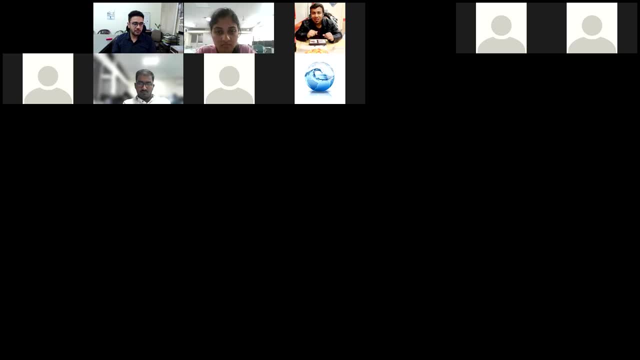 and make the apps that google earth and make the apps that google earth engine app that i showed you. that was one engine app that i showed you. that was one engine app that i showed you. that was one very small example, but people have very small example, but people have. 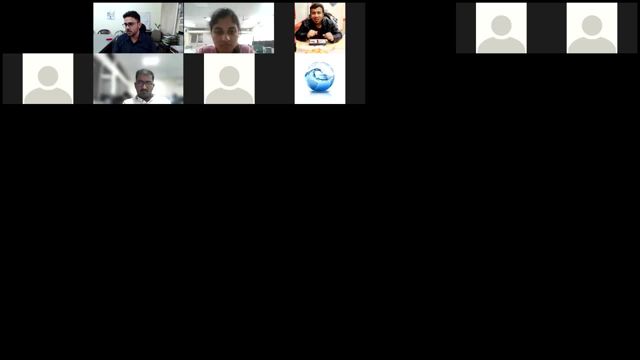 very small example, but people have developed very advanced apps on google, developed very advanced apps on google, developed very advanced apps on google earth engine, which can enable a lot of earth engine, which can enable a lot of earth engine, which can enable a lot of things, especially in terms of real-time. 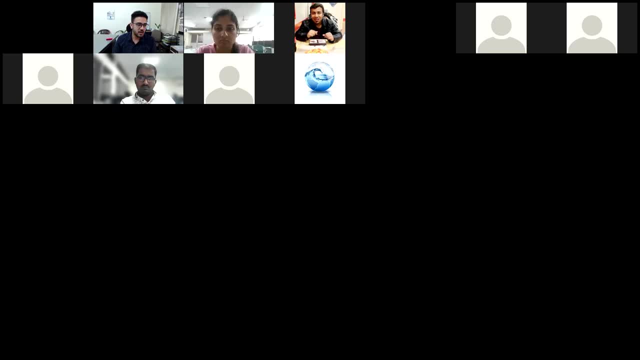 things, especially in terms of real-time things, especially in terms of real-time predictions of the thing, the real-time predictions of the thing, the real-time predictions of the thing, the real-time forecast of the different hydrological forecast, of the different hydrological forecast of the different hydrological variables, and that could be something. 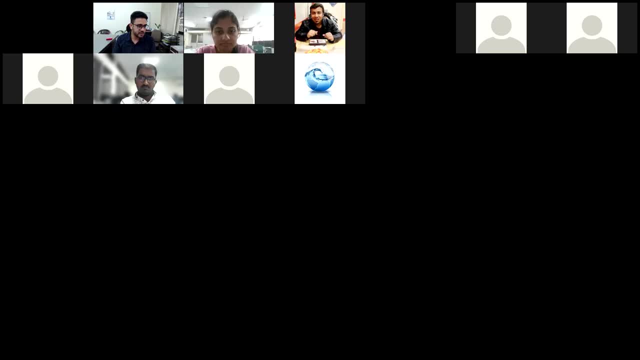 variables and that could be something. variables and that could be something. probably after this hands-on we'll see, probably after this hands-on we'll see, probably after this hands-on we'll see many of our students, many of our students, many of our students, using these tools for their projects. 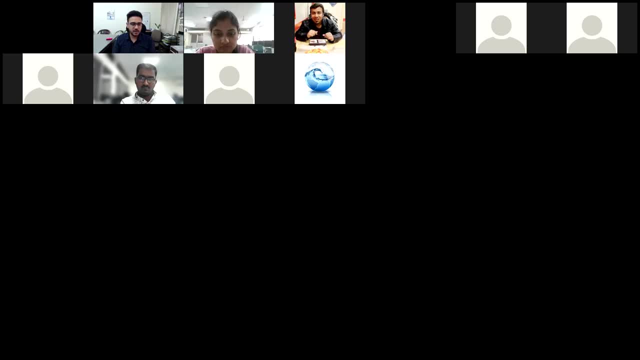 using these tools for their projects, using these tools for their projects. so, with this, i think we have uh reached. so, with this, i think we have uh reached. so with this, i think we have uh reached at the end of day one of this prabhaha, at the end of day one of this prabhaha. 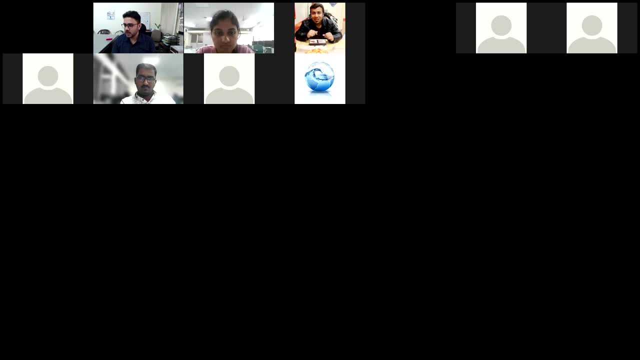 at the end of day one of this prabhaha, wherein we had two wonderful workshops, wherein we had two wonderful workshops, wherein we had two wonderful workshops. today in the morning, we had a workshop. today in the morning, we had a workshop. today in the morning, we had a workshop on tu flow, and now we had this wonderful 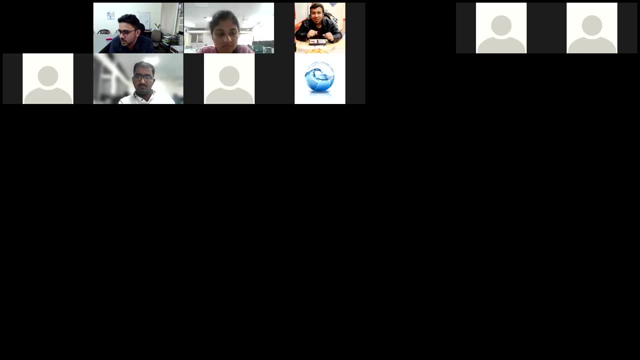 on tu flow, and now we had this wonderful on tu flow, and now we had this wonderful uh talk as well as a hands-on session by uh talk, as well as a hands-on session by uh talk, as well as a hands-on session by shukant on google earth engine. 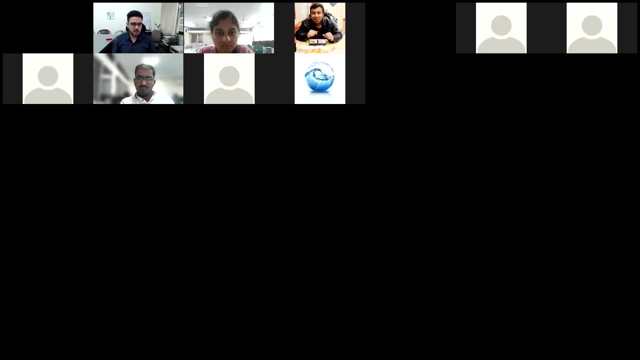 shukant on google earth engine. shukant on google earth engine. so i think we can now conclude, professor. so i think we can now conclude professor. so i think we can now conclude professor berchesh, berchesh, berchesh, if you want to add some concluding